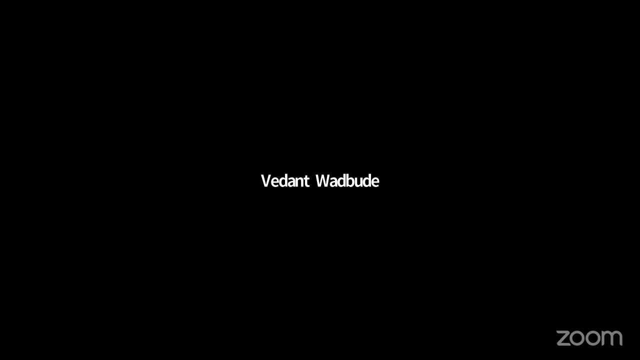 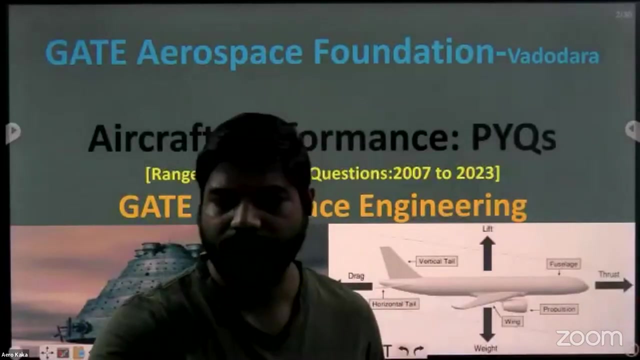 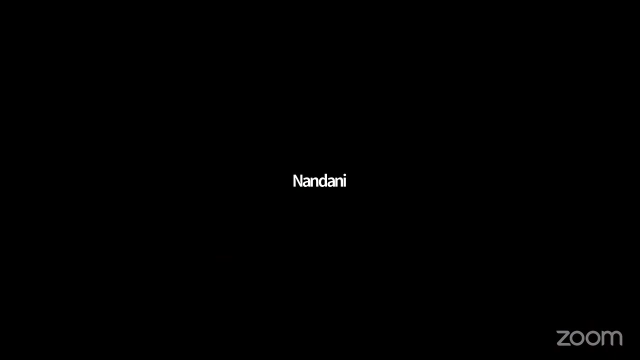 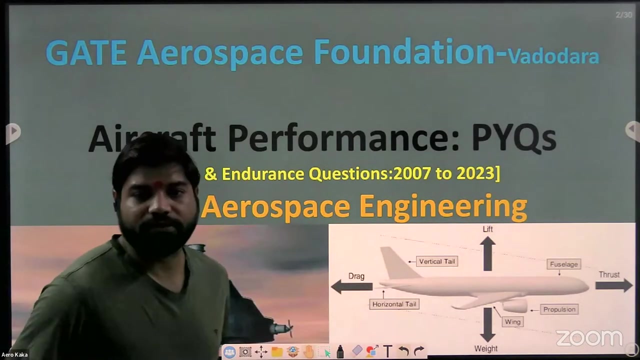 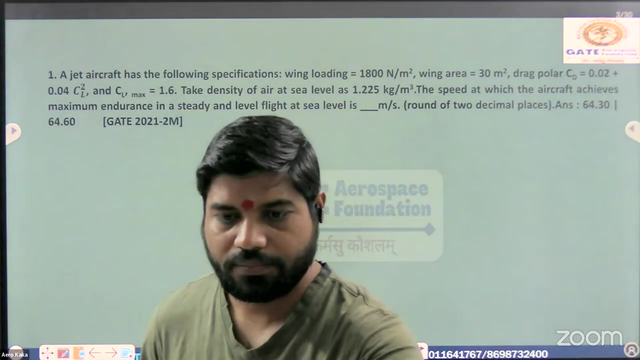 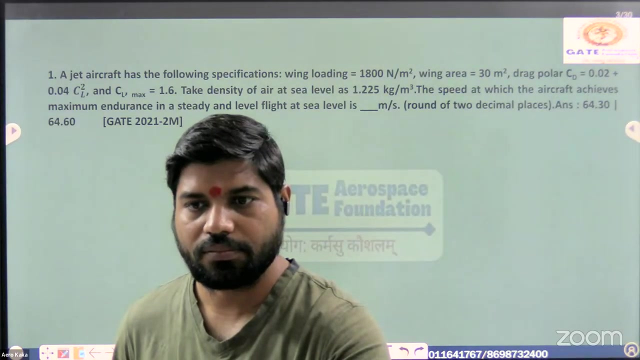 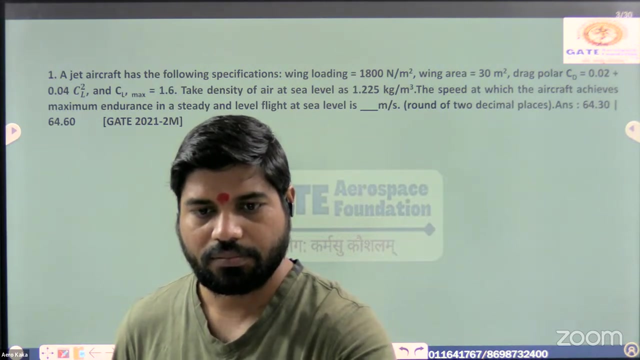 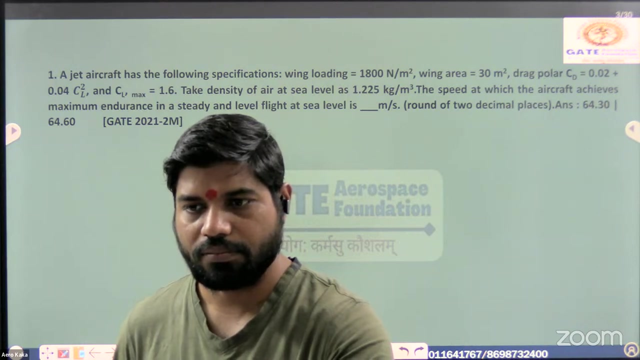 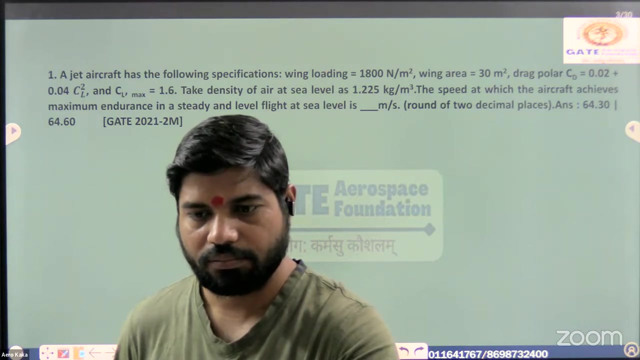 Thank you. Thank you, Hello, Hello. Can you hear me okay? Can you hear me Yes, Okay, Okay. so today we are starting just friends and endurance problems. problem again Something wrong. Can you check, please? Okay. 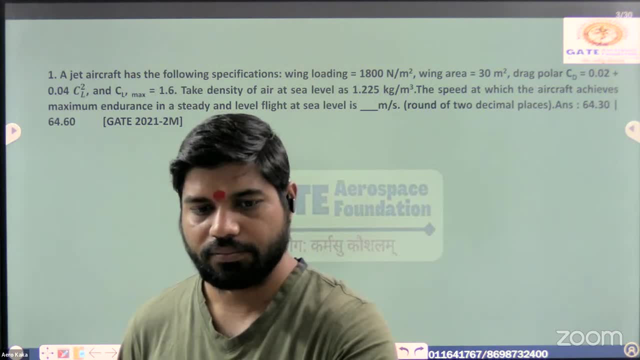 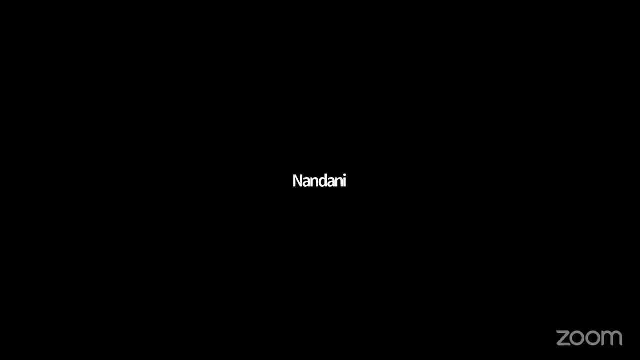 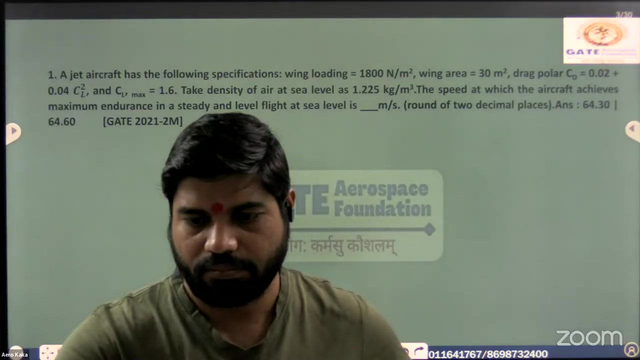 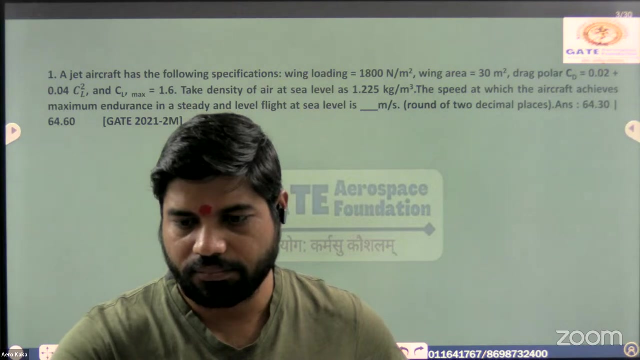 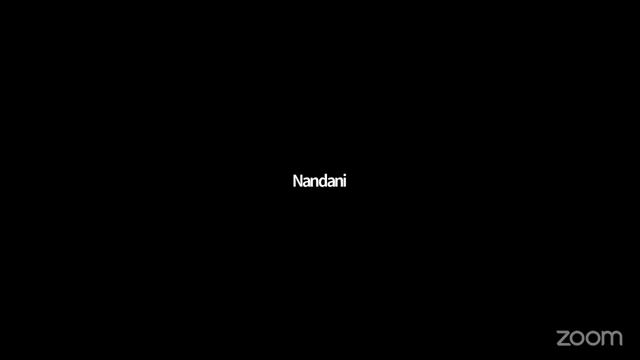 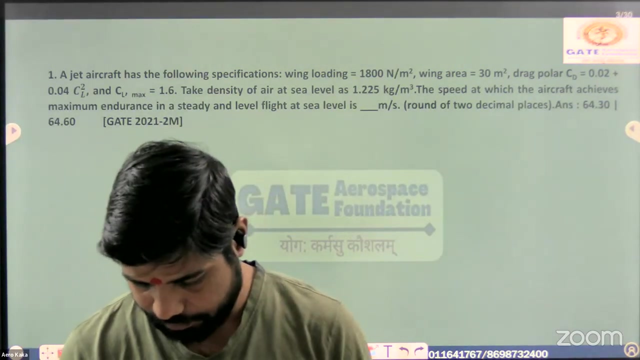 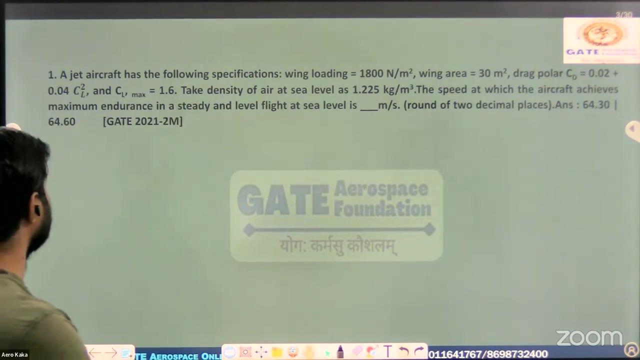 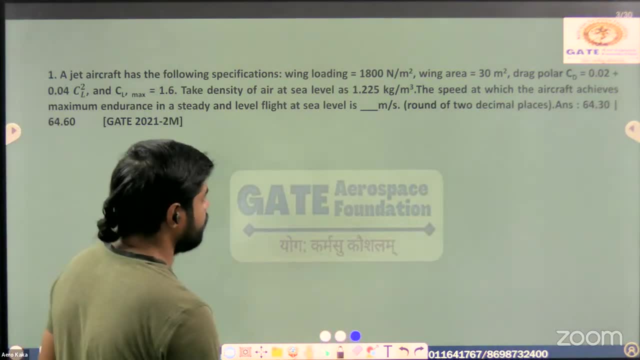 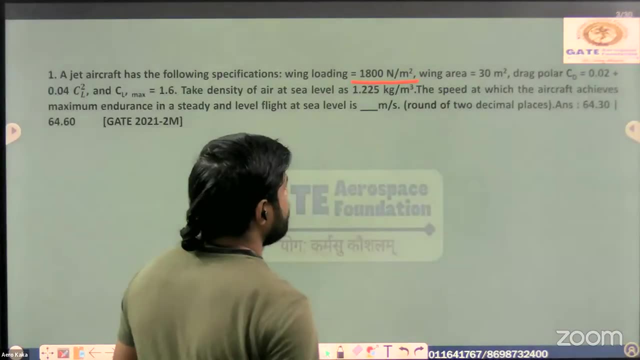 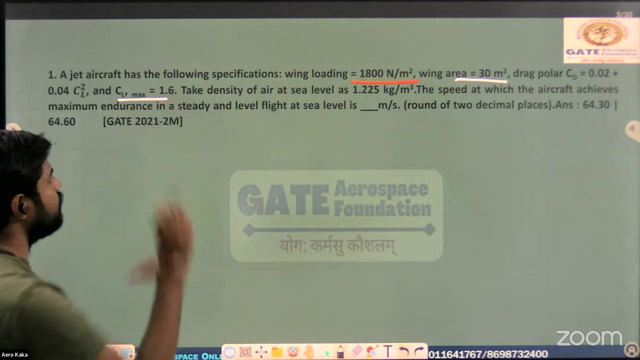 Wing loading is given here like 1,800 Newton per meter squared Air is given 30 meters squared drag polar of this aircraft is given CL. max value is given to you. We are saying: take the density of air at sea level is 1.225 kg per meter cube. 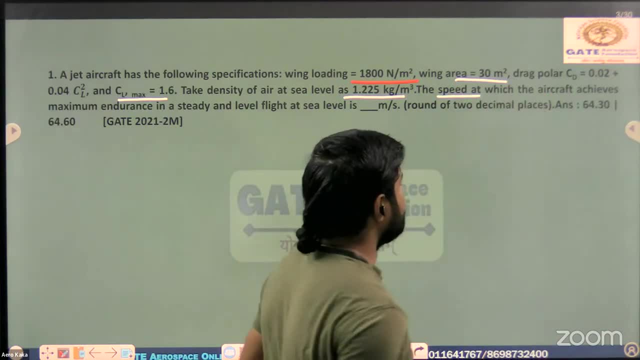 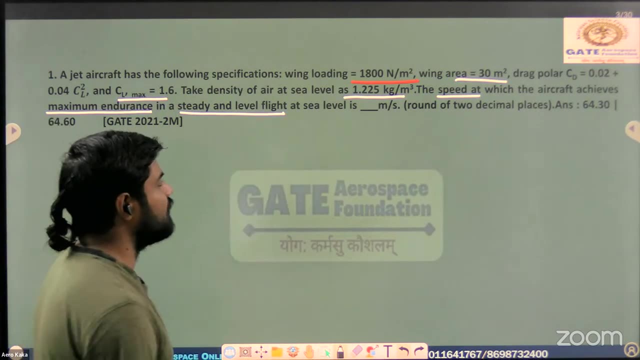 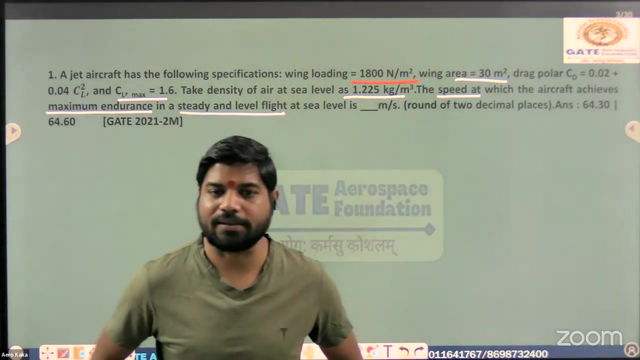 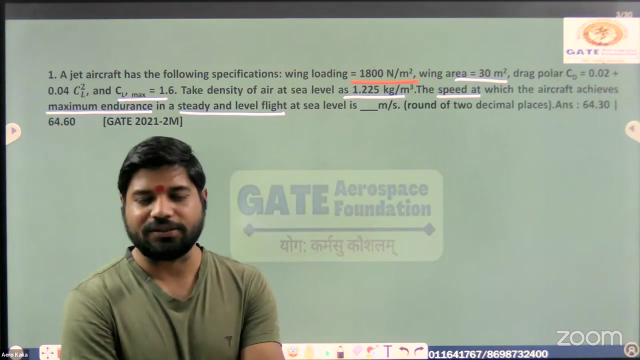 Now, the speed at which the aircraft achieves maximum endurance in a steady and level flight- Please underline this- at sea level is in meter per second, round out to two decimal places. So can you solve this problem? Yes, How do I approach? First of all, which aircraft is this jet engine aircraft or is it piston based? how do you? 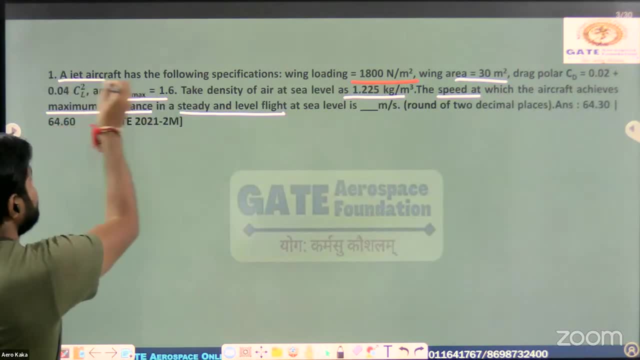 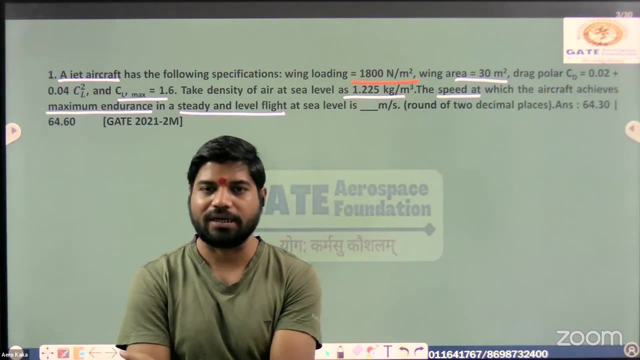 see propeller. this aircrafts Just simply written here. It's a jet aircraft, right? So generally in range and endurance, if you are dealing with just jet engine aircraft, then here we have two formula. one is endurance, another one is what? 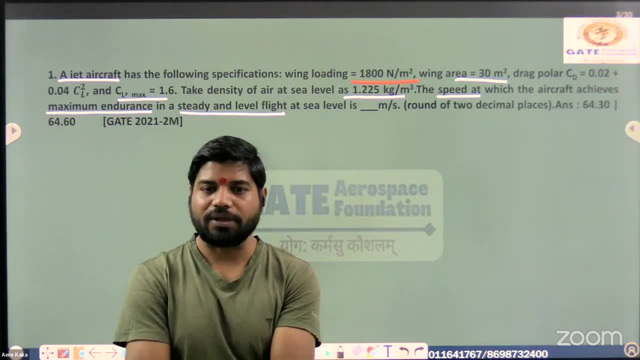 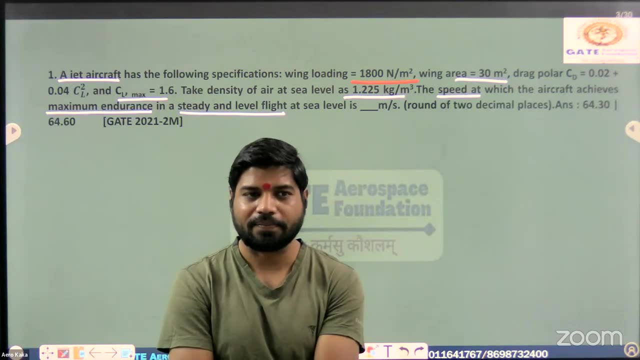 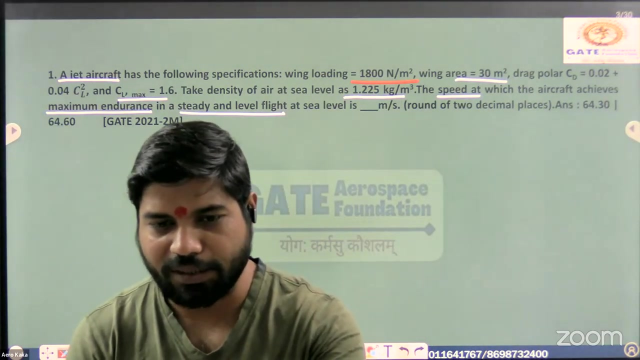 Rens formula right. Similarly, we are having for this piston base, or you can say propeller based. also have how to approach, Okay, aircraft, right. so what are the formulas? anyone for this jet engine? yes, anyone. okay, please comment in chat box. if you know, please comment in chat box. 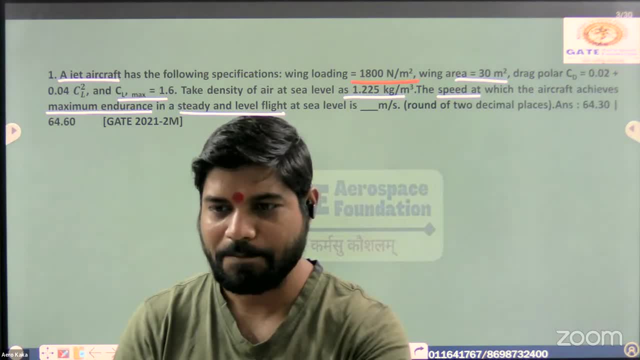 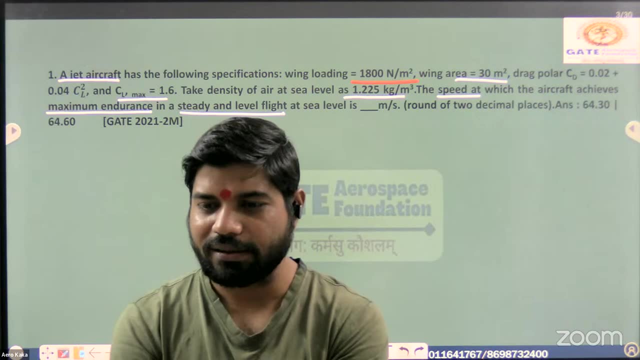 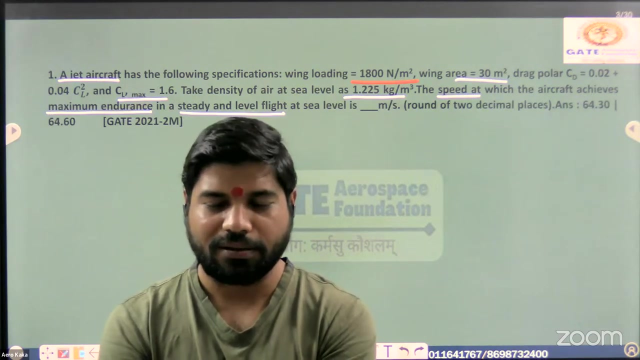 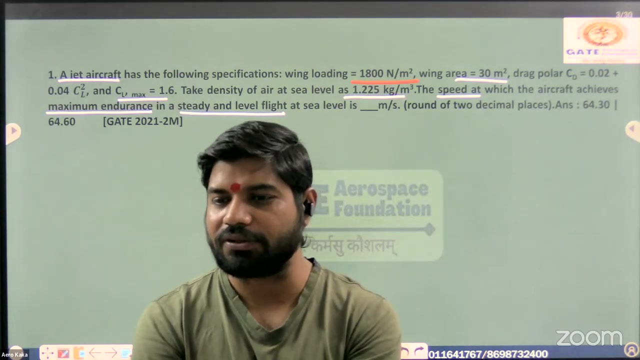 or just please unmute and answer. what is the formula narshamma? are you there? parsha, are you? what is the formula capital r, which can do? what is the formula khushi, are you there? no capital, uh, for jet engine aircraft capital r is it was true? 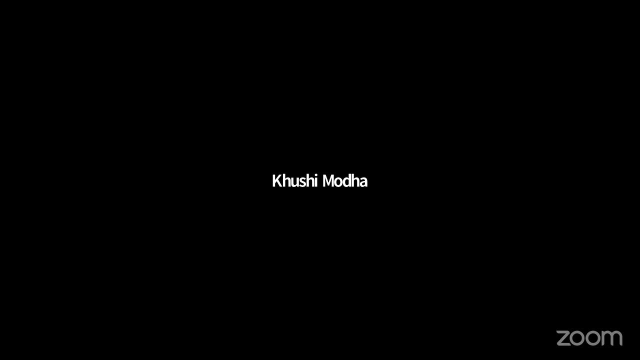 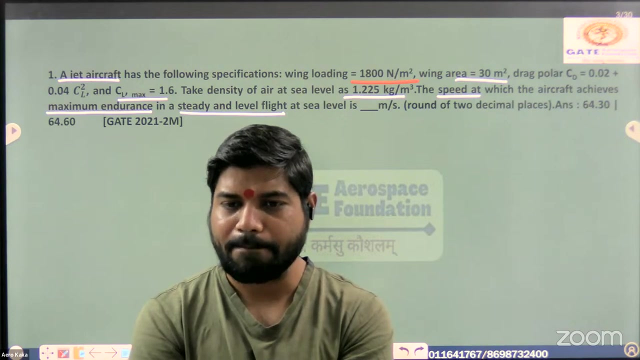 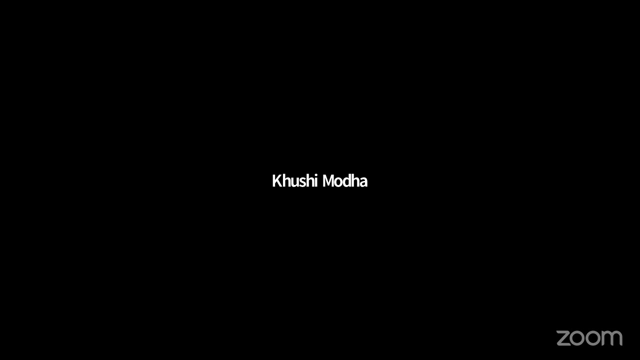 can you? can you come again with this range formula? okay, what is capital r? r is equals to 1 upon ct uh cl power. 1 by 2 by cd under root. 2 by rho infinity s. 2 divided by rho infinity s w node into w node raise to 1. 1 by 2 minus w 1 raise. 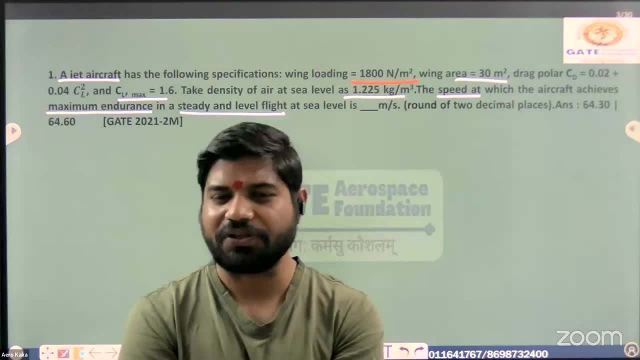 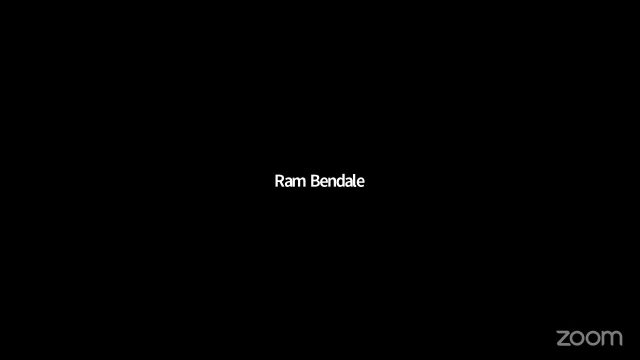 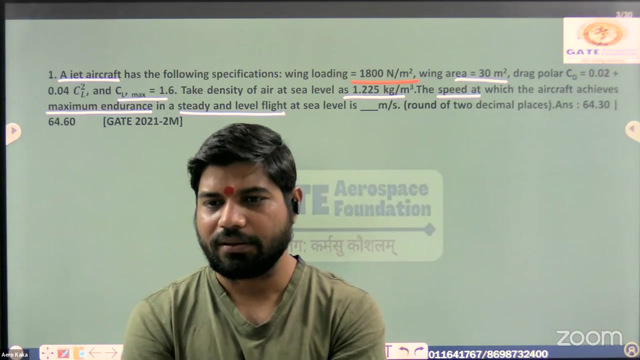 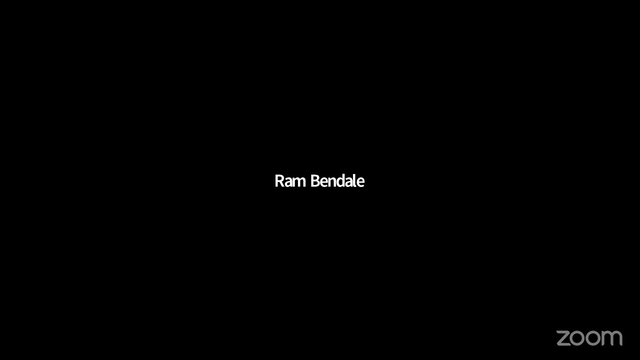 to 1 by 2. are you sure any, any, any other student? sorry, sorry, sorry, sorry. 2 by t s fc. okay, tell me what is the formula: 2 by t s fc into root of 2 rho, or 2 by rho s into cl raised to 1 by 2 by cd, into root of w 1 minus root of w 2. 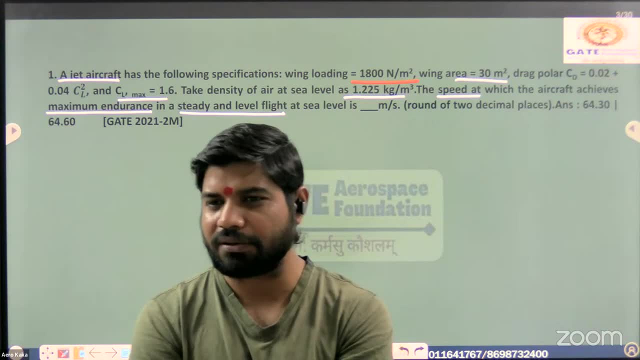 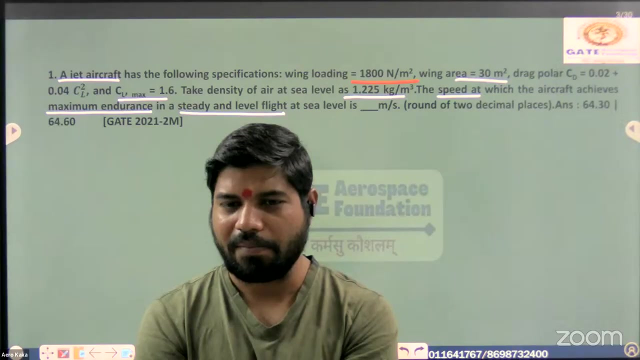 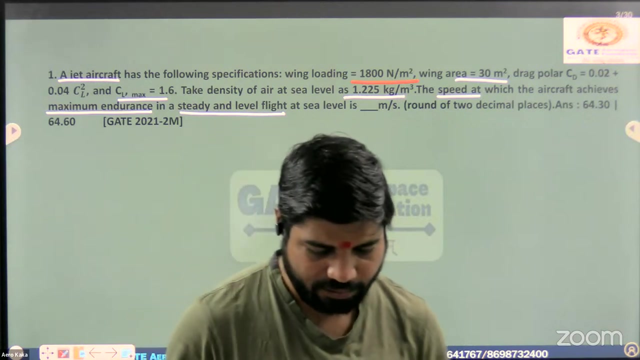 okay, now, which one is correct. khushi, your formula is correct. or what's your name? ram ram, yeah, so which one is correct? so please take care, okay, please revise properly. if you forward the formula, then then how can you answer this question? okay, so right now, ram's formula, capital r, which can do: 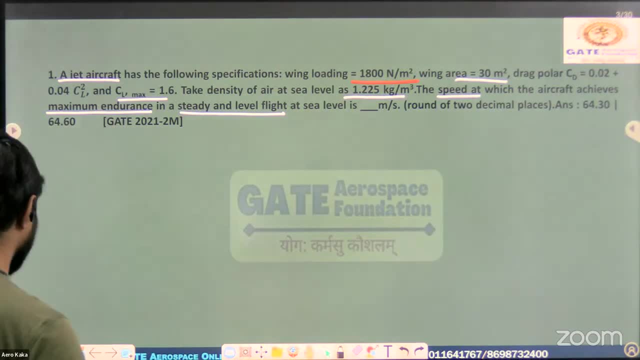 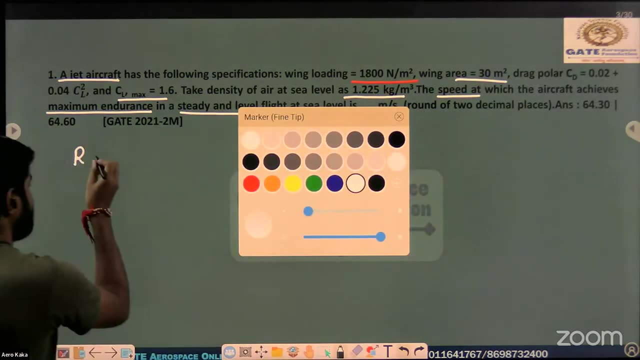 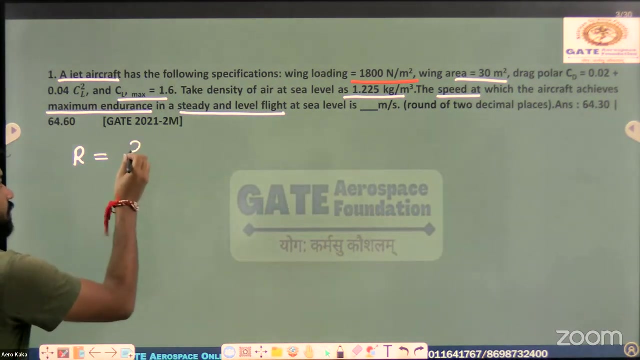 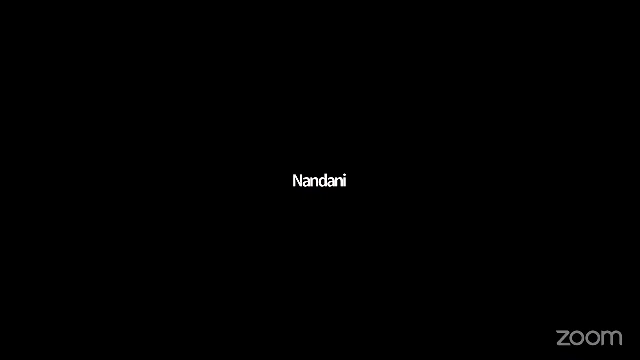 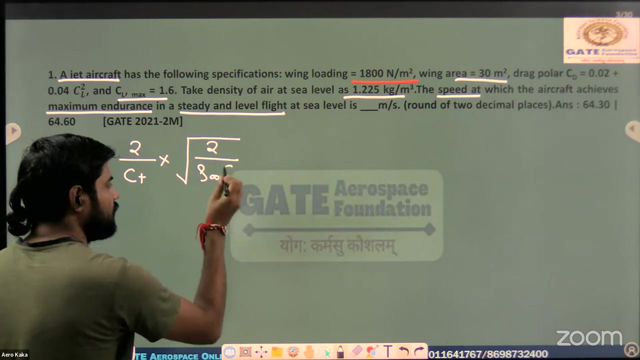 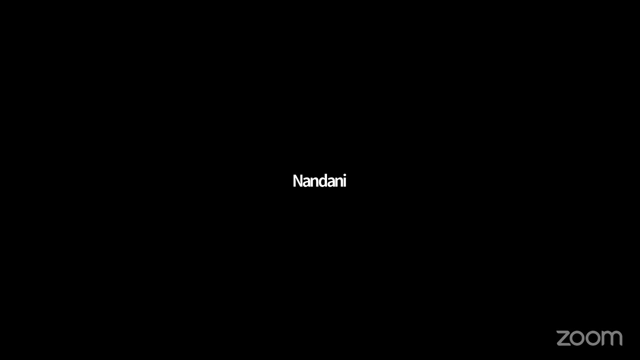 right now capital r, which can do what is the formula 2 upon ct, 0 x 2. into what is next root of c, l, root of 2 upon rho infinity, s, rho infinity into s. into how much cl raised to 1, 1 by 2 upon c d. 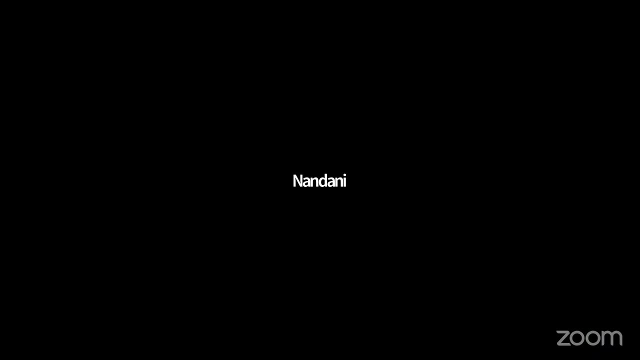 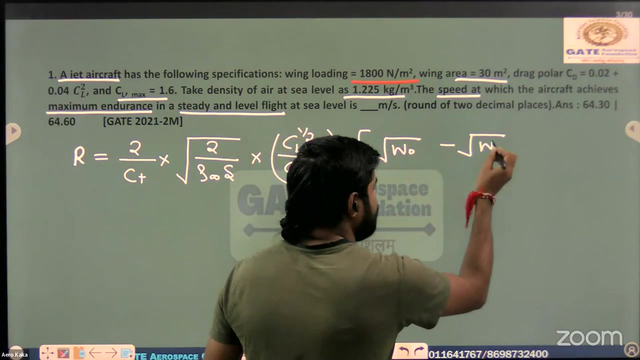 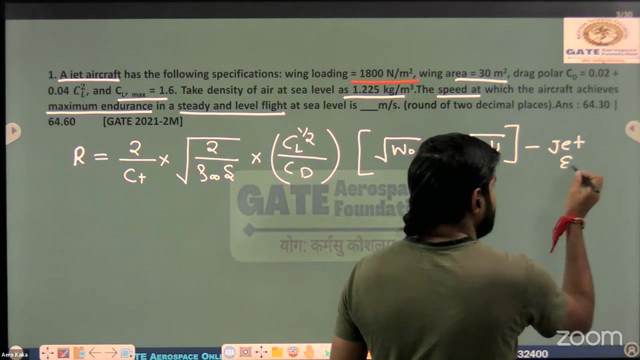 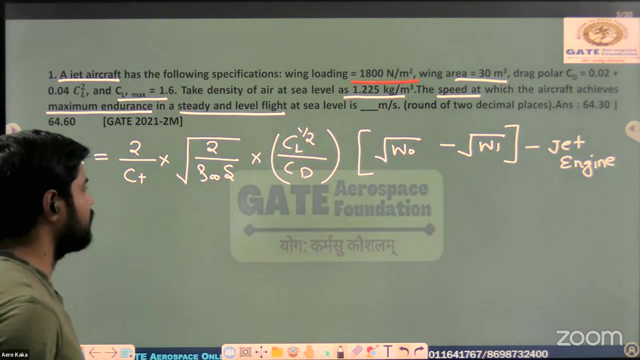 right into how much. yes, root w naught minus w root w1. root W naught minus root of W1, right, That's your RANS formula for this: jet engine, aircraft, For jet engine power plant, or you can say aircraft Now. so what is given in this question? 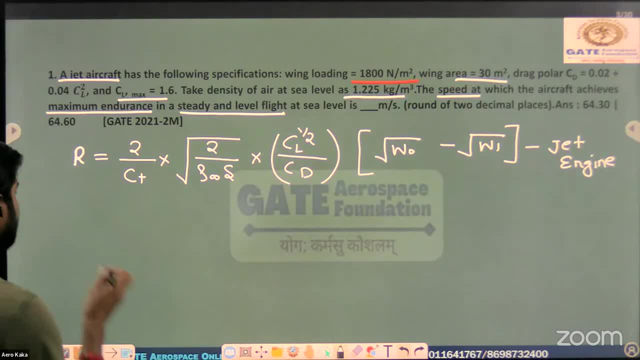 What is given. Let's write down: Bing loading is given, So generally defined, the Bing loading small w, is equal to capital W upon S, which is given here How much 1800 Newton per meter square. or you can say it's a passcode, Then Bing area is given, capital W is equal to 30. 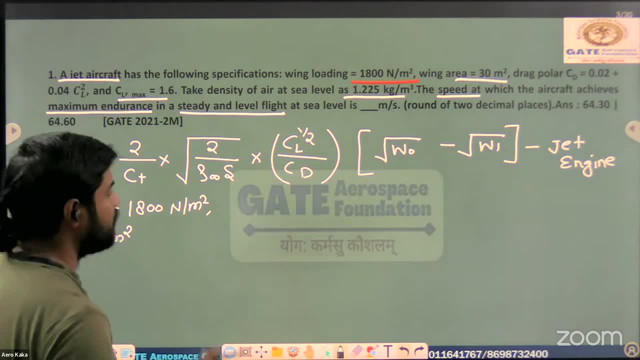 meter square. Then drag polar of this aircraft is given. Ct is equal to how much 0.02 plus 0.2.. 0.04 CL square comma. CL max value is also given here. CL max is given 1.6 comma Take. 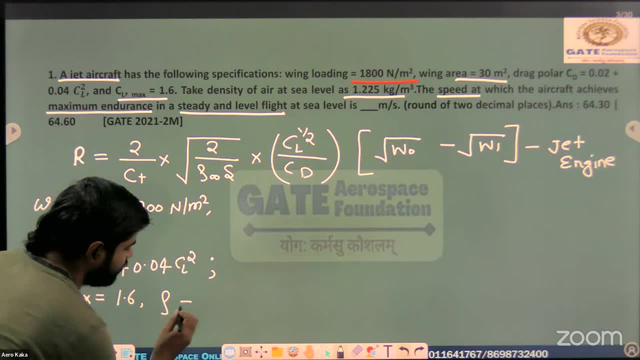 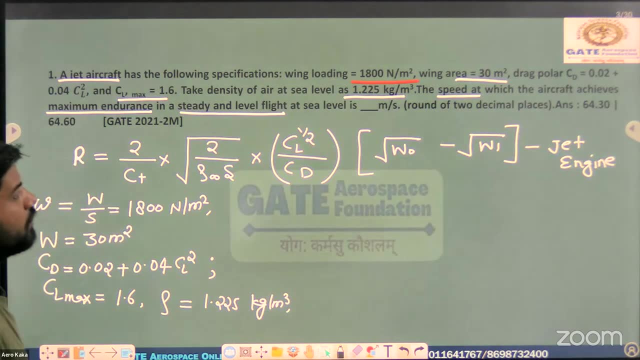 density of air at sea level. So density given here rho is equal to 1.225 kg per meter cube. right Check the speed at which the aircraft achieves the maximum endurance. so they are asking: what is the speed of this aircraft for maximum? 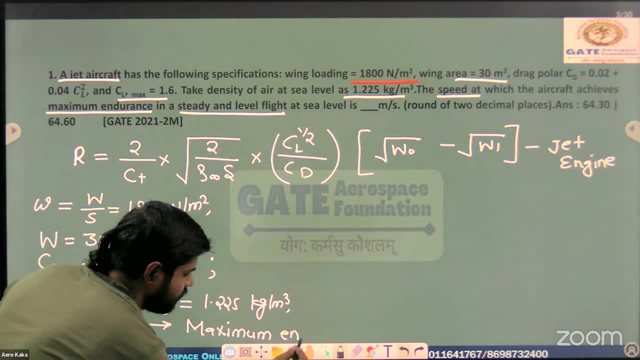 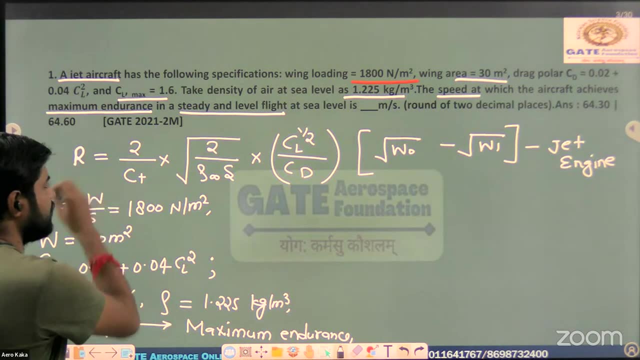 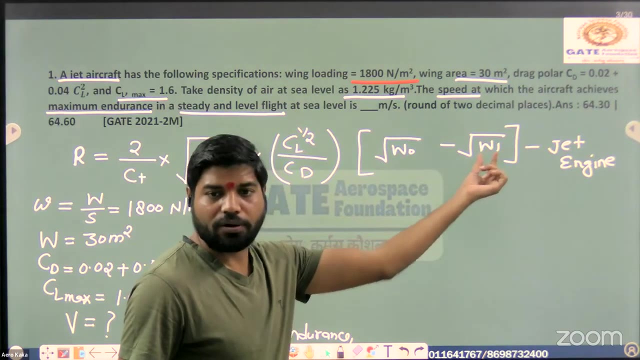 endurance. now how to approach this question. look, if you look at this range formula, if you keep all the parameters in, like what is the cross takeoff bit right? what is the w1 here? or you can say we have no issue at all. then cl raise power 1 by 2 upon cd. this is nothing, but you can see. 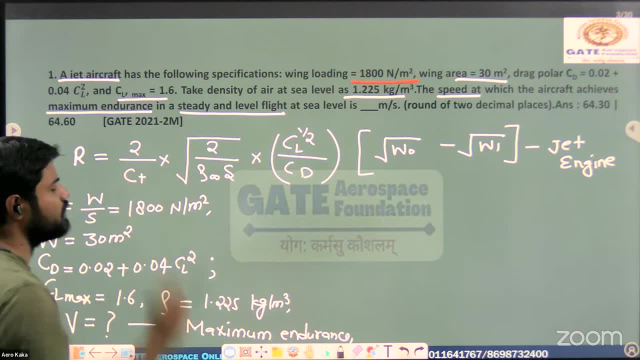 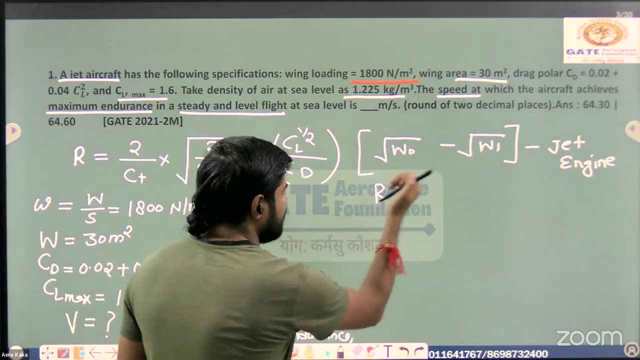 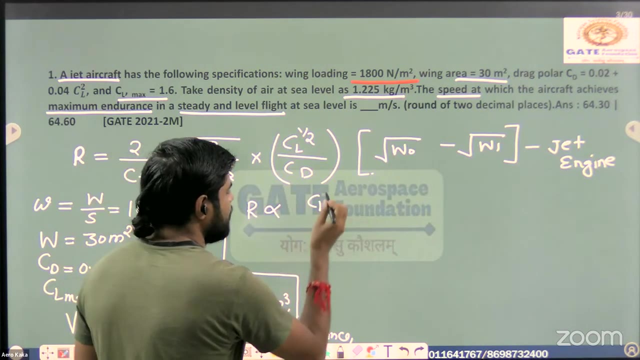 rho infinity into s, and this is nothing but 2 upon cd. if you keep all the parameters same, or if you look at this carefully, right then here you can write: r is directly, r is directly proportional to cl. raise power 1 by 2 upon cd. which condition is this? 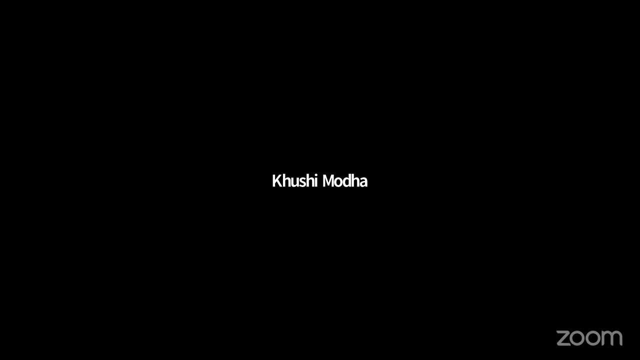 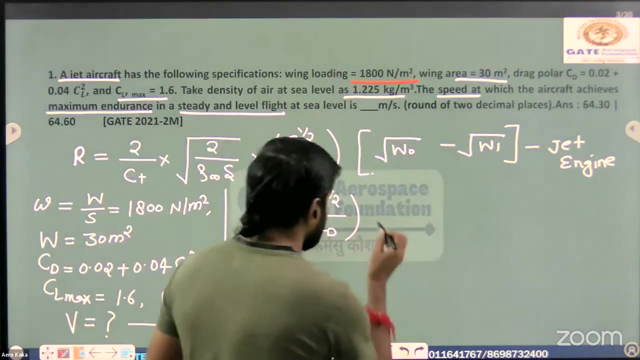 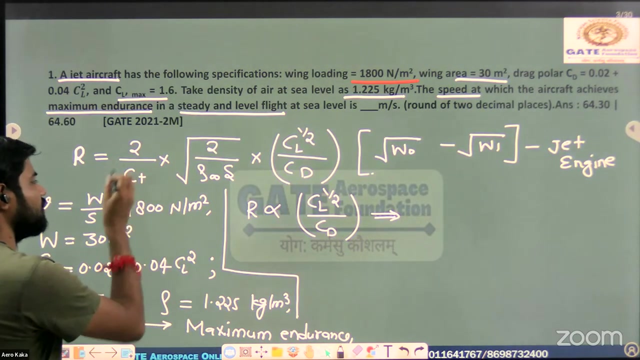 is it minimum, is it minimum drag condition, minimum power condition or minimum dyv condition? which condition is this minimum dyv condition right? so you know that very well. if suppose, if you want to maximize the range right of this jet engine aircraft you must have, you can see lower amount of b. what is this ct here? 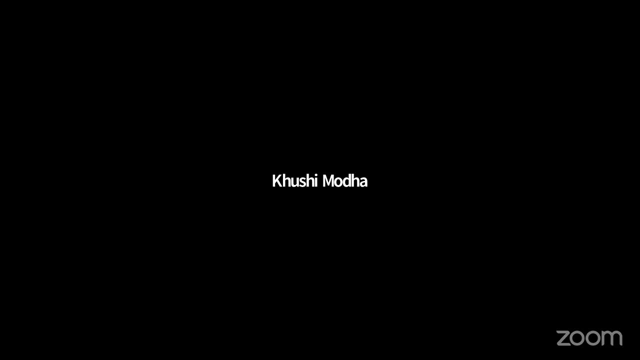 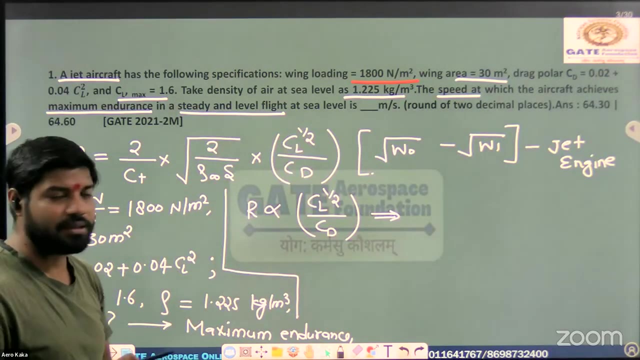 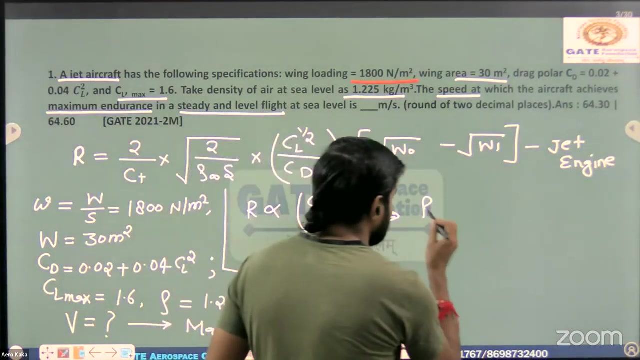 anyone. what is this ct here? you can say, this is nothing. but you can say density capital s? here is nothing but against, it's a wing plane form area, right. so what you can write here, or or what you can understand, if suppose if you are flying this aircraft, that means right. or let's discuss r is something like this: check. 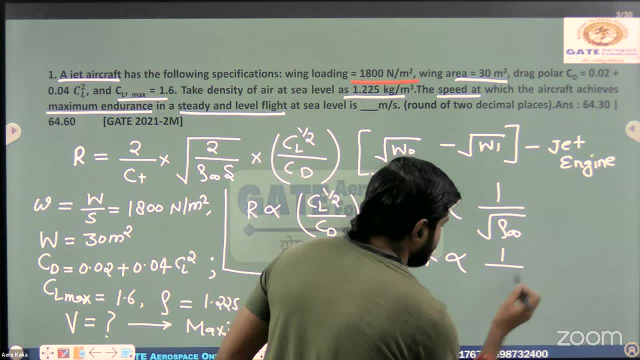 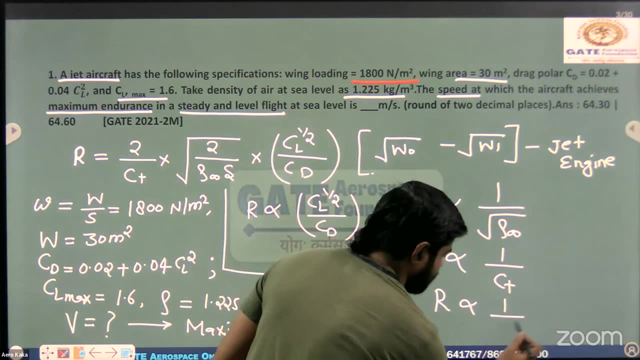 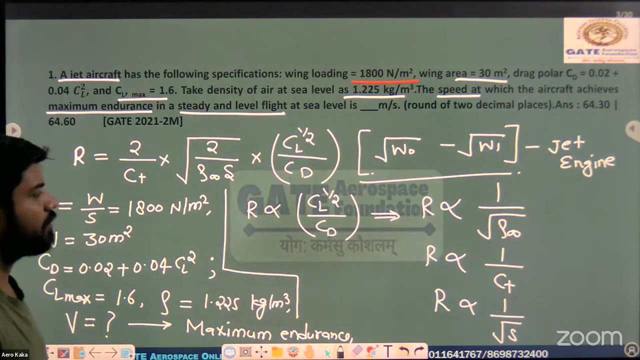 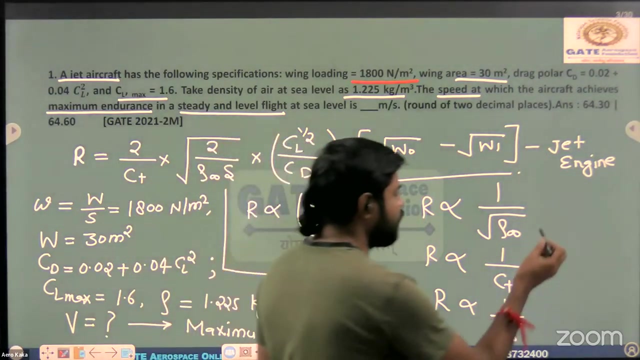 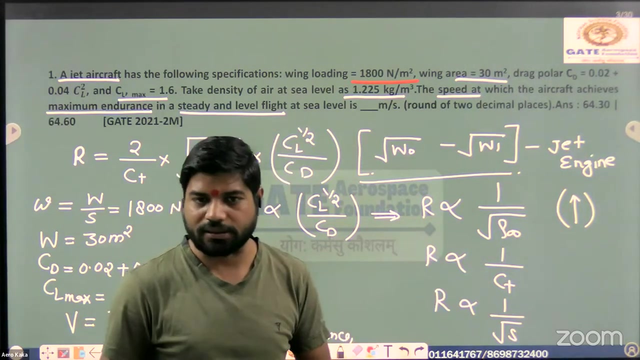 agree, then r is also. then any other parameter? yes, then obviously this one is also there. so from here what you can observe. if suppose, if you want to maximize the range of this aircraft, we have to fly the aircraft at higher altitudes, why? because as the altitude increases then you can see the density decreases, are you agree? 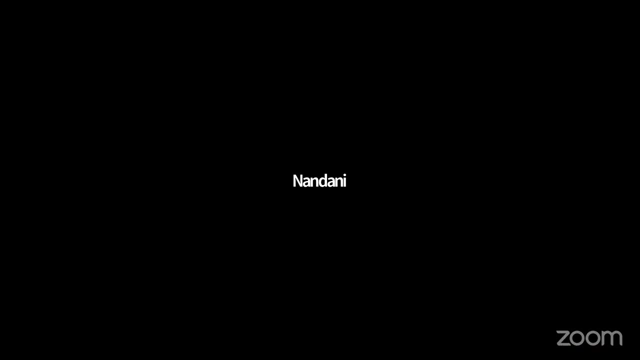 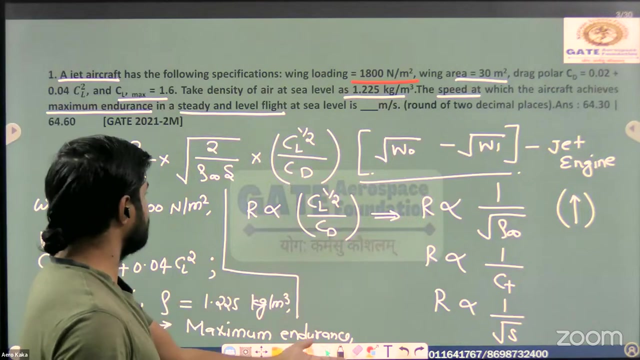 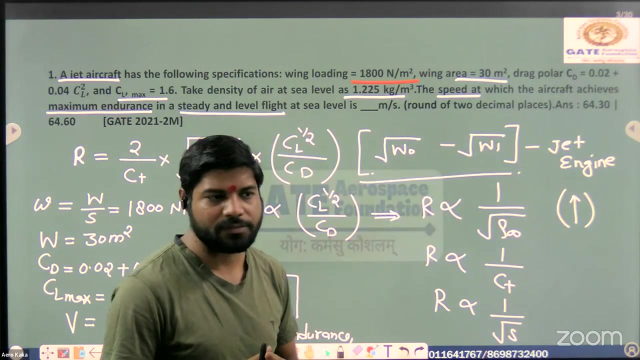 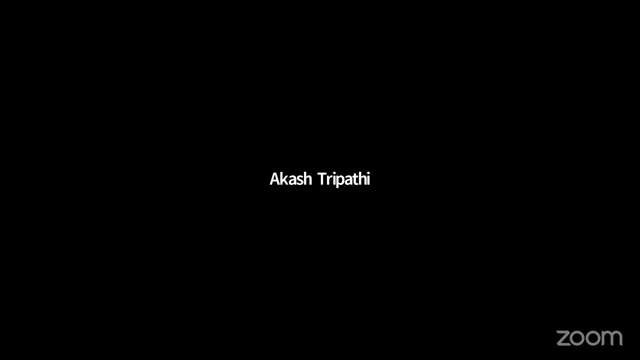 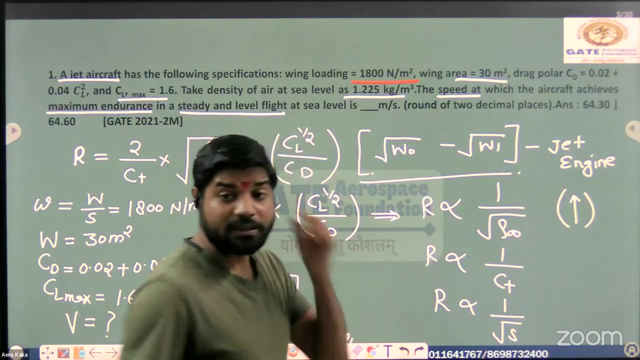 yes, okay, let's discuss. what about the rent. then we will deal with this and there is no sure thought. okay, so in this case, what happens? so is it endurance for more rents formula? I think this is rents formula, right? yes, we are going to discuss these all things, okay? so what I want to convey? yes, please. 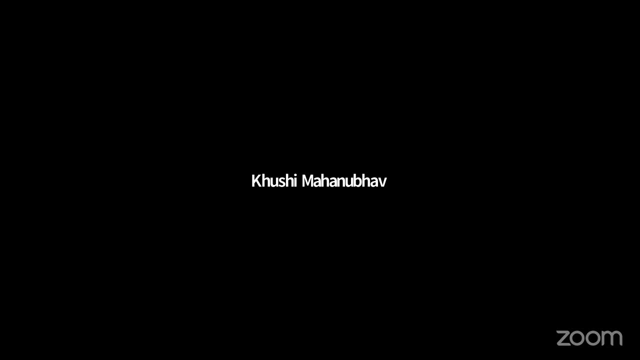 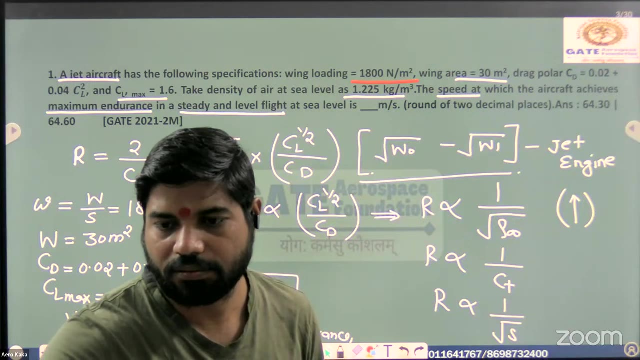 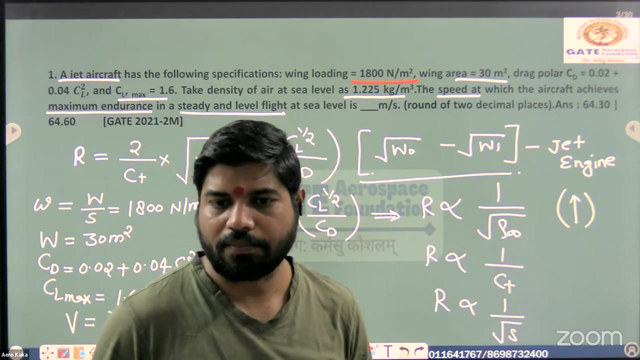 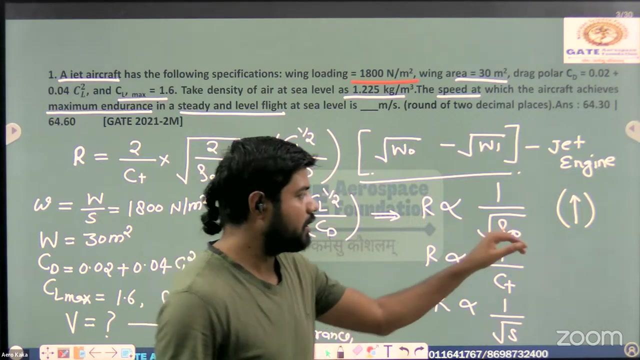 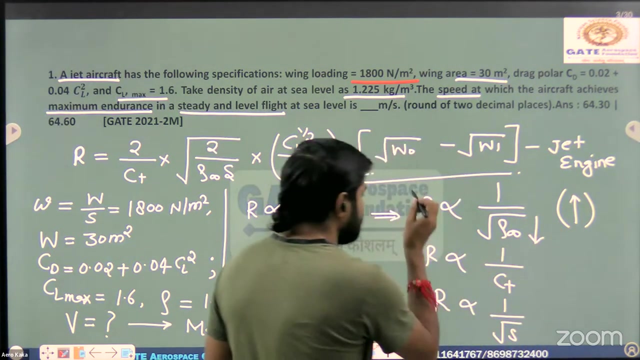 sir, focus more on the screen. okay, okay, just wait now. okay, please check. yes, okay, so here, if suppose, if we talk about the rent of this jet engine aircraft, right then as the altitude increases, then the ambient density decreases. it means that what this denominator value decreases, then the value of capital R increases. okay, please. 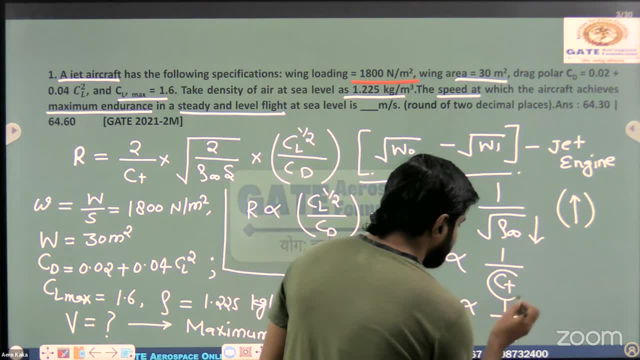 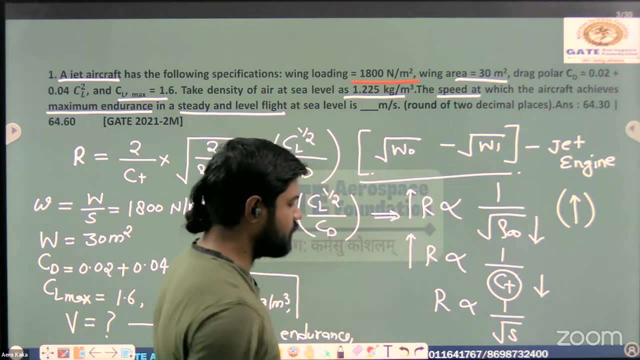 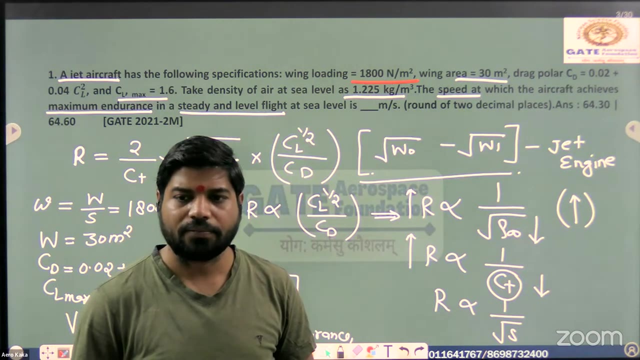 remember, it's a final revision, and here this is CT. right again, if the thrust specific fuel consumption decreases, then the range of the aircraft increases. similarly you can write for this capital S, or you can say beam loading also. so shall I ask you one question? you can answer that question in our official 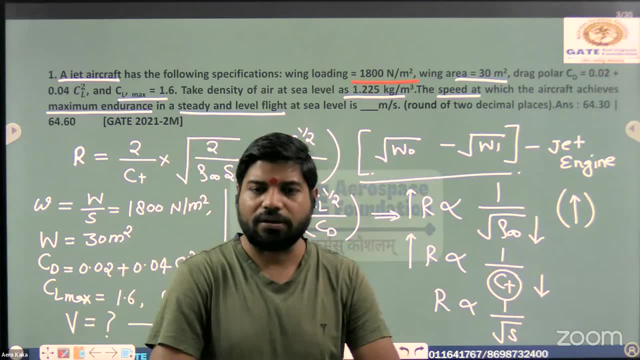 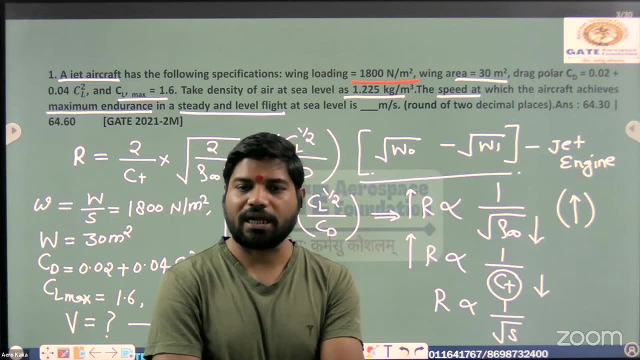 group. okay, okay, which one is required? if suppose, if we talk about, you can see the landing as well as the takeoff as well as the cruise flight. so which one is desirable? high-wing loading or low-wing loading during the loose flight, or, you can say, during the steady-state level? 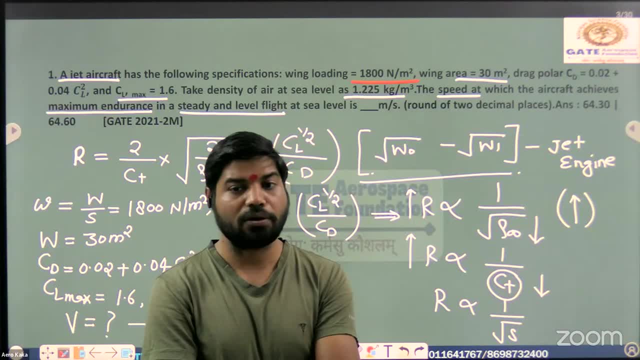 flight which? which wing loading is required? high-wing loading or low-wing loading? you should have to answer in our official group. okay, yes, sir, and then what is required is required, or you can say what is desirable for. you can say the landing as well as the for the. 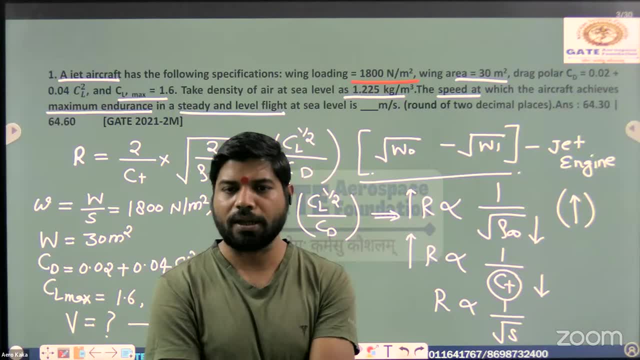 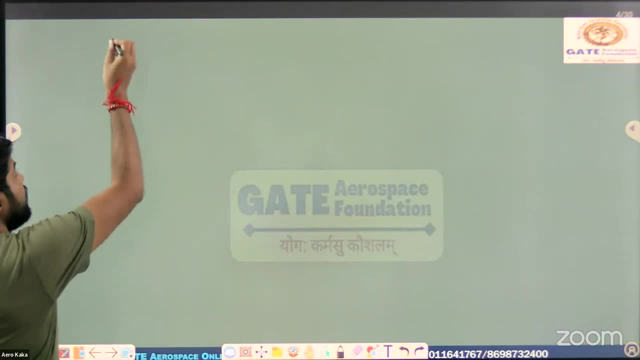 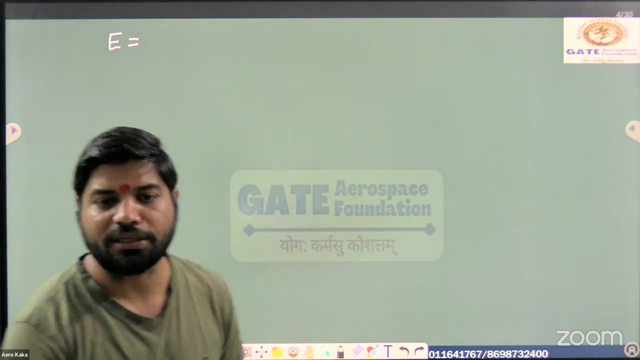 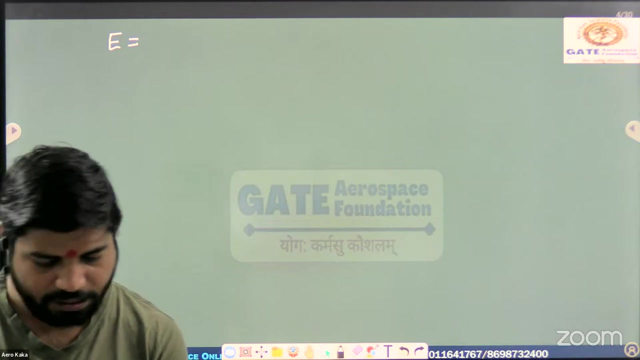 takeoff high being loading or no being loading, okay. okay, now here let's write down what is our range formula. sorry, endurance. formula e is equal to? what is the formula one upon yes, what is the formula capital? e is equal to 1 upon ct. check hello. e is equal to 1 upon ct into cl upon cd, or 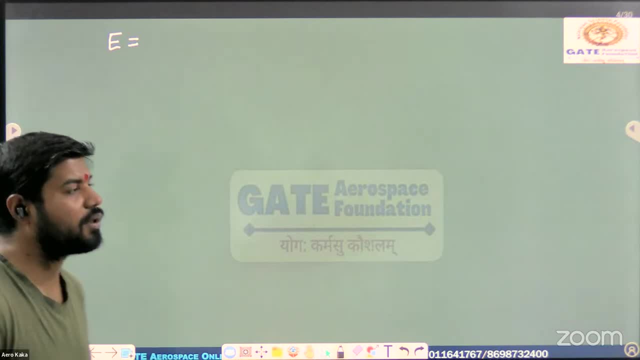 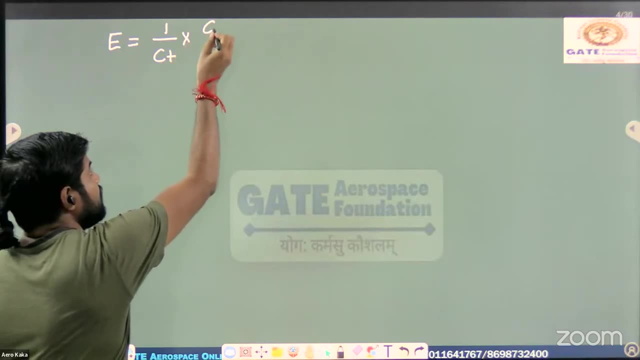 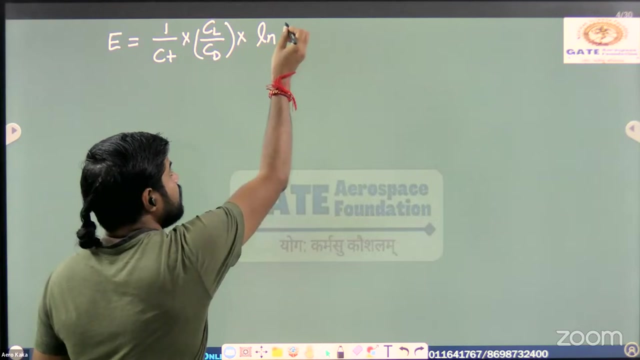 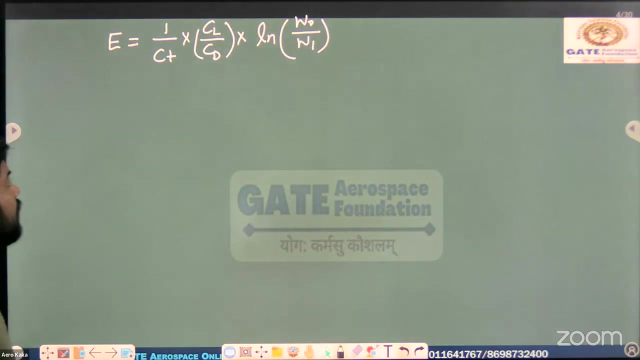 you can say l y d ratio into ln of w naught upon w1. right, check one of them right into how much cl upon cd, into which is nothing. but you can say ln of how much w naught by w1. okay, now, from here, as you can see again, endurance is, you can delete something like this. 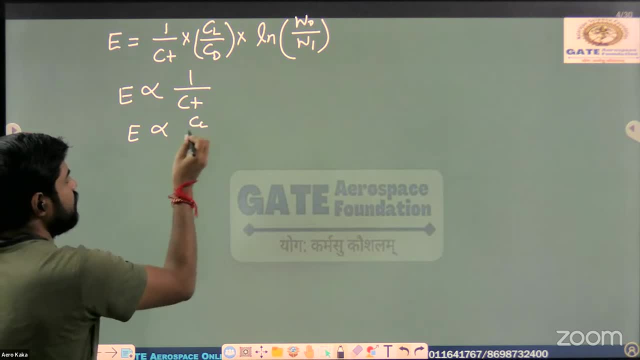 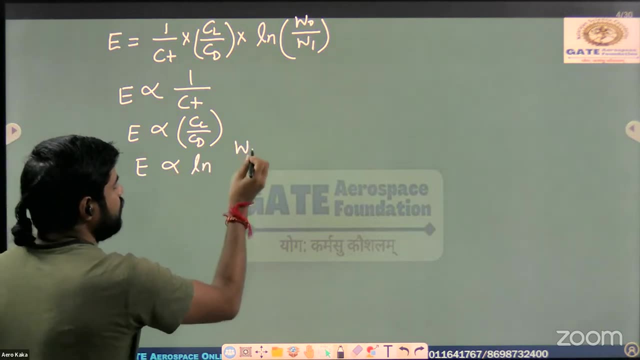 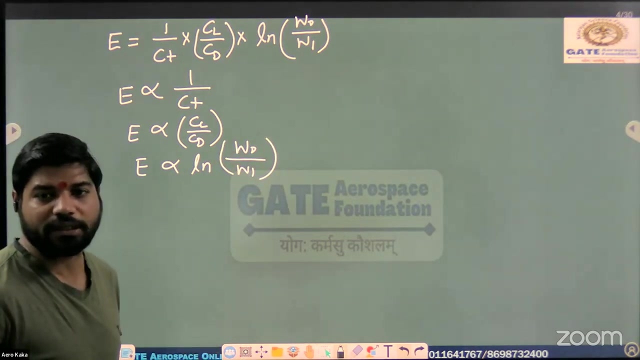 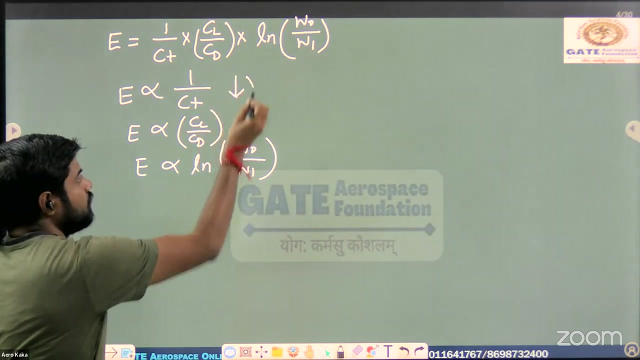 then again, is directly proportional to cl upon cd. and again you can write, is directly proportional to ln of w naught upon w1. so how we can, how we can integrate these, the endurance of this aircraft, if suppose the ct is low, then the e value will increase, right? if suppose? 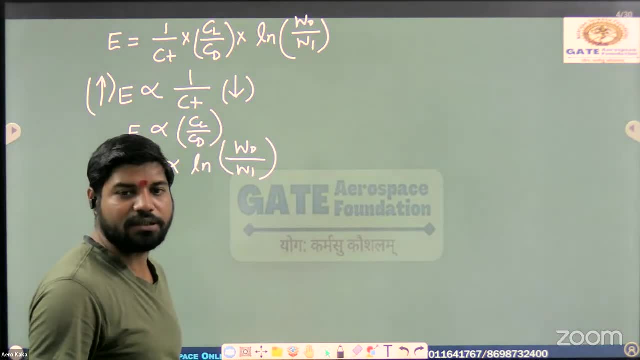 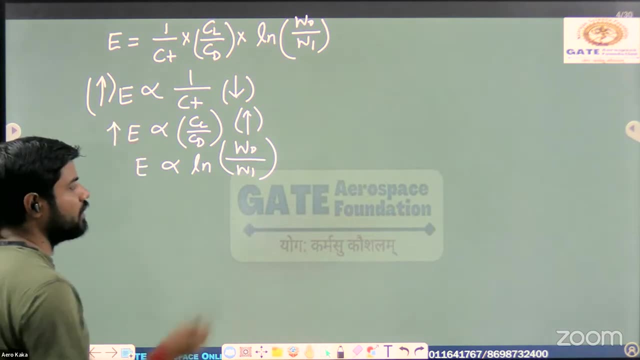 anyhow, if you increase the l by d ratio, or you can say cl by cd ratio, or you can say aerodynamic efficiency, if suppose this value increases, then this value is also increases. again, what is this? w1 or w? naught here, either you can write, w1 is nothing. what you can 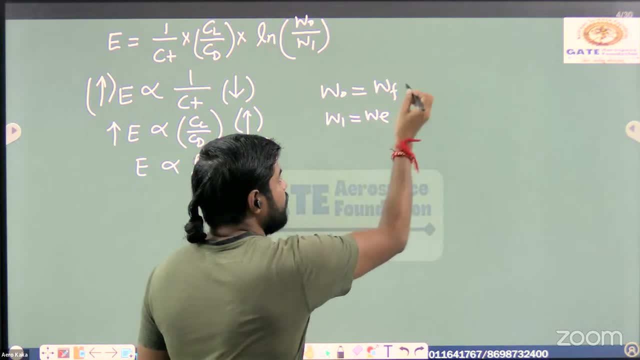 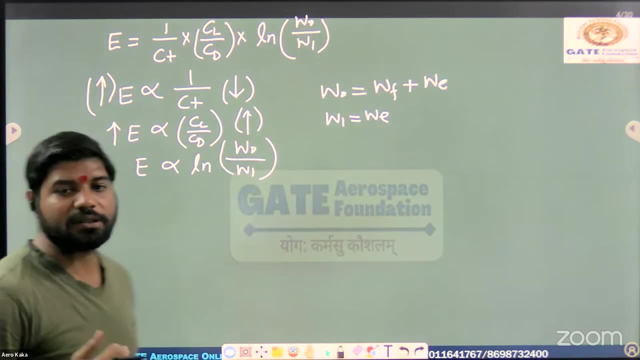 say w e here. this is nothing. but you can say the fuel of weight, weight of the fuel plus. you can say empty weight, or you can say it's a during the flight. generally we consider it's a instantaneous weight. okay now, so from here, what you can write. you can write here: e cans to e max. 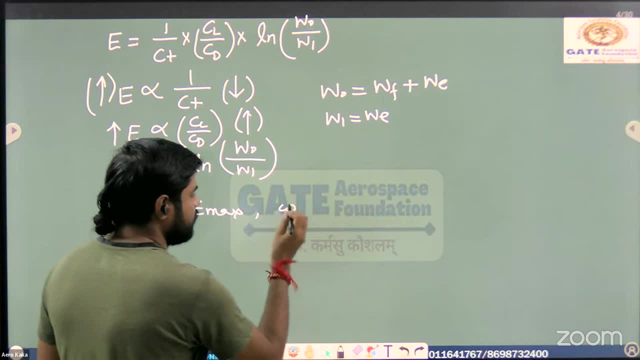 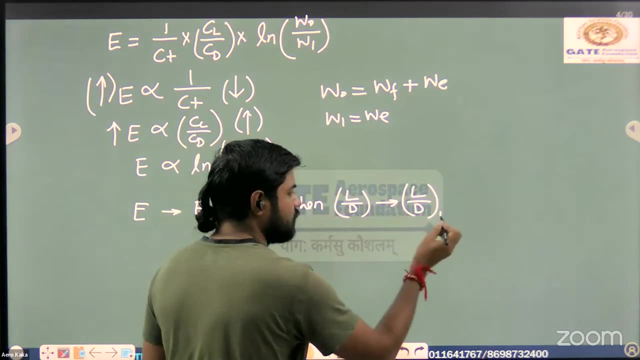 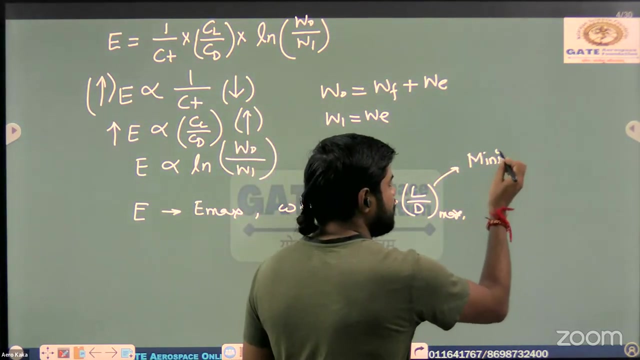 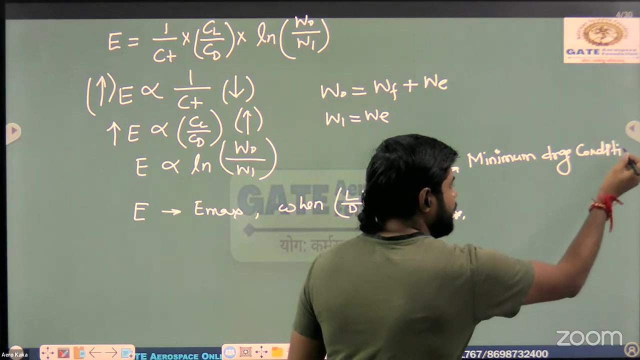 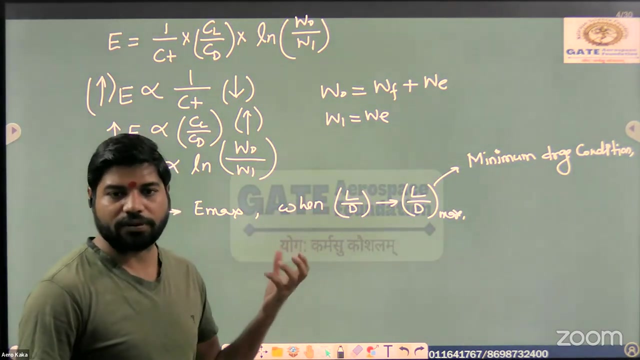 when l y d ratio becomes l y d max right. so which condition is this? this is nothing, but we generally call it is the minimum drag condition. so meaning what if? suppose, if you want to maximize the endurance of this aircraft for a particular fuel tank, for a particular amount of the fuel, then we should have to fly. 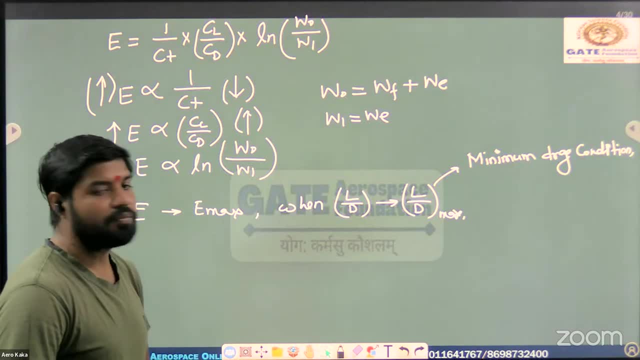 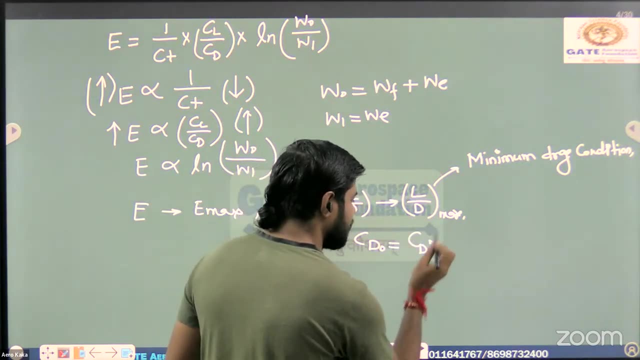 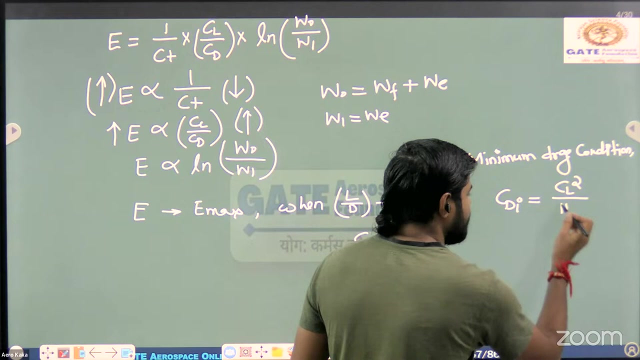 or pilot should have to fly this aircraft under the minimum drag condition. so what is your minimum drag condition? simply, this cd naught is equal to cdi. right now, from here, you know very well the cdi is nothing. but you can say cl, square upon pi, e, ar. right now, just calculate what is the value. 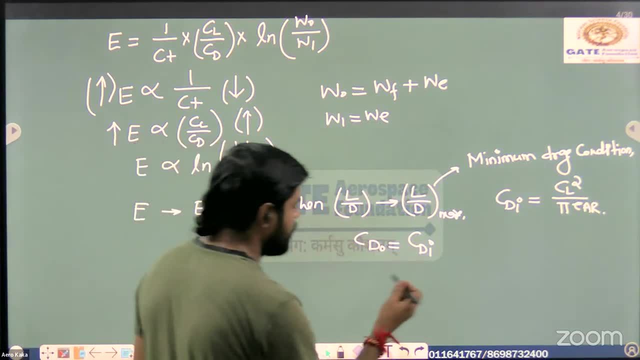 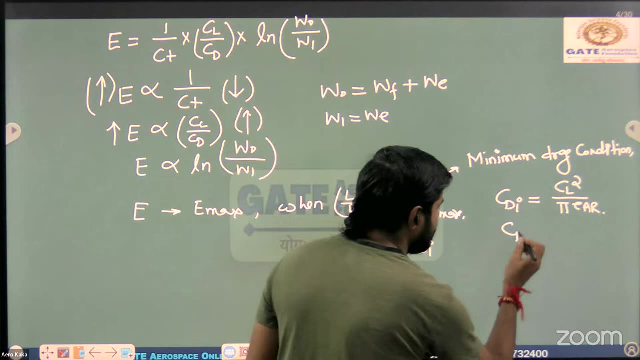 of cl with the help of this one point. so can you, can you calculate? yes, we can. so we can write here: the cd naught is nothing but. or simply you can write: this cdi is nothing, but you can say how much tcl is square right. so this ed naught is. 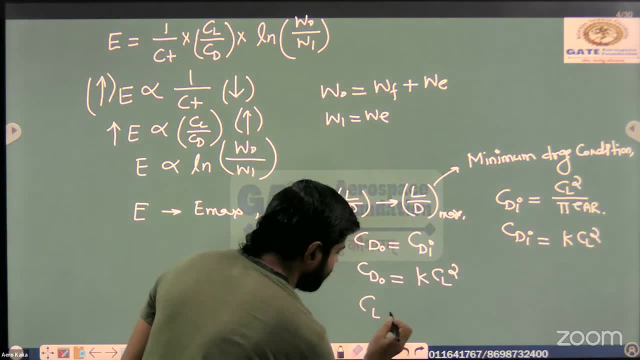 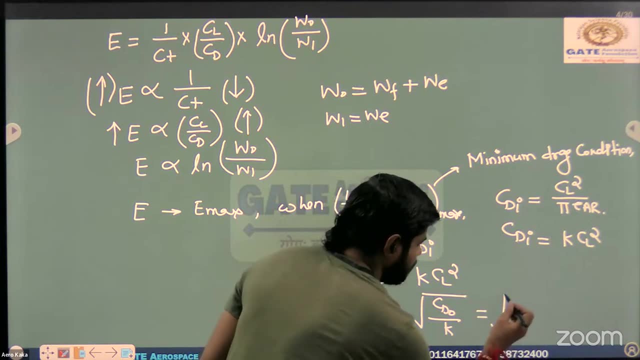 nothing, but you can say tcl square. now, from here, can you calculate what is the value of cl, which is nothing, but you can say root of cd naught upon k. now just simplify: what is the value of this cd naught here? yes, please, can you tell me what's the? 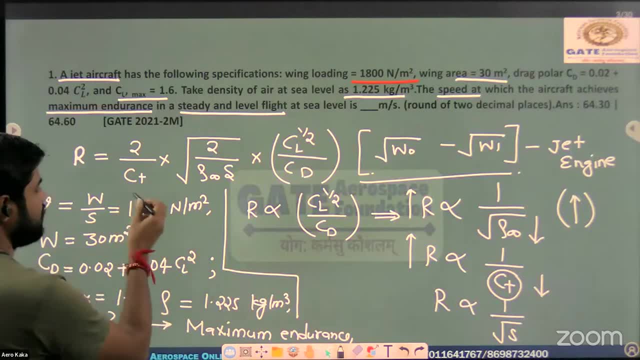 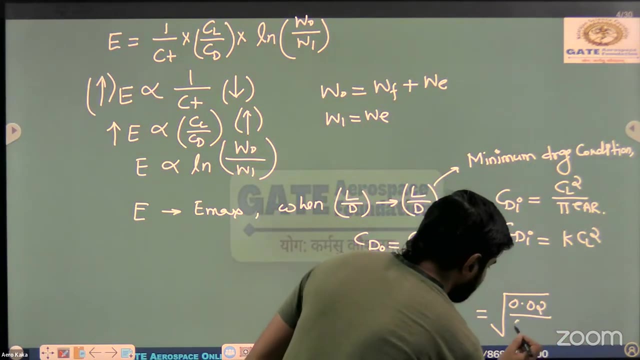 of CD naught. CD naught value here is given 0.02 and K value is given 0.04.. CD naught is how much? 0.02.. K value is 0.04.. So how much? we will get 0.7071.. So we will get this. 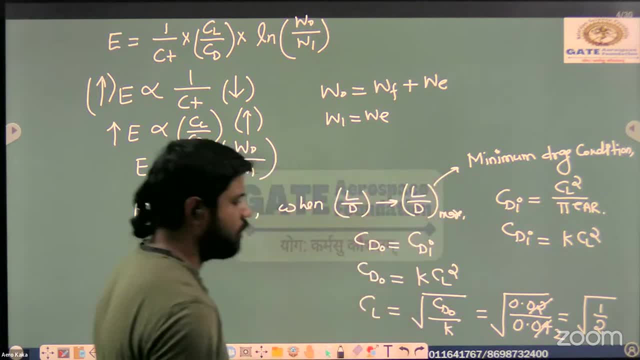 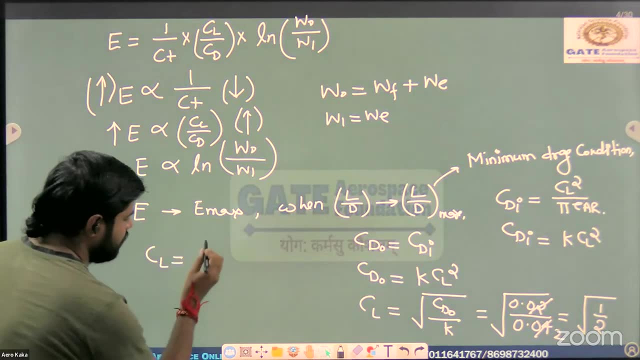 value is how much 1 by 2.. Check, please, Are you getting this one? Yes, sir, Okay. So what is the CL? You can write: this is nothing, but you can say 1 upon root 2.. Agree, Now what? 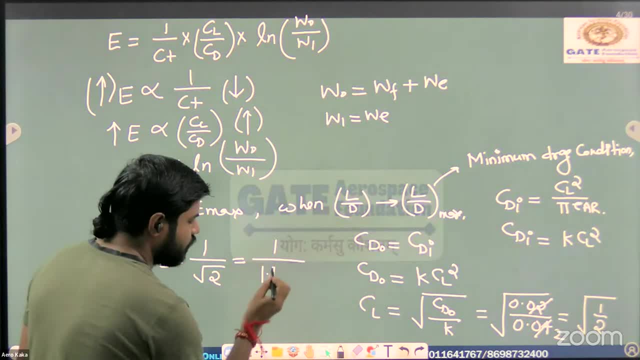 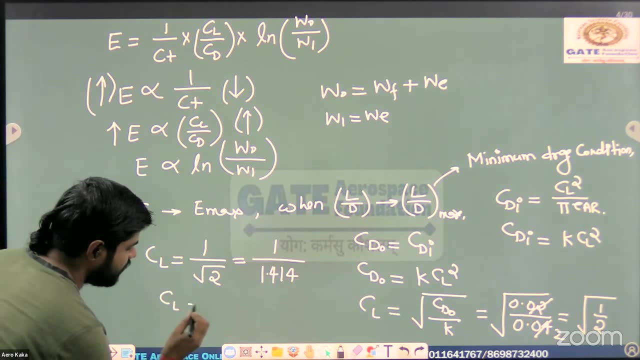 is root 2?? You can say this is nothing but 1.414.. Please verify. Yes, sir, Okay, So if you simplify it further, how much we will get? What is the value of CL, How much you are getting? 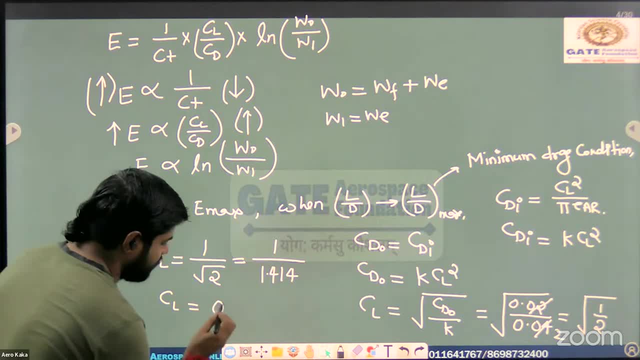 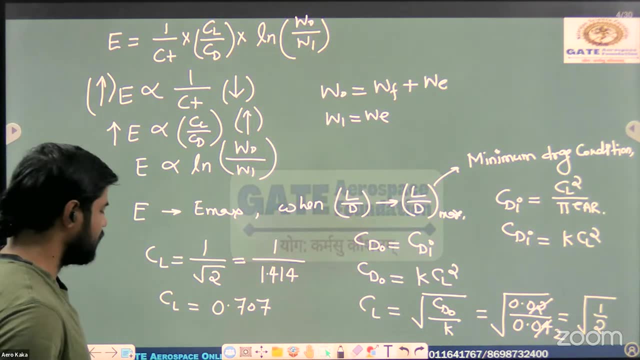 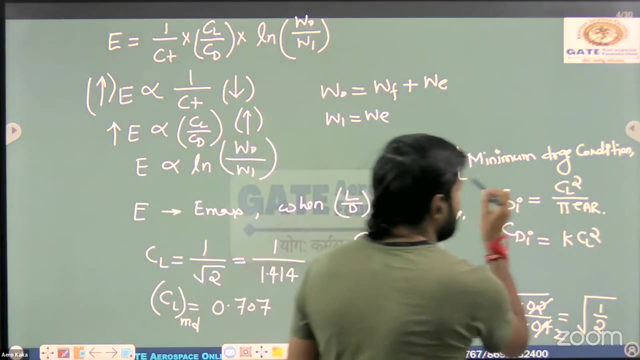 0.7072.. This value is 0.707.. Right, Once you get the value of CL right. This value is corresponds to what? It corresponds to minimum drag condition. or you can say: this value corresponds to minimum drag condition, Agree, Check Now, once you get the value of. 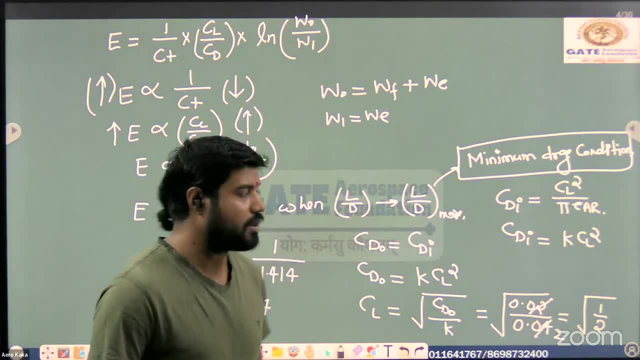 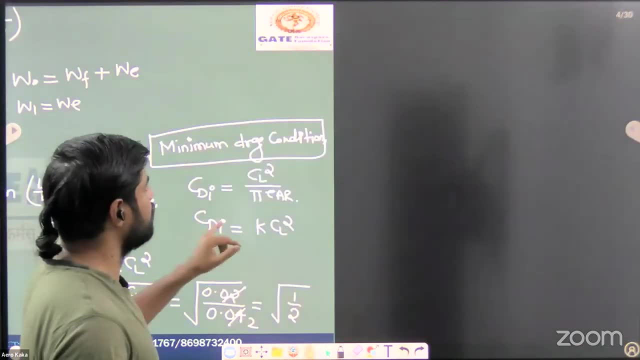 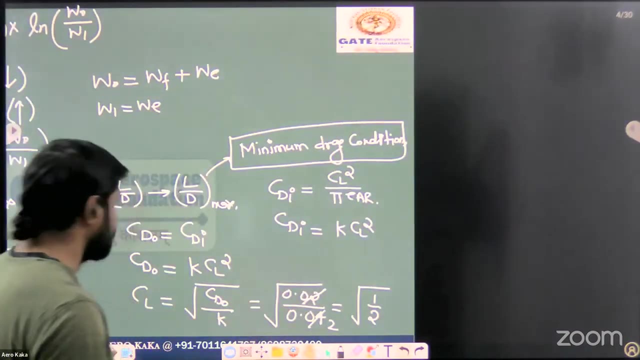 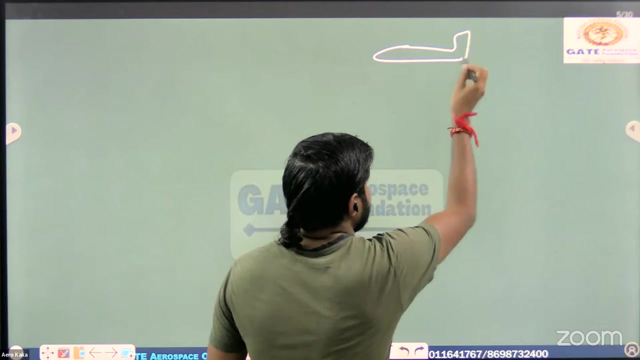 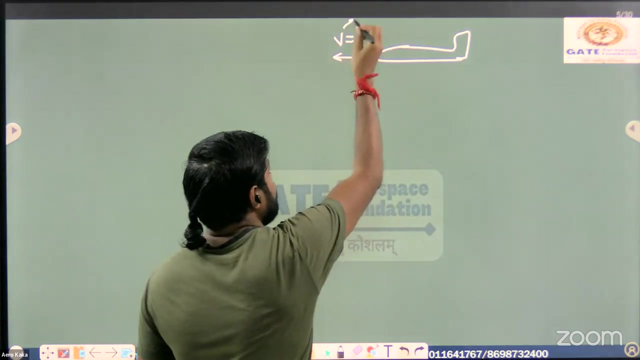 CL empty. now it is very easy to calculate The speed of this aircraft. for example, let us consider. Let us consider: this is the aircraft which is flying at certain altitude, having the forward speed B. So they are asking: what is this? B for maximum endurance, Right. 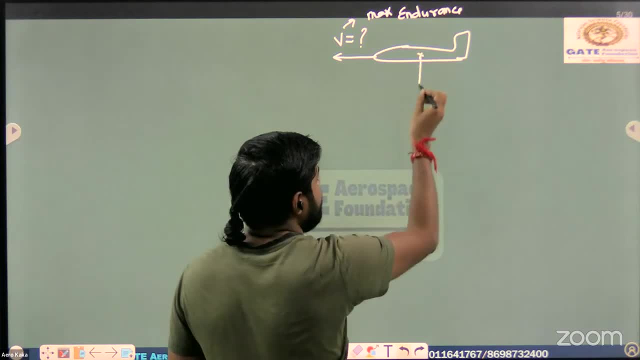 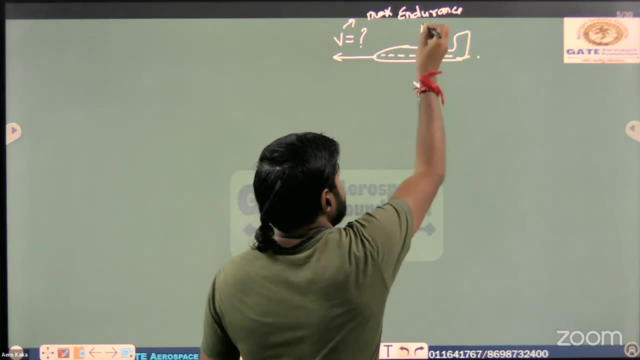 No, It is flying in a steady state, in level flight only. So you can write here: This is the weight, which is X vertically downward, then this is our flight path, this is the lift, this is the thrust and here the drag. So the aircraft is flying in this condition. 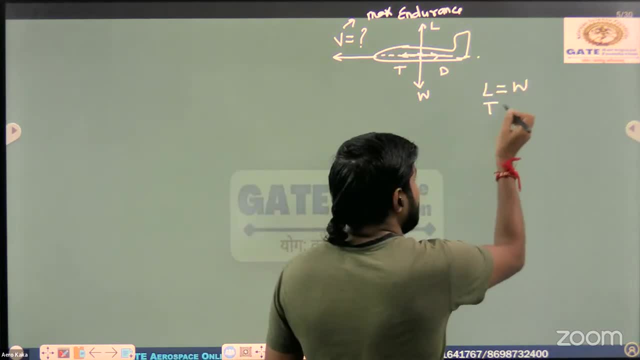 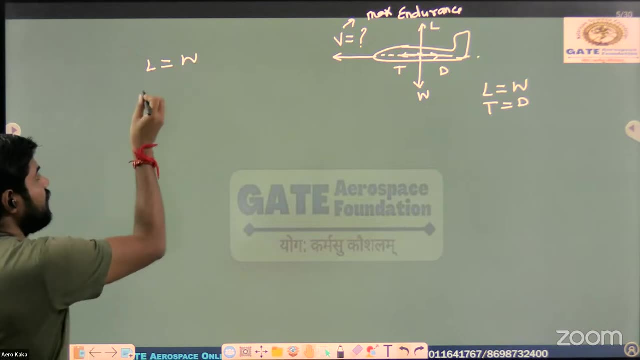 or you can say L, which is equal to W, and T is equal to T. right Now, from here, we can write L which is equal to W. What is L Does not matter. remember, this is a deliberate size. Please note: you have to make theestion of the height and then I will no more say. 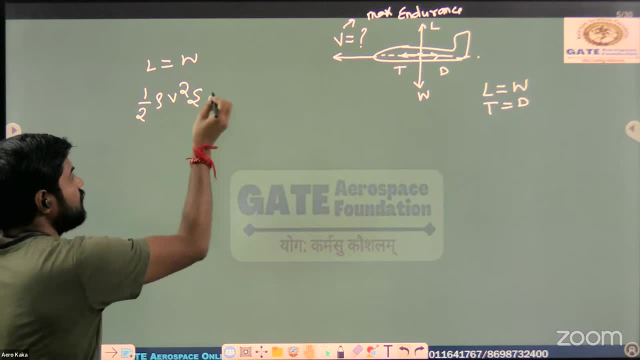 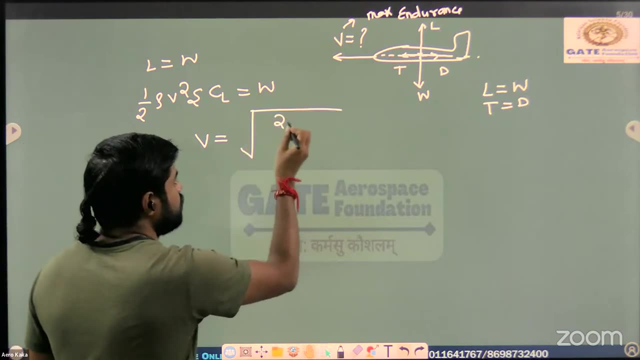 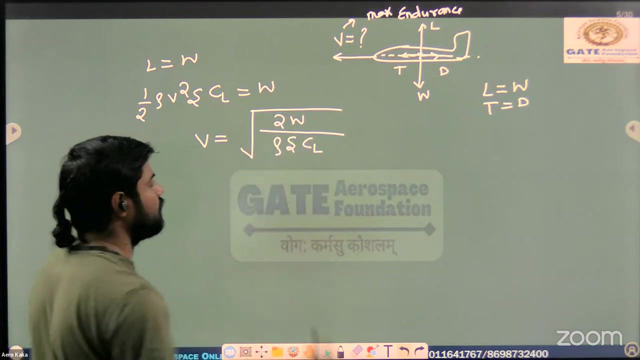 1 by 2 half rho V square S into C L, which is equal to W. So calculate what is the value V from here. We will get root of 2 W divided by how much. Yes, rho S into C L. Yes, please. 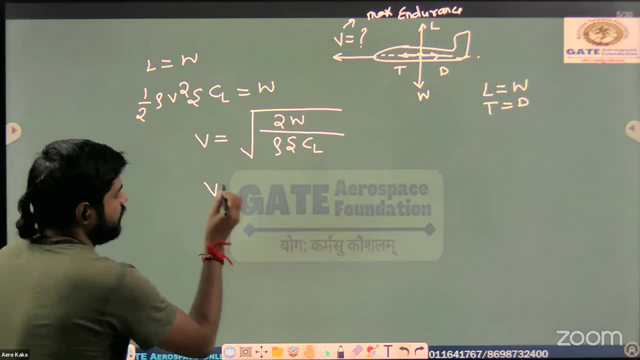 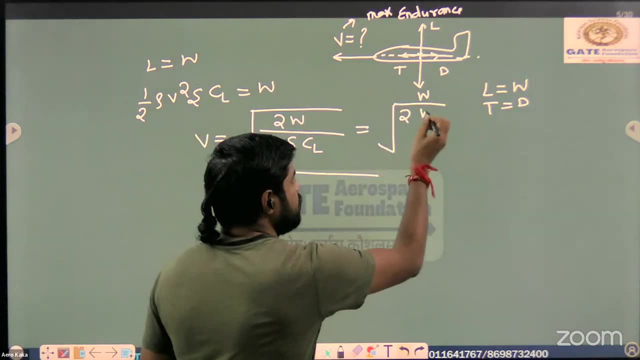 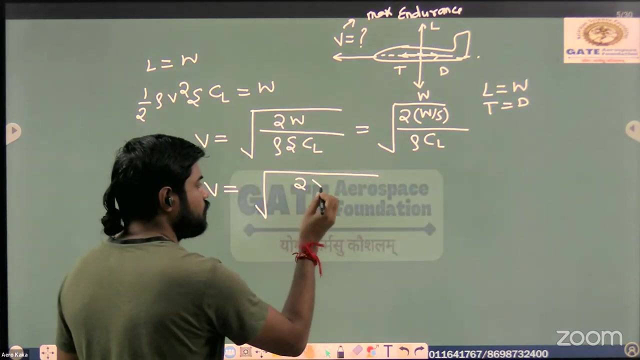 Clear or not. Now we can calculate. in this question the value of W by S is given. So you can write here the 2 into W by S. It is directly given in this question, divided by rho into C, L. Now it is a 2 into what is the value of W by S, or you can see being loading 1800 or 600?. 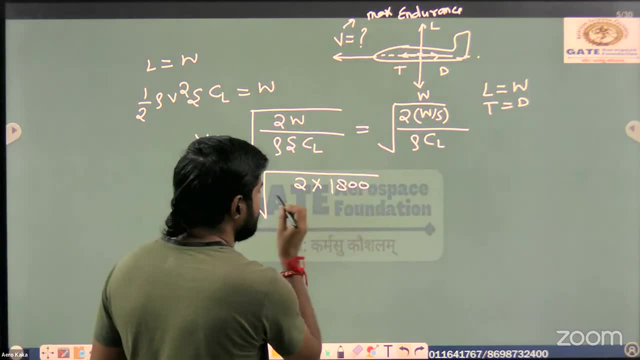 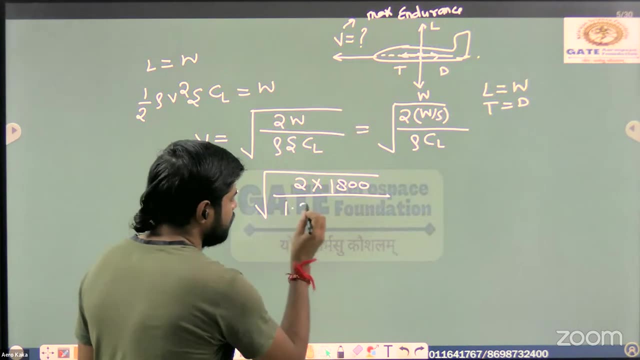 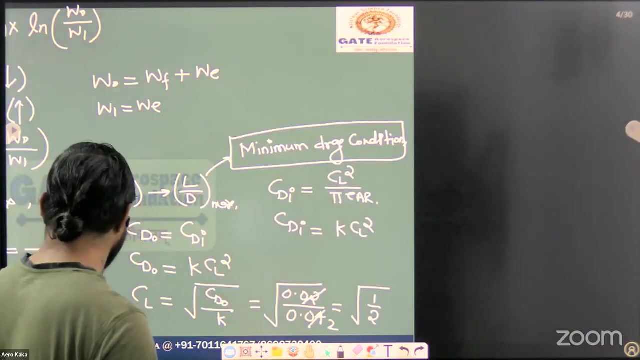 1800.. 1800, right divided by what is the density, they are considering 1.225.. 1.225, okay, into what is the lift coefficient? we are getting 0.07.. We are getting 0.707.. 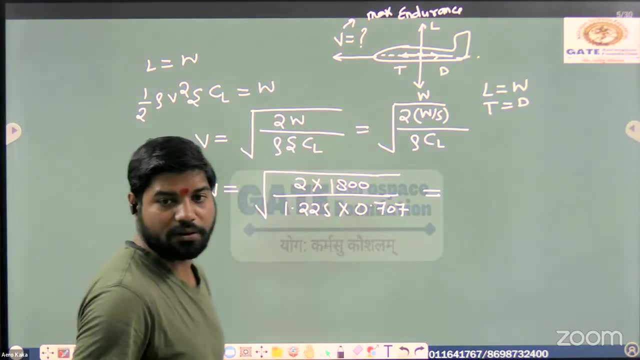 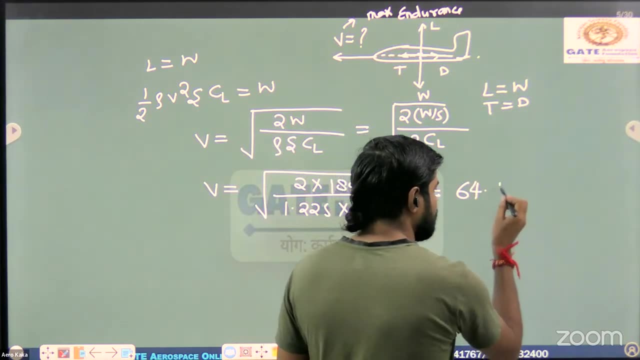 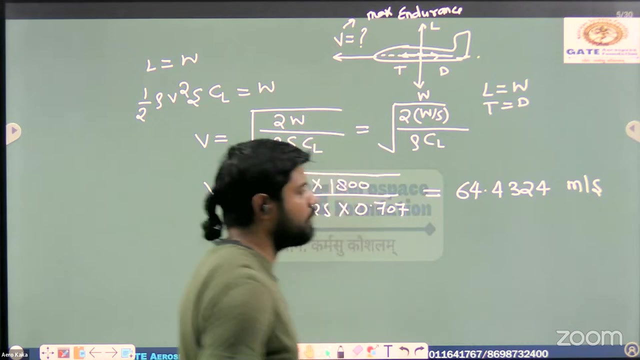 Now just simplify and let me know what is the value of this thing, How much you are getting? 64.47234.. 64. 234.. 47234.. Okay, please come again, Sir. 64.434.. 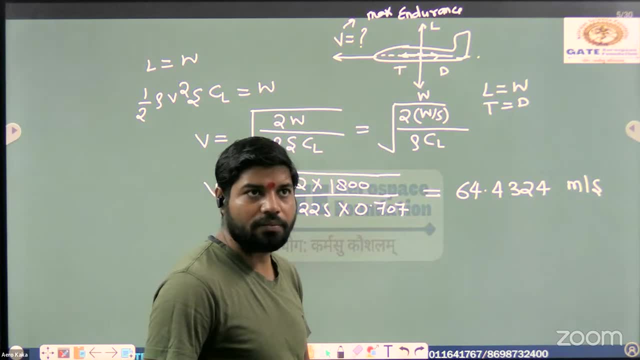 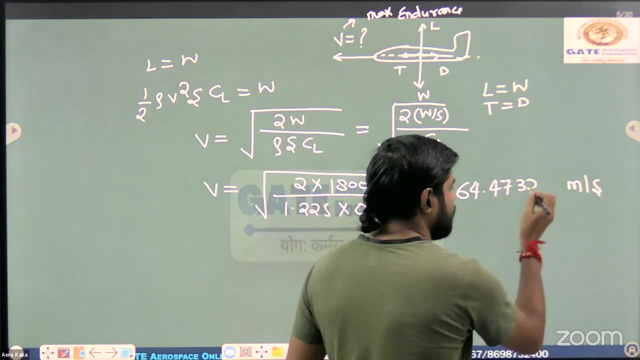 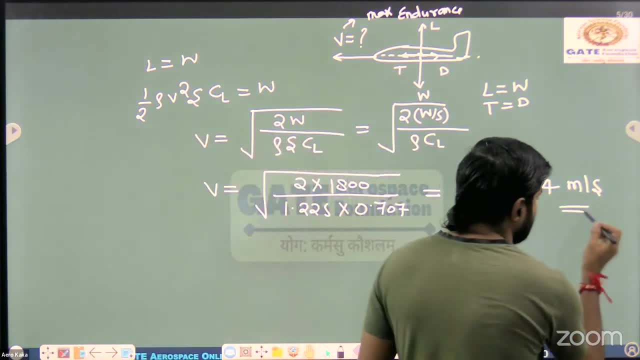 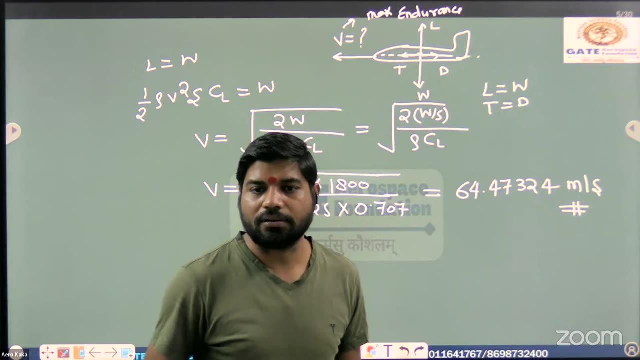 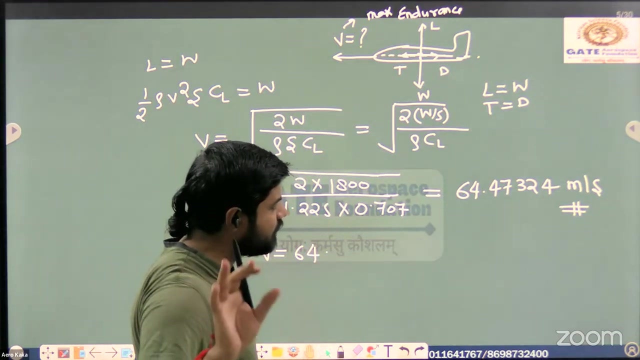 Please verify this value. please verify Hello. Please comment the checkbox, yes or no. Are you getting this one? Yes, sir. Okay, So the final value we are getting, which is equal to how many decimal points we are asking. are they asking the nearest integer or up to the two decimal points? 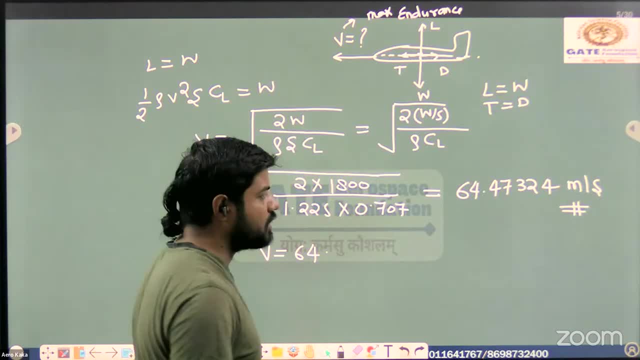 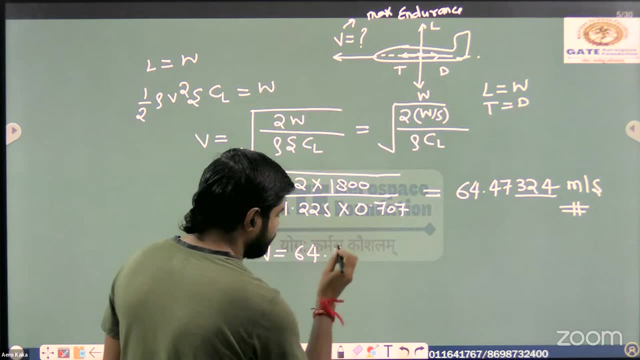 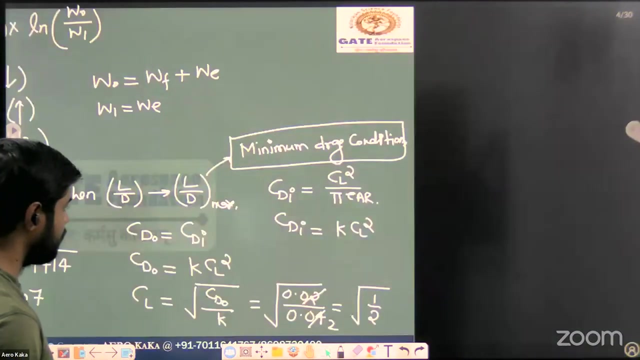 point or three decimal point, what they are asking up to two decimal point, right, so obviously we can neglect these three. we are getting 64.47 meter per second. that's your final value. let's check whether this value is in the range or not. how much we are getting 64.47. so the 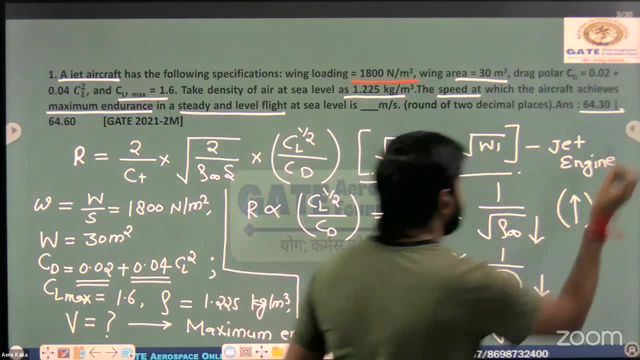 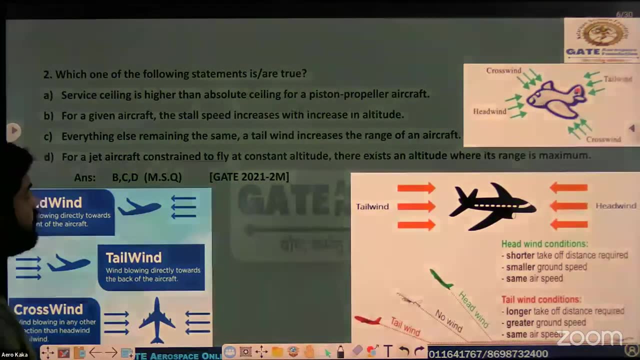 range is given here: 64.30 to 64.60. right now let's discuss another question. this question they have asked in GIT 2021. it's a MSQ type question. they are asking which of the following statement is, or are, true? please consider this one. first one: surveying ceiling is higher. 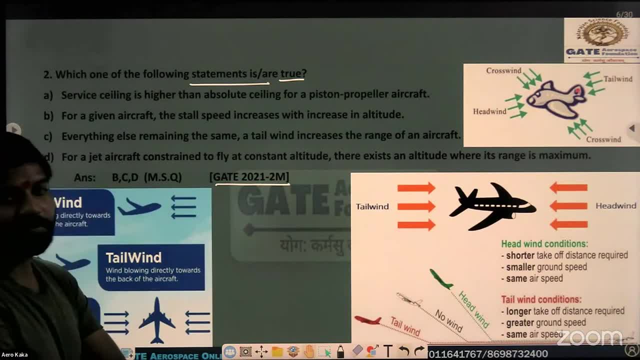 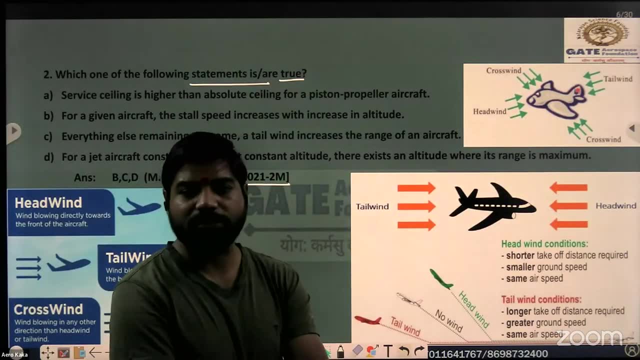 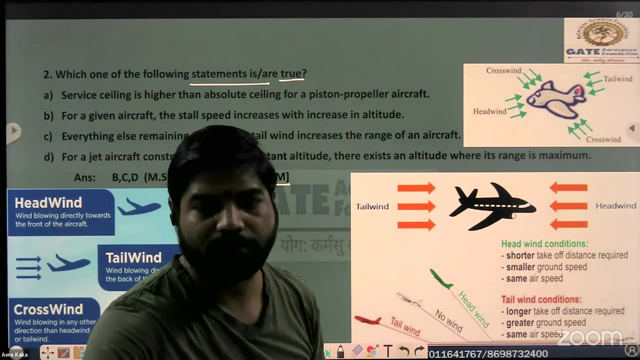 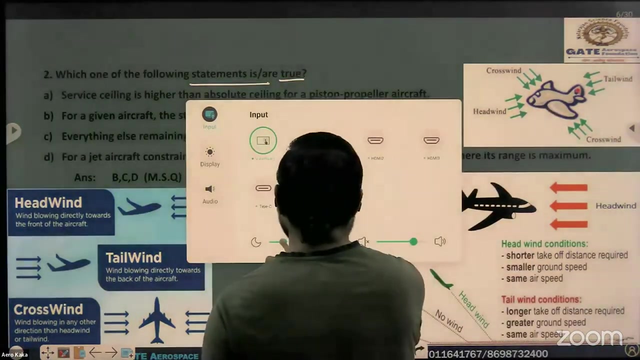 than the absolute ceiling for a piston propeller aircraft. is it true? false, see, doesn't matter which aircraft is this right? the absolute ceiling is higher than what the service ceiling agree. check, please. are you agree or not? yes, sir, your service ceiling is higher than sorry. your absolute ceiling is higher than what. 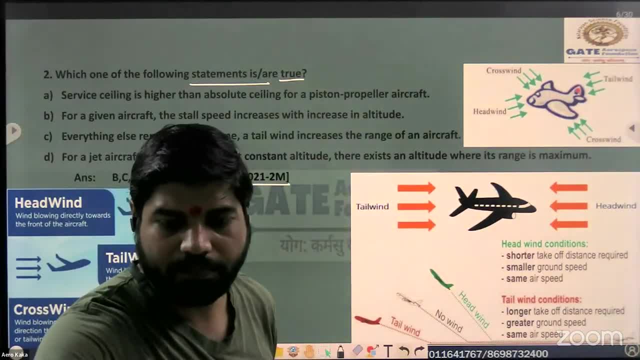 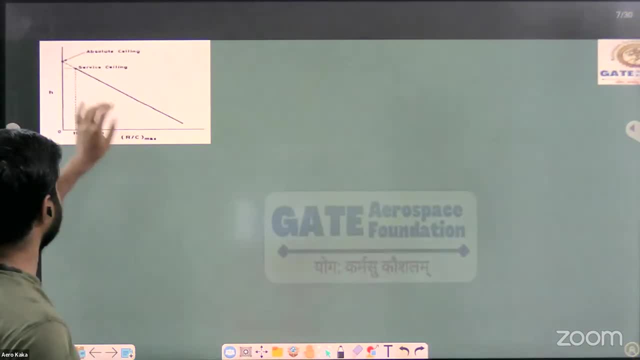 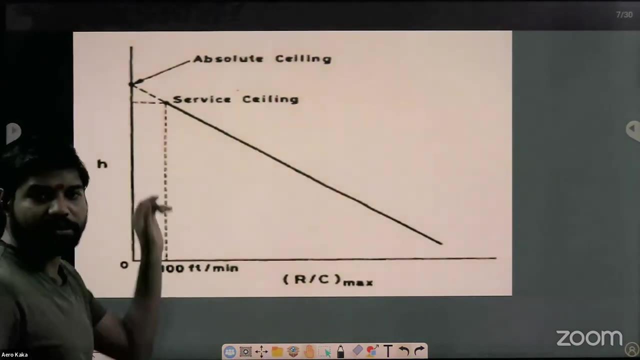 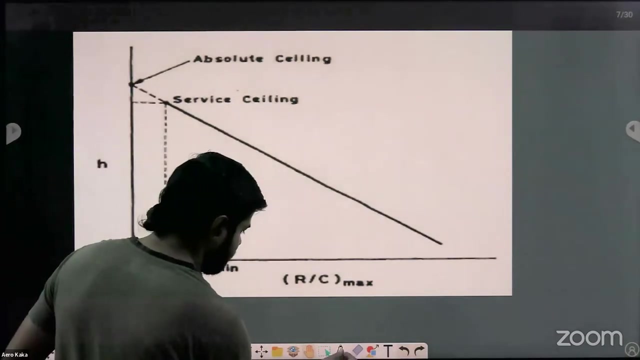 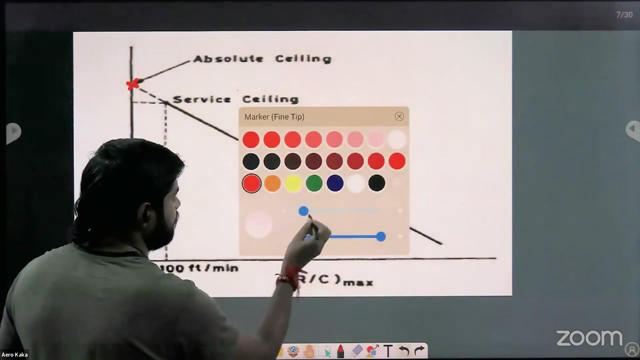 service ceiling value. right, check now let's see what is the answer to this question. but even if you want to check the diagram, then it is something like this: can you refer this one? this is absolute ceiling, service ceiling. here rate of climb is given right and here this point is nothing but the same, that this altitude is nothing, but you can. 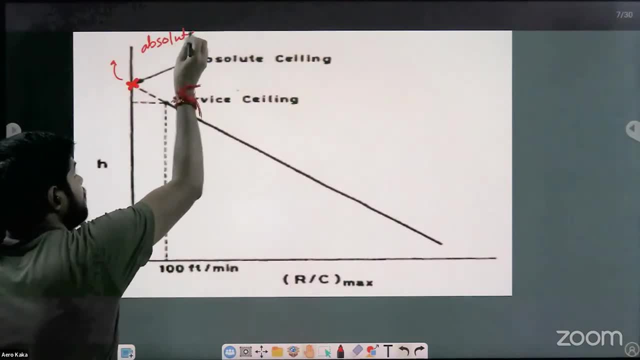 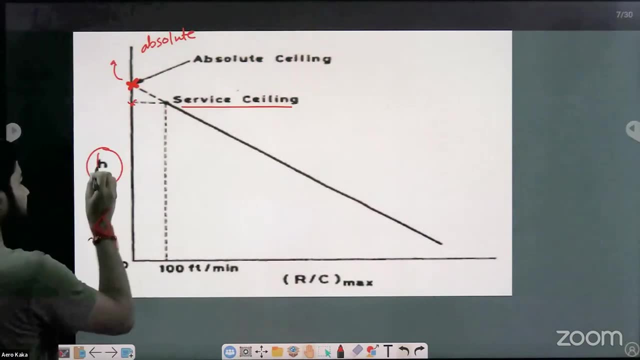 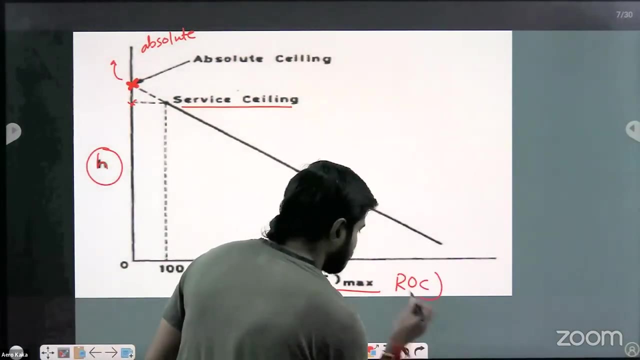 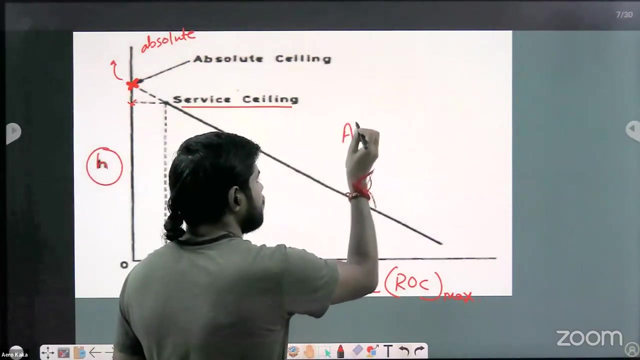 say it's a absolute ceiling, ceiling, and this is nothing. but you can say it's a service ceiling: here, right here, this is what you can say: h, which is nothing. but you can say altitude, here, this is what you can say: it's a roc. max means rate of climb, right. so your absolute ceiling. 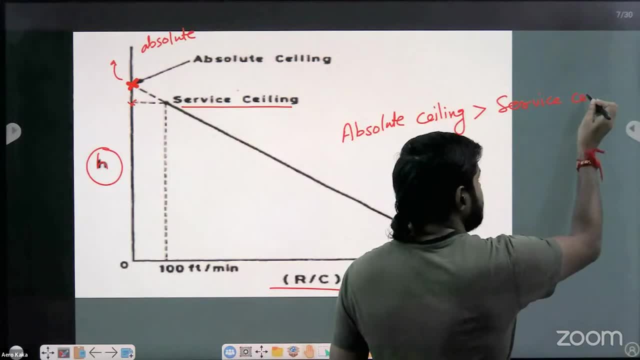 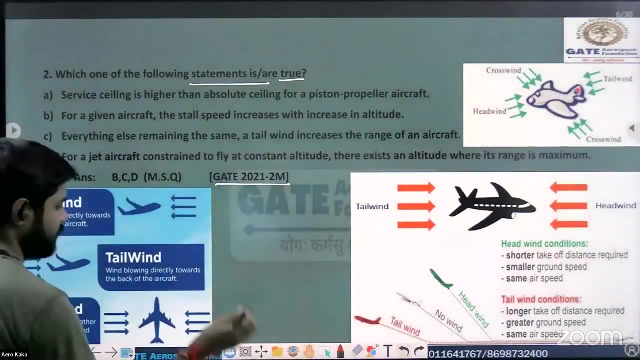 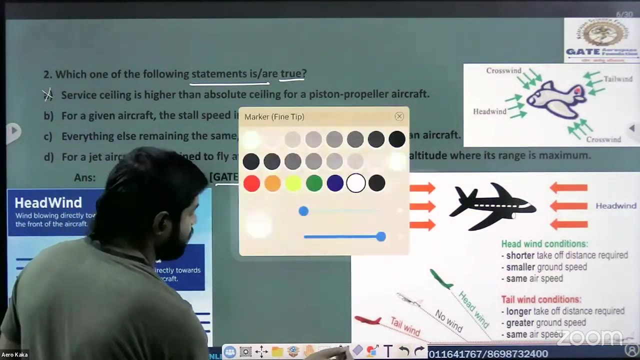 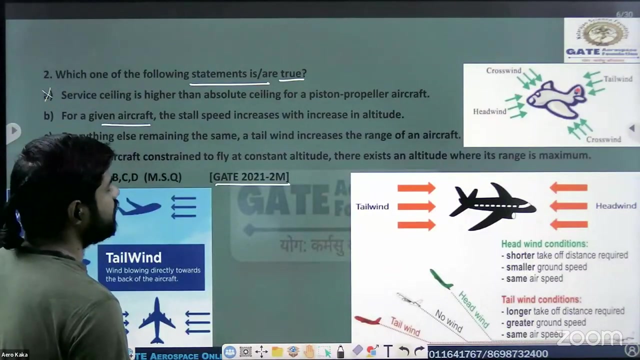 right. so your first option is incorrect. now we talk about the second point. here you are saying for a given aircraft: okay, this tall is speed increases, width increase in altitudes. i think we have discussed this question in last session. i will touch on that as well now. the response rate, which is not confident. 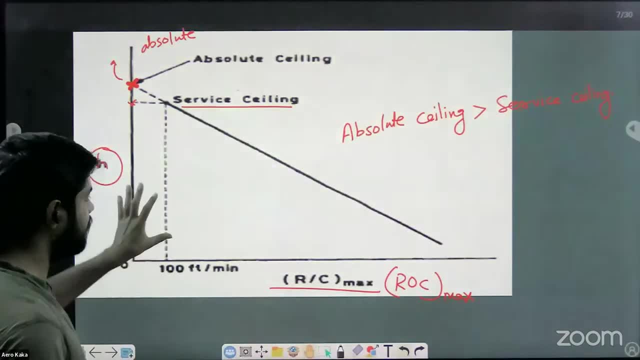 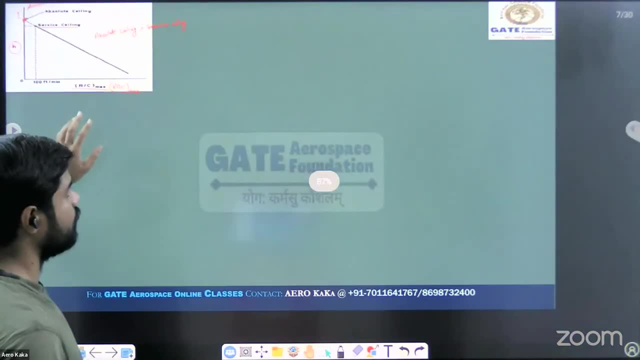 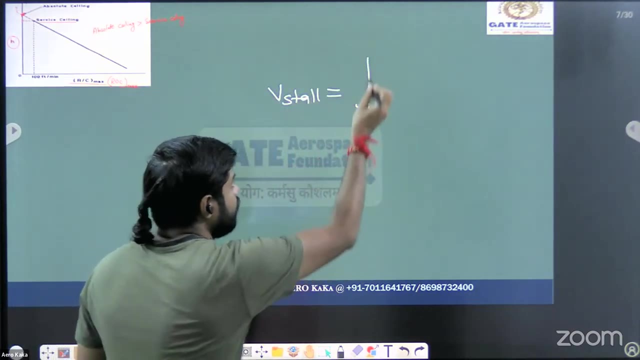 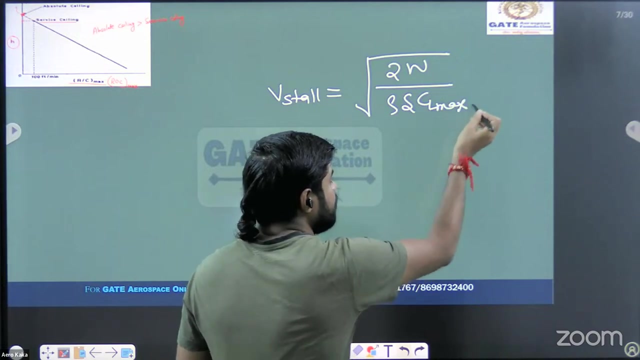 class. right Now, what is our stalling speed? Look the minimum speed at which airplane can. okay, if suppose. if you want, if you write this formula, B stall is equal to root of 2 W divided by rho s C L max right. Clear. Now what are they asking? They are asking. 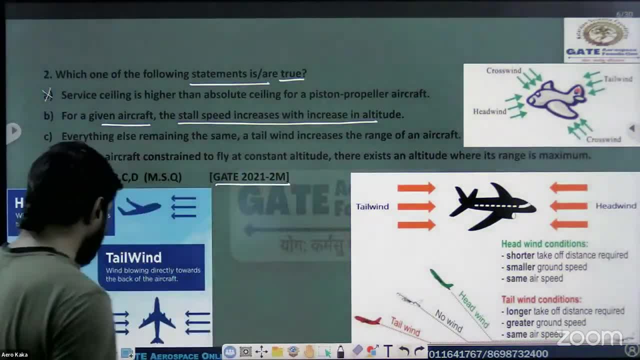 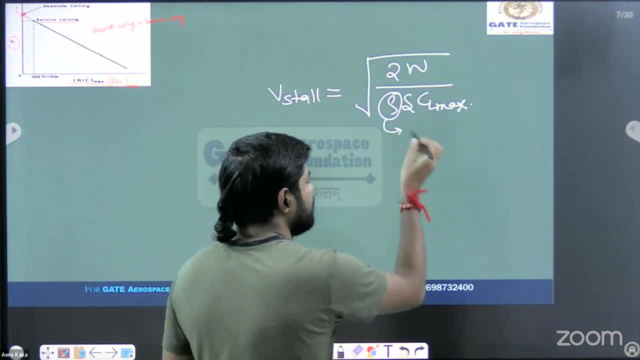 for a given aircraft is stalling. speed increases with increase in altitude. Just comment Now here: this density is the parameter which is associated with the altitude right. Why? Because, as the altitude is the parameter which is associated with the altitude right. Why? Because, as the altitude? 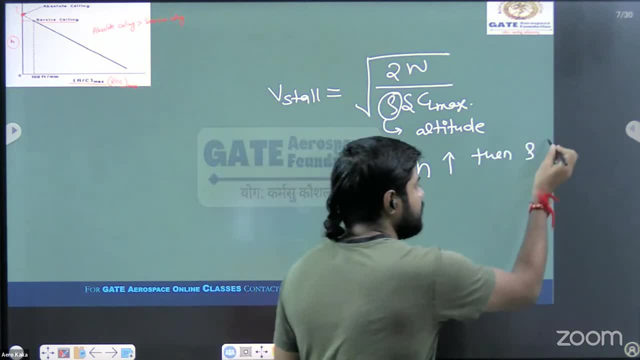 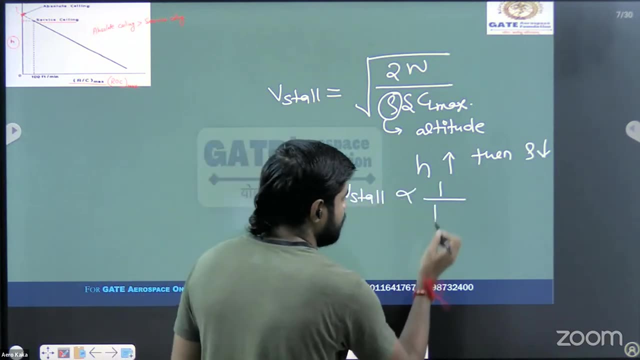 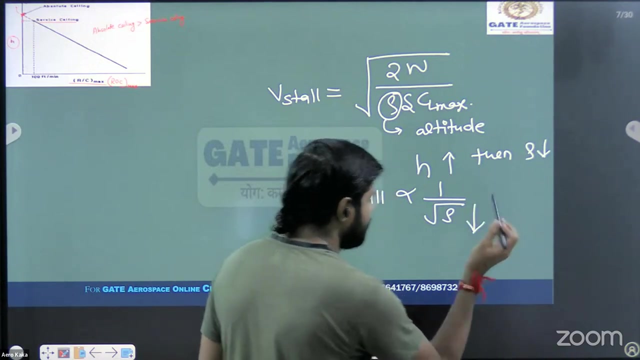 is the parameter which is associated with the altitude right. Why? Because as the altitude increases, then your density decreases. So from here, if you want to write like we stall, here is something like this: So as the entity increases, this density value decreases, then. 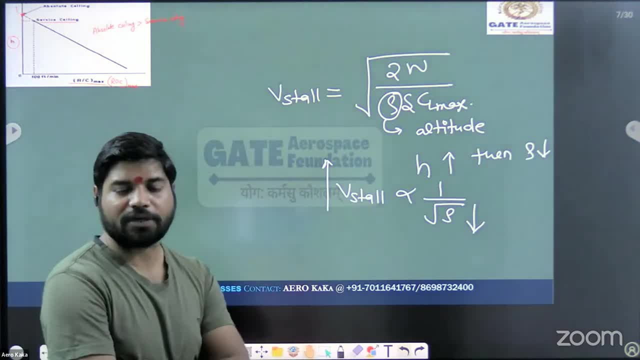 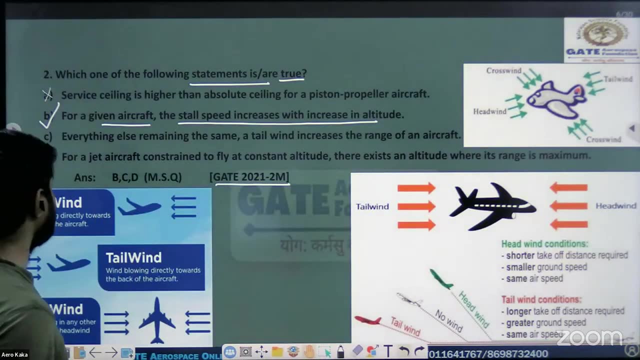 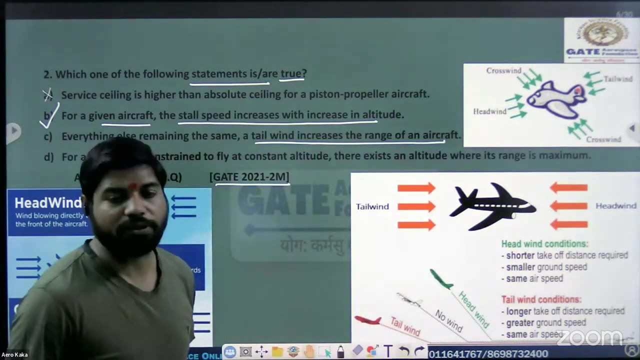 your stalling speed increases right? Check me, Yes, Yeah, So your option B is correct. Second one: everything else remaining the same: the tailwind increases the range of an aircraft. So even I have given one formula right. It's how to calculate the range of. 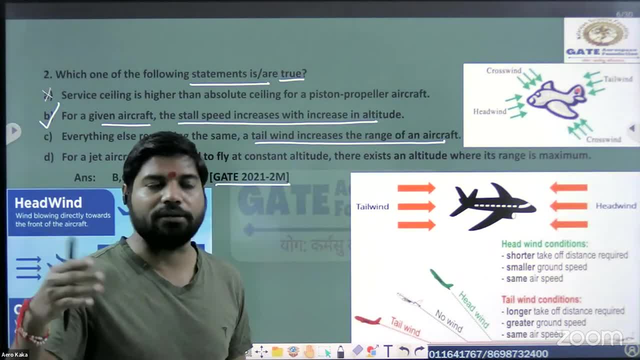 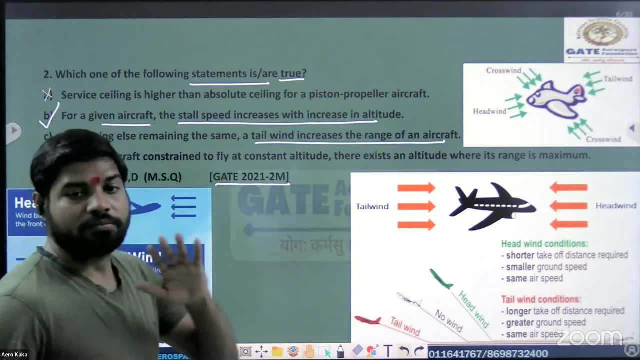 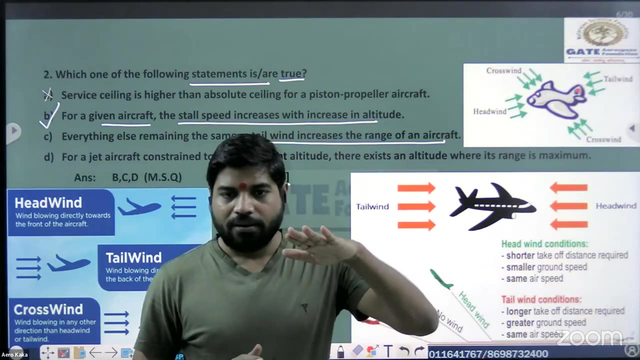 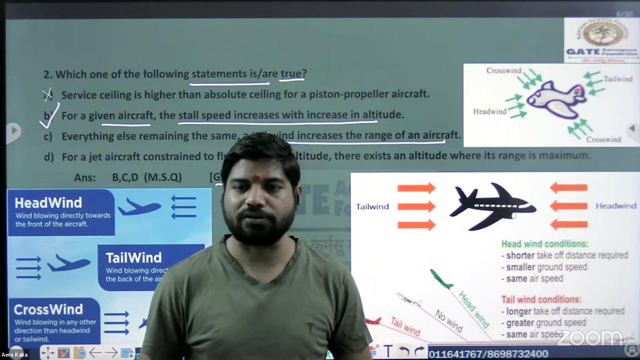 the aircraft in wind right, Or you can say in wind model, or you can say with zero wind model right. So here you should have to remember like during the takeoff and landing, right During the takeoff and landing. during the takeoff and landing, your headwind is the favorable right. Say yes or no. 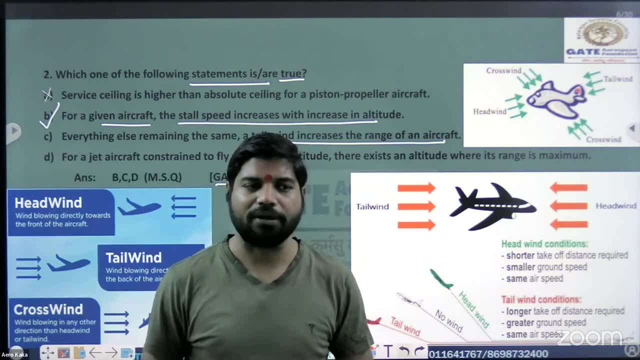 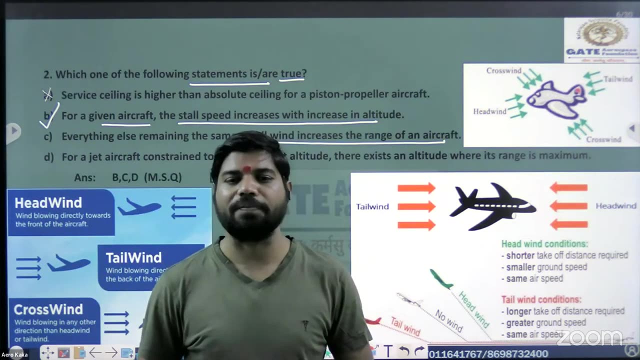 Yes, sir, Let's discuss one more time here. During the takeoff and landing, headwind is preferable. or you can say: headwind is favorable, But during the cruise flight, or you can say: during the steady-state and level flight, what happens Anyone, Your tailwind is the. 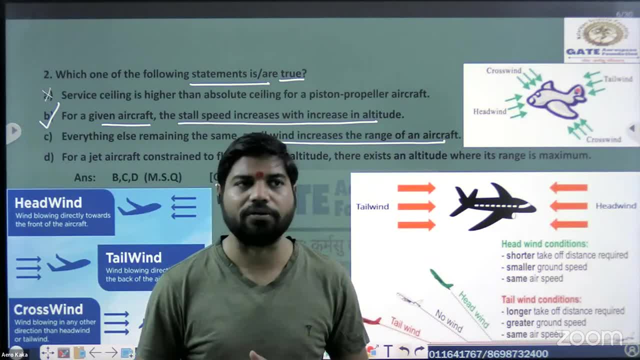 favorable. Yes, So that's the reason why it increases the range of the aircraft, Because, you know, the range of the aircraft is not a function of the airspeed, but the range of the aircraft is a function of the ground speed. right Check, please. Are you getting? Please go. 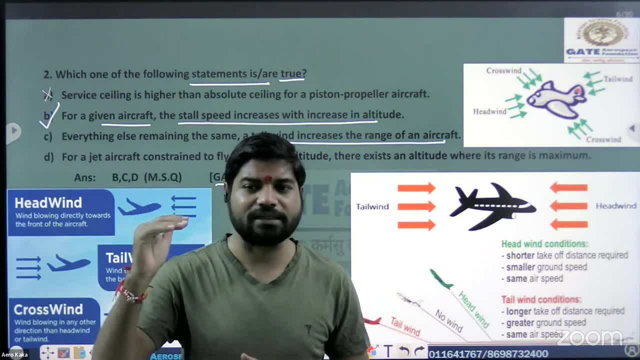 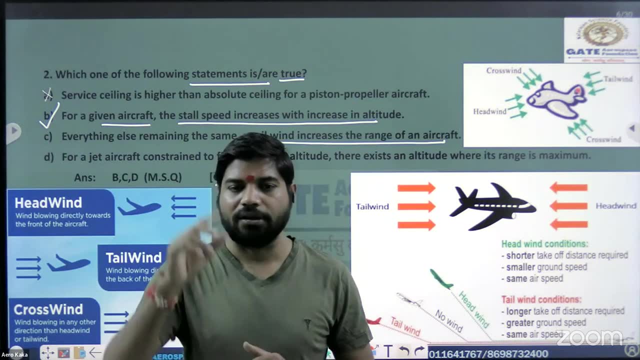 through the formula. Are you getting this or not? Please wrap up notes properly. Please keep devising as much as you can Clear. The range of the aircraft is depends on the airspeed. Yes, Okay, Yes, Okay Okay. 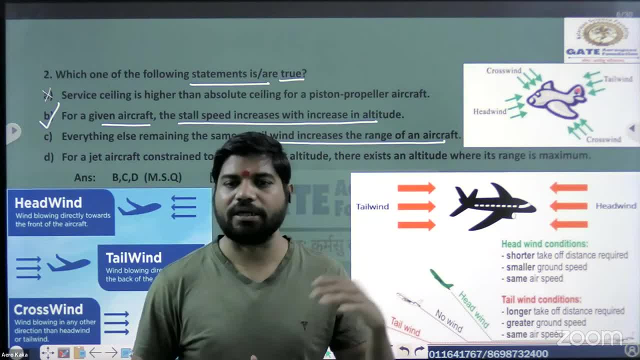 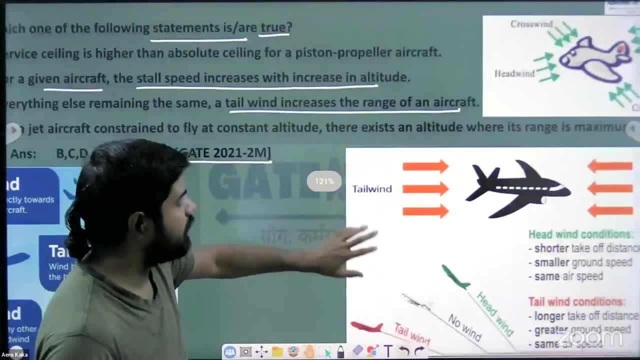 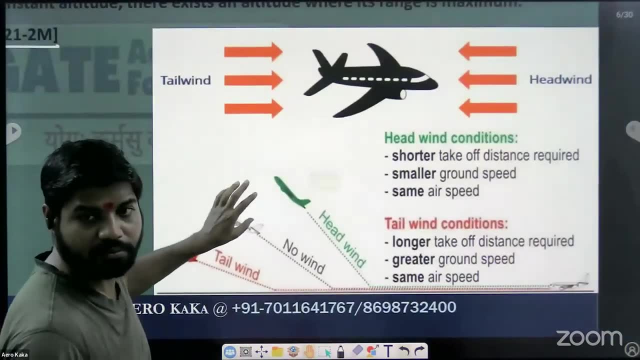 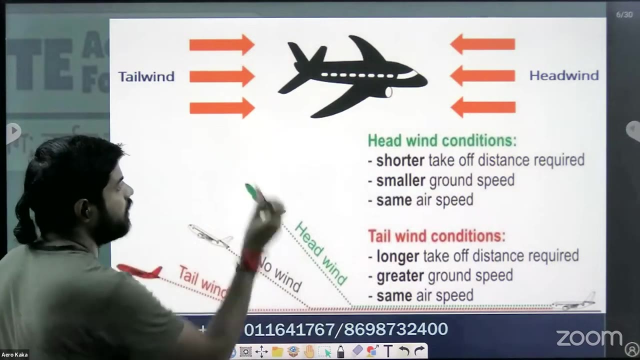 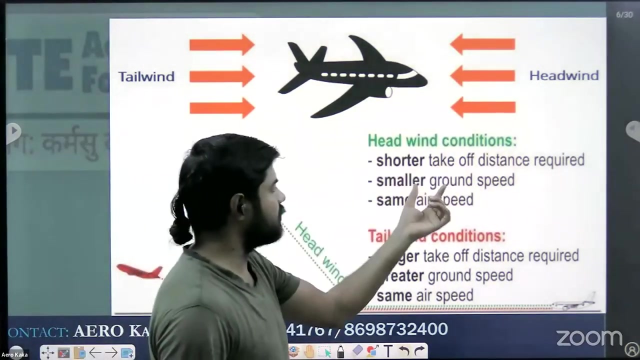 a tailwind. Let me explain this one also here. Let's say: this is the aircraft, right? Is it visible to you, Is it Okay? So let's say we can consider two cases here. One is tailwind And this is nothing, but you can say headwind here. Now this is another diagram, So headwind. 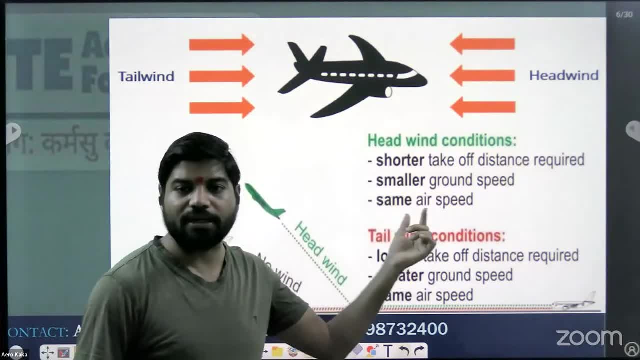 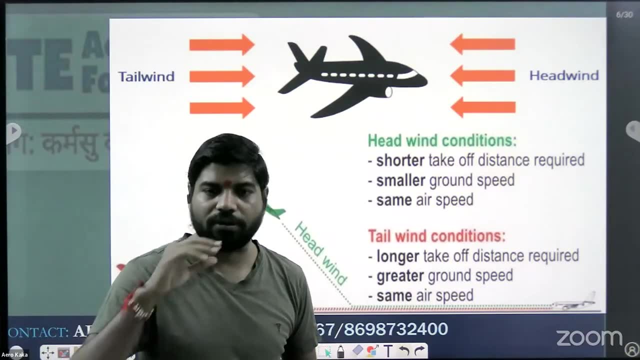 distance you can see during the time of takeoff. it requires a shorter takeoff distance required. or you can say: if suppose, if the aircraft is, if aircraft encounters the headwind, then the takeoff distance will be shorter. Second one: you can see a smaller ground speed and 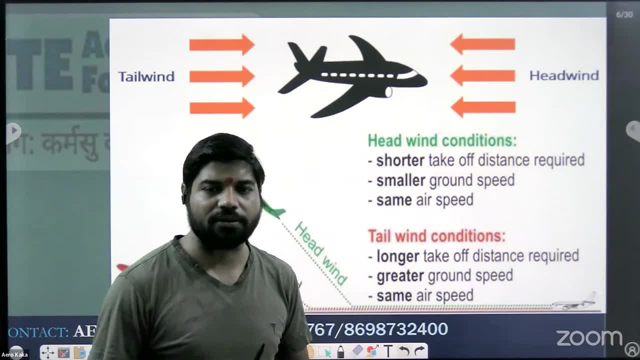 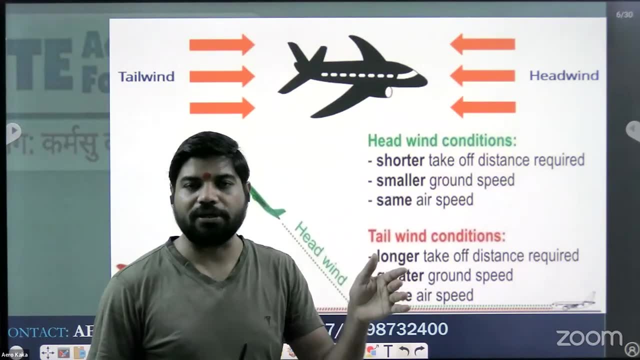 here. there is no change in the air speed of the aircraft. Is that clear? Please take care. There are two velocities or you can say speeds. One is ground speed, That's we define BG. Another one is what, Another one is nothing. 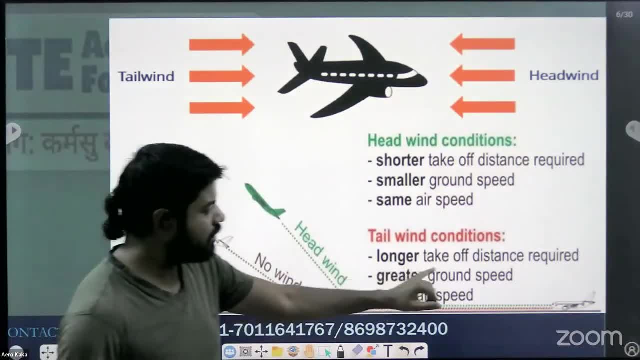 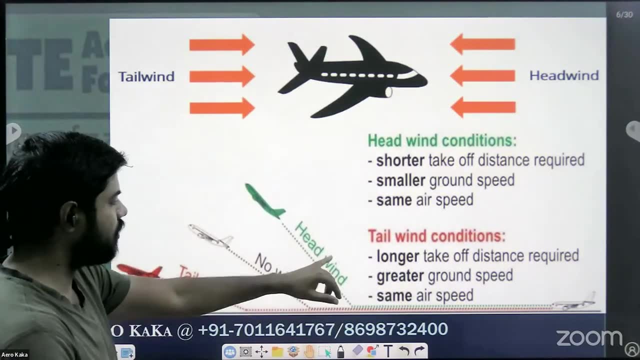 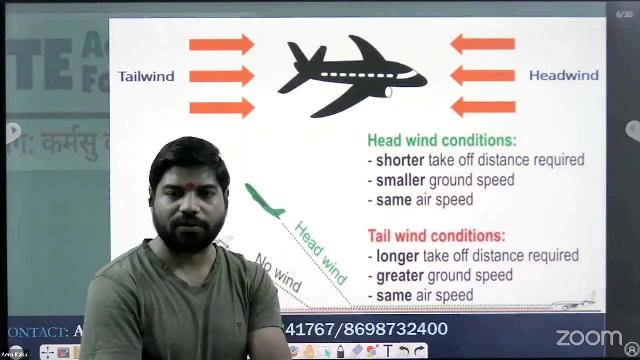 but you can say air speed. Then again, for tailwind, longer takeoff distance required greater ground speed and same air speed. This is for what. This is for the tailwind conditions. Is that clear? If suppose, during the time of takeoff, if suppose there is a tailwind. 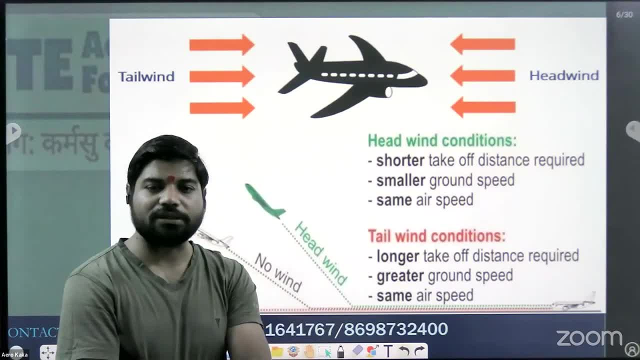 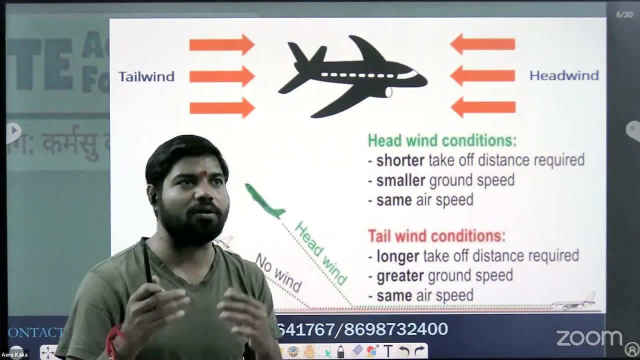 then the takeoff, then the takeoff distance will be shorter. So this is the tailwind distance. The takeoff distance will automatically increase. The reason is what You know. we have discussed few examples or you can say numericals in the class like how this takeoff distance. 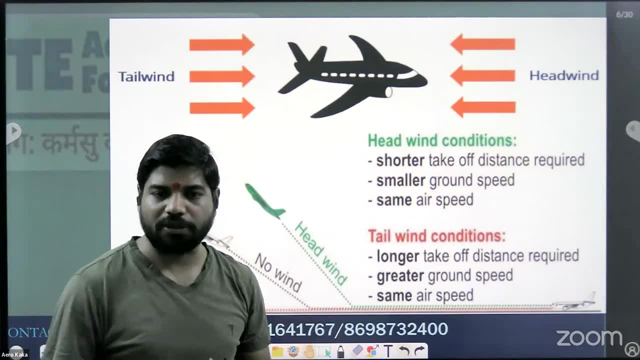 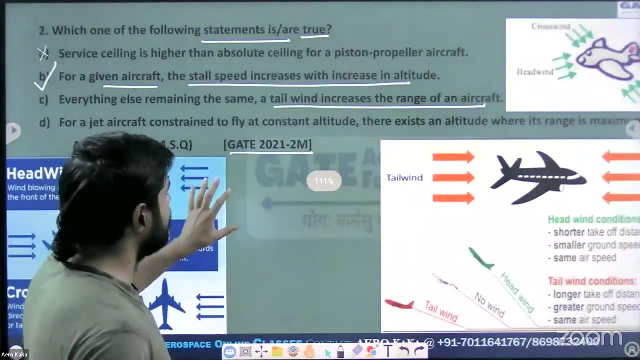 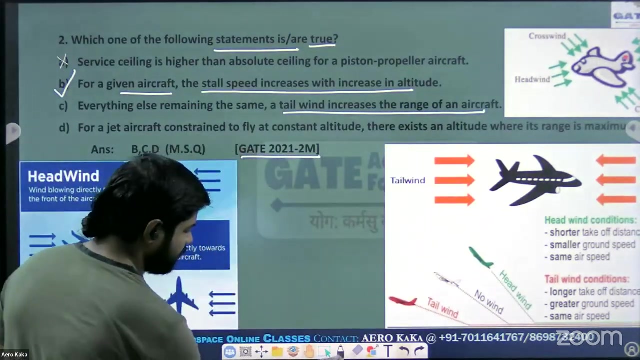 is is associated with the- you can say the ground speed of the aircraft, right? Or what is the effect of the wind on this takeoff and landing distance? So please go through the class notes, Everything else remaining same. The tailwind increases the range of an aircraft. Yes, that's. 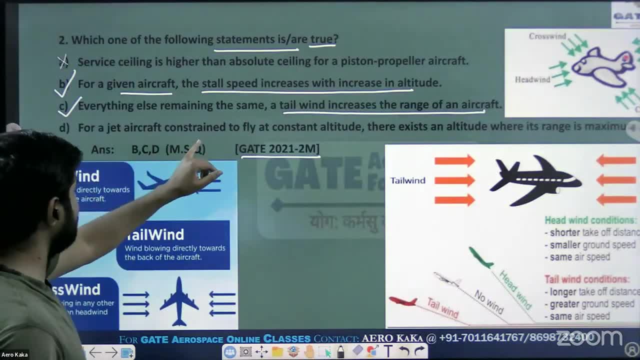 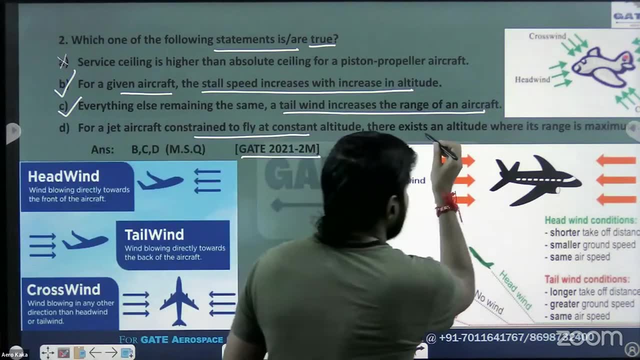 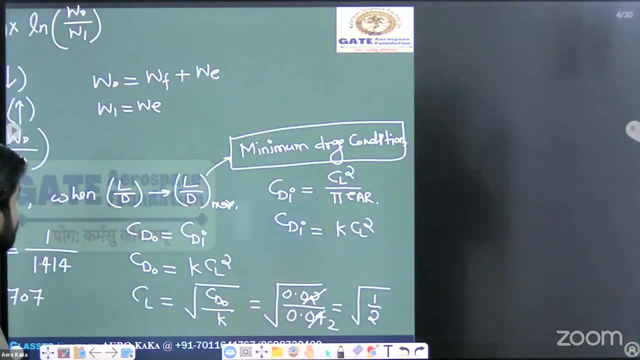 correct Option D for a jet aircraft. for a jet aircraft, constant to fly at constant altitude, there exists an altitude where its range is maximum, Right? So just go through the previous question Now look carefully, This is our range of aircraft. 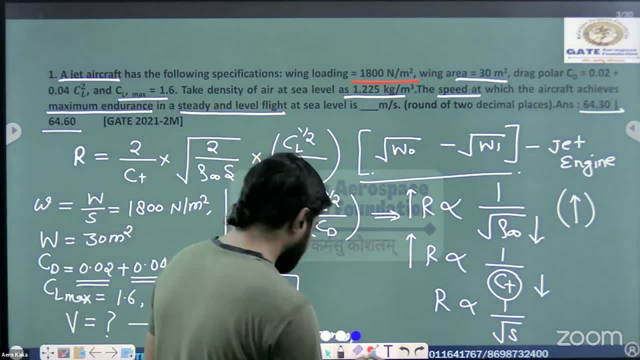 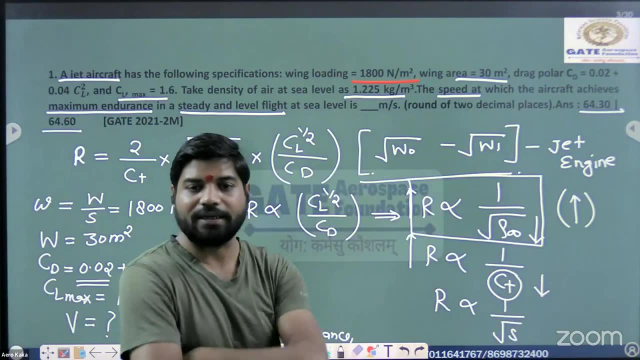 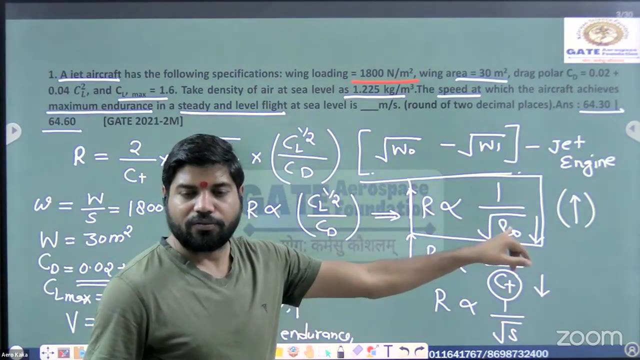 This is our range of aircraft, formula right Check. So our range here, range of the aircraft is, depends upon what. It depends upon the density. Say yes or no. Am I audible? What is this density here? This density is directly associated with the altitude of the aircraft, So as the altitude increases, then the ambient density decreases. If the ambient density decreases, it means that what The range increases, But there is a certain limit, or you can say depends upon your power plants, like how powerful it is or whether it is producing the required amount of the thrust at higher. 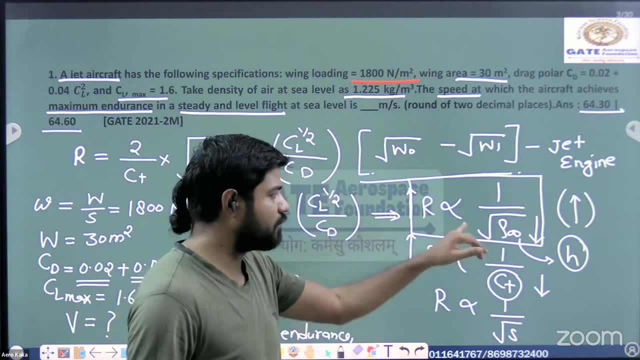 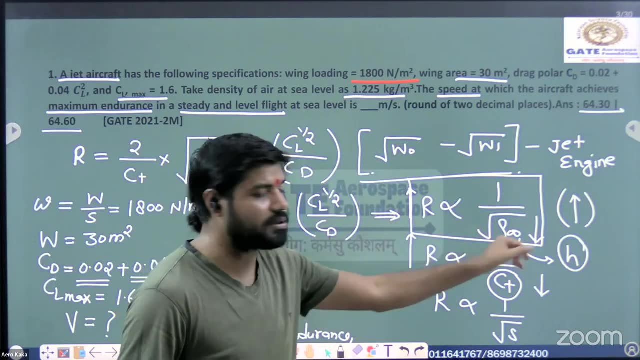 altitude or not. So during the design phase itself we have to decide, like, what should be the maximum altitude, or you can say absolute ceiling, as well as the service ceiling of the aircraft. So we have to take care of this density value also. Okay, So the option D is also. 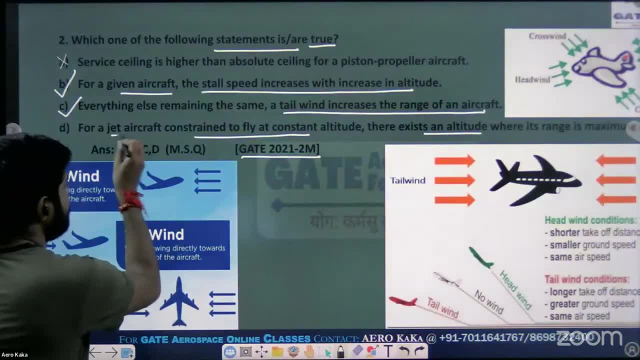 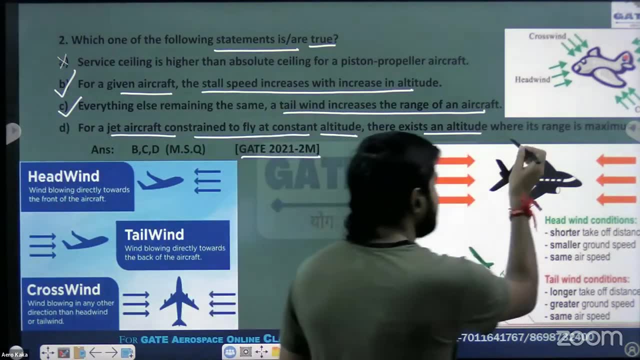 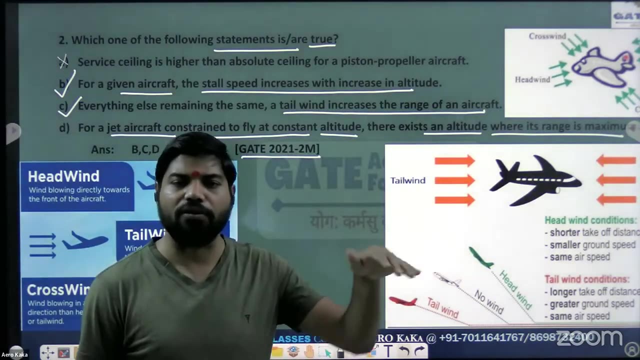 correct. For a jet aircraft especially, it is written: it's a jet aircraft, constant to flight at constant altitude. there exists an altitude where its range is maximum. Yes, So it means that what If? suppose if you are flying a jet engine aircraft near to the ground? obviously, 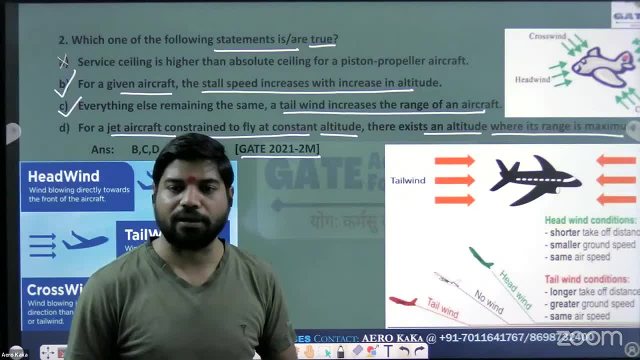 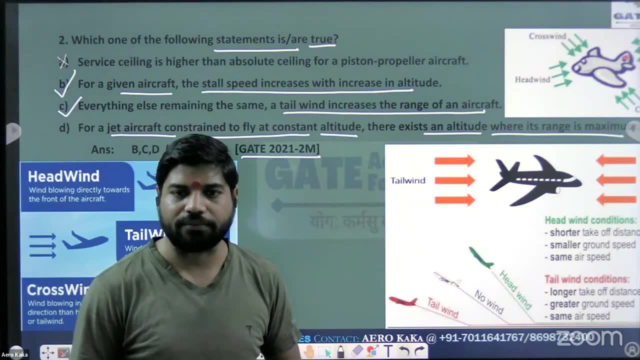 its range will decrease. Can you relate? Hello, Yes, Can you relate? Yes, By keeping all the parameters same. So here, option B is the range of the aircraft. So if you are flying a jet aircraft, essentially, if you are flying a jet aircraft, essentially if you arejumping, 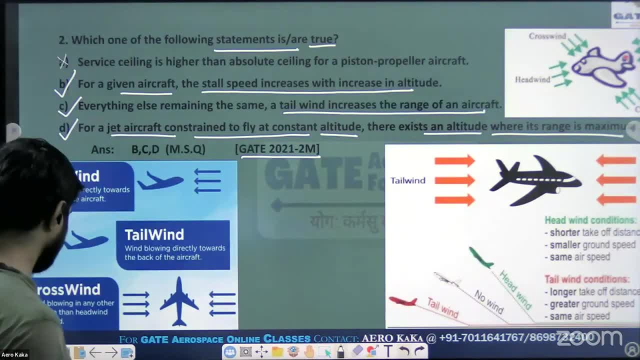 the aircraft. actually, things are different, right? So you will need to actually calculate the range of the aircraft and what is the range of the aircraft, as well as to calculate the range of the aircraft. Okay, So this is the explanation, like: what is a headwind, then what is a tailwind, and 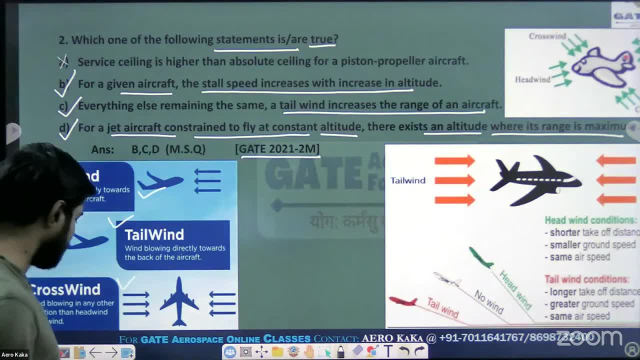 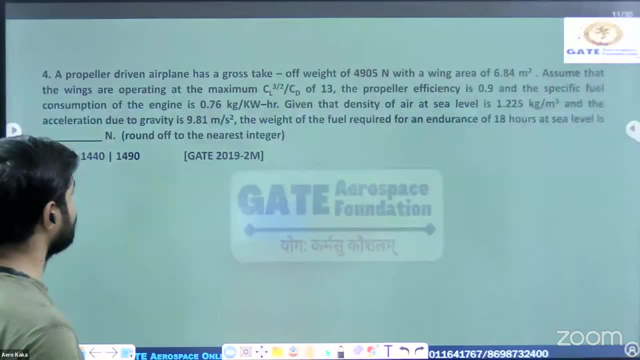 what is the crosswind? Okay, We have drawn these all diagrams during the live lectures. Now, next question: A propeller-driven airplane has gross takeoff weight of 4905.. What is the take-off weight of 4905?? This is the correct answer. 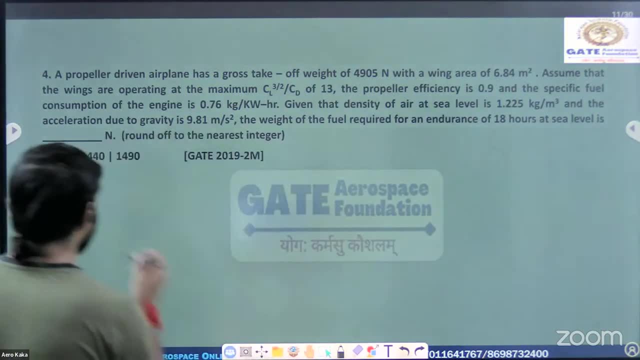 The propeller-driven airplane has gross take-off weight of 4905.. What is the take-off weight of 4905? What is given? here You can see gross takeoff weight: W naught is given. Which airplane is this? It is a propeller driven airplane. Takeoff weight is given 4905 newton. 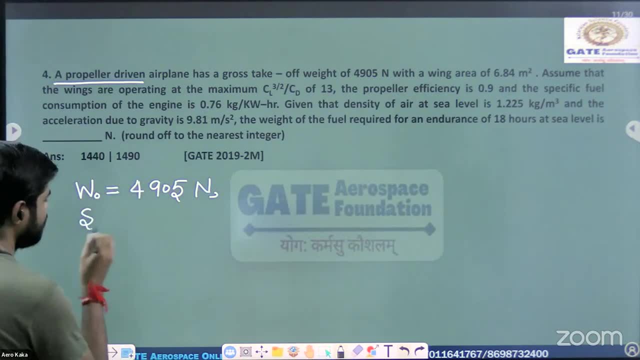 Then the bing area is given here 6.84 meter square. Then assume that the bings are operating at maximum CL raised power 3 by 2 upon CD of 13. What is given here, CL raised power 3 by 2 upon CD max, is given here 13.. 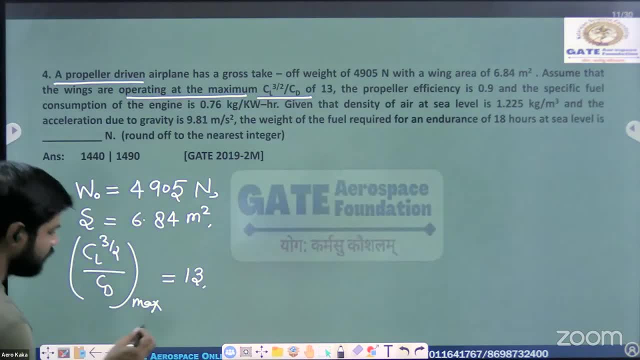 The propeller efficiency is 0.9.. Your propeller efficiency, eta p, is given 90%. Okay, Then, and the specific fuel consumption of the engine is 0.76 kilowatt per hour. So what is given here You can write C, is given here 0.76 kg per kilowatt hour. 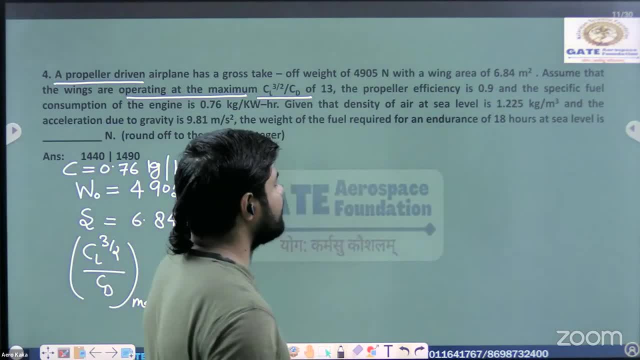 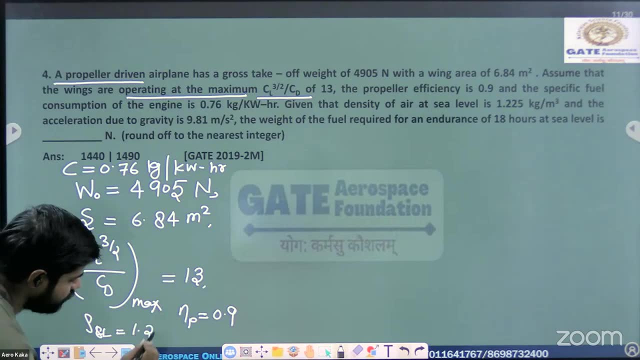 Okay, Then, given that the density of the air at sea level is 1.225.. So density at sea level is also given 1.225.. 1.225.. So density at sea level is 1.225 kg per meter cube. 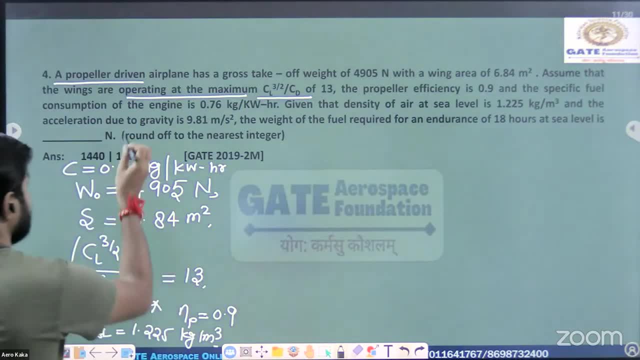 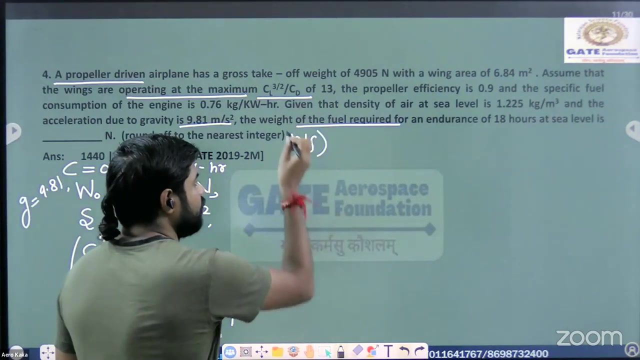 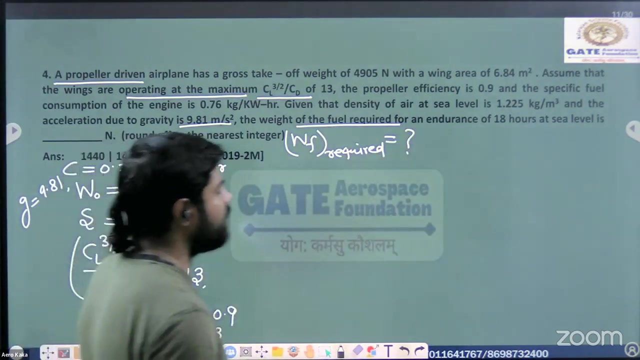 And the acceleration due to gravity is 9.81.. So G is given here, 9.81.. Okay, The weight of the fuel required. You are seeing you are asking, like, what is the weight of fuel required For endurance of 18 hours? 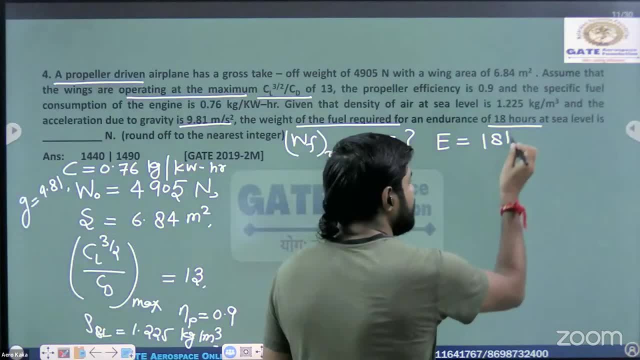 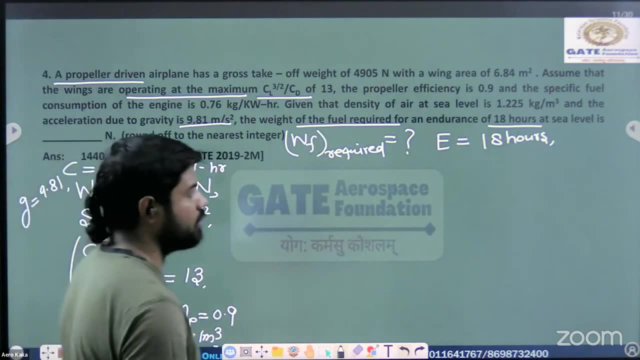 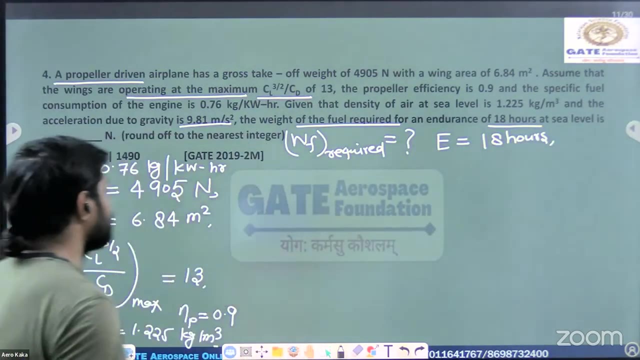 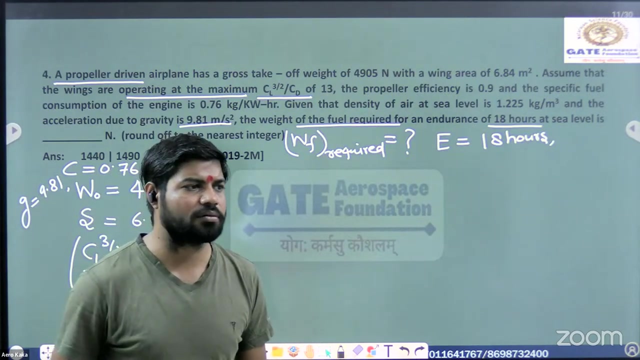 So endurance here, given 18 hours under sea level conditions in Newtons, they are asking, Yes, How to approach this question. You know, most of the time I have seen during the semester exam right As well as end semester exam, or when I used to, means check. the means answers means copy. 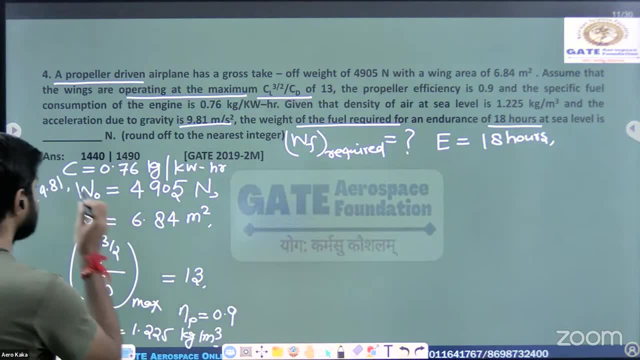 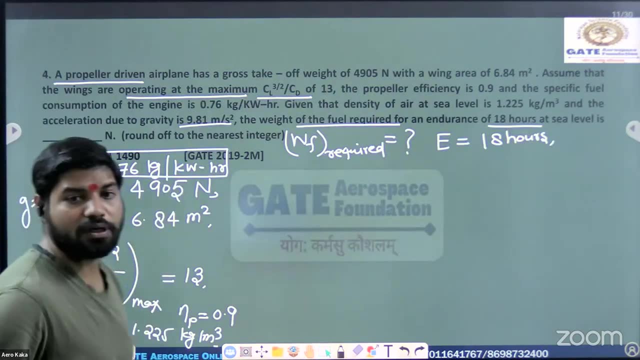 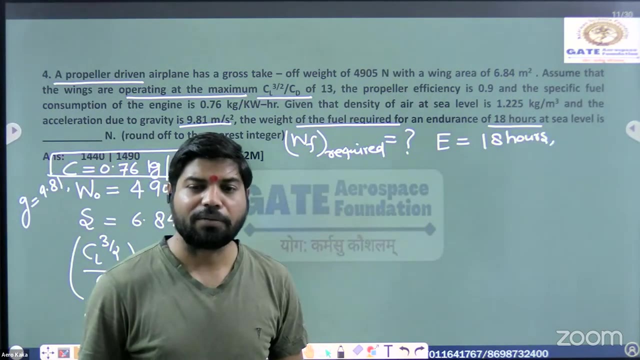 I have seen most of these students generally make the mistake at this particular point only. They generally take this values in pv's only because they are used to of this C value in propulsion, right? Am I audible or not? So here, while you are using this formula, endurance formula, please make sure all the units should. 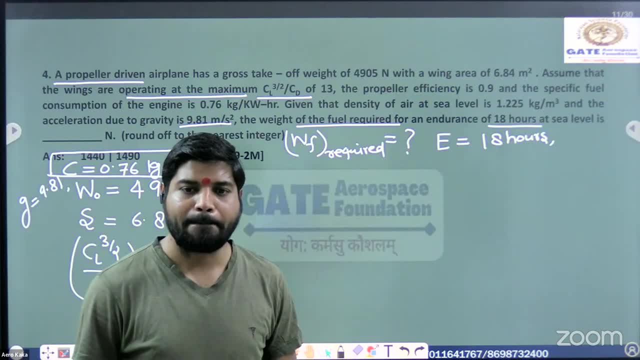 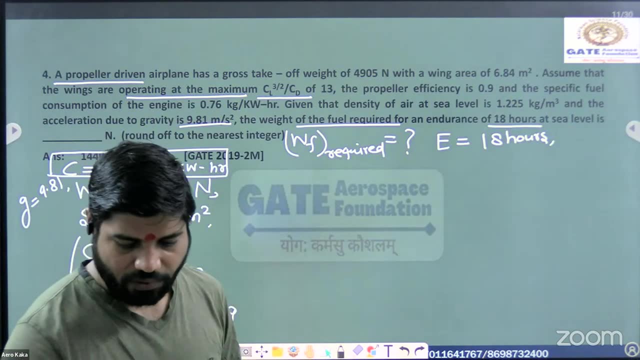 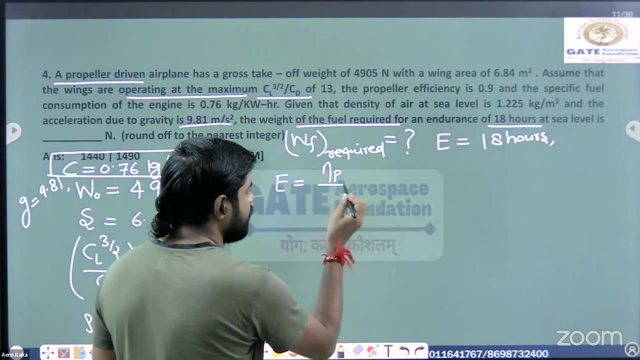 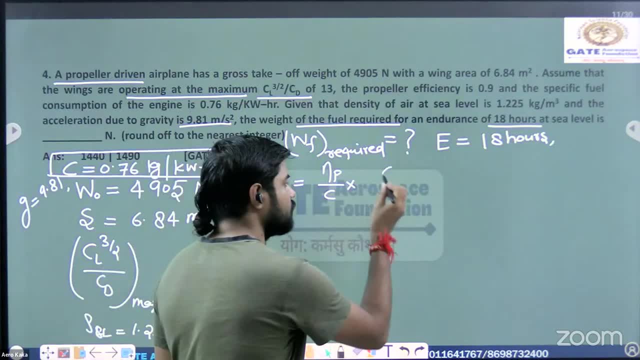 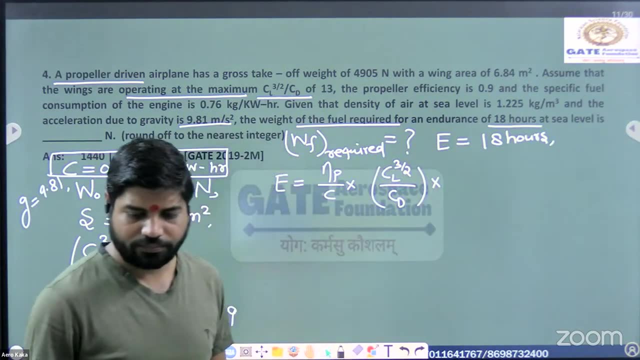 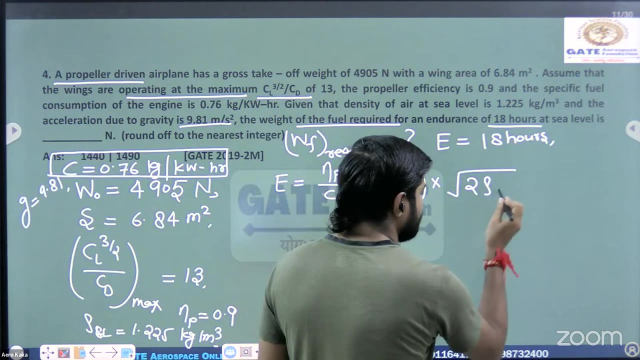 right, Yes, sir, Into what is the next term? Root 2: rho infinity into S. Okay, Okay, Okay, Okay, Okay. So this is eta P throughout. root root two: Yes, Yes, Into how much? One upon. 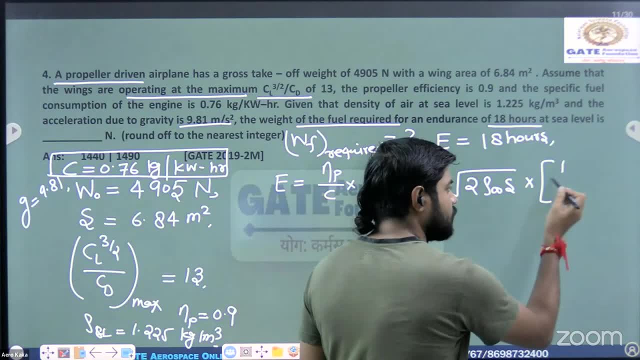 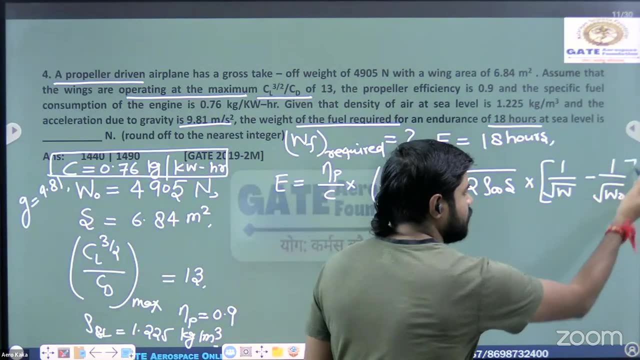 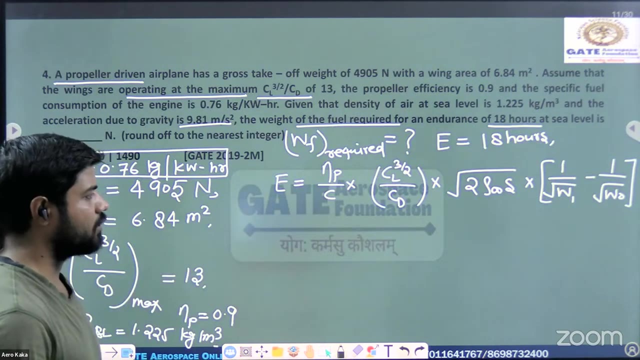 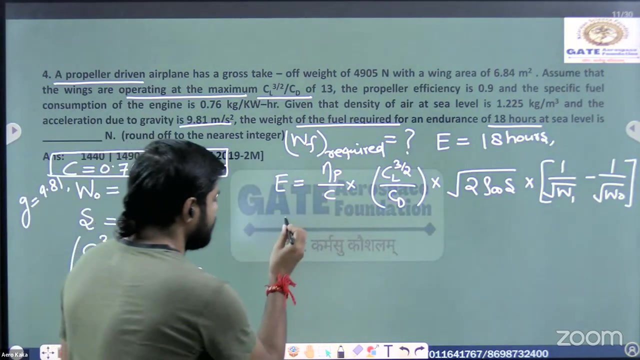 One upon root w minus one upon root w naught Right. That's a formula. Now, even if we look at the endurance of this aircraft, right, particularly for this propeller driven airplane, this E is proportional to what Proportional 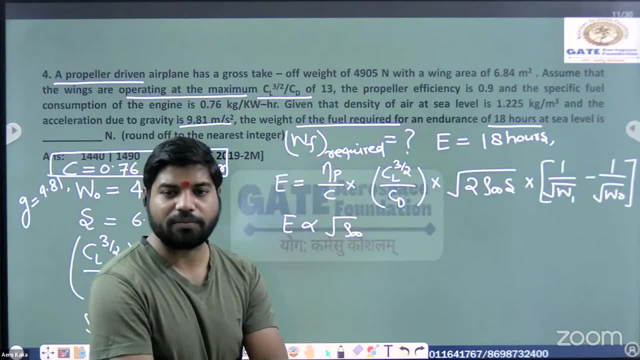 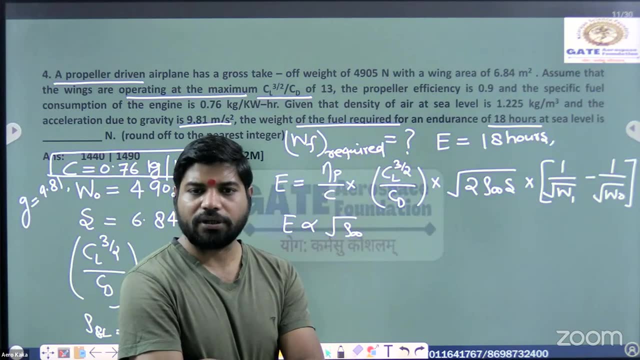 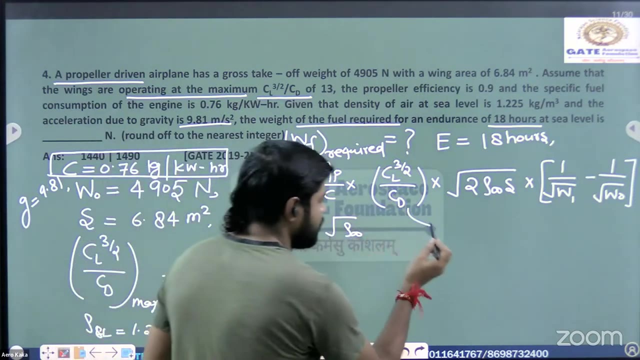 to rho infinity Right Check. It means that what If suppose, if you are flying the, if the pilot is flying this propeller driven aircraft means near to the ground- then definitely its endurance will increase. Right, Then if suppose, if you want to maximize the endurance, 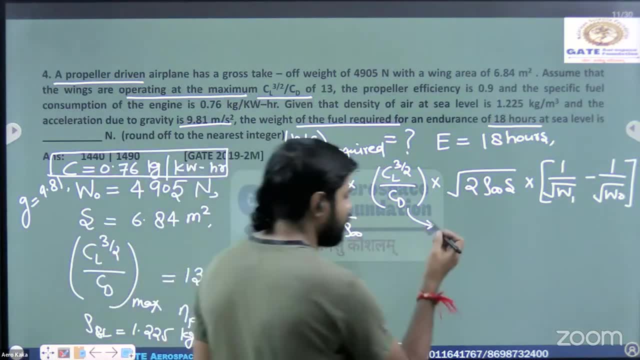 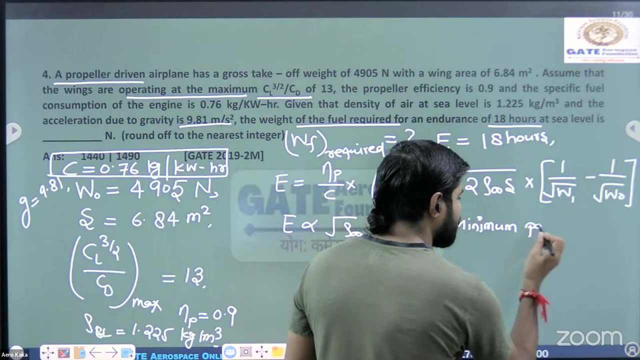 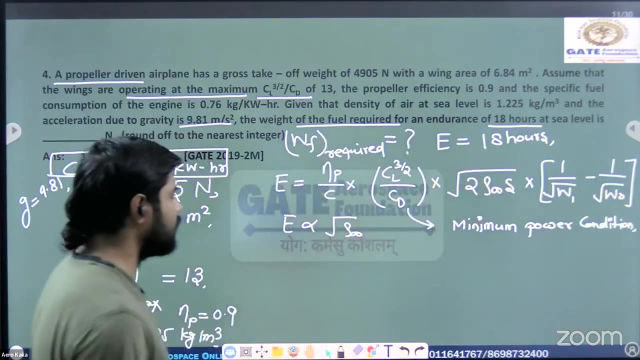 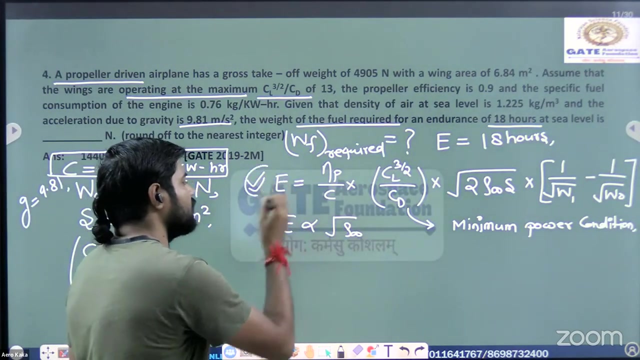 of this propellant based aircraft, then we have to fly this aircraft under minimum power condition. Under minimum power condition- Right Check please. Then obviously the propulsive efficiency- sorry, propeller efficiency- is high. then the endurance will also increases. 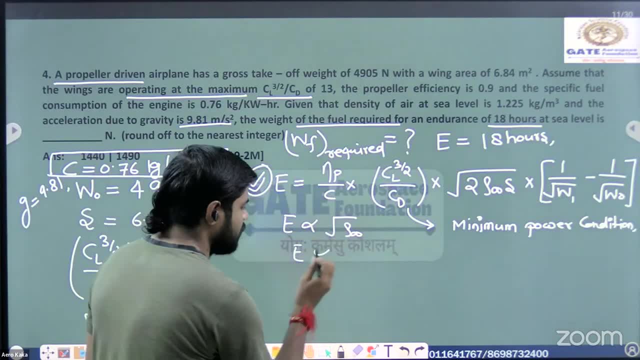 Okay, Now again, this E is proportional to rho infinity, Something like this. It means that what If the value of C is decreased? then the endurance is also increased. But the question is that, how to approach this one? Anyone? How to approach? 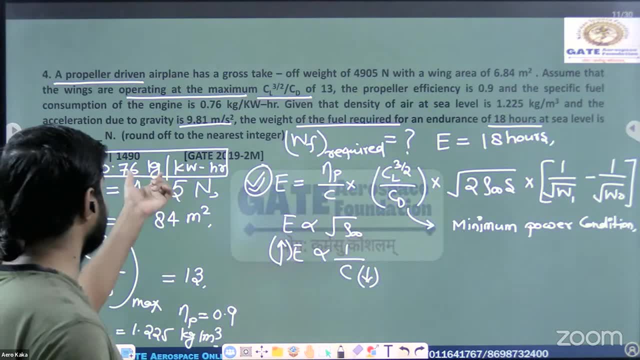 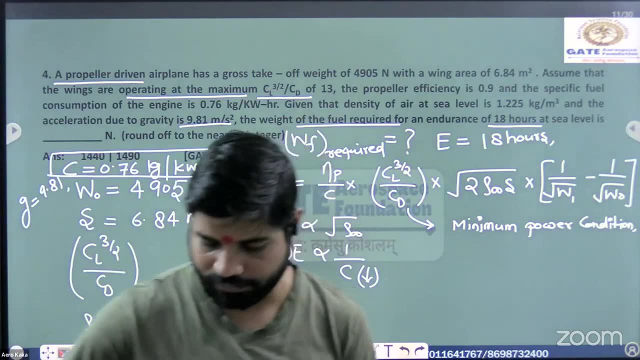 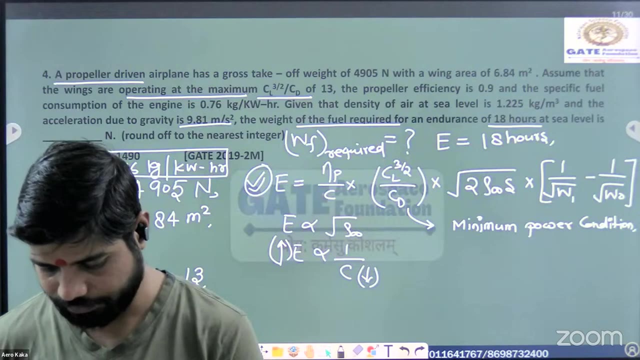 First of all, convert the C value into Newton per watt seconds. Please convert it and let me know how much you are getting. Yes, anyone? Sorry, it is coming 2.071 into 10 to the power minus 6.. How much? Come again 2.. 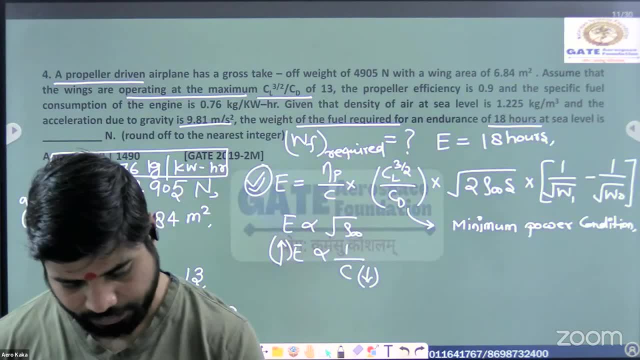 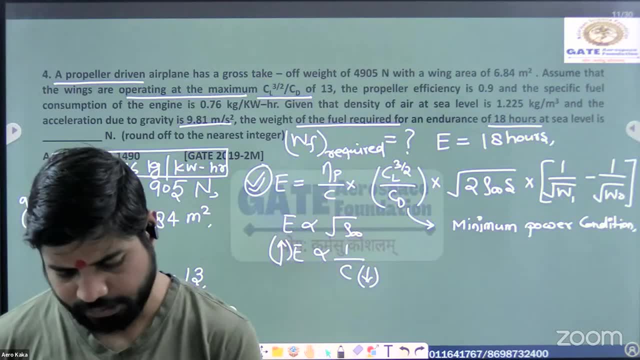 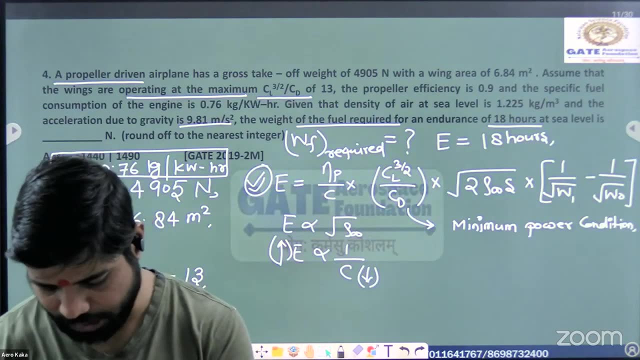 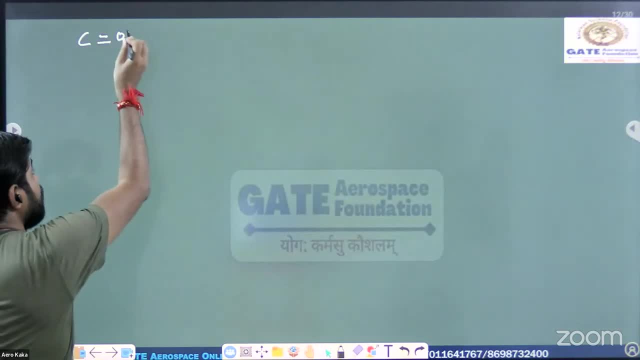 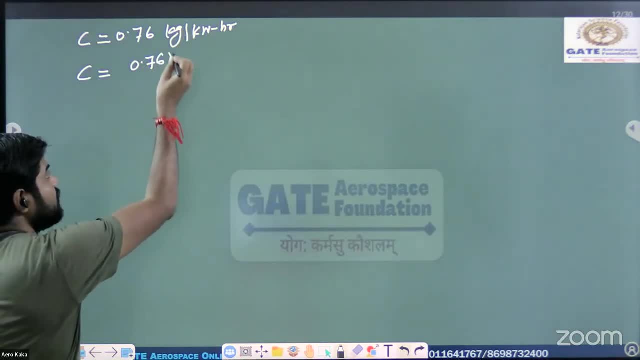 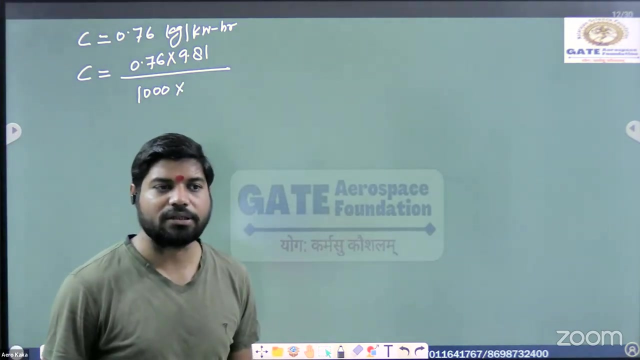 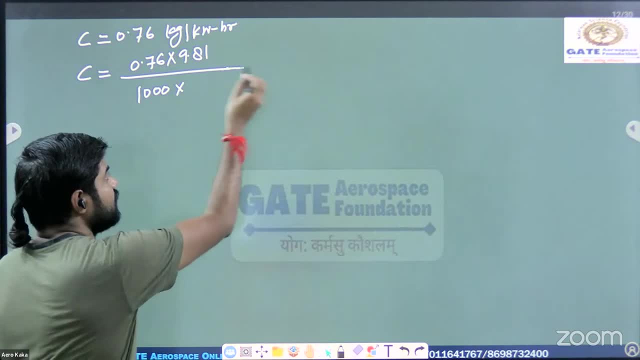 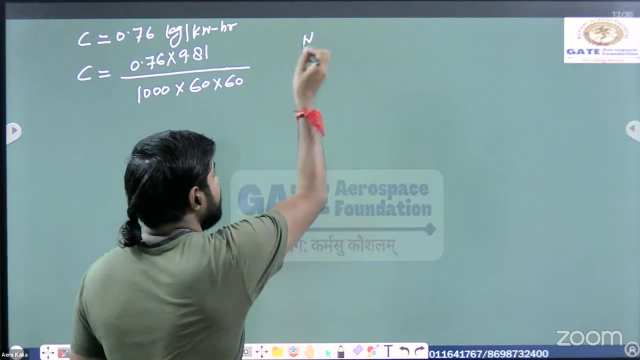 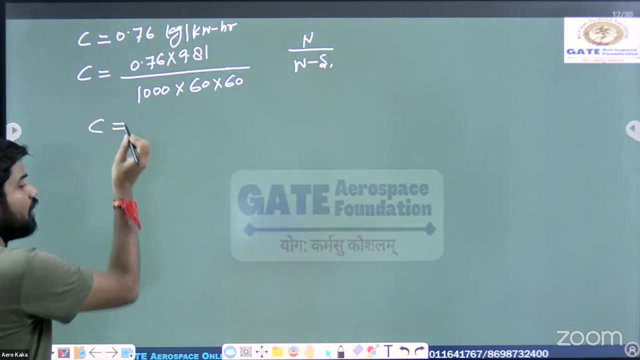 60 seconds, So you can write here: it's a 3600. or simply you can write 60 minutes and then minutes you can convert into seconds, If you simplify it. or let me write here the units Newton divided by how much, One second, That's it. So if you simplify it further, how much? 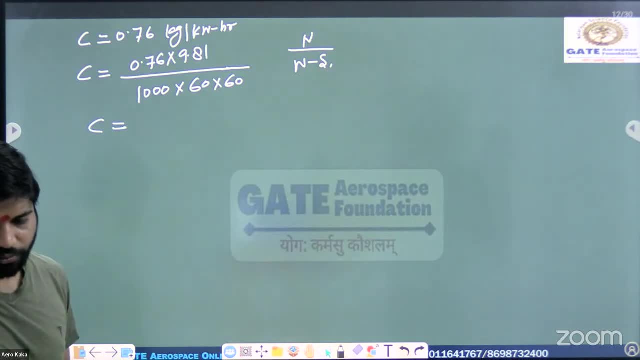 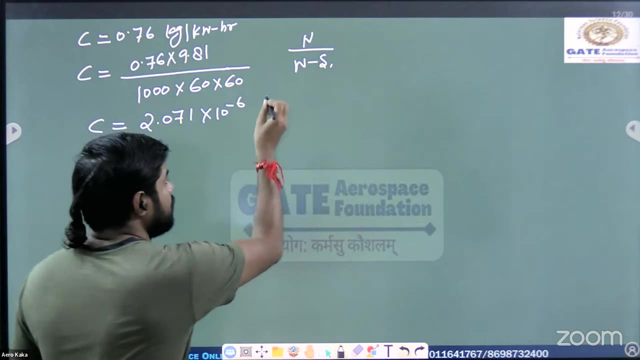 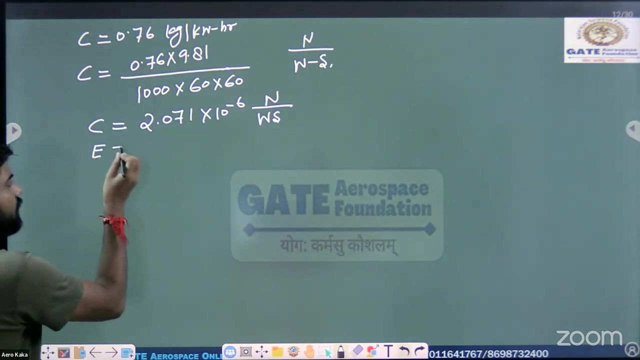 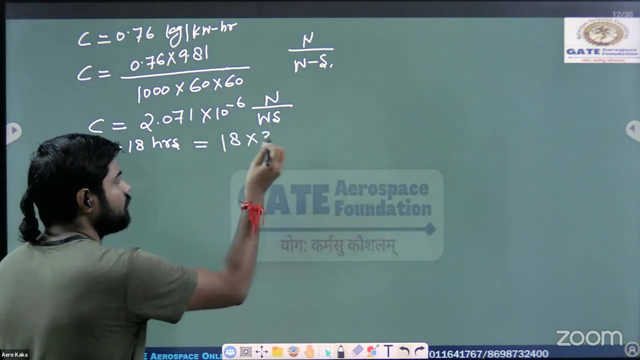 are you getting Zero point 2.071 into 10, to the power minus x Newton per watt second. Okay, Now E here is given how much 18 hours, right, 18 hours. So you can convert into the seconds. You can write it as 18 into 3600.. That's it. Now just apply the formula E, which. 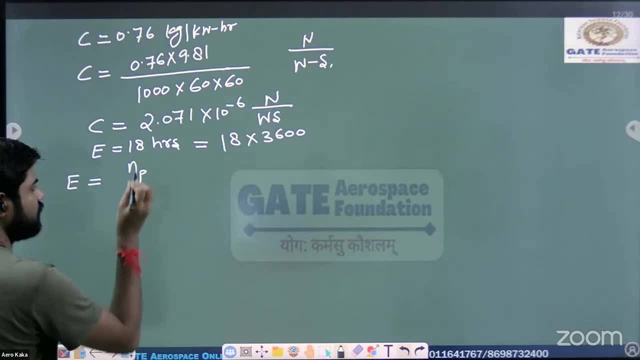 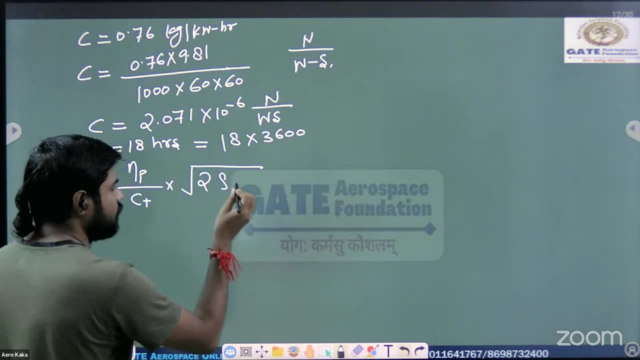 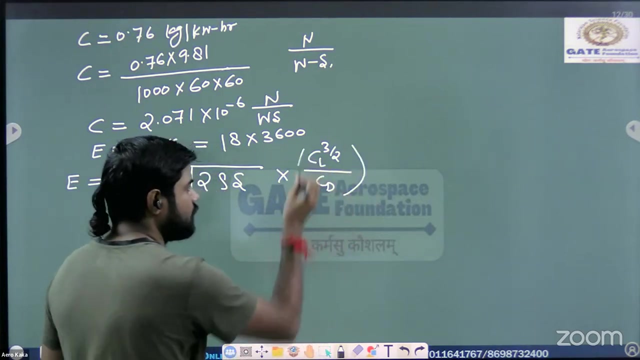 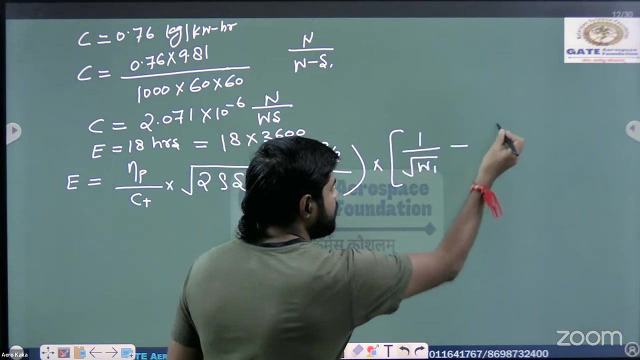 is equal to theta p, That's the propeller efficiency divided by ct into root of twice of rho, into s into cl. raised power 3 by 2 upon ct, into how much 1 upon root of w1 right minus 1 upon root of w0.. Please verify this value. Hello, this last term can you verify? 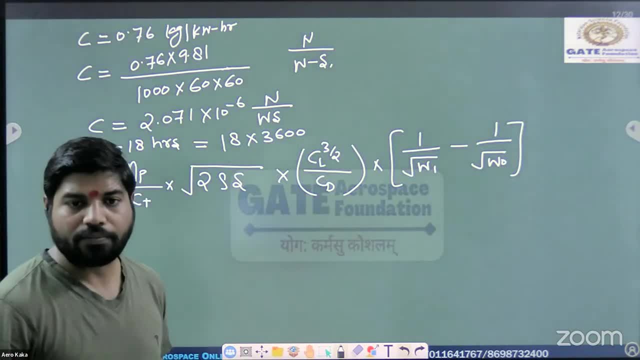 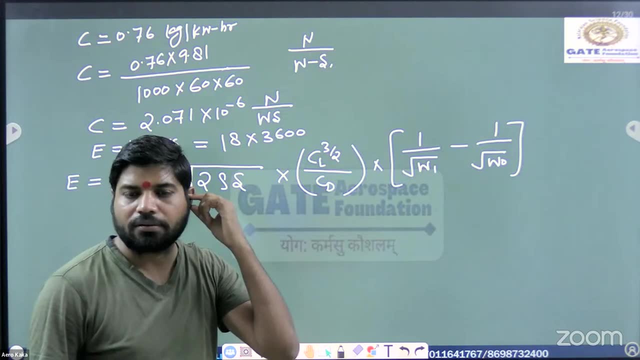 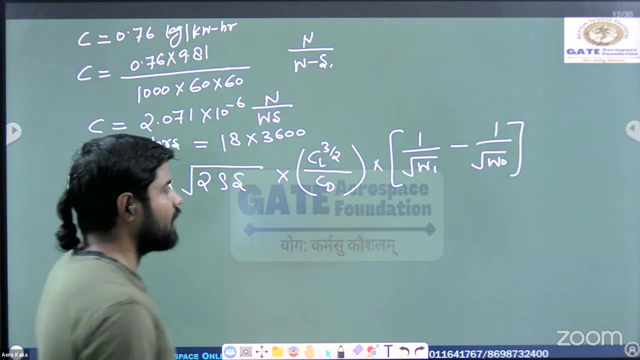 Is it correct or not? Is it correct? Yes, Hello, 1 by root w minus 1 by root w0.. So this is correct, right? That's what I'm asking. Yes, sir. Okay Now what I'm doing here, since. 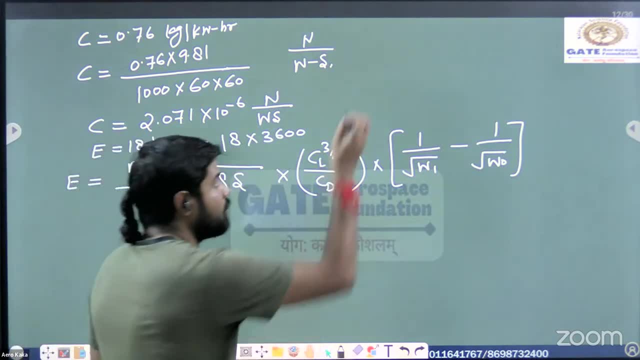 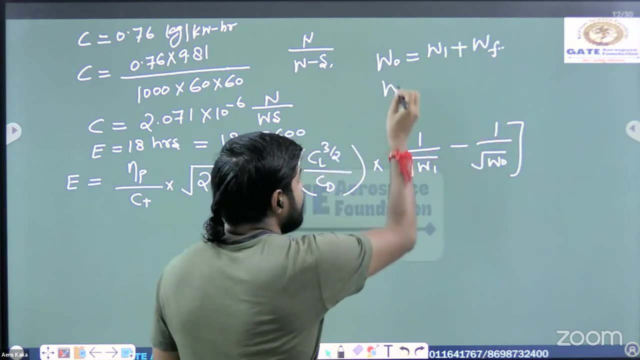 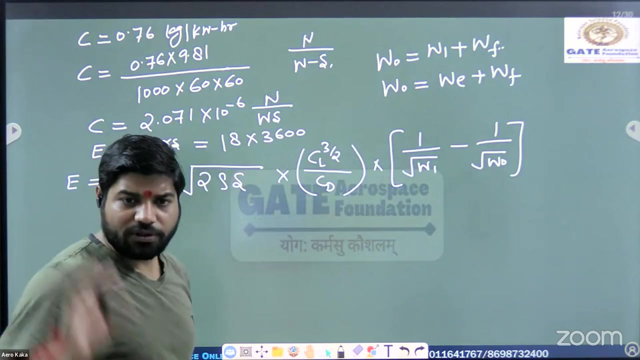 you need what is the weight of the fuel. So please remember this: w0 is nothing, but you can say w1 plus wf. or simply you can write this: w0 is nothing but equal to w1 plus wf and you can say we plus wf. Just go through the derivation part. We are taking this w1. 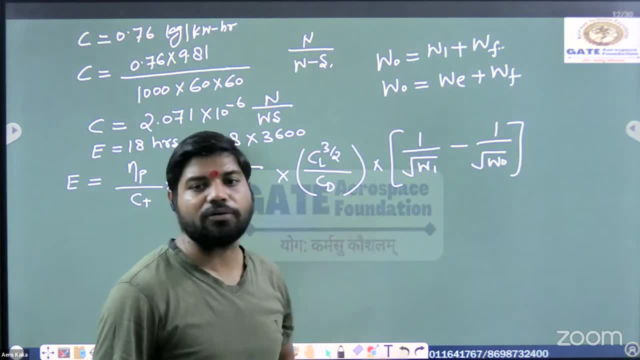 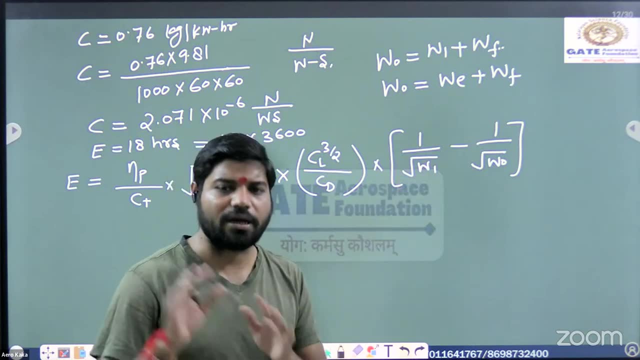 is nothing. but you can say: we right, It's just nothing. but you can say weight of the generally. students get confused at this particular point, Like why you are taking it's an empty weight. Yeah, empty weight is quite different, because your overall weight, this w0, is weight. 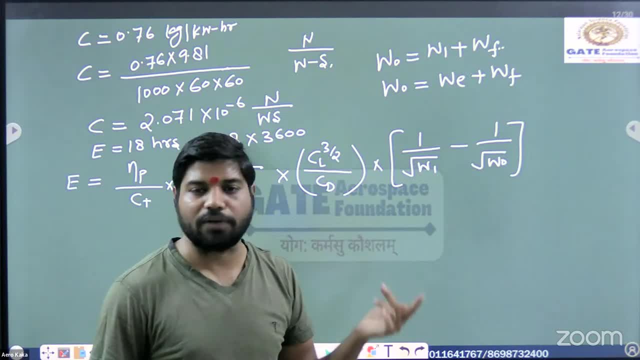 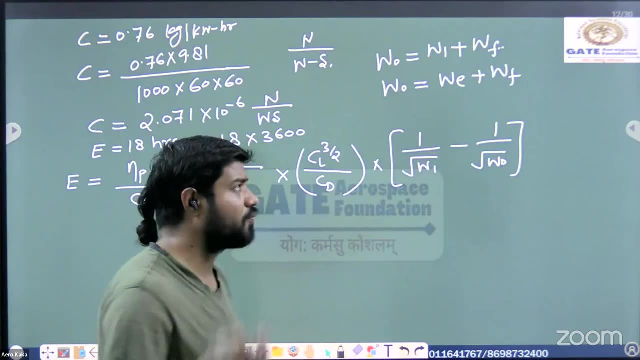 of of. you can say we, then weight of the fuel, then payload weight is also there, then weight of the. you can see So many weights generally we have to consider right. So for simplicity I'm considering this: w1 is nothing but you can say we, no issue at all. Or if you want to keep this, 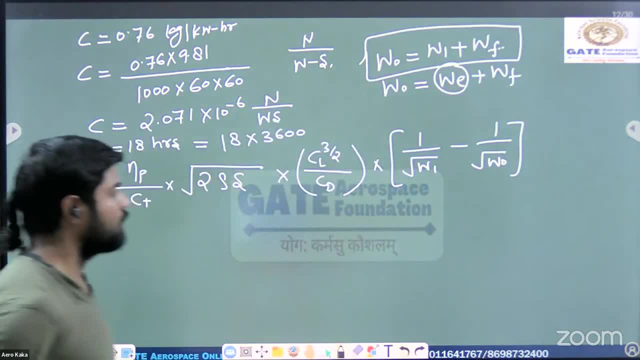 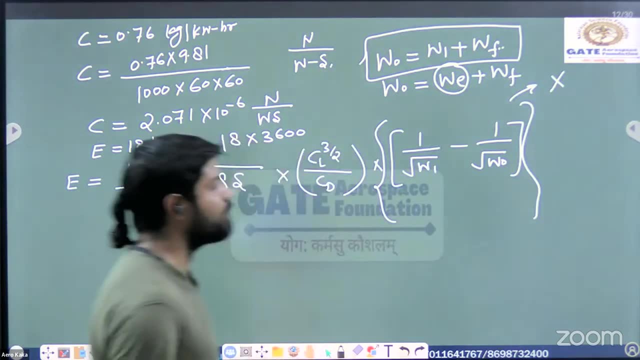 w1, no issue at all. Okay Now. so what I'm considering? I'm considering this bracket as a capital X. Let's consider this is nothing, but you can say capital X, Because if you look at this left hand side and right hand side, right, we have to know like what is. 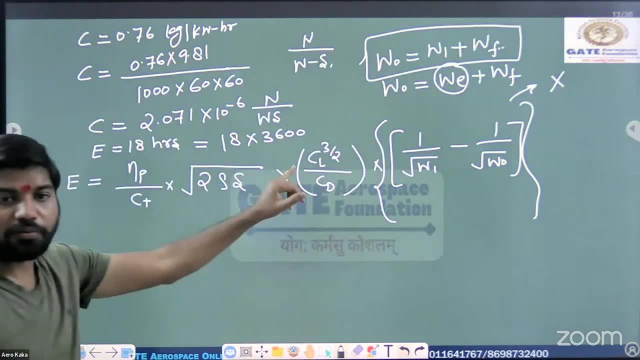 the weight of fuel in this case. So Cl is equal to 3 by 2 plus w1 plus w1 plus w2 plus w2.. So Cl is equal to 3 by 2 upon. Ct is known to us row value as well as capital. S is known. 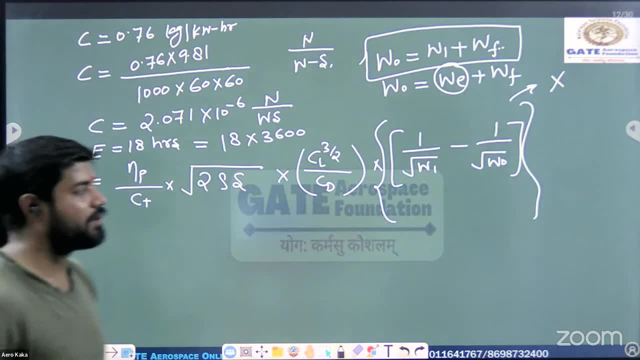 to us propulsive efficiency. Ct as well as E is given right. So if you are going to calculate like, if you are putting all these values here, it's quite difficult. So consider this X and calculate the value of capital. X is nothing, but you can say what is the. 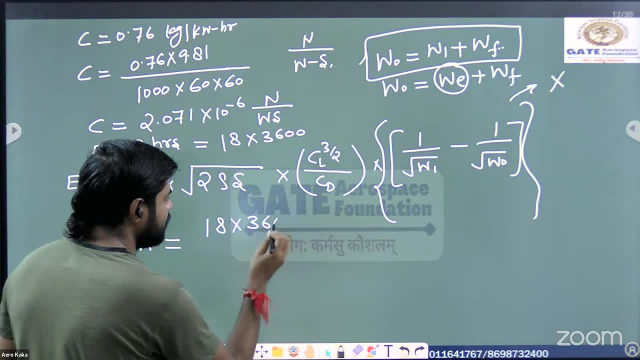 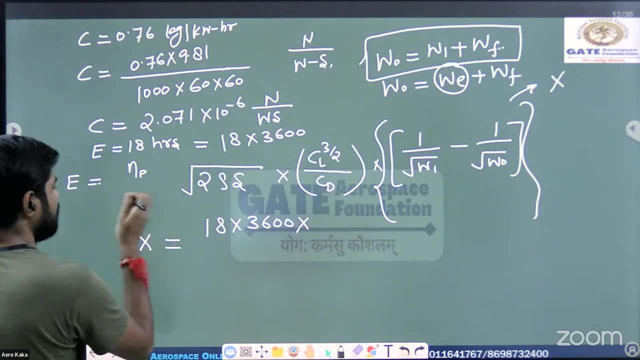 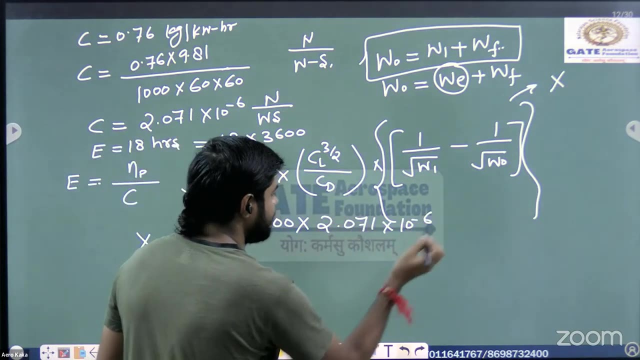 E here You can write it as 18 into 3600.. Now what is the value of C here? This C is nothing, but you can say that's not Ct, It's a C. I'm considering It is 2.071 into 10, raised power minus 6 divided by how much? 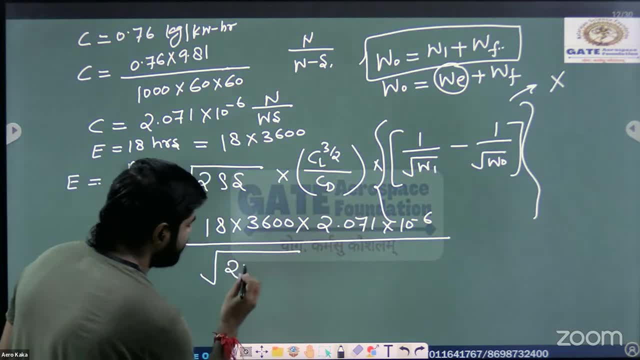 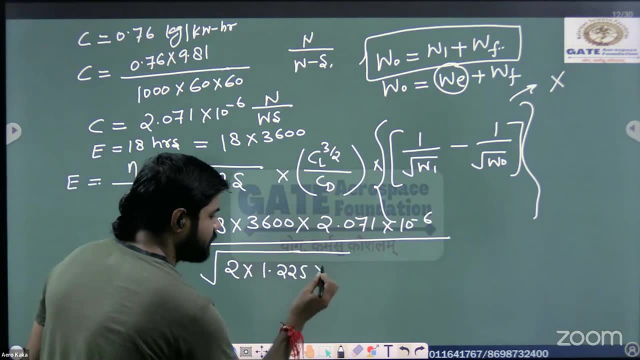 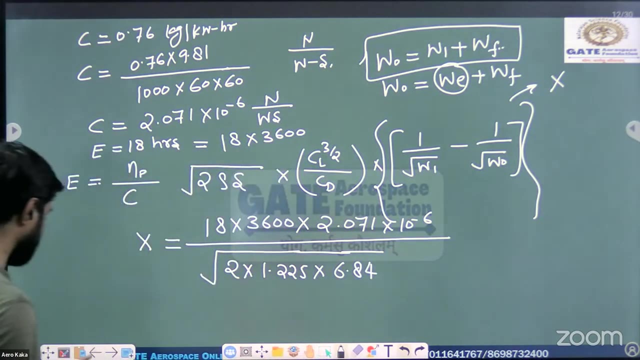 Yes, Root of 2.. Density is how much Can you tell me Density? 1.225.. 1.225.. What is capital S here? 6.84.. Are you sure 6.84?? Yeah, 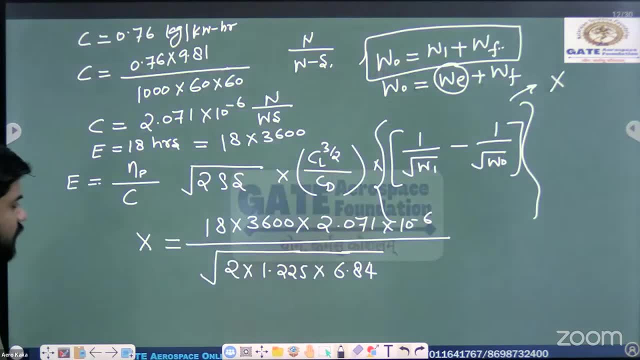 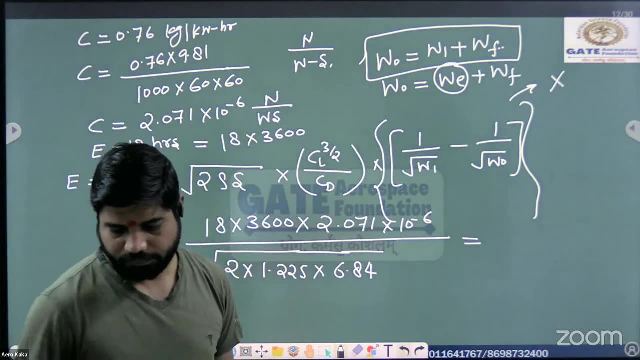 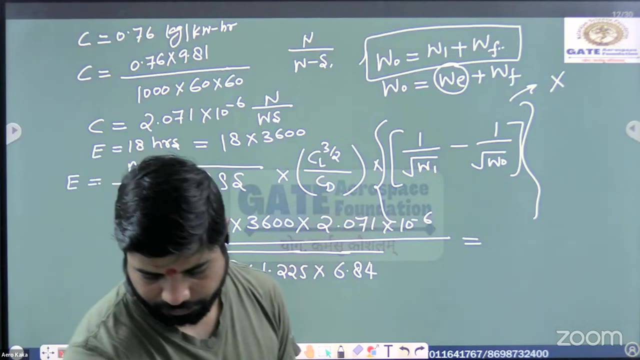 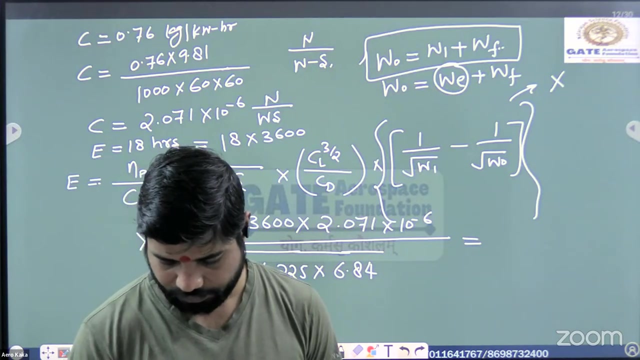 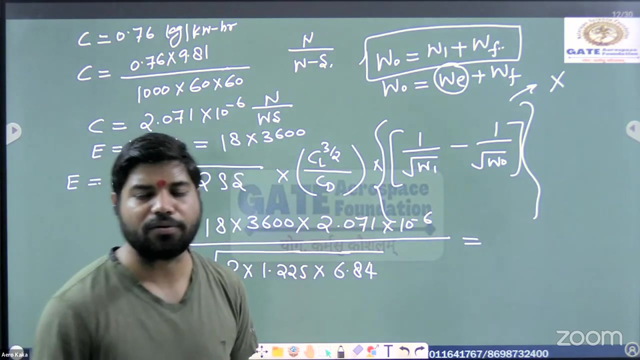 6.84. it is given. Now, just simplify it and let me know how much you're getting. Yes, How much we are getting Anyone? Yes, How much you're getting Sivarana? are you there, Hushi? 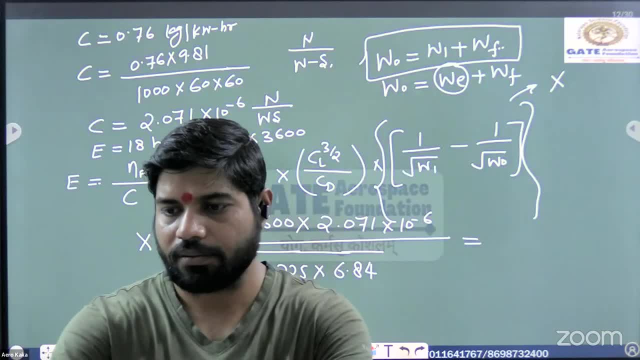 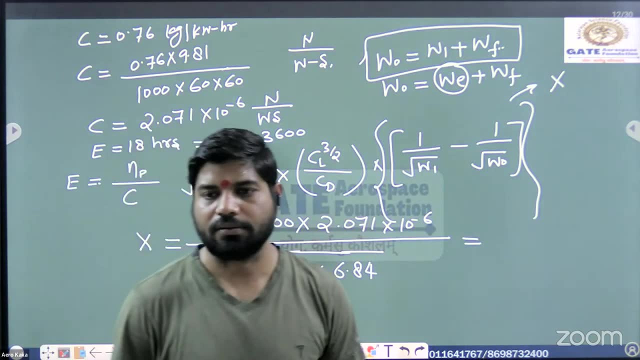 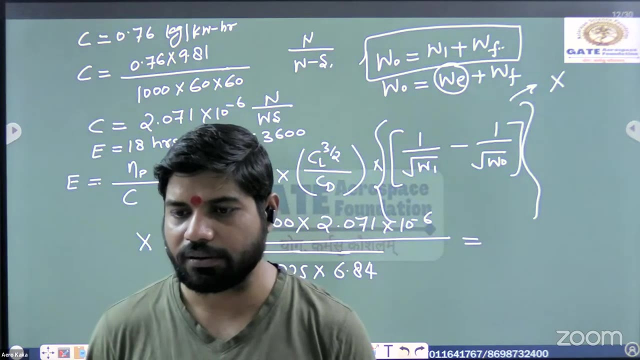 Mitali. Sir, it is coming 0.032784.. Wrong, Yes, Narishma Nandini, Mitali Hushi, Manavav, Ishika Zanvi, How much you're getting? 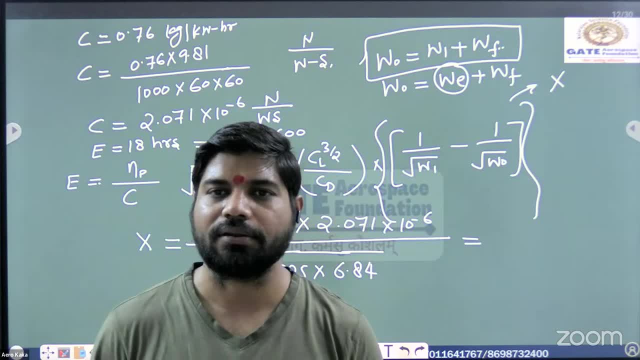 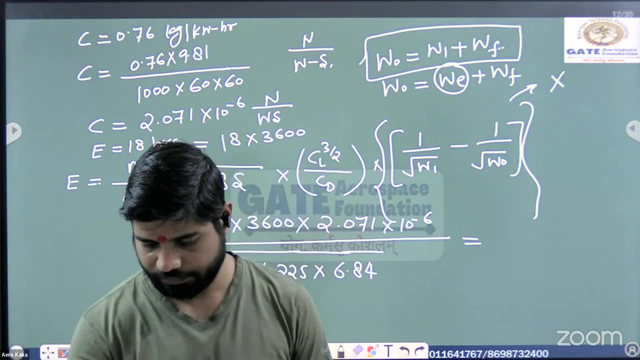 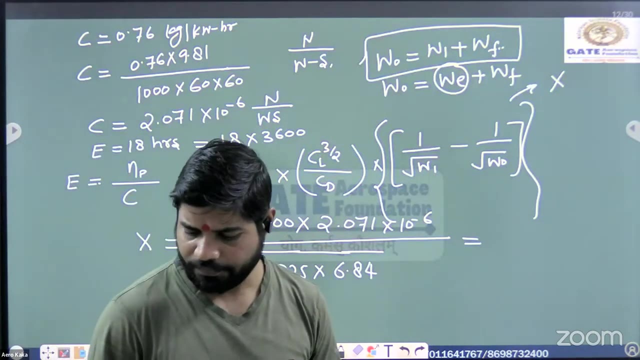 Riya. Yes, How much you're getting. Yes, How much you're getting? Two.527.. 2.527 into 10, raise to minus 3.. Two point 5272 into 10, raise to minus 3.. 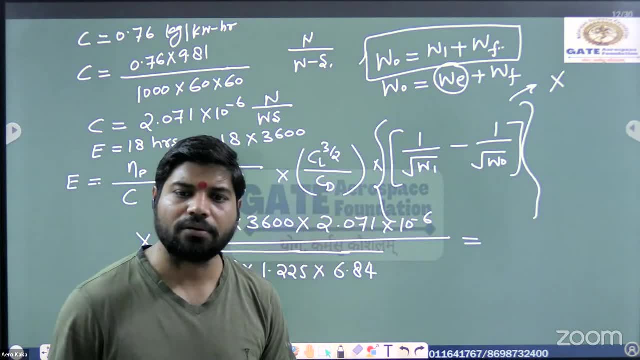 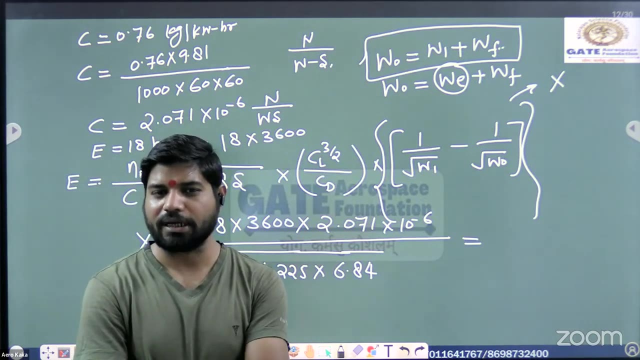 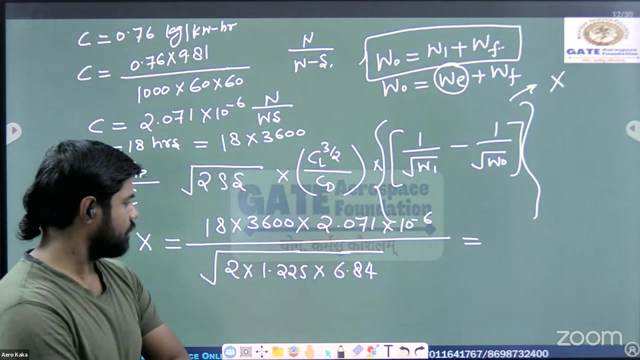 Okay, Any other person? Sir 0.03276.. 0 point 0.03276.. yes, we are having exam in next week, right, and still you are. you are doing this calculation mistake. very good, keep it up. yes, sir. 0.0327826. 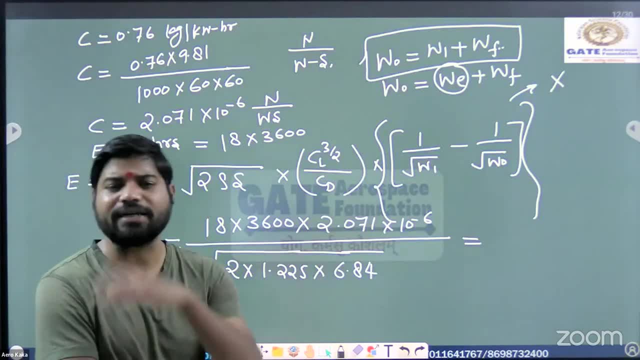 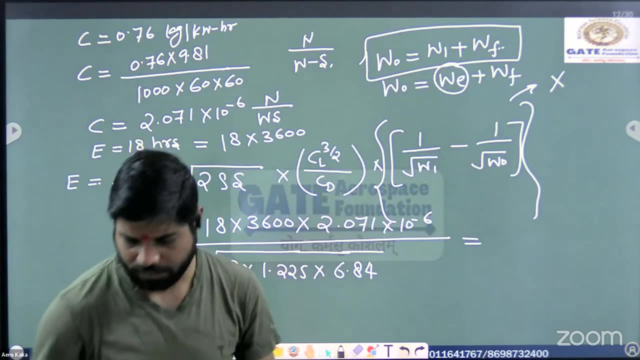 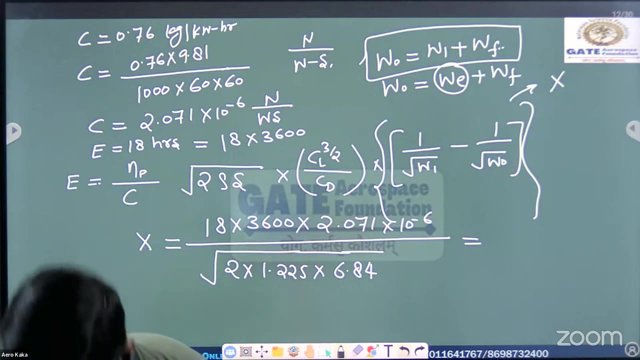 how much 0 point in 10 to the power minus 3 or 10 to the power minus 5, whatever, ok, let me check my calculator, Simran, how much you are getting calculator calculator sir, who the n? p value? yeah, eta p value is also there, right? 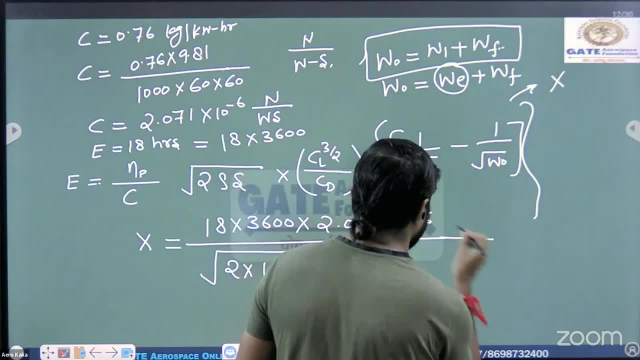 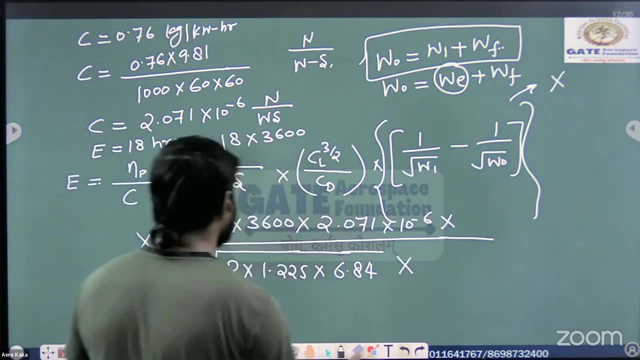 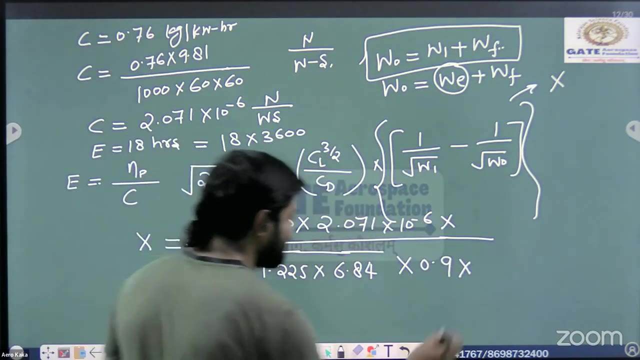 c l 3 power 2 upon c d value. yes, you are right. so generally we have to take this eta p also right. so what is this eta p? it is given 90 percent right and c l raise power 3. y 2 upon c d is also given how much. 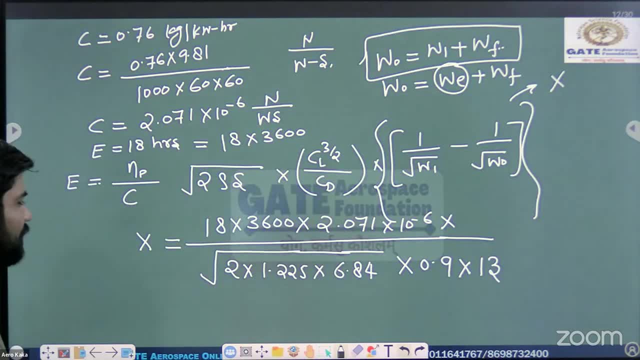 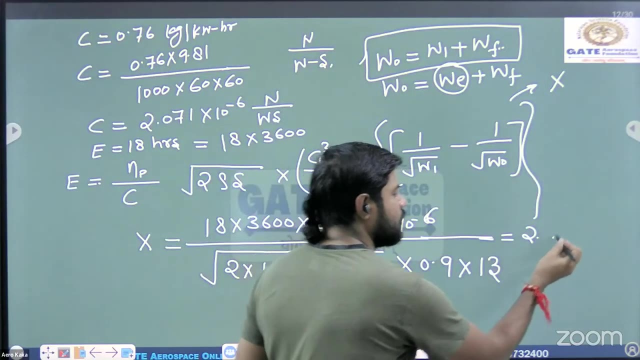 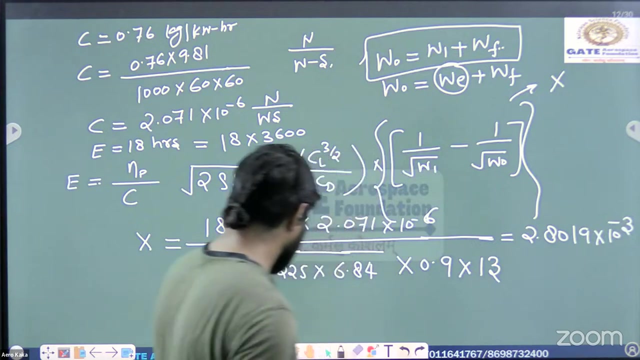 30. yeah, now we will get the correct one. yes, how much you are getting? 2.80 into 10 to the power minus 3, 2 point 8019, 8019 into 10 to the power minus 3. yes, sir, ok now. 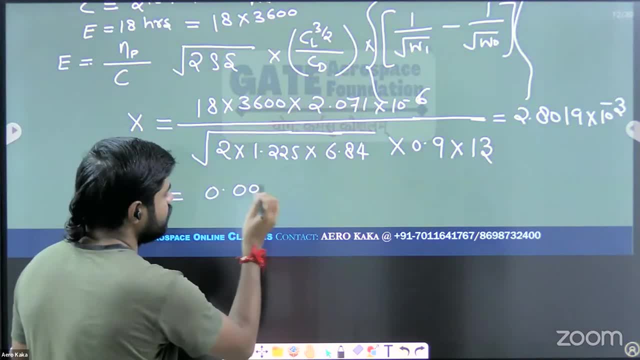 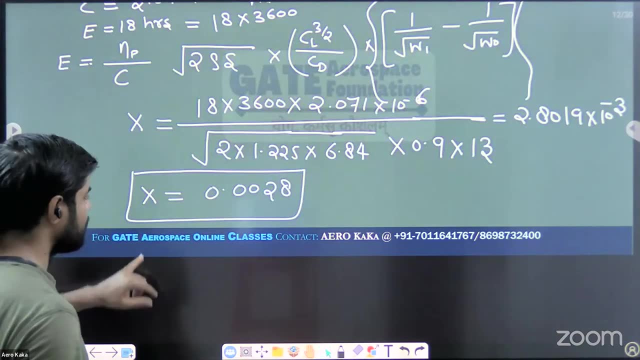 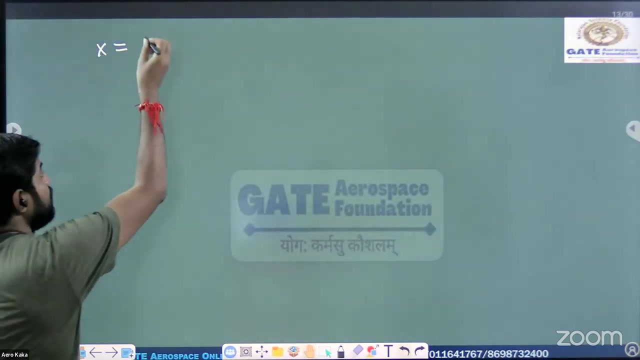 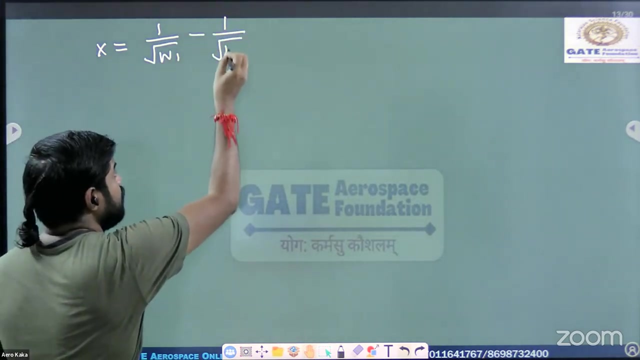 so let me write here you can write: it's a 0.0028. shall we write: that's the value of x? now, what is capital x? what you have taken? this capital x is condition x is nothing. but we have taken 1 upon root of w, 1 right check minus 1 upon. 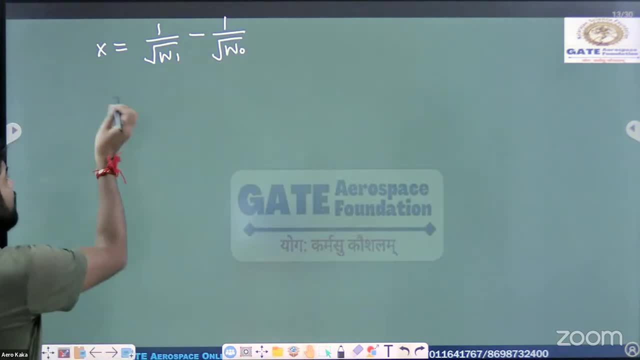 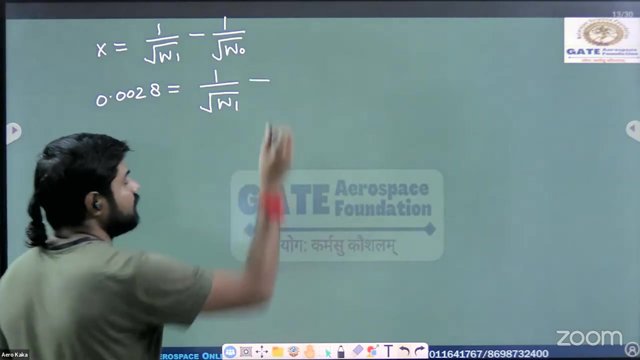 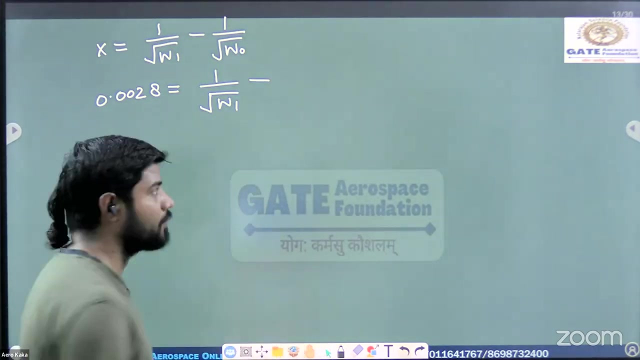 root of w naught say yes or no. so this x values how much- 0.0028 now- the overall weight of this aircraft is given or not? yeah, given or not, I think it's given How much it is. It's a 4905.. You can write: it's a one. 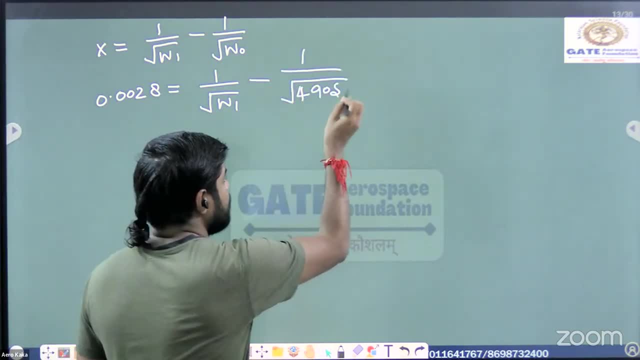 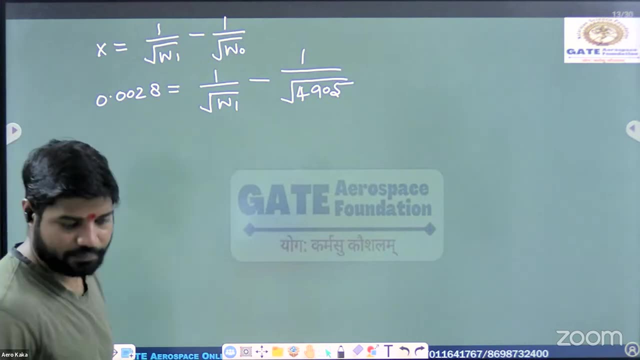 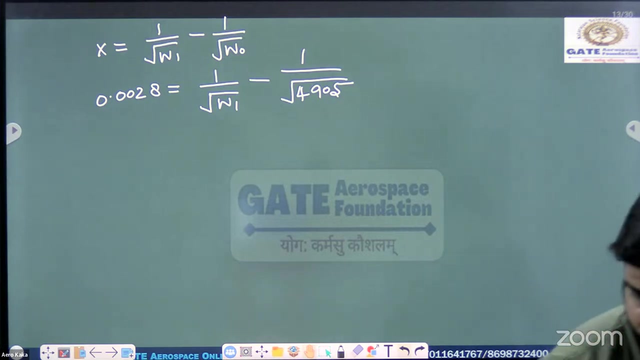 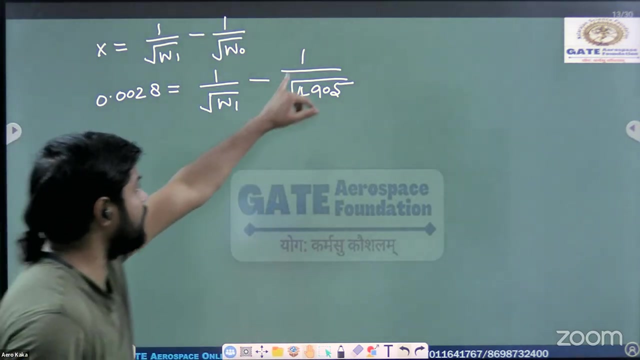 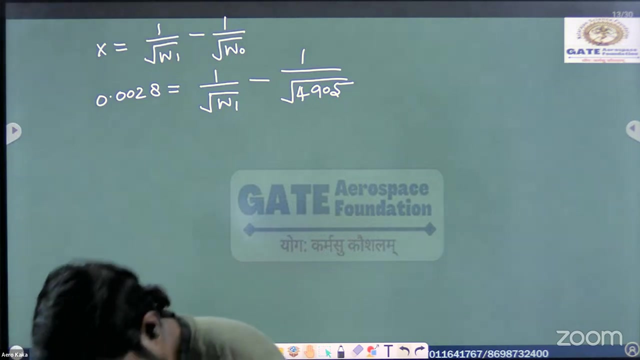 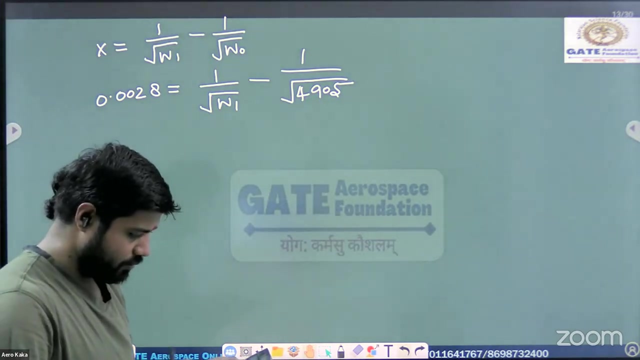 upon root of 4905.. Now just simplify and let me know how much you're getting. Yes, what is this value? Can you tell me how much you're getting this one? Yes, anyone, Sir? W13460.20.. 4905. root of this value. How much, How much? 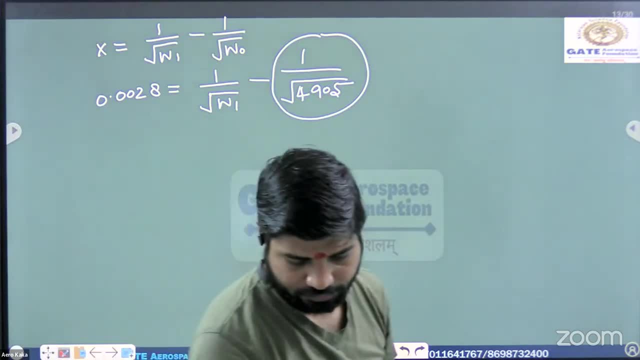 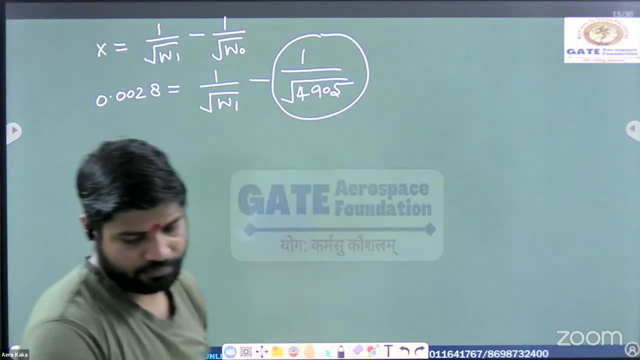 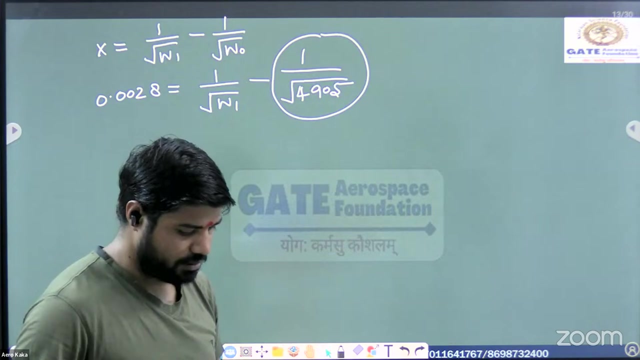 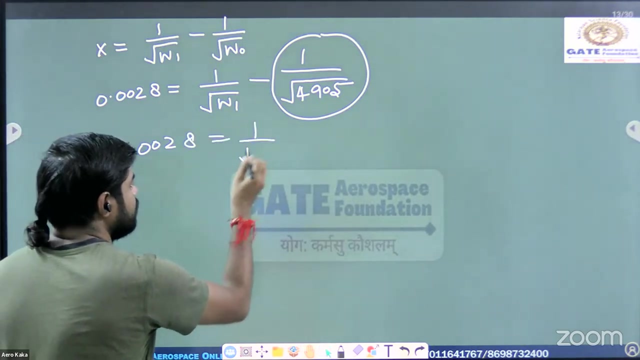 This value How much you're getting. How much you're getting 0.0142.. 0.0142.. So you can write it's a 0.0028.. You just have to do one upon root of W1 minus 0, point How much. 0. 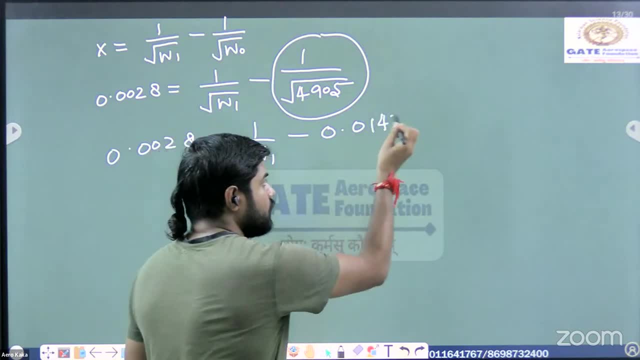 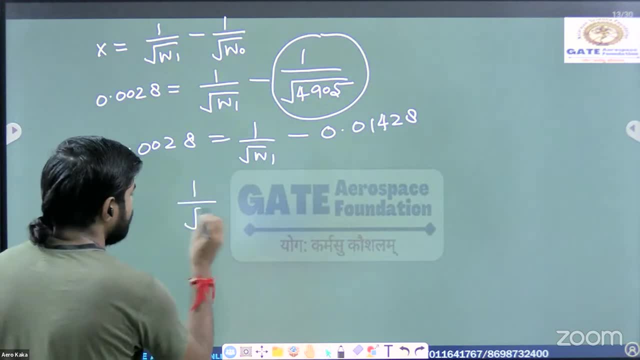 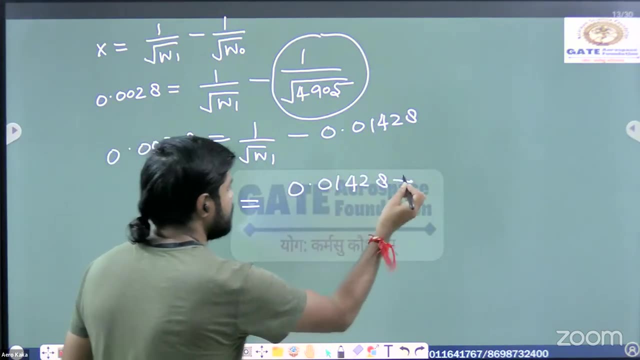 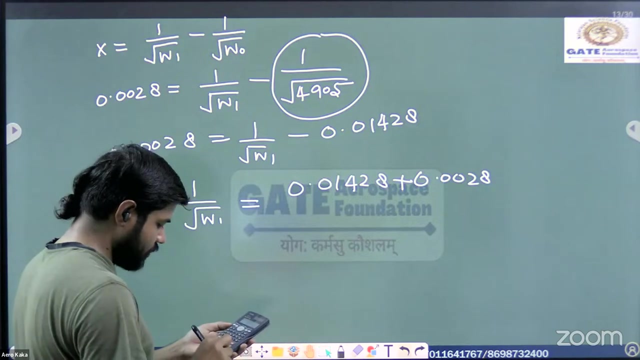 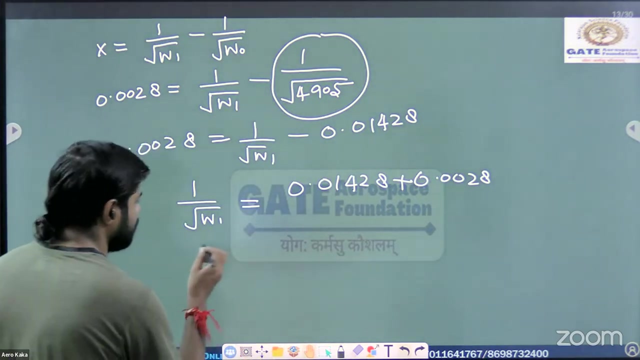 Now from here what you can write: the one upon root W1. which equal to how much? Tell me 0.01428 plus 0.0028.. So 0.0028 plus 0.01428 is how much, 0.01428 plus 0.01428.. 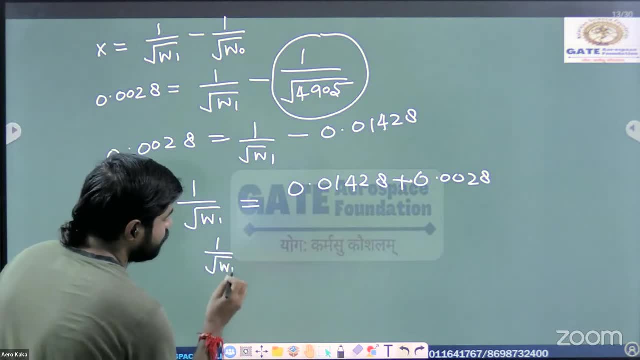 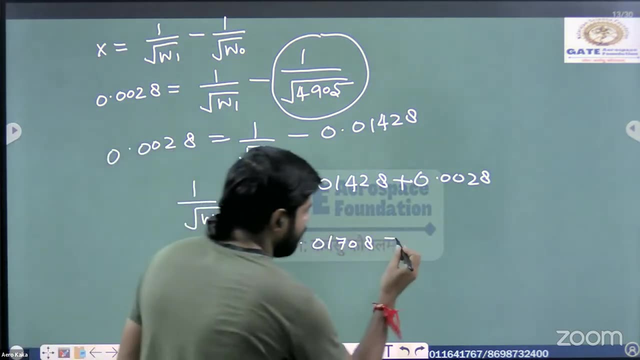 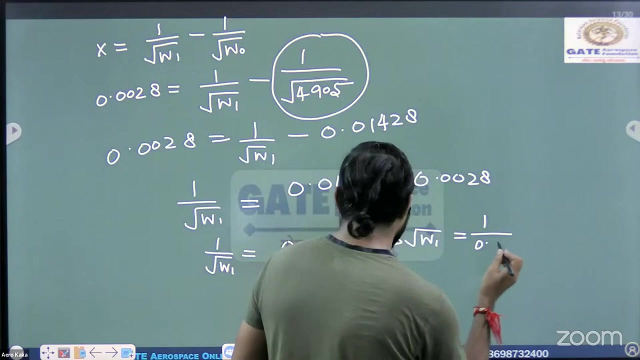 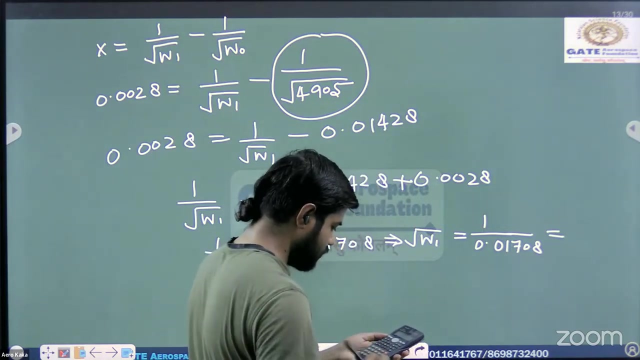 we are getting 1 upon root w1, which is equal to 0.01708.. Are you getting this value? Check, please. Yes, sir, Now from here what I can write. I can write root w1, which is equal to how much? 1 upon 0.01708.. So, 1 upon answer, Are you getting? it is a 58 point something. 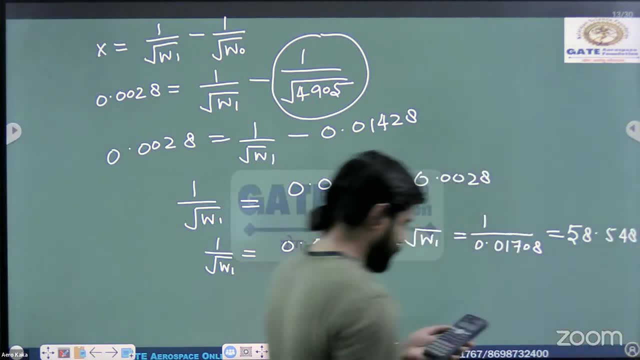 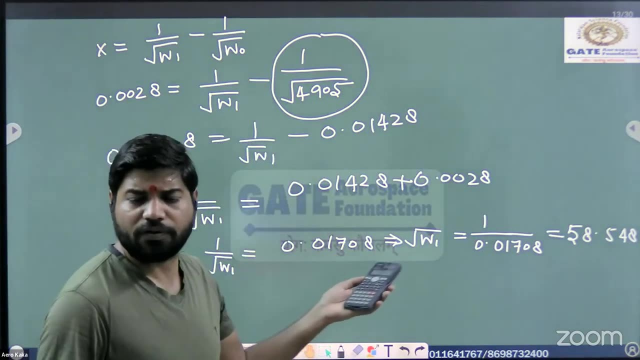 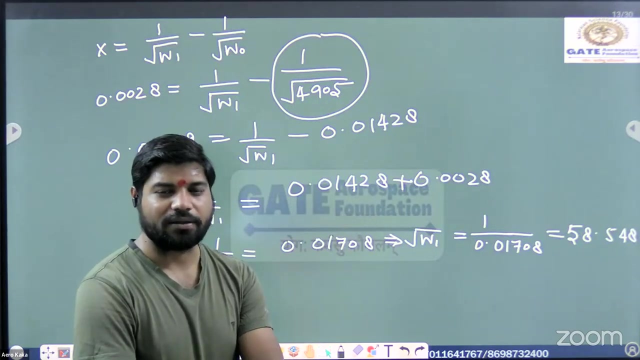 58.5.. Yes, sir, 58.553.. Right, So that's the value of root of w1.. Right, So what you can, if you want to calculate the value of w1, what you have to do: Squaring, Squaring, sir. Yeah, So I have given this problem as a homework, I think last semester. 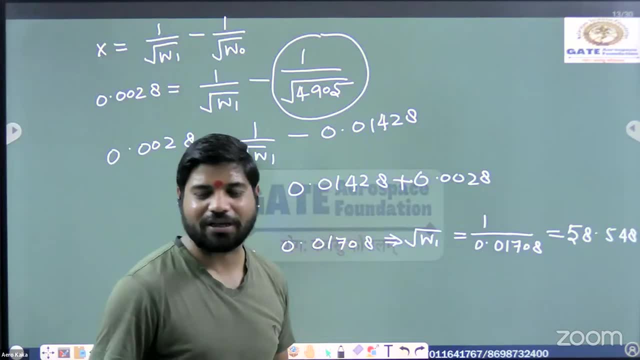 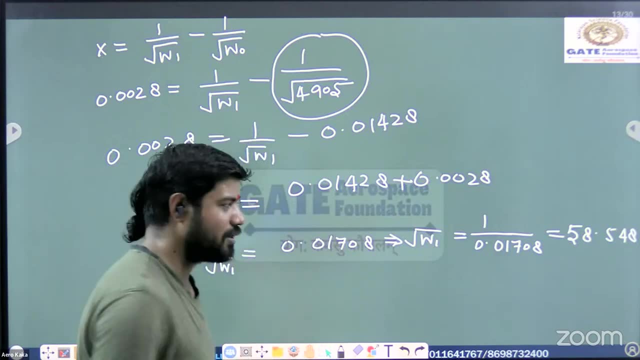 and some of the students. you know what they did. They have taken the square root of this particular value again to calculate the value of w1. So what you have to do is you have to calculate the value of w1. So please don't do that. So just square on both the side. 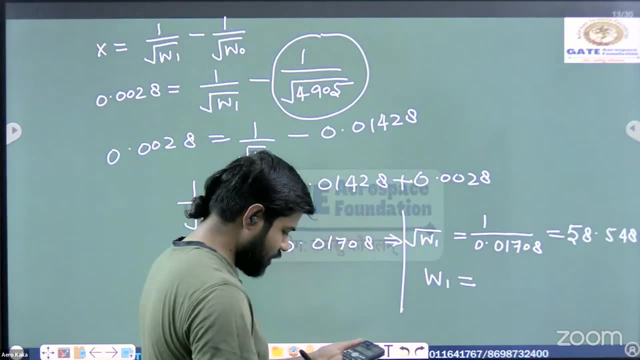 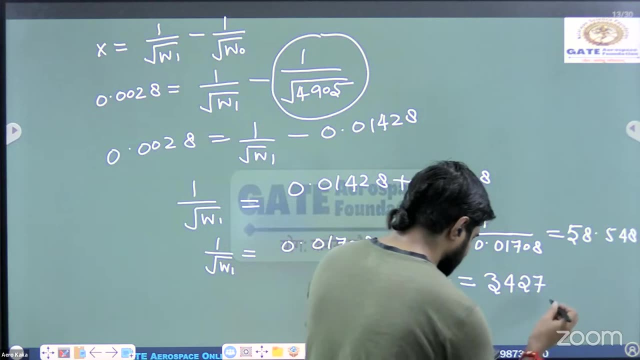 What do you get? w1 is equal to this square of this. one is how much? 3427.. Are you getting? Yes, sir, 3427.86940.. Right, So that's the value of w1.. Now, what is the w0?? This w0 is: 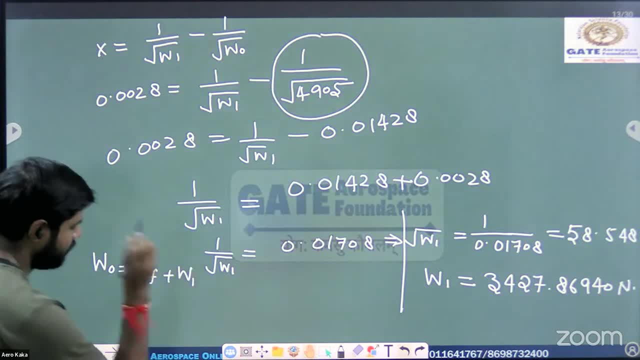 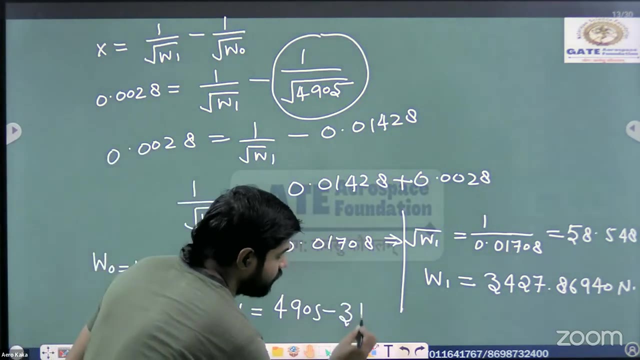 nothing, but you can see weight of the fuel: W0 plus this w1. here Now wf is nothing, but you can see w0 minus w1.. So w1 is given here 4905.. 4905 minus What is the value of w1? It's a 3427.8694. 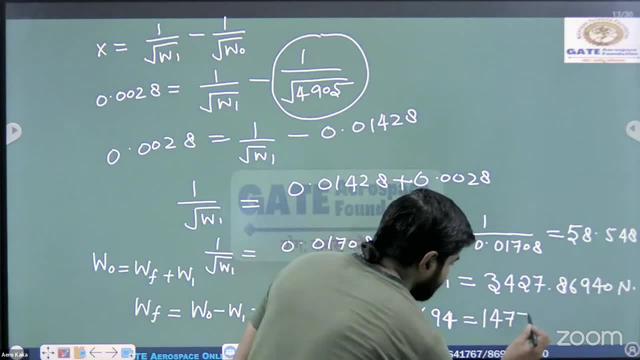 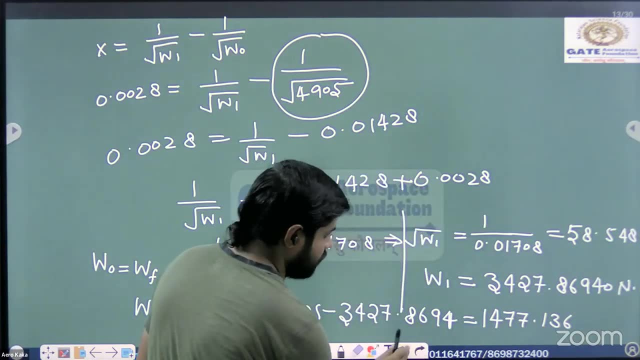 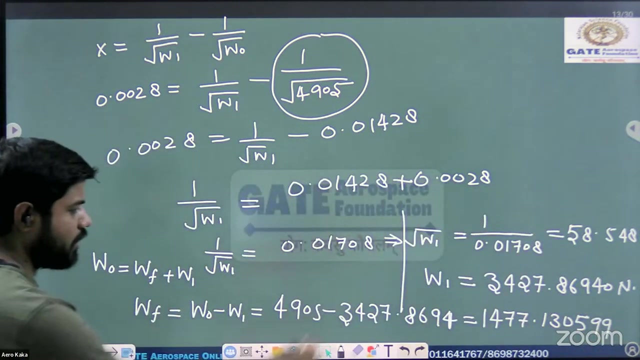 1477.1306.. 1477. Right, 1477.136, something up to three decimal point, Otherwise 130599 you are getting right, if I'm not wrong. Yes, sir, Right up to the three decimal points, or yeah, up to three decimal. 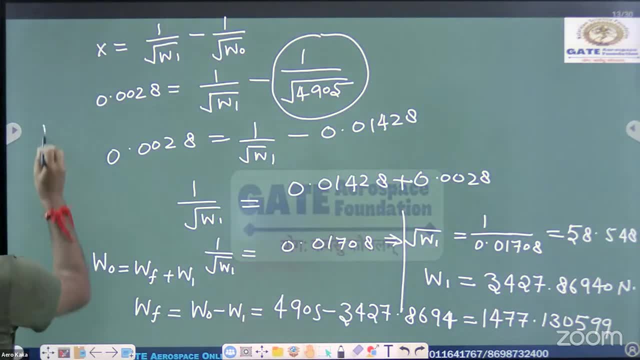 point we can write Wf which could do how much 1306 Newton up to quarter. So this is not decimal point Up to three decimal point, Wf to 1.. So I said only because some case in less than 10, 11, bless my pencil. 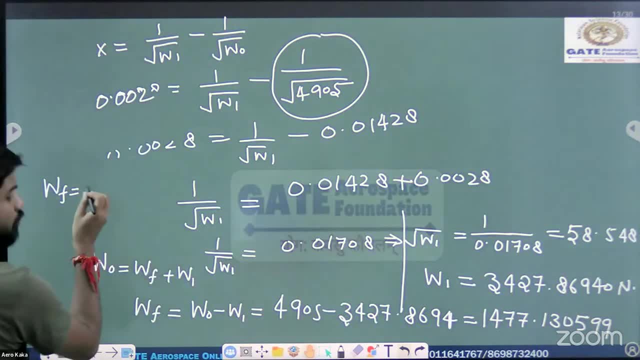 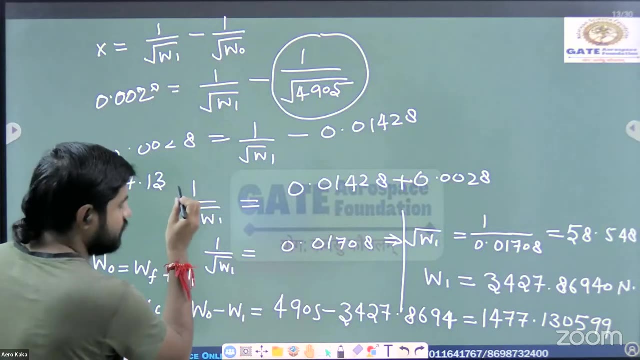 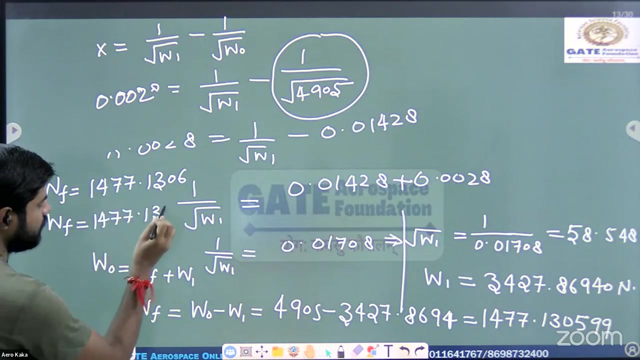 1477point Sea Wf. is 1477 actually from? reflection is coming from there. to look at this corner. 1477point I should use except up to four decimal points, three decibels coming from can write: it's a 1477.131 right check So what they are asking: nearest integer or up. 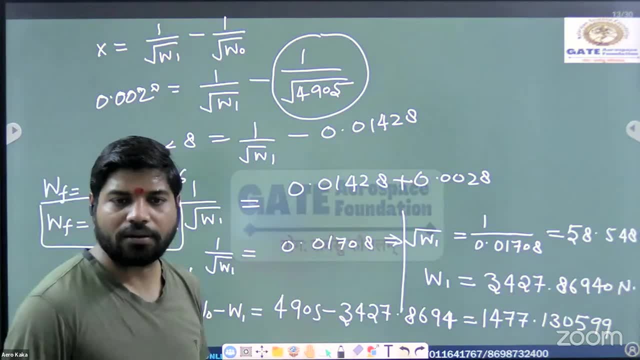 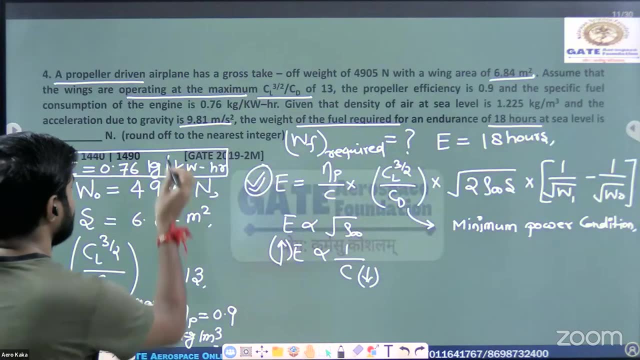 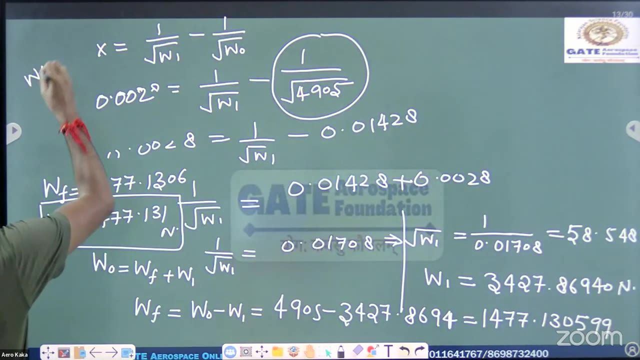 to 2 decimal point or 3 decimal point. what they are asking, Sir, nearest integer. Are you sure that's right? yeah, they are saying round off to the nearest integer. So what is the nearest integer? here you can write the nearest integer WF is nothing, but you can say 1477, Newton. that's your final answer. 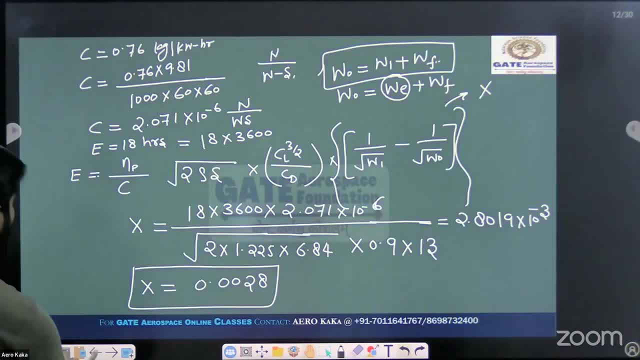 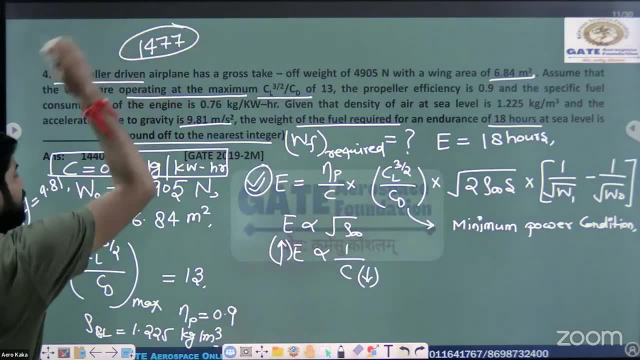 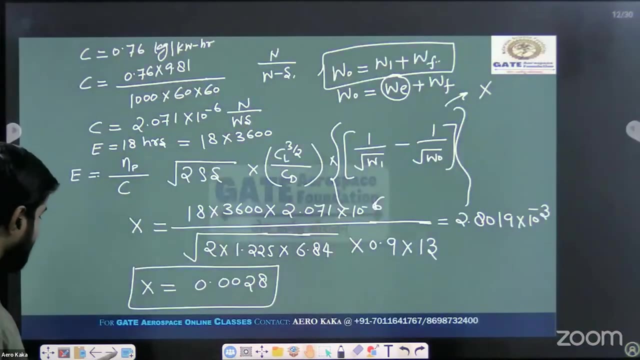 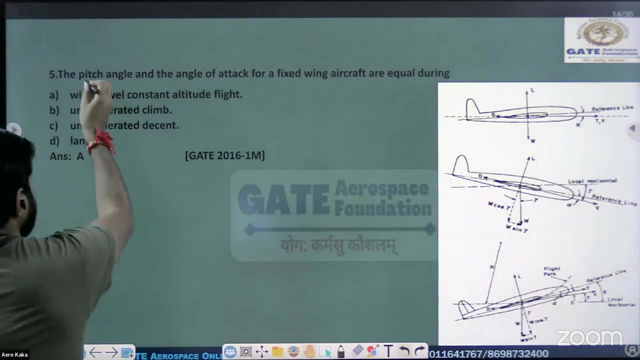 Let's check whether this is within the range or not. We are getting 1477 right. 1477 check here. range is given. 1440 to 1490. right means our calculation is correct. Now again, let's look at This particular problem once again: the pitch angle and angle of attack for a fixed wing. 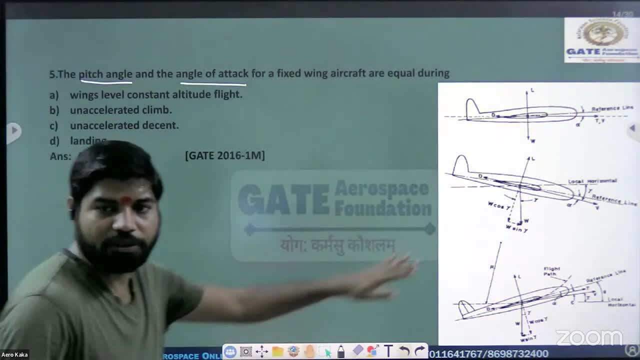 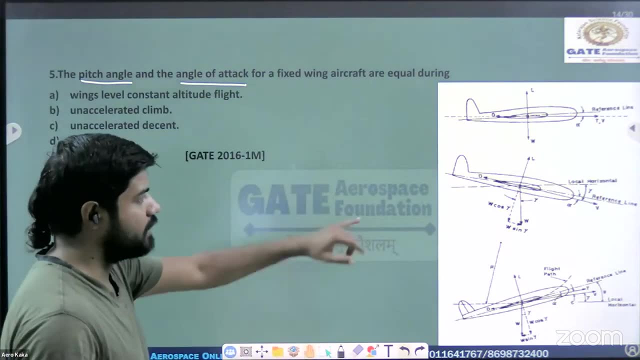 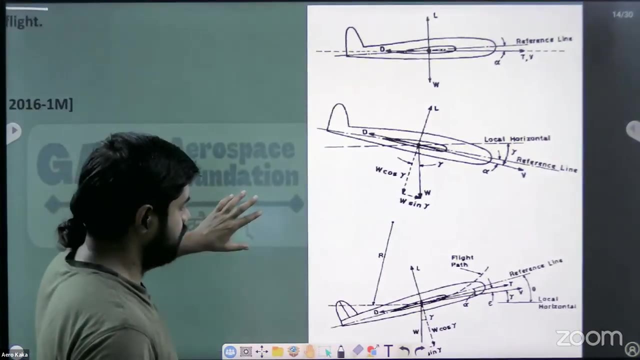 aircraft are equal during. is it visible to you, this particular diagram? is it visible to you, please let me know first. Yes, sir, If not, let me zoom it Now. visible If you look here. Yes, sir, During the cruise flight, or it is a steady state in level 5.. 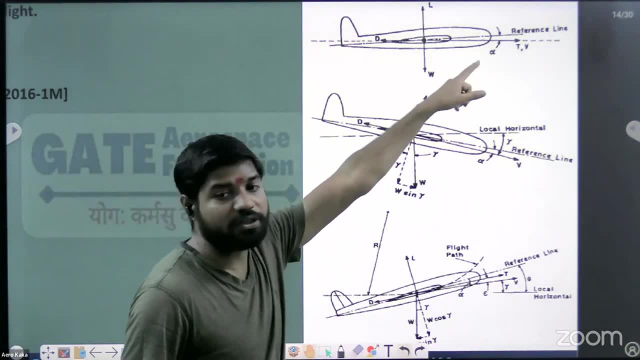 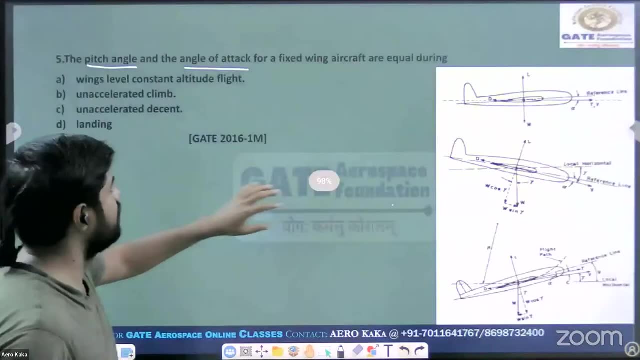 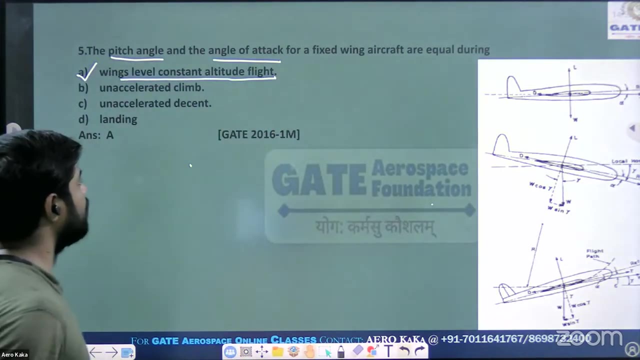 Yes, sir, You can see that only your pitch angle is exactly equal to you can see the angle of attack. Okay, So the correct option here is what, out of the given options, Option A Gains level: constant altitude flight, unaccelerated flight, climb. 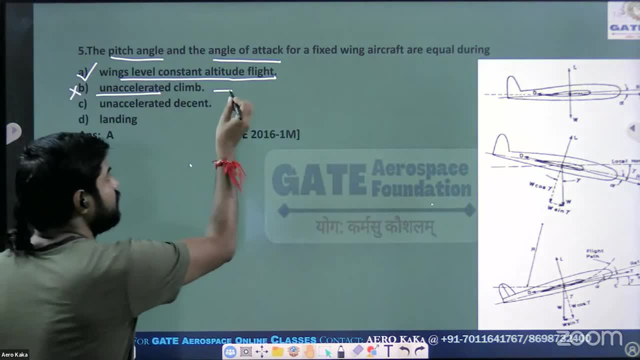 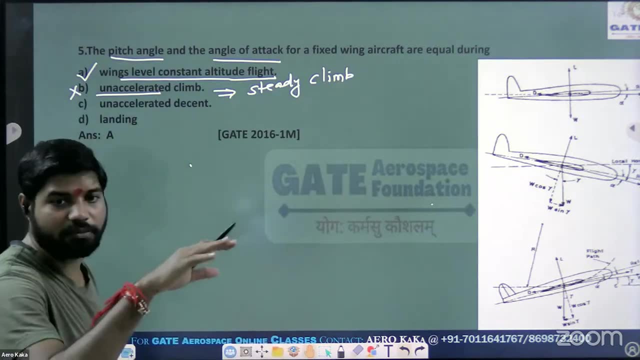 No, What it means to be unaccelerated means that's nothing, but you can say it's a steady climb. right, Please take care. What we call it's a steady climb Means The forward speed is remains constant. or you can say acceleration is equal to zero. 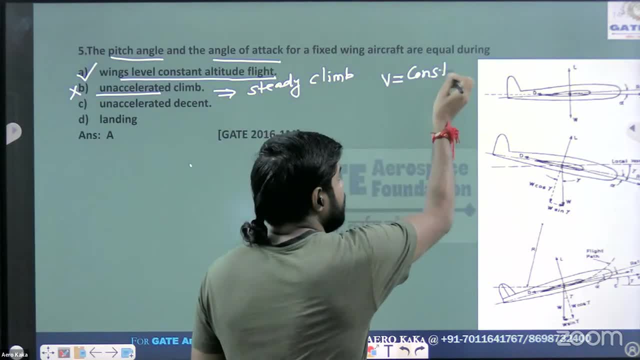 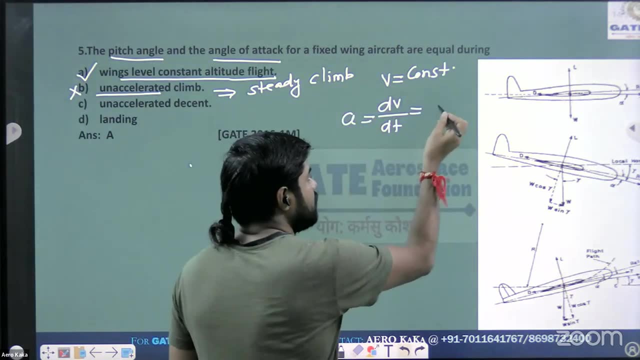 It's very simple: If B is equal to constant, right, Then what is the value of dv upon dt? and this dv upon dt is nothing, but you can say acceleration, So this value is zero. Why? Because if you are differentiating any constant, let's say this is C, So what is the differentiation? 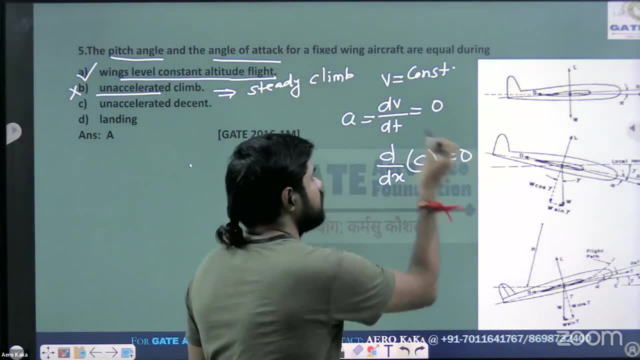 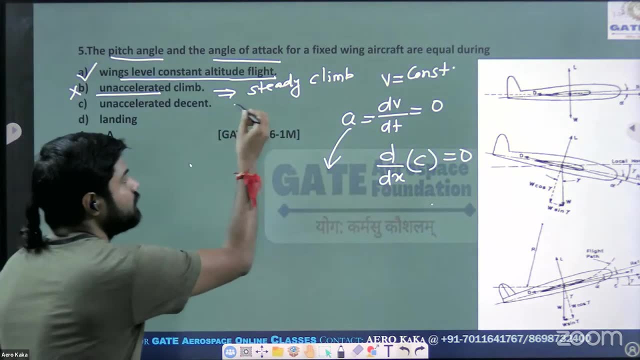 of any constant. It's a zero, only right. So A is equal to zero. It means that it's a unaccelerated flight. or you can say unaccelerated flight, Or you can say unaccelerated climb is nothing, but you can say steady climb. 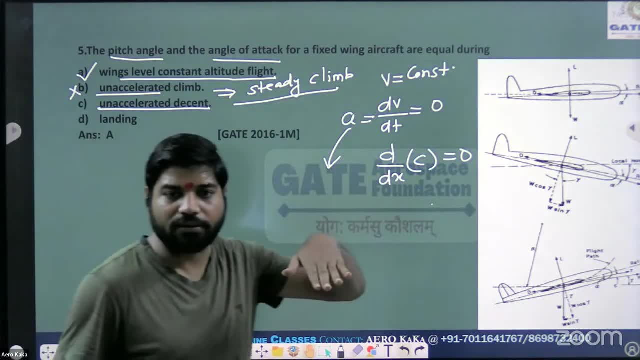 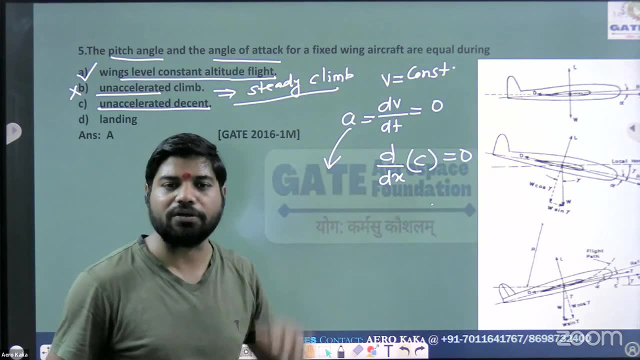 Again, it's an unaccelerated descent. What it means to be descent? You can say it's a gliding right Check. So here what happens? Here? rate of climb becomes negative, only right ROC. or you can say the vertical speed becomes negative. 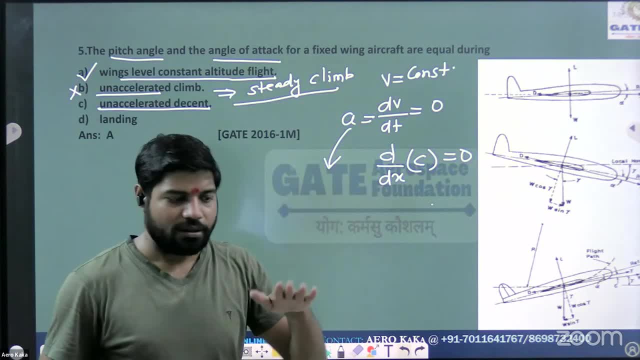 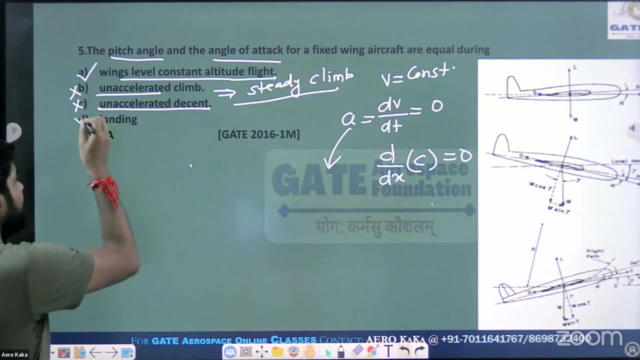 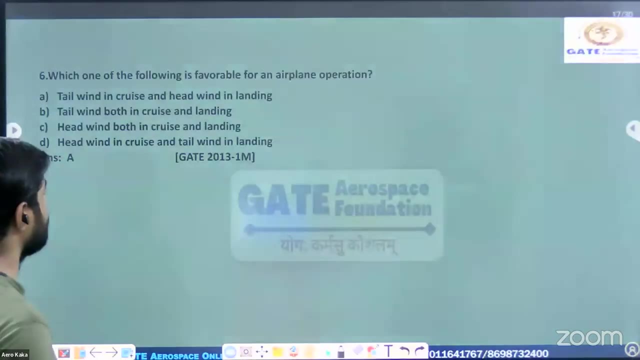 And during the climbing, what happens? Your vertical speed is positive. That's the only difference. So this is also wrong. and obviously during the landing. So the option A is correct. Now again, they have asked the same question they have asked in GATE 2030.. 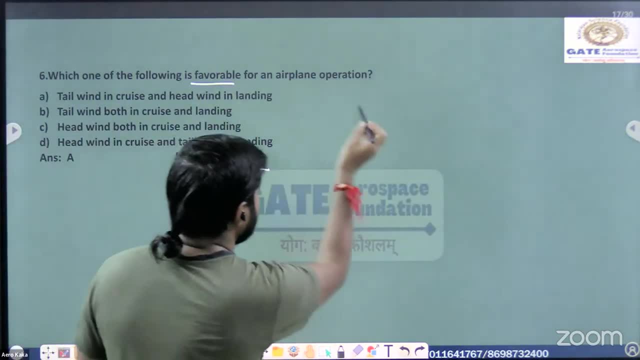 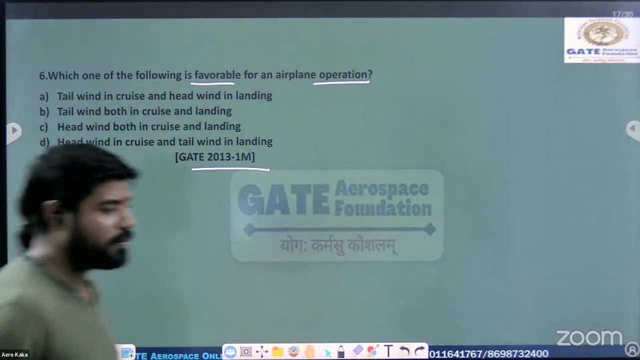 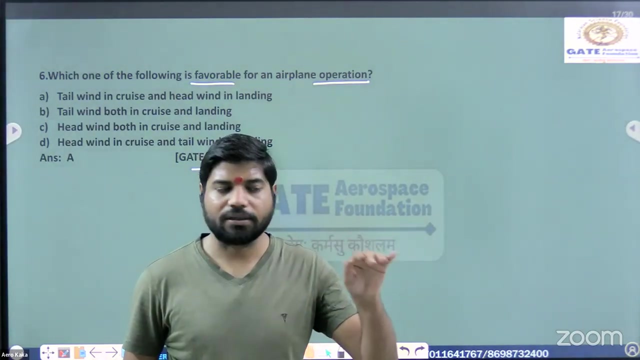 Which one of the following favorable for airplane operation. So first, tailwind in cruise and headwind in landing. So please remember like what During the time of takeoff and landing, Where- Takeoff and landing- this headwind is favorable right. But during the time of cruise- or you can say steady state in level flight- your tailwind is favorable. Okay, So just find out which option is correct. First option: tailwind in cruise. Second, headwind in landing option is correct. Option B here: tailwind both in cruise and landing? no, not at all. 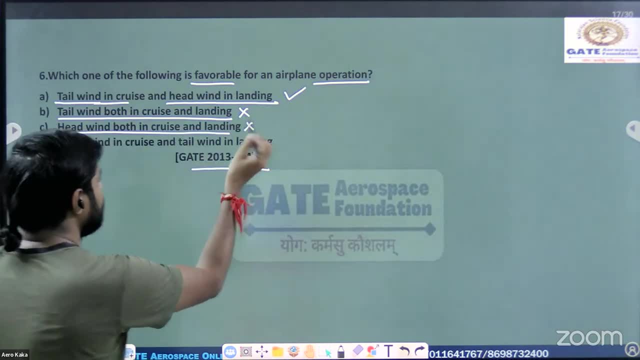 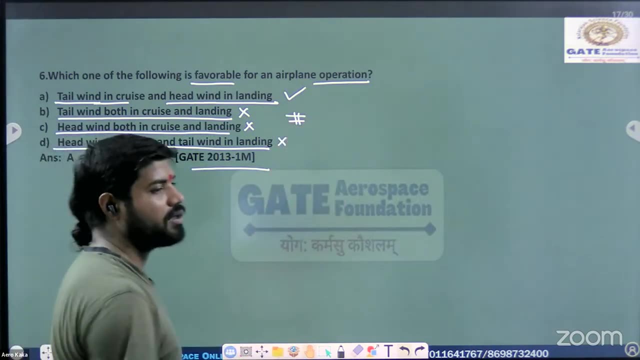 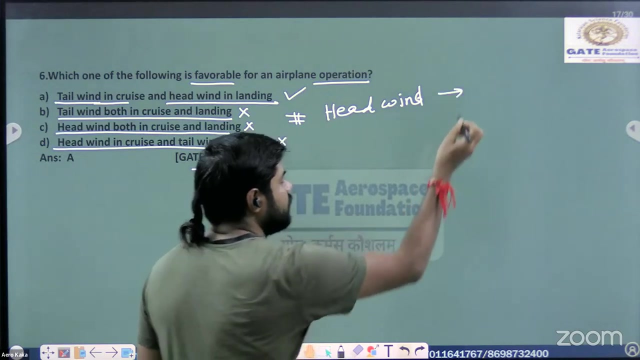 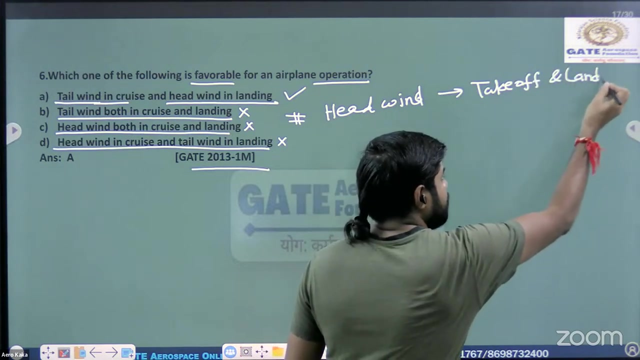 Headwind both in cruise and landing: no, Headwind in cruise and tailwind in landing- no. So if you want to write down something, you can write here one statement like: what Headwind is favorable during what Takeoff and landing Why? During the steady level flight or cruise flight, Your tailwind is favorable or it's a desired, So option A is correct here. right Check Now if an aircraft takes off with 10% less fuel in comparison to its standard configuration. 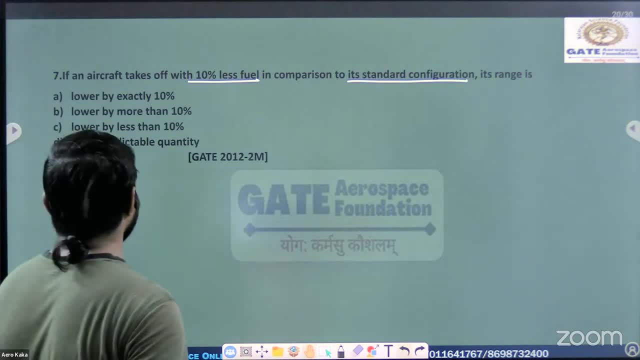 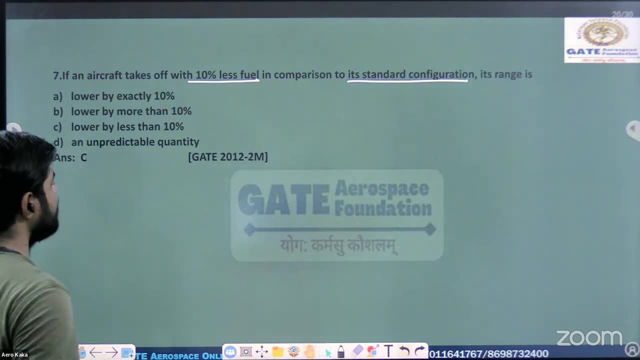 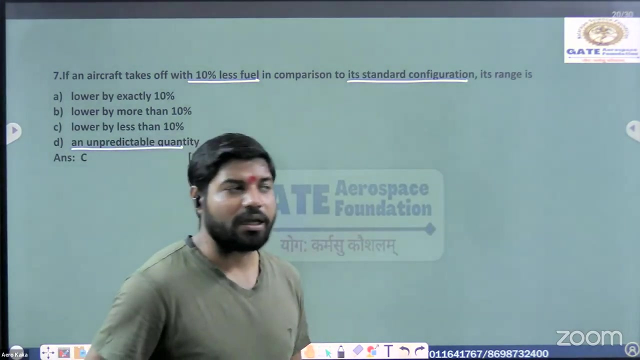 Its range is lower by exactly 10%, Lower by more than 10%, Lower by less than 10%. An unpredictable quantity. Yes, How to approach this question? Really, this question is very, very, very standard. No, Another problem with this question is that they are saying an aircraft, but they haven't mentioned 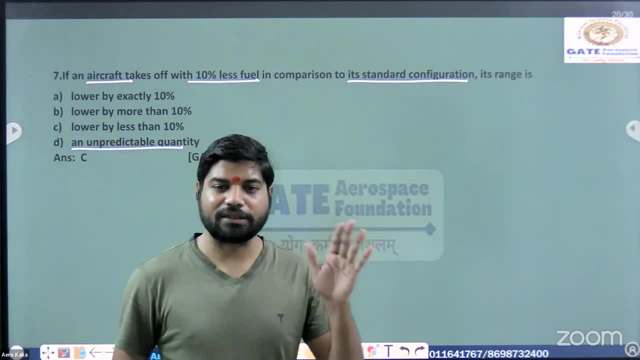 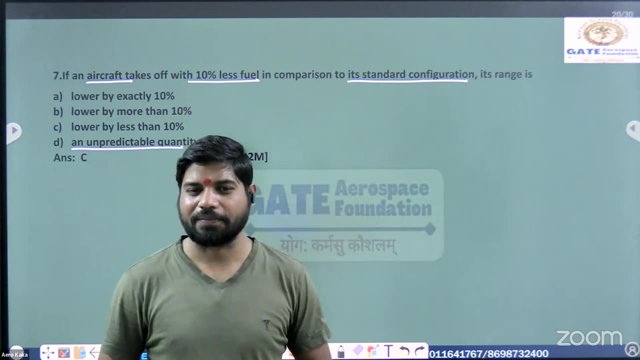 Hello, Am I audible? They haven't mentioned whether it's a propeller based aircraft Or whether it's a jet engine aircraft. Do you know? Hello, Check, Yes, Am I audible or not? They haven't mentioned like which kind of aircraft is this? 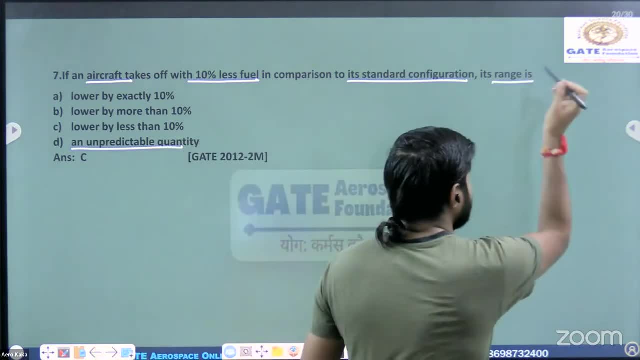 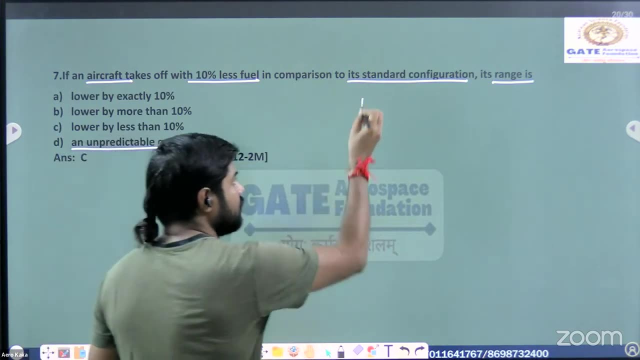 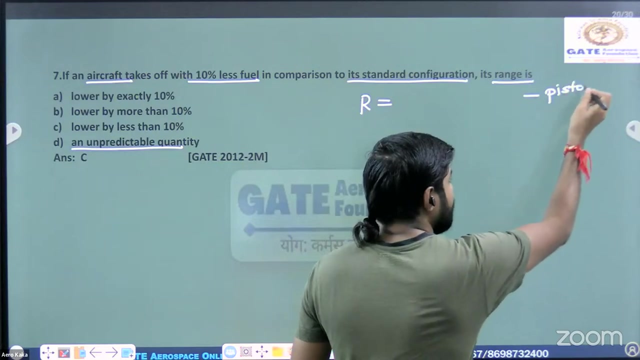 And they are talking about here the range of this particular aircraft. So how to approach this one? So what is the range formula? What is the range formula for piston engine aircraft? First, Can you tell me For piston engine aircraft? 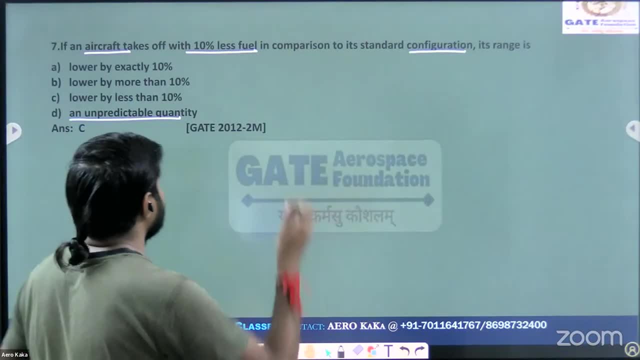 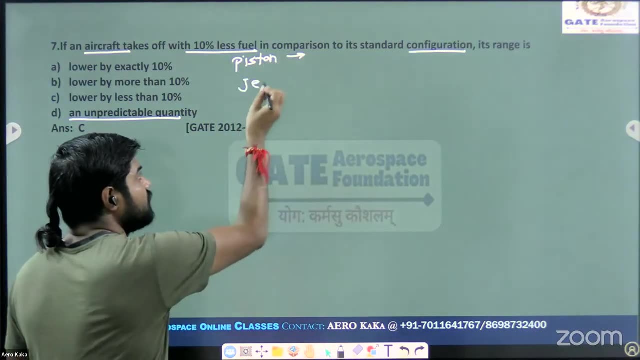 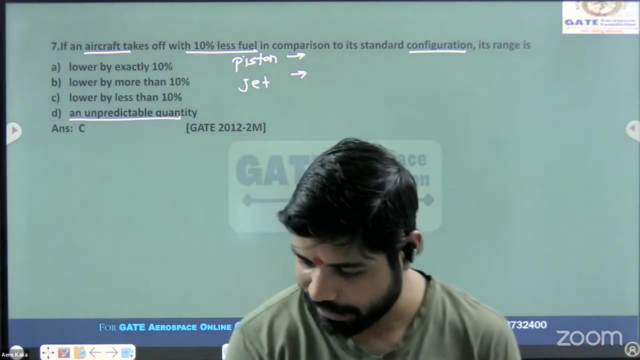 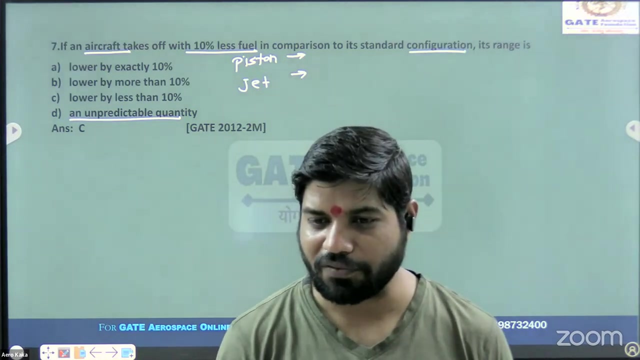 Just wait For piston engine aircraft, Then for jet engine aircraft. Yes, What is the formula? Yes, Please, Please, keep revising as much as you can, Otherwise you will struggle during those three hours. Remembering the formula is also important. 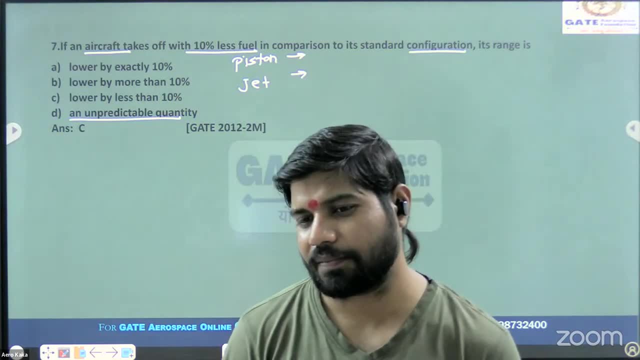 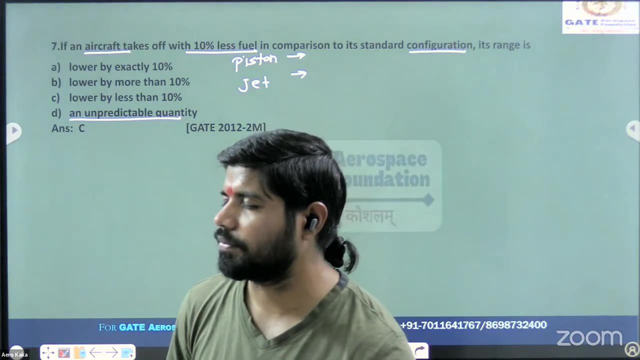 Sir Nita, prop by C into C, L by C, D, L, N, W, naught by W 1.. Okay, Come again. What is it, Sir, Sir? Sir Nita, prop by C, C, L by C D into L, N, W, naught by W 1.. 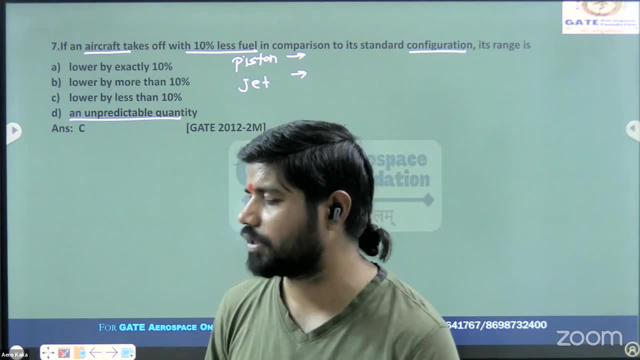 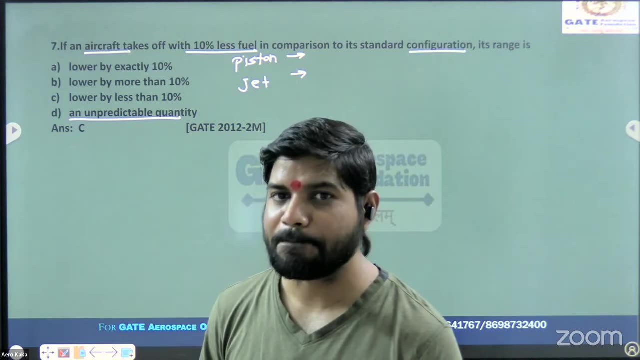 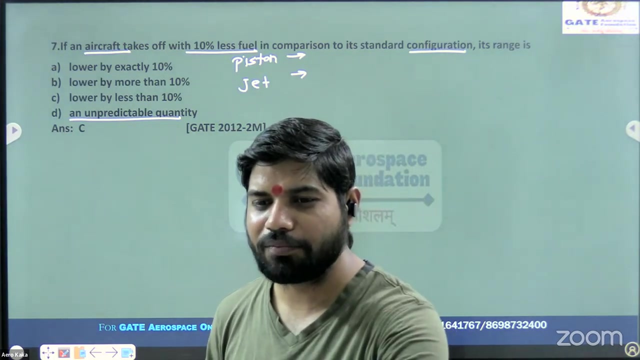 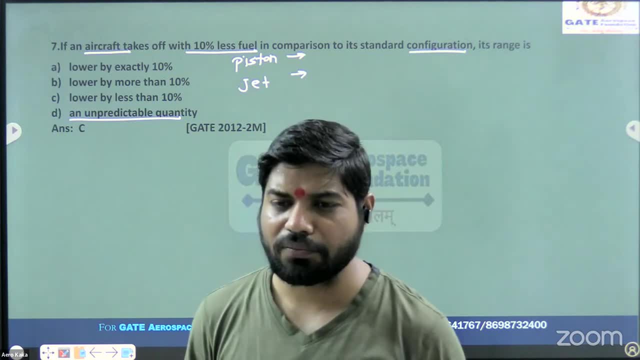 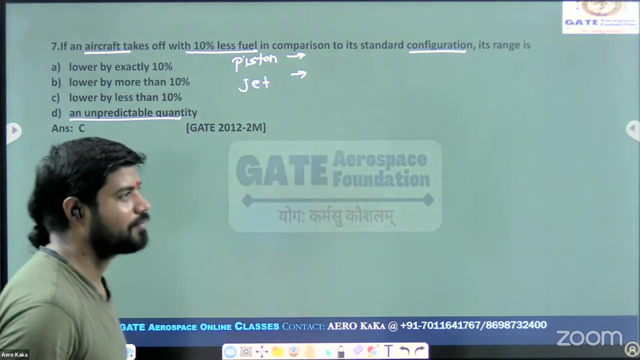 Let me check as a reminder, Sir. Okay, So you are wrapping your notes. Very good, Keep it up, Sir. Sir, Sir, power is 0.5 by cd under root, 2 by rho infinity s w naught raised to 1 by 2 minus w1 raised. 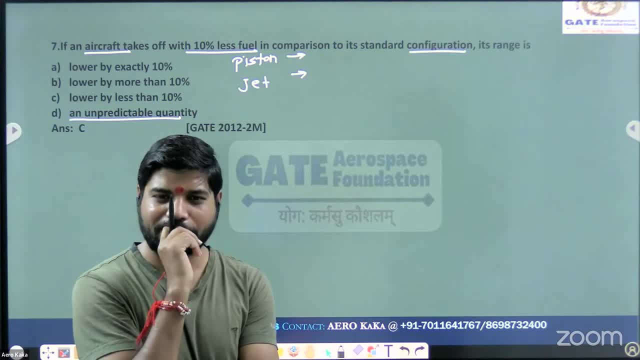 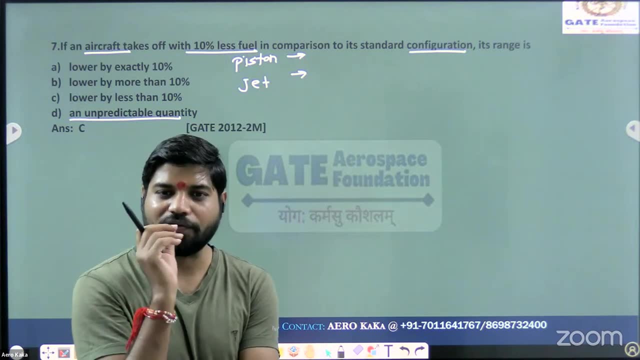 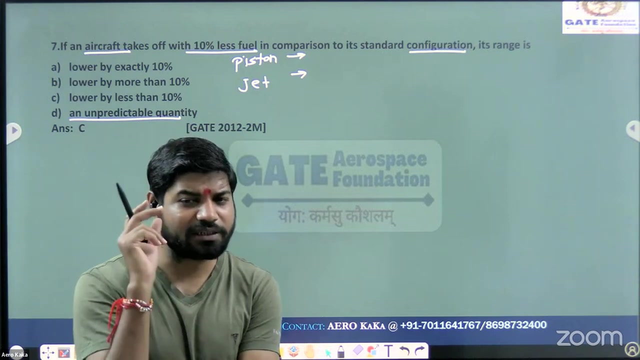 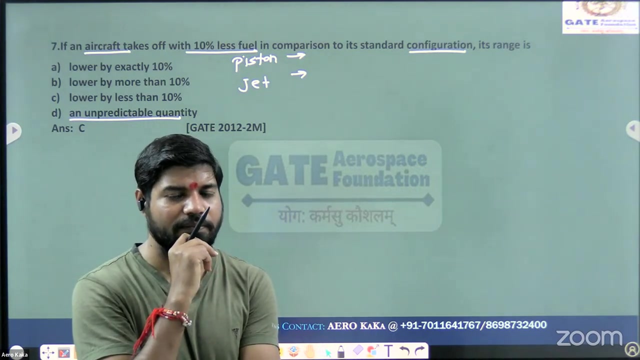 to 1 by 2.. Another one, Another problem. I am talking here about the range of a piston as well as the jet engine. aircraft Cl raised power. what is that? Cl upon cd? what is that? Yes, Cl upon cd, Sorry, yes. 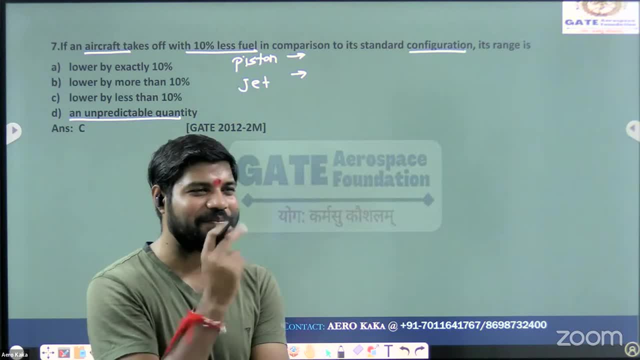 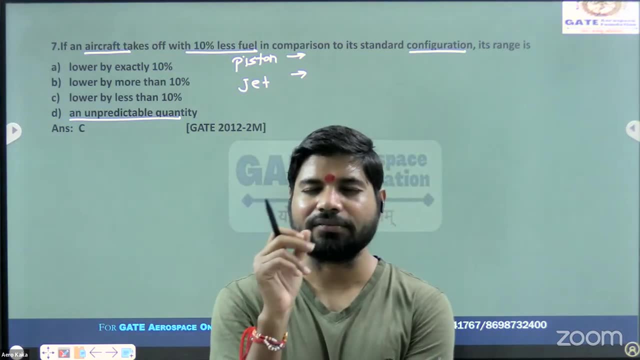 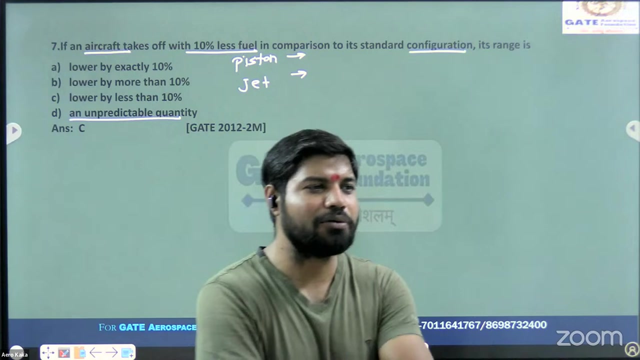 sir, Cl upon cd only. Okay, good, Okay, write down: For piston engine aircraft you can write: r? u is equal to eta y? c. Write down: r? u is equal to eta y c in Cl upon cd: ln of how much ln of w naught upon w1. 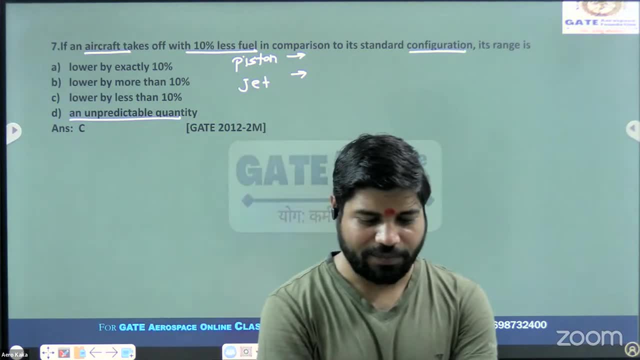 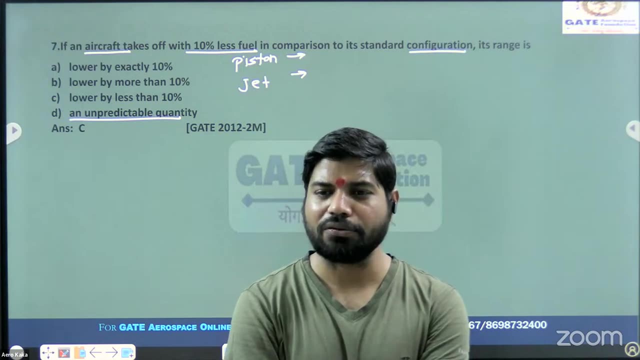 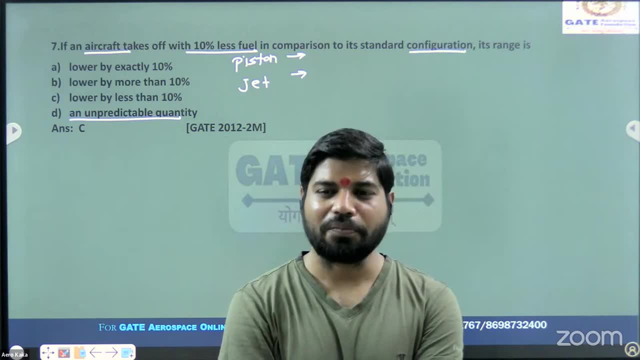 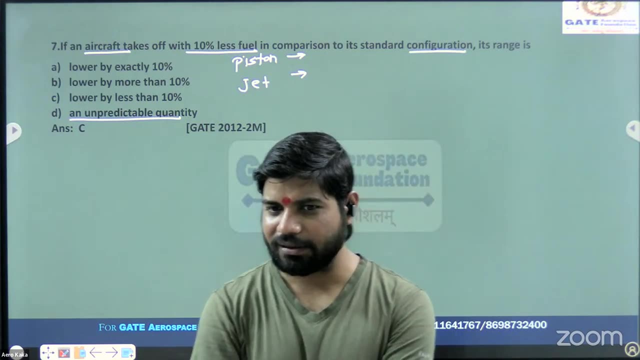 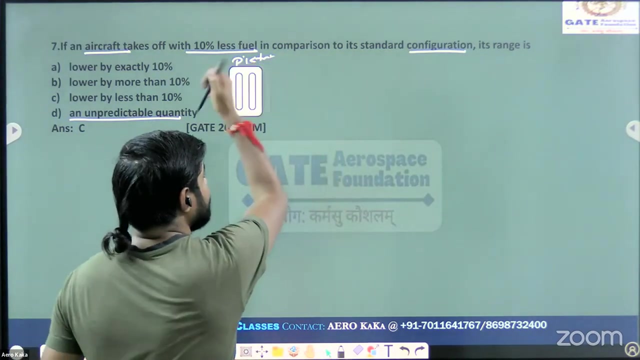 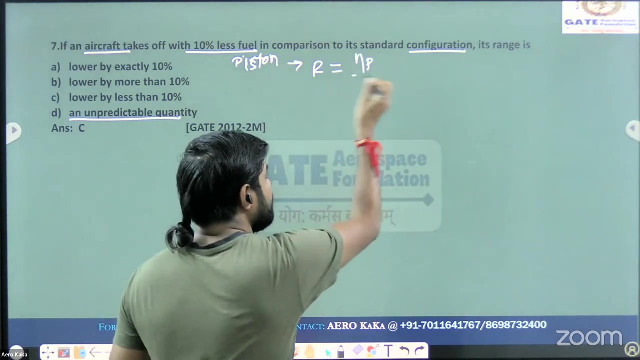 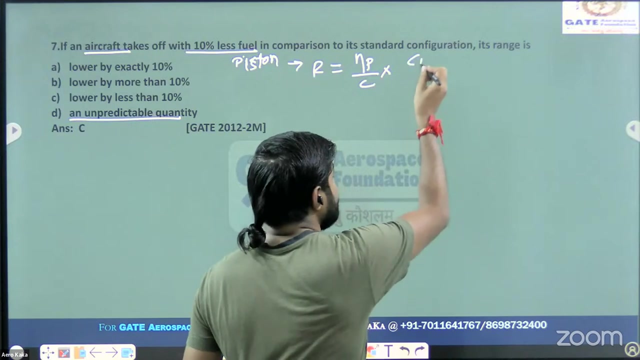 Cl power: 0.5 by cd, 1 by 2 upon cd in bracket root of w naught minus root of w1.. Is that clear Check? So just write down: r? u is equal to eta y c For piston engine aircraft. r? u is equal to eta y c into how much Cl upon cd or l by cd. 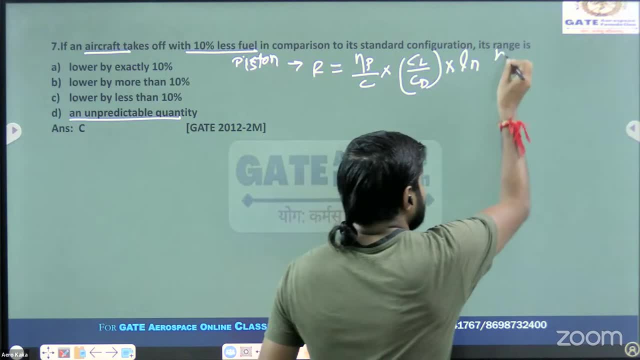 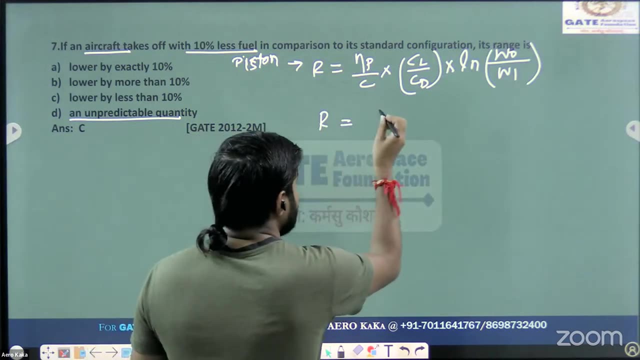 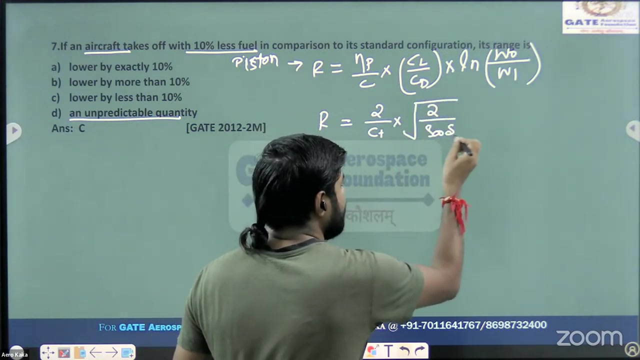 into ln of w naught upon w1.. Okay then r? u is equal to how much? here It's a 2 upon cd. Check into root of 2 upon rho, infinity into s into Cl. raised power 1 by 2 upon cd. into how much. 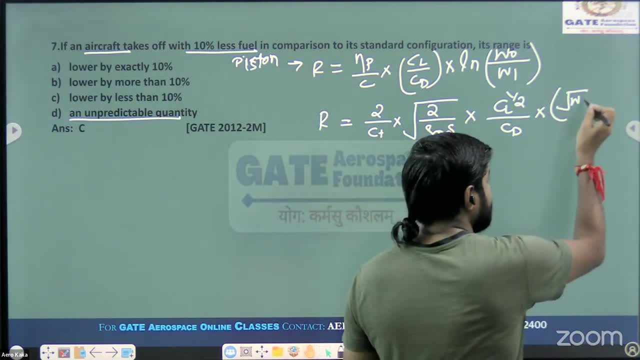 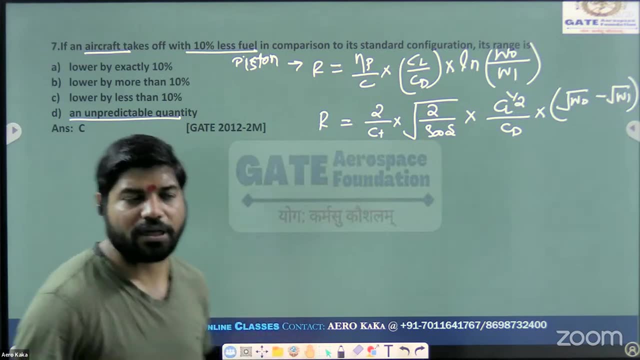 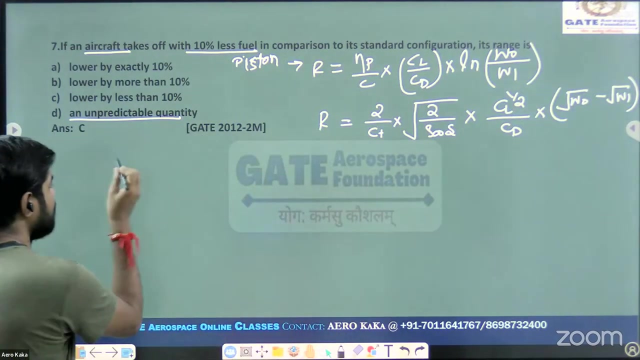 Yes, please. Root of Under w naught Minus root of Under w1. W1. Right. So now we are just only talking about like in terms of the fuel weight. So if you keep all the parameters, same right. So from these two conditions we can write: 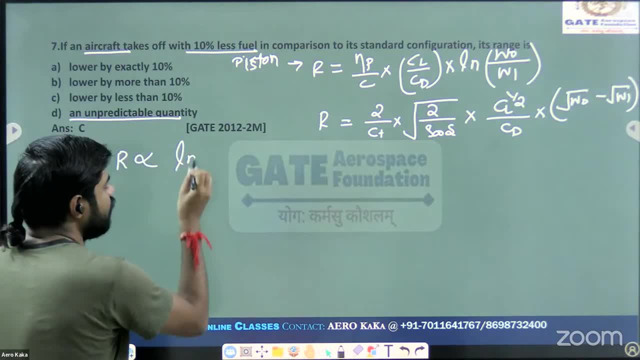 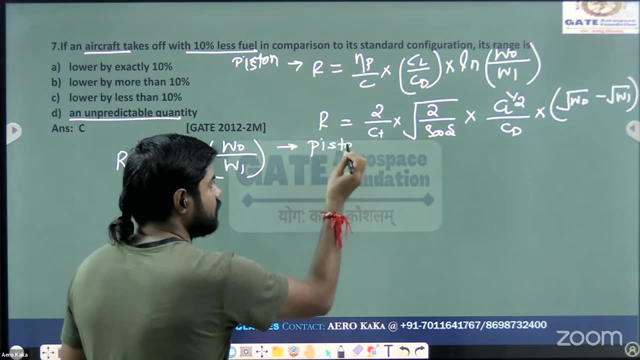 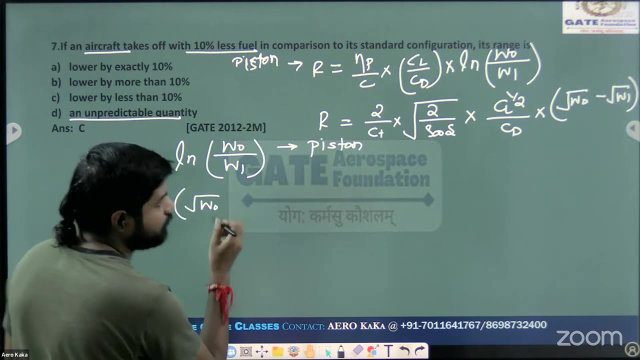 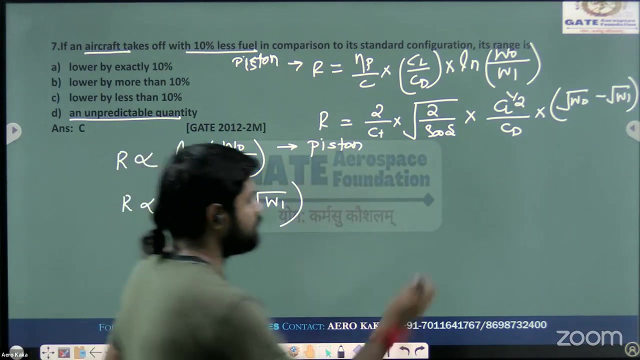 r is directly proportional to ln of w naught upon w1 for piston engine aircraft, And here r is proportional to root of w naught minus root of w1.. Check please Now. what is this w1?? Look, this w naught is made up of. we can say wf. 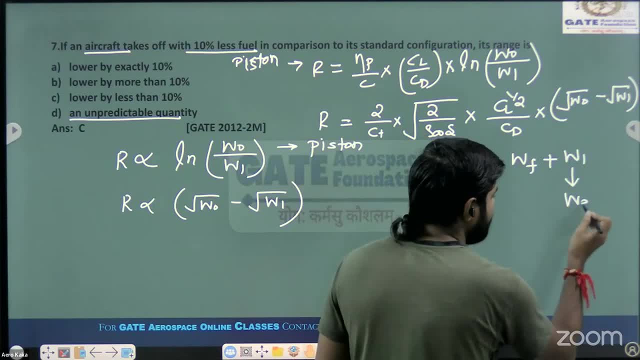 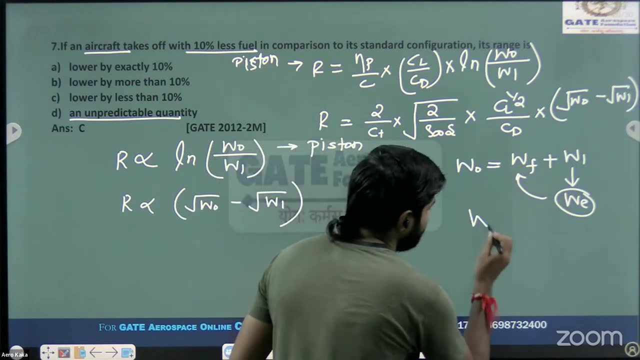 This w1 is nothing, but you can see We are considering yourself, w, this is the weight of the aircraft, except weight of the fuel. So let's consider, And that here, w0, u, Wf, That's what I'm considering at this particular point. 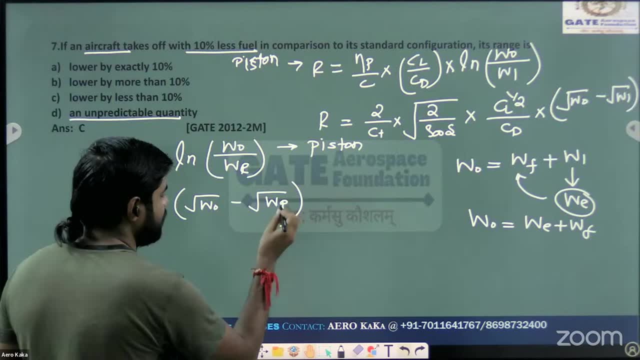 So here you can take: This is we and this is also we. So First we have to discuss with jet engine or piston engine. Let me know first Which one is frequently used, Which is most commonly used. First we're talking about the jet engine. Second, you are cheeky as compared to the. it can be counted in the vehicle whether it's a jet engine or a piston engine. So first we've got a job right. A jet engine From the engine, a piston engine to the engine. So yeah, the engine engine When Pilot mechanics utilises. 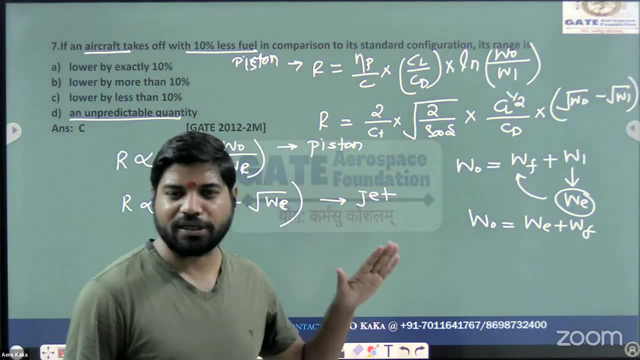 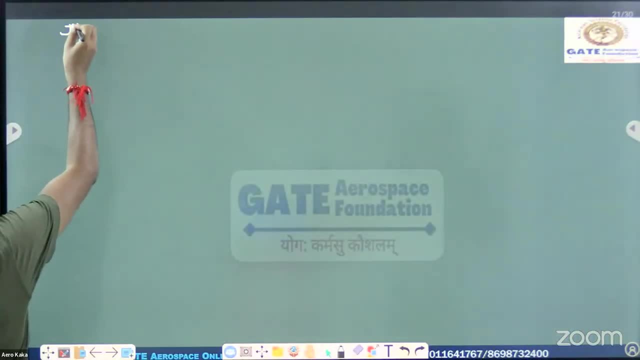 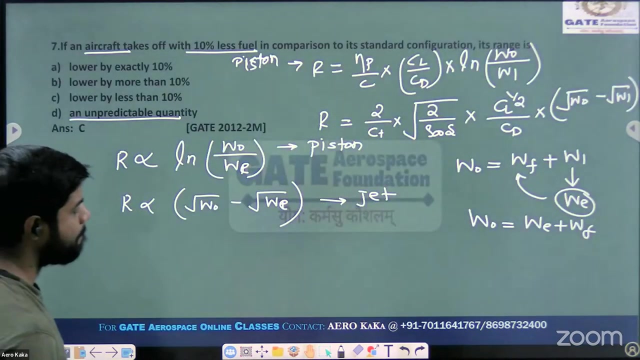 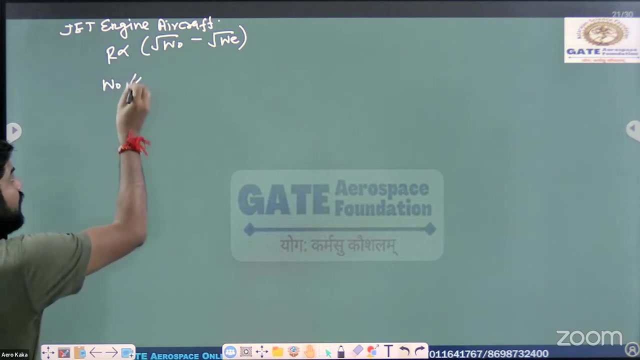 me know first which one you want to discuss here: jet engineer numbers, jet engine aircraft. okay, so right now for that engine aircraft, for jet engine aircraft, r is proportional to root of w naught minus root of w right. check, please, are you agree? okay, let's say w north and w e is the actual configuration. 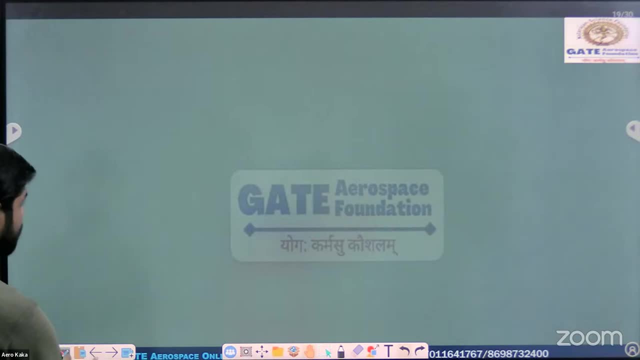 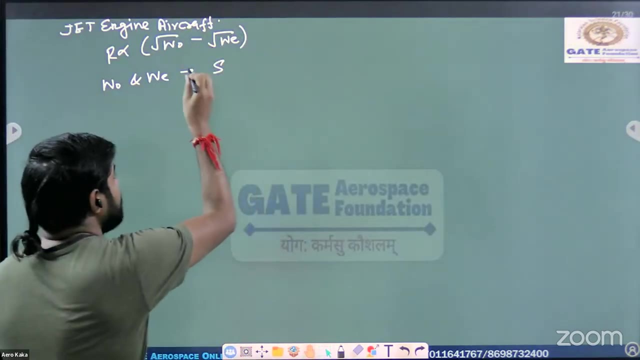 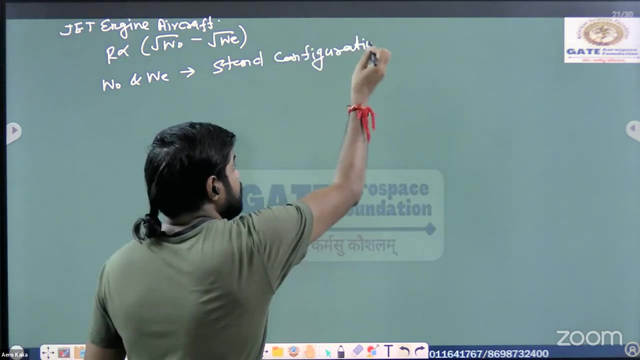 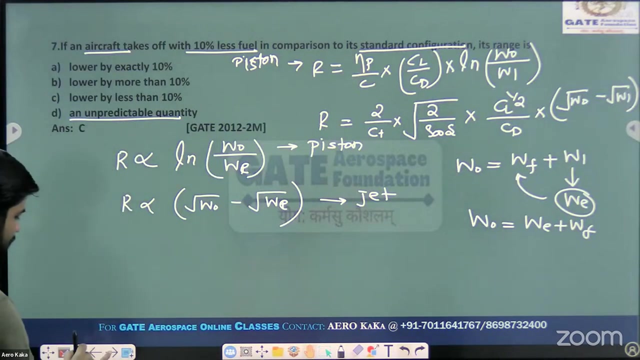 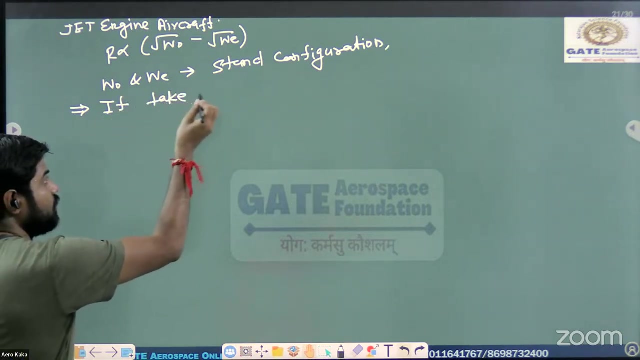 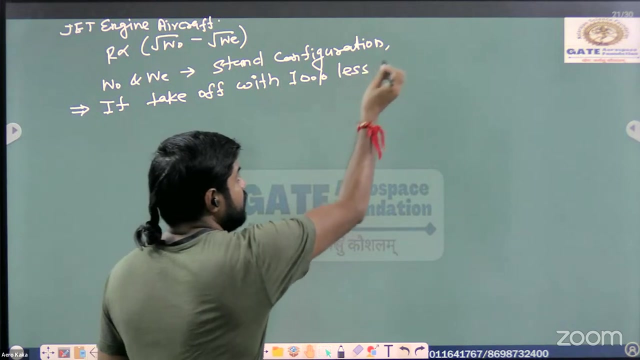 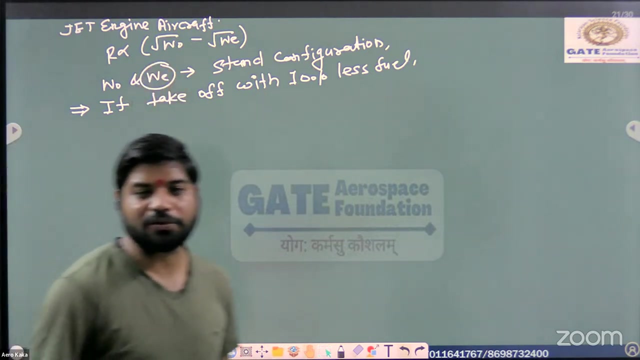 actual oregon city standard configuration corresponds to stem. let's say now what this is. if suppose it takes up with 10 percent less fuel? if take off with 10 percent less fuel, then what happens? is there any change in w e? hello, if suppose if this aircraft carries 10 less amount? 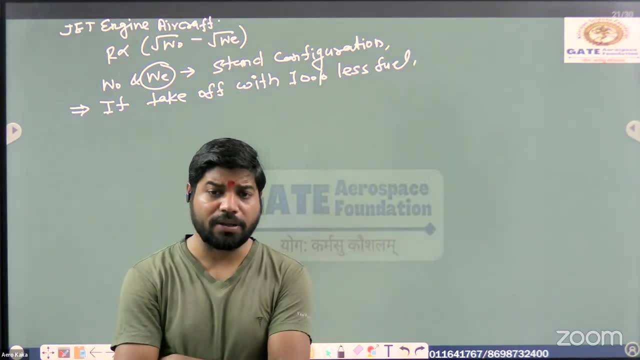 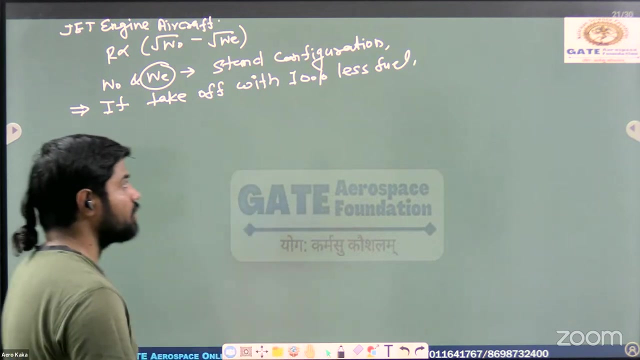 of the fuel. then is there any change in this w e? which weight will increase or decrease? or you can see which is the function of this wf here. obviously, w not only right. hello, am i audible? check, yes, sir. so here, whether it is carrying 10 percent more amount of the fuel or it is carrying 10 percent. 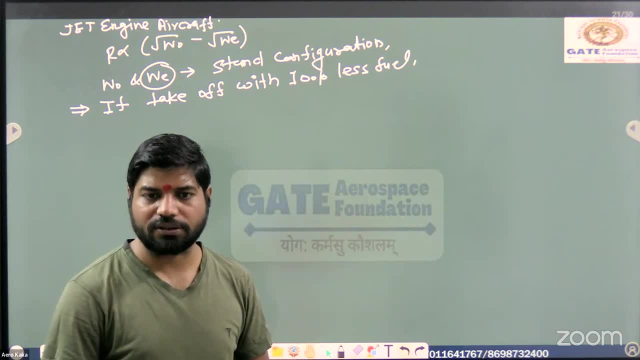 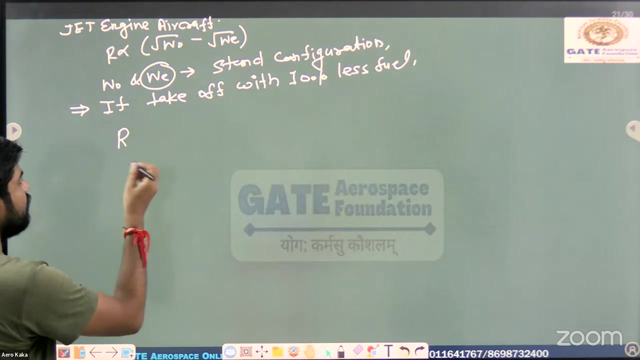 less amount of the fuel, the value of w? e is not going to change, right? am i audible? i did. are you getting this one or not? so just just discuss. so let's consider. okay, in this case, consider, this is nothing, but you can say r prime here. okay, the range. in this case i'm considering. 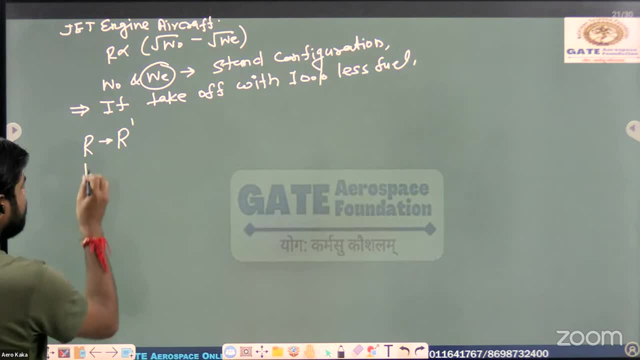 okay, this is nothing, but you can say r prime here. okay, we range. in this case, i'm considering, Let's consider this: r becomes r prime, w0 becomes w0 prime. in this case, and your, we is not going to change Okay, so let's write here this r prime is proportional to how much. 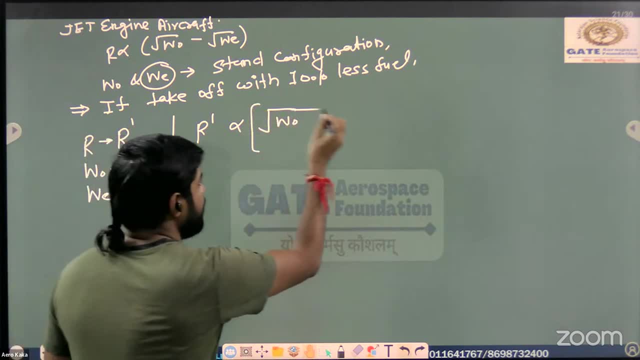 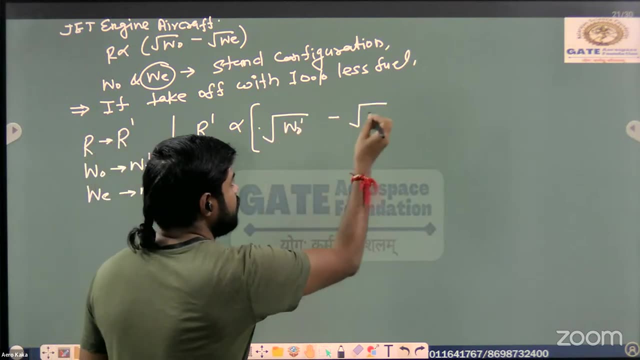 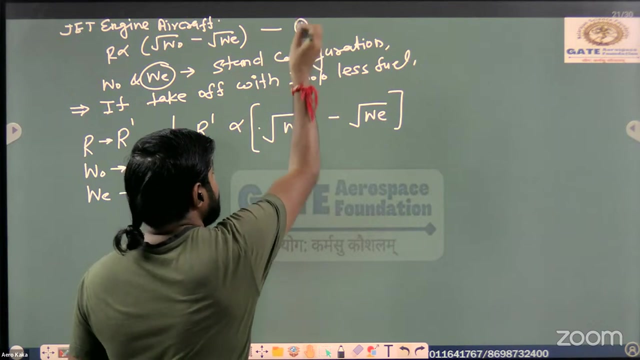 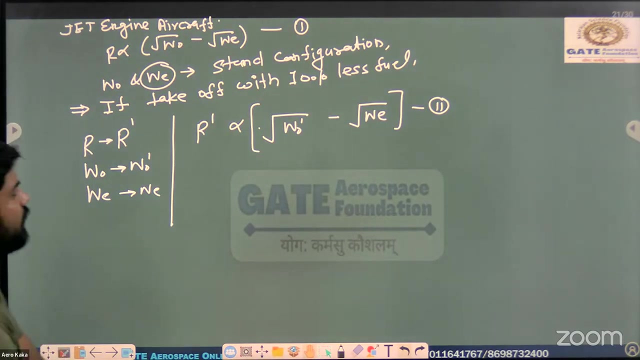 root of w0, check. So I am writing here: it is w0 prime minus root of we check. Here goes let's say this is nothing, but you can say equation number 1. and this is nothing, but you can say equation number 2.. Or if you want to simplify it further, right, what we 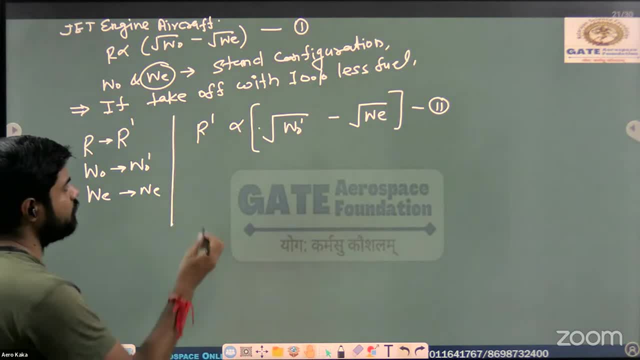 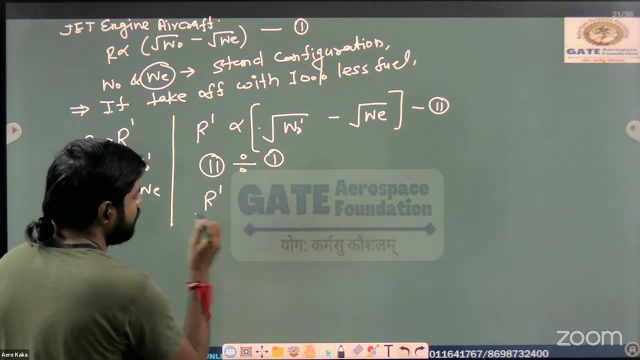 can take. Okay, no issue at all. Take the ratios of these two. take here, let's do it here, Let's do it here. Take the ratios of these two. take here, let's do it here. Let's divide equation 2 by equation 1.. And what you can write, You can write r prime upon. 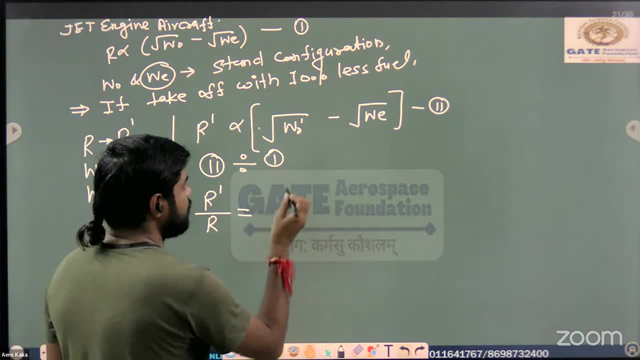 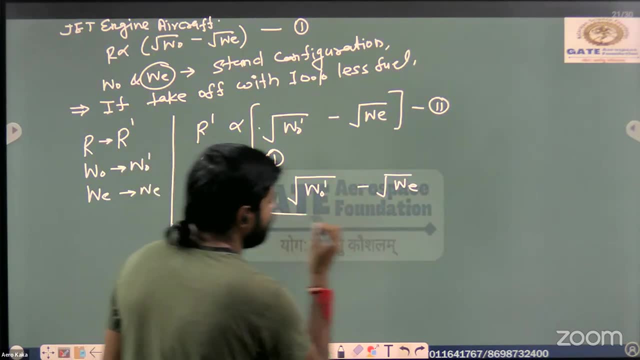 r, which equal to how much? Yes, how much we will get Root of w0 prime minus root of we. check please. Divided by how much Root of w0 minus root of we. Are you agree? Check please? Yes, sir, Okay. 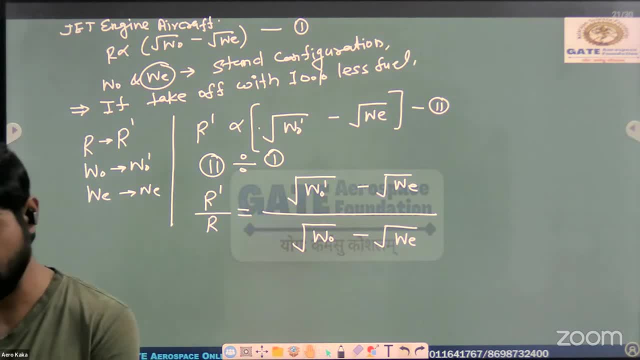 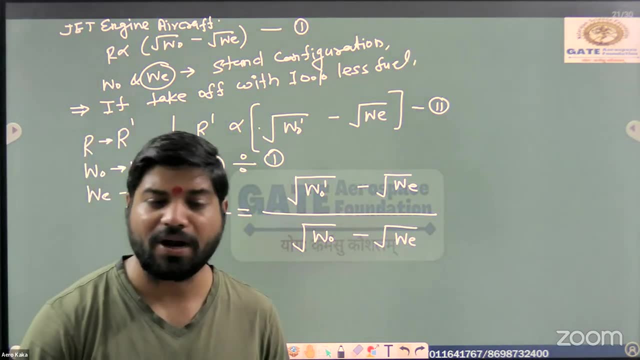 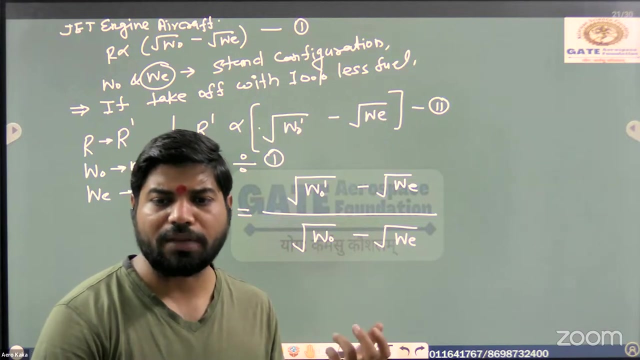 Now what you can do, Anyone, What we can, Taking under root we common from the numerator and denominator. What you can do here, Just remember: w0 is nothing, but you can say we plus wf, right. Similarly, what you can write: w0, prime, which equal to how much We plus. 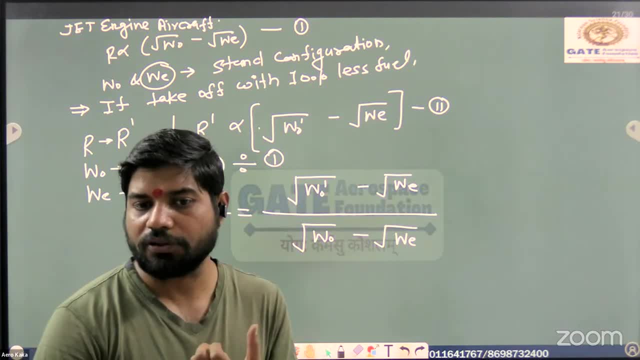 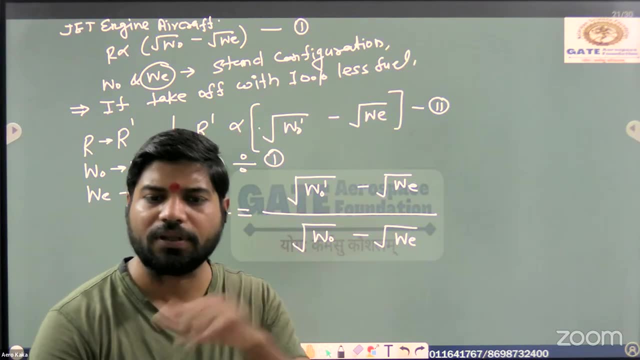 0, 10% less amount of the fuel. So please take care. Then you can write w0 prime, which is 0.9 times of wf. Just put here and simplify, You will take. or you can simplify it further in terms of what you know: w upon wf, or you can say wf upon w. Consider that wf upon w. 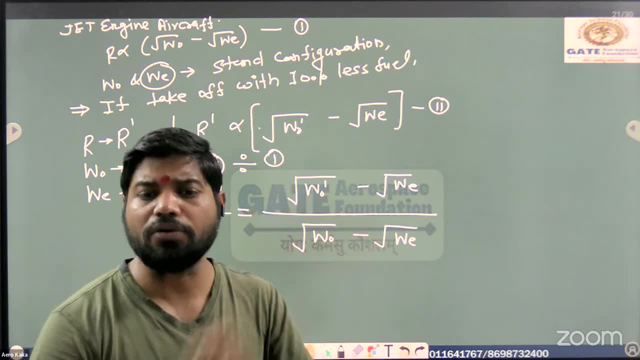 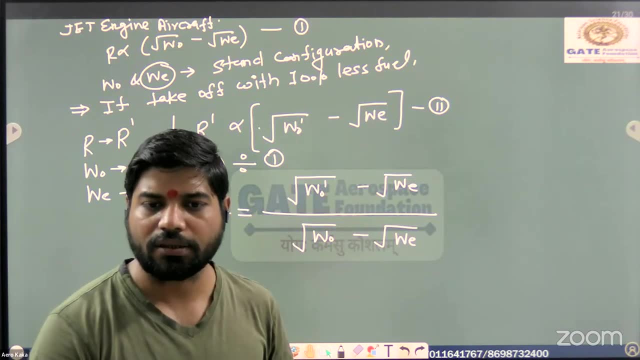 or w upon wf as a x, and take the two limits When this x tends to 0,, then what happens? And then, second is what When this x tends to 1.. Okay, So you can take both the hypothetical conditions You can take. let's say this x is equal to x tends to 0. So first consider: 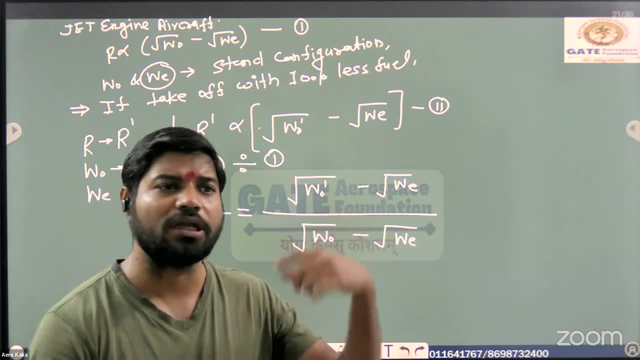 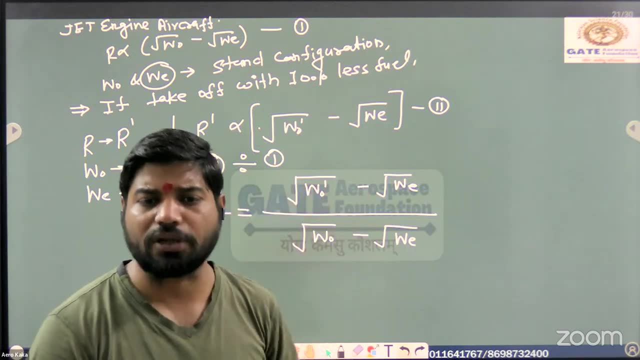 x is equal to 0.1, then consider x is equal to 0.2, 0.4,, 0.5, 0.6, and let's say up to 0.9 or 0.99.. Even you can consider x is equal to 1 and calculate like: what is the range. 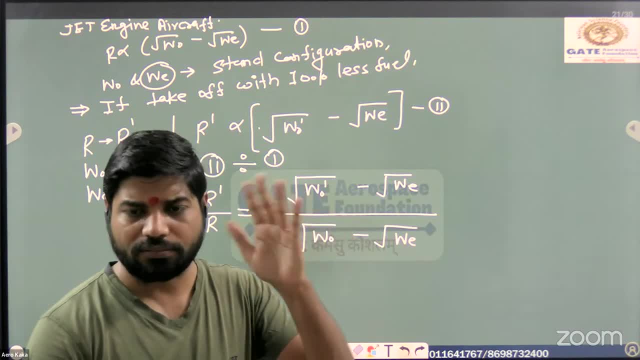 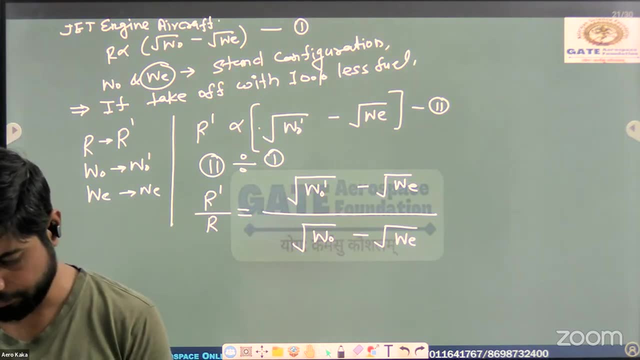 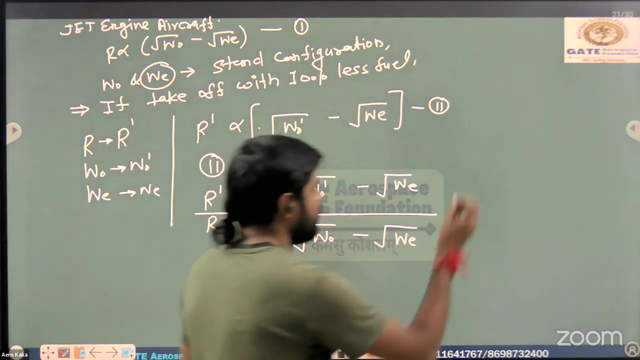 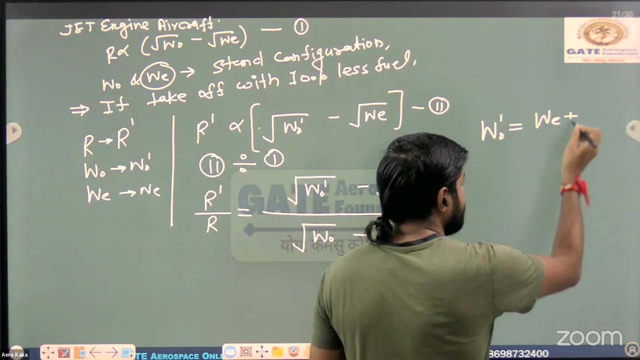 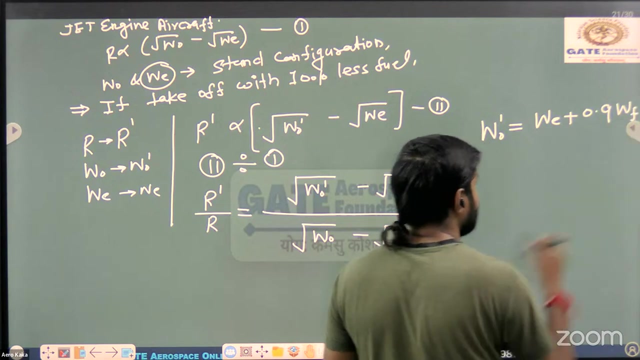 here, Whether it is decreasing or increasing, means beyond 10% or not. So just calculate, Take your time. Okay, Let's define once again. So this w naught prime is equal to how much here? You can write it as we plus 10%, less amount of the fuel. So you can write your 0.9 wf right. 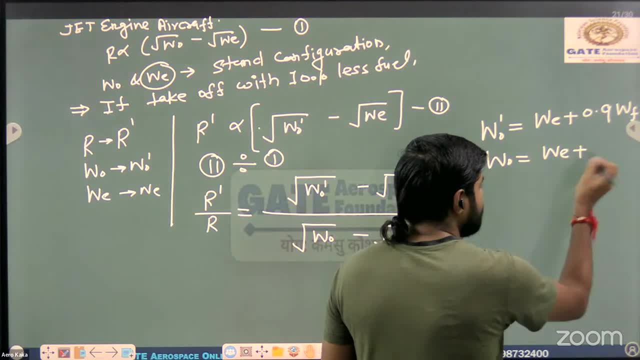 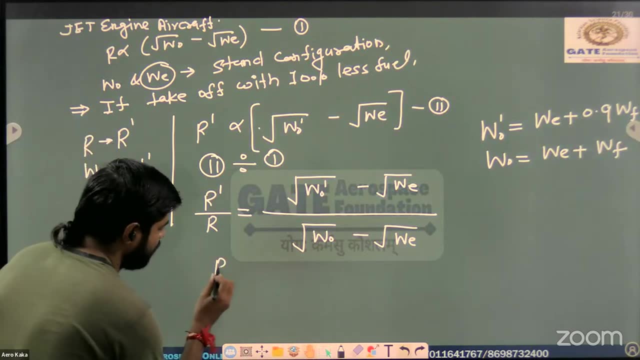 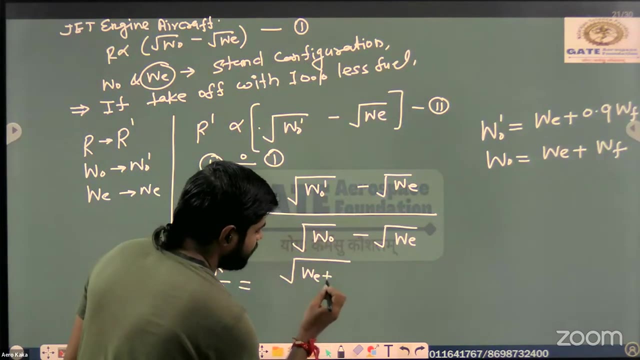 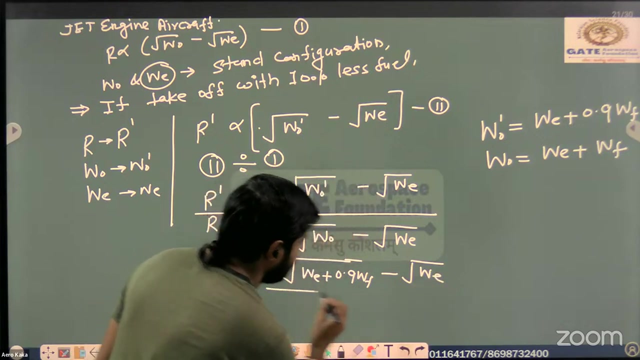 What is your w naught? It's the actual condition: we plus wf Right Check. Put here and simplify R. prime upon R is equal to root of what is w naught. It's a we plus 0.9 times of wf, minus root of we divided by root of w naught, minus root. 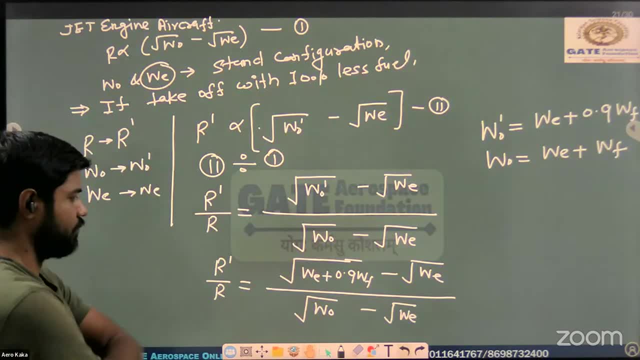 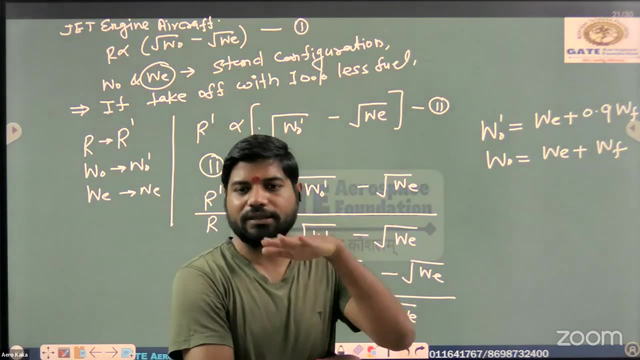 of. we Check Now what we can do. Since this is a w naught, we can write it as wf minus wf. This we value is not going to change right, Whether it is carrying the same amount of the fuel, less amount of the fuel, or you can say more amount of the fuel, So you can. 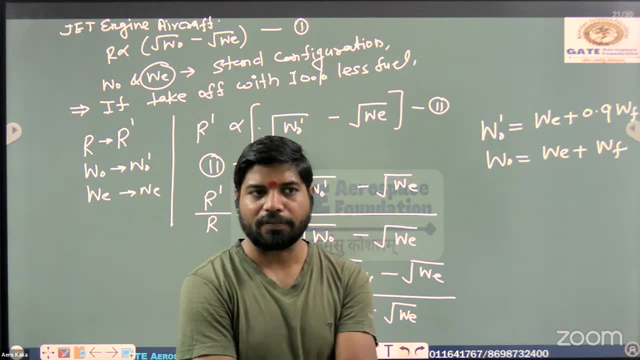 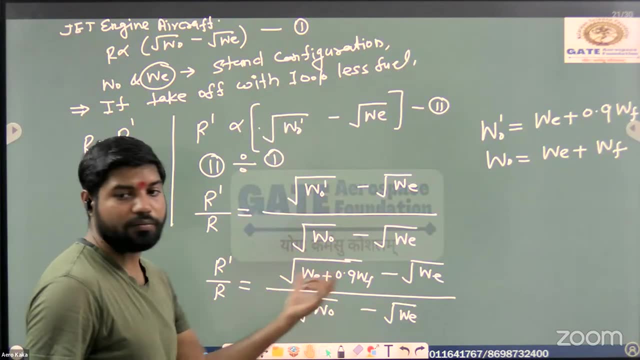 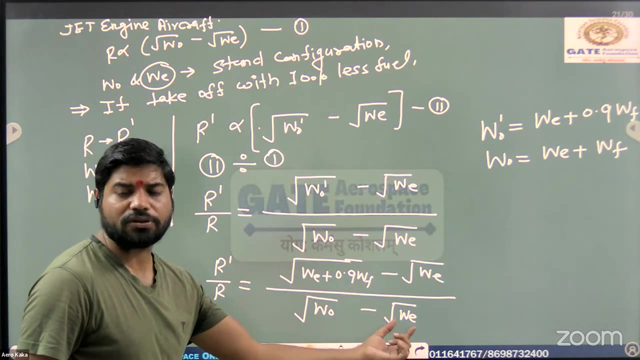 take this we common here. Okay, Am I audible or not? So we can take this we common in this. and then we can take this root of w common in this numerator. Similarly, we can, or we can, follow the same approach, You can take root of w common in denominator, and just simply. 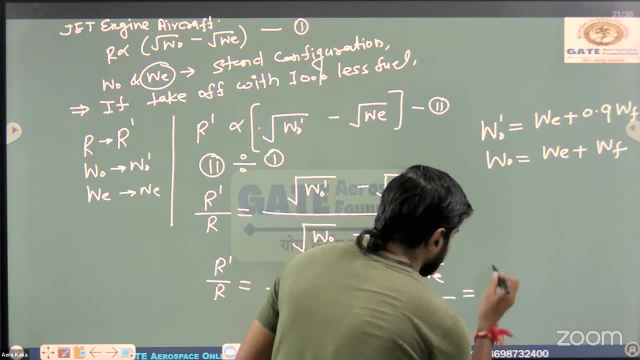 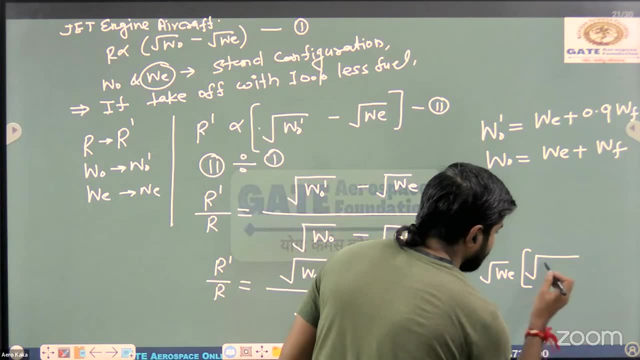 call it. So let me write here: root of w, e. If you are taking the common in the numerator, then how much you will get, You will get root of. let me write first: 1 plus 0.9 times of how. 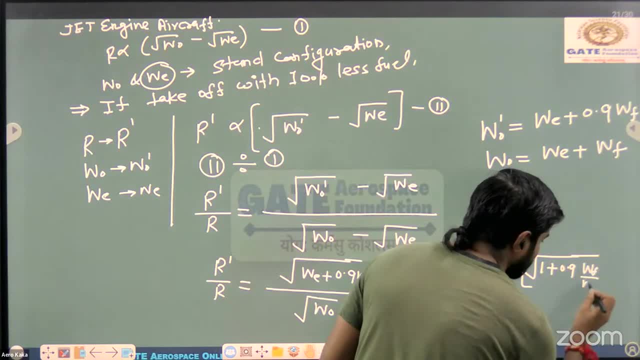 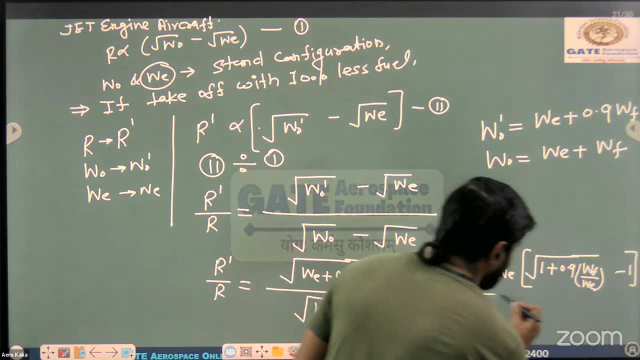 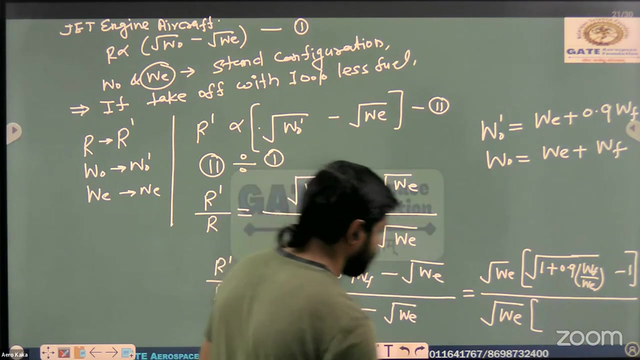 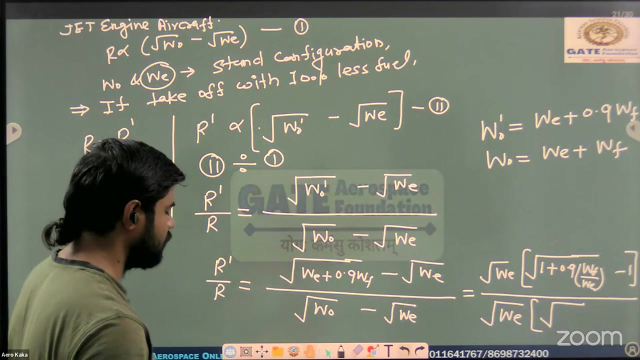 much wf upon. we Please verify: Yes, sir, Minus, how much Minus. 1. Agree Divided by take here root of w, e common in denominator as well. so how much will get root of how much w naught? what is w, what is w plus w f? this w naught is: 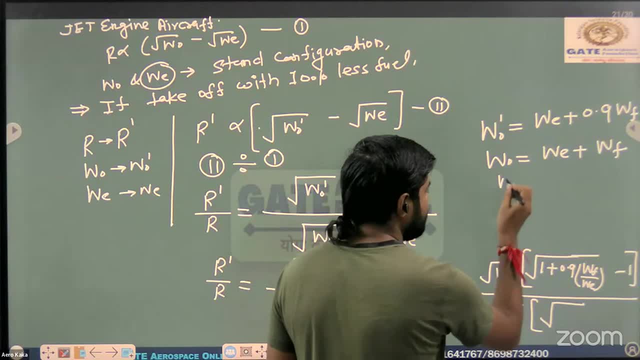 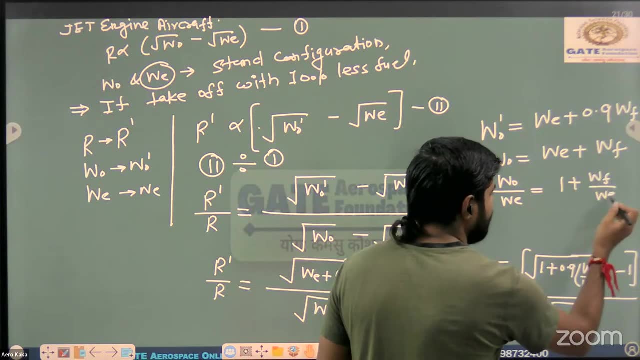 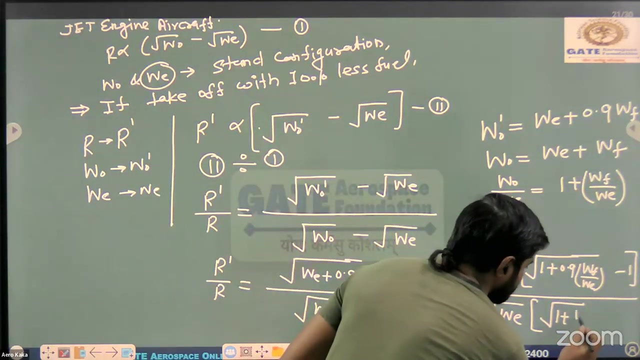 nothing but w e plus w f, right? so if suppose, if you are writing this, w naught upon w e, so this is equivalent to what 1 plus w f upon w e. please verify, agree, check. yes, sir, hello, so shall i write here directly? i can write here: it's a 1 plus w f upon w e, plus how much plus. 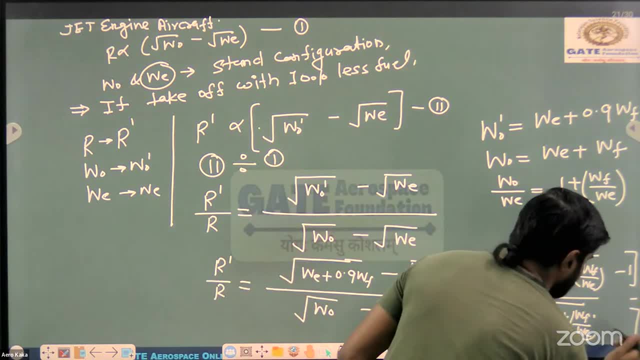 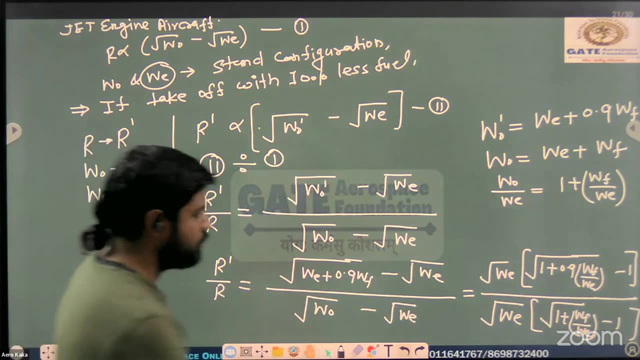 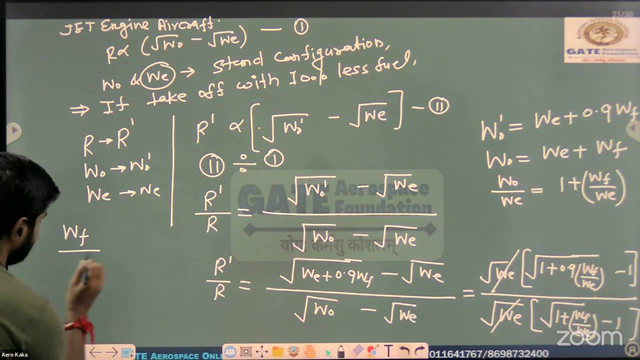 1 here, plus 1 or minus 1. sorry, minus 1 minus 1, clear, okay. so this root w e and root w e is get cancelled. now what we can assume. let's consider this: w f upon w e, where it's a fraction right weight of fuel divided by, you can say empty weight or you can say your, your, your. 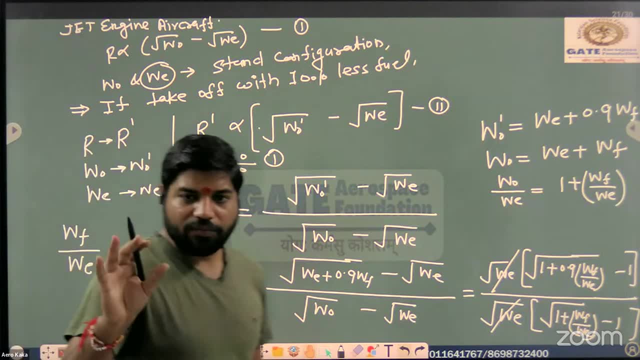 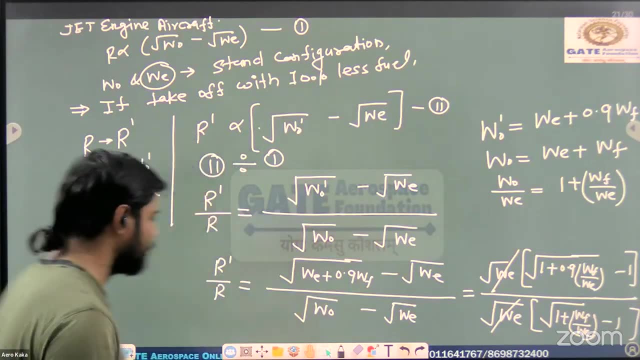 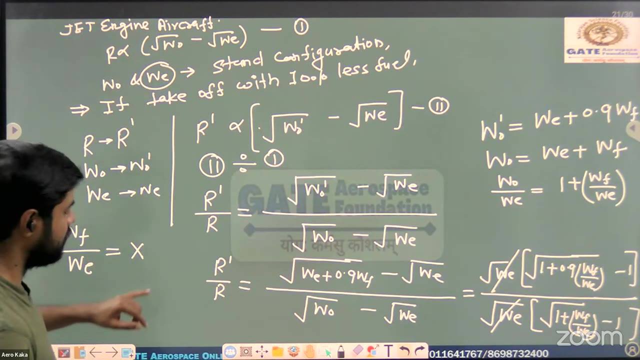 means the weight of the aircraft. it's the overall weight of the aircraft without- or you can say excluding, the weight of the fuel. that's it okay. so here let's consider: this is nothing, but you can say capital x here. okay, so what i can write, if suppose, if i want to write here further, 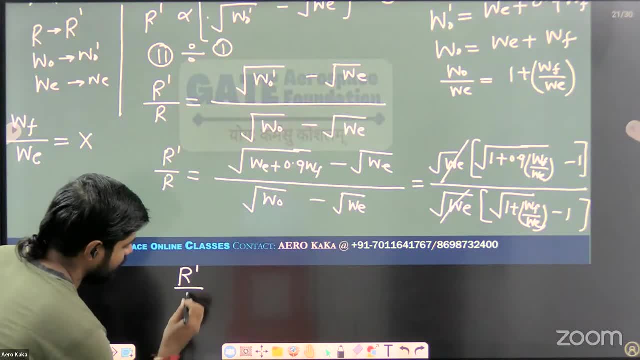 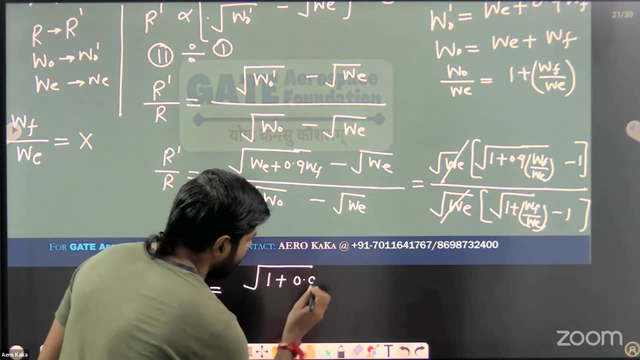 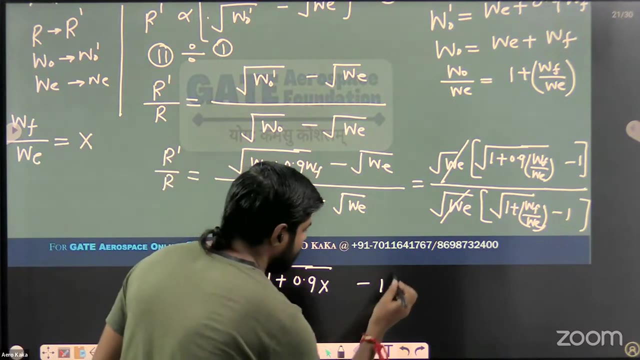 i can write here: it's r, prime, how much you're getting. you can write: it's a root of 1 plus 0.9 x, agree, check, yes, minus. what is the value of root 1? it's a 1 only. that's why i've written directly 1 here. okay, divided by how much? 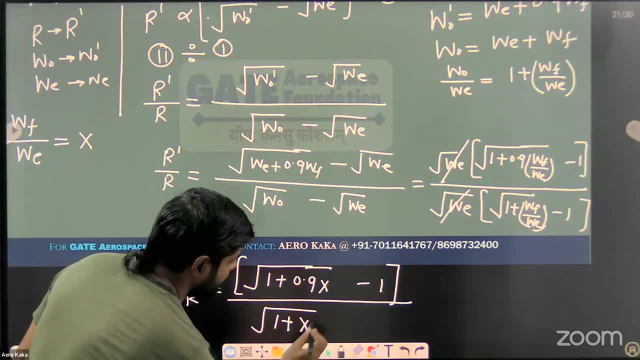 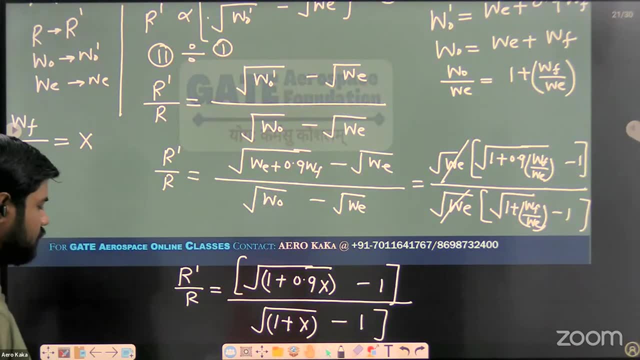 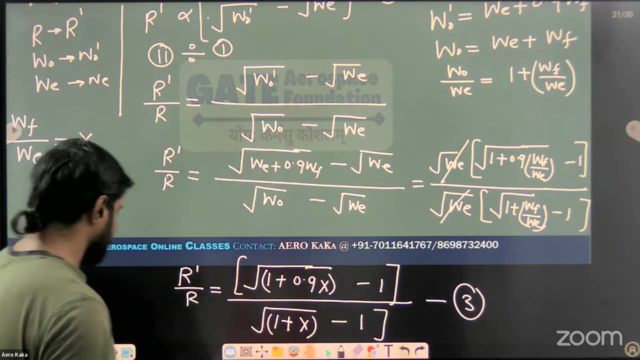 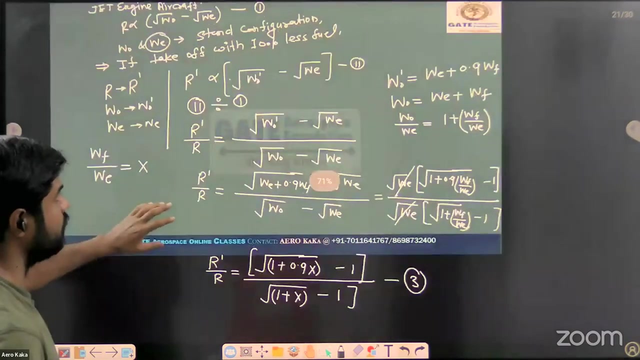 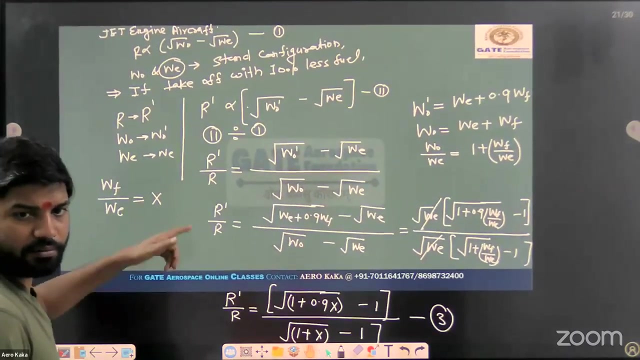 root of 1 plus x- right check, please- minus 1. hello, am i audible or not? yes, this is nothing what you can see. question number three: okay, just help me. do you want these ppts? if you want, i can share with you. hello, okay. so so here you can write. 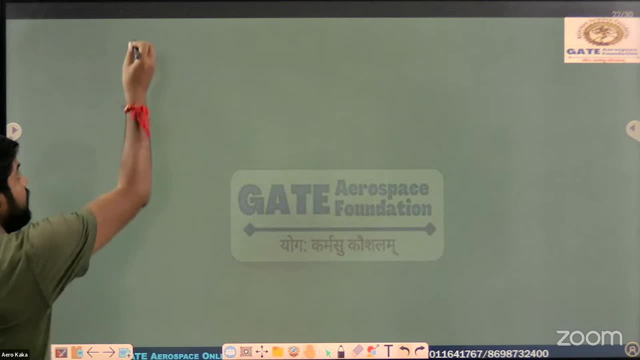 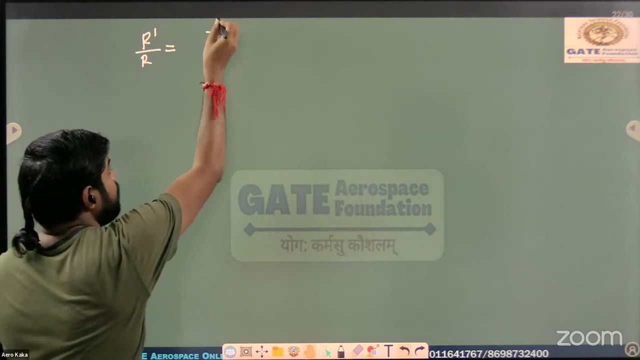 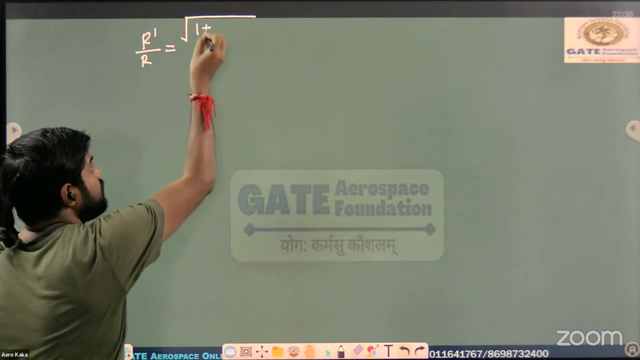 here you can write this: tell me how much we're getting r prime upon r usual. yes, please, how much you're getting, sir, 1 plus 0.9, right? yes, sir, root of 1 plus 0.9 x. right minus 1 minus 1, that's in numerator divided. 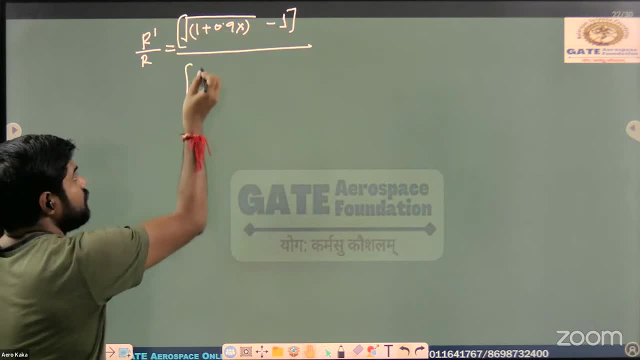 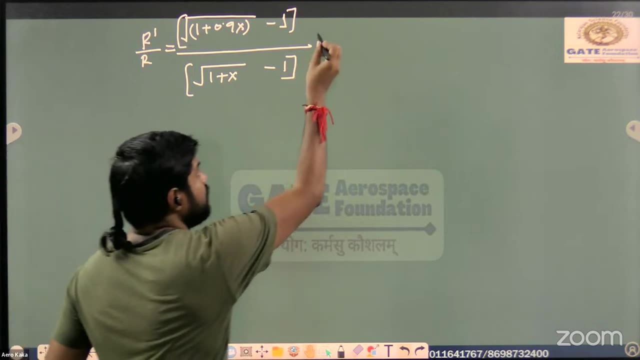 by how much? root of 1 plus x, root of 1 plus x, root of 1 plus x. one plus x minus one one. that's what we have taken. situation number three: now, what is required, they're asking. what is the percentage change right? what asking, they're asking. 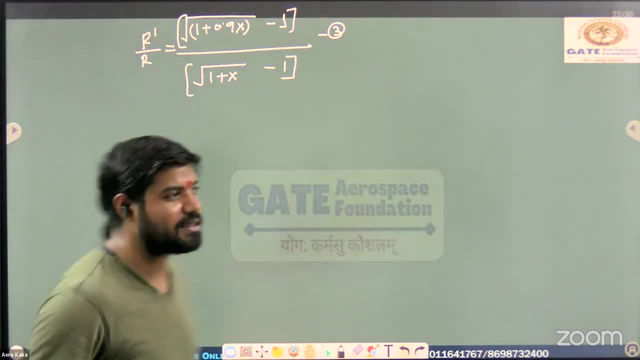 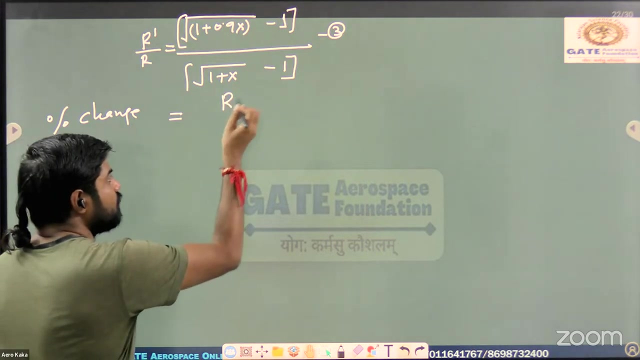 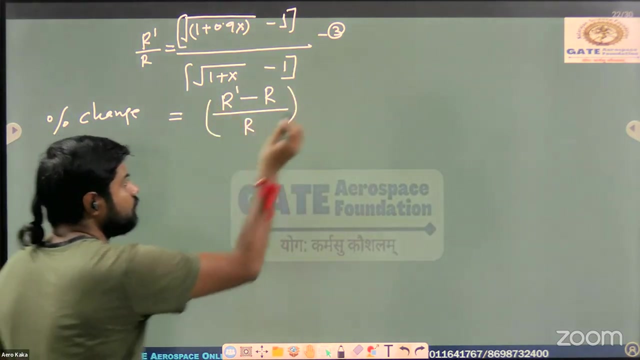 what is the percentage change? how to how to calculate the percentage change? yes, so you can write the percentage change is how much here? percentage change in range: you can write. it's a final value, that's r prime minus initial value, divided by initial right into 100 percent. 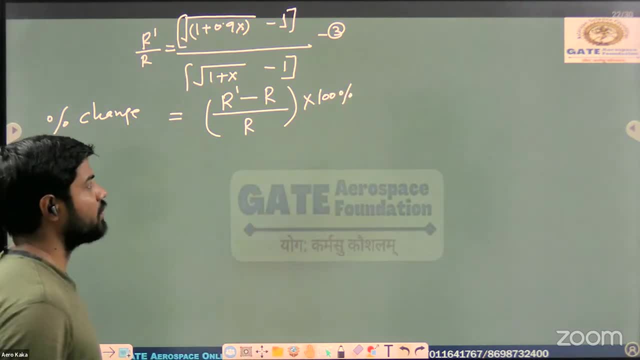 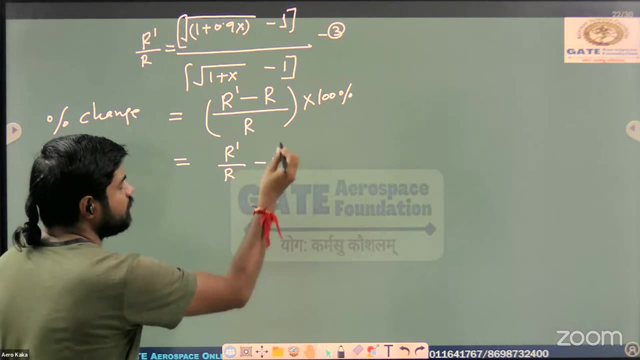 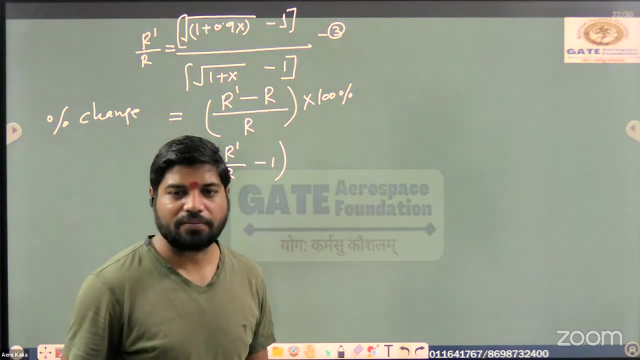 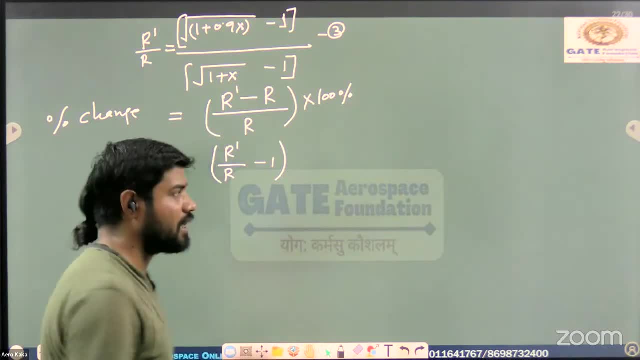 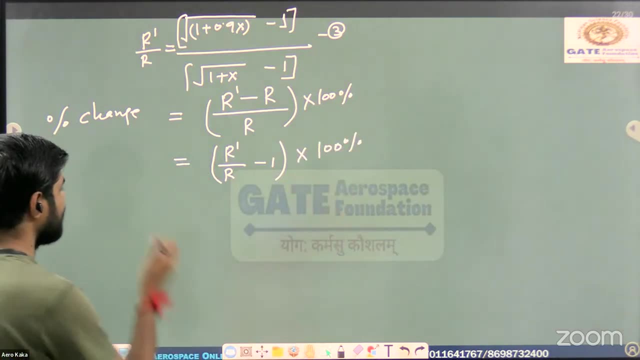 you are having. you are having this r prime upon capital r, right, just calculate what is this r prime upon r minus one, okay, and then calculate what is the percentage change. so just wait, okay, let me write here: this r prime upon r minus one is equal to how much you can write. it's a root of. 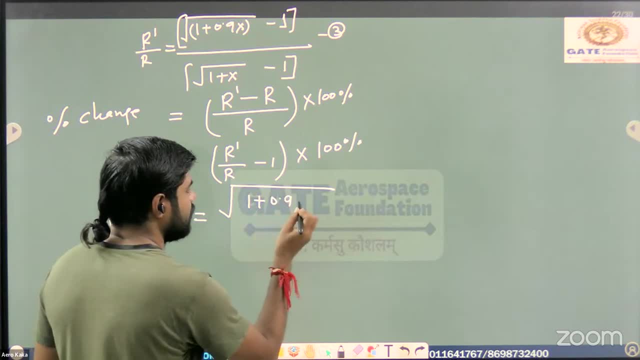 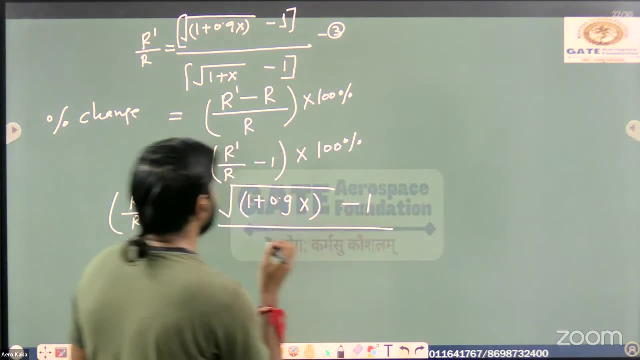 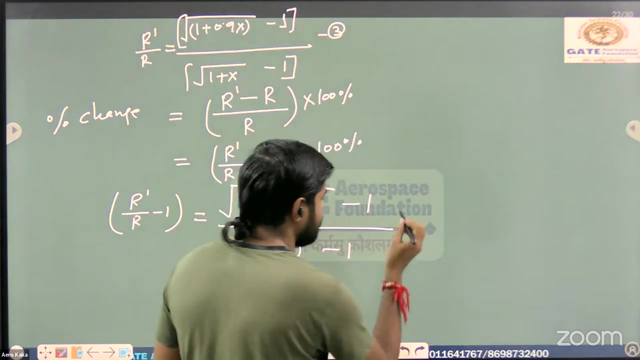 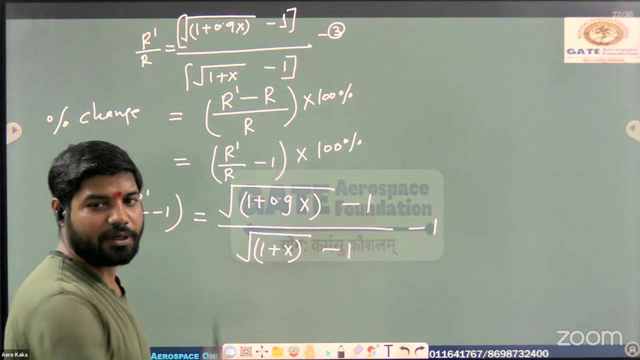 one plus 0.9 x, right? please correct me if i'm wrong. divided by root of one plus x, minus one, and then minus one here, right, check, clear. now just simplify it further. take this else here as a root of one plus x, minus one here. so we can write here: this is nothing but. 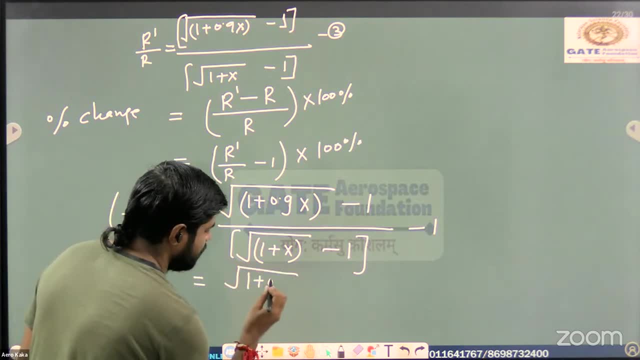 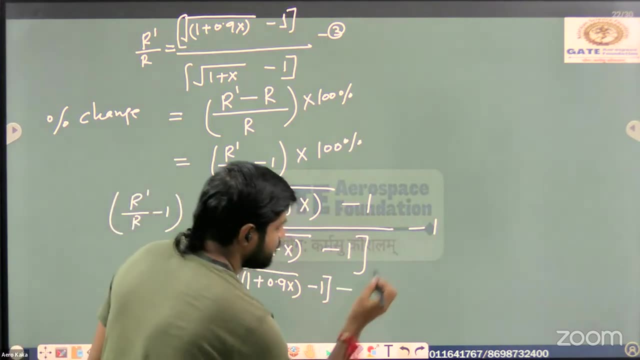 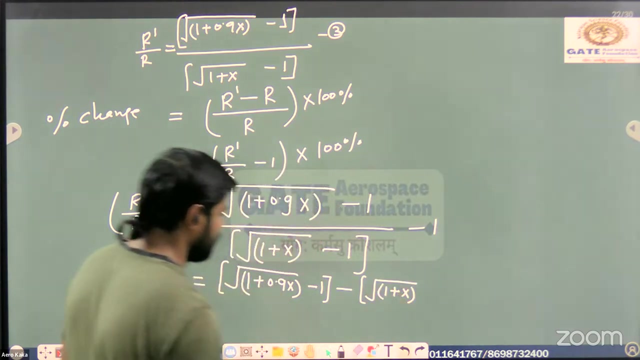 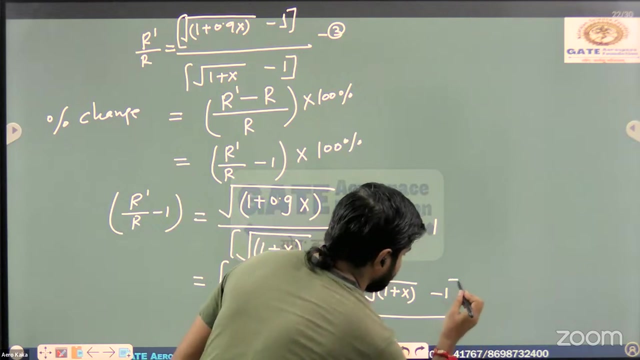 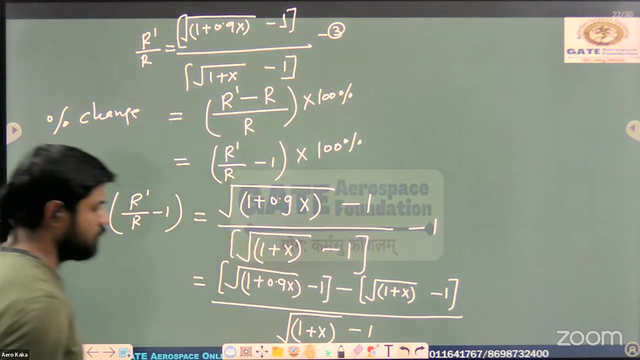 you can say root of one plus 0.9 x. okay, minus one, that minus how much. in bracket you can write root of one plus x. agree, check minus one. divide by how much root of one plus x minus one. so if you simplify it further, what we can write those: 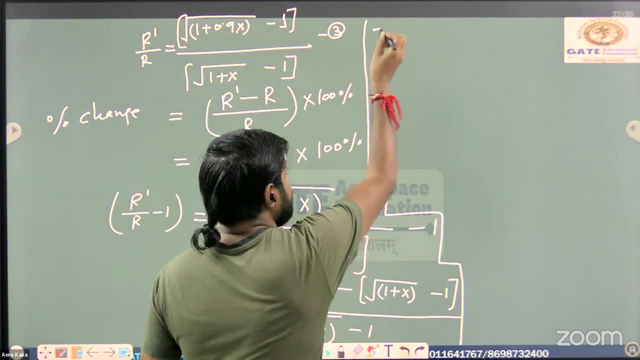 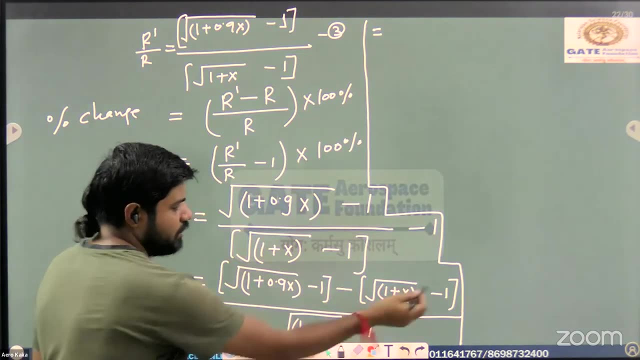 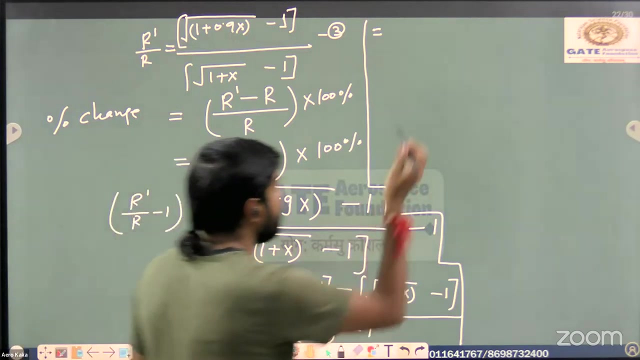 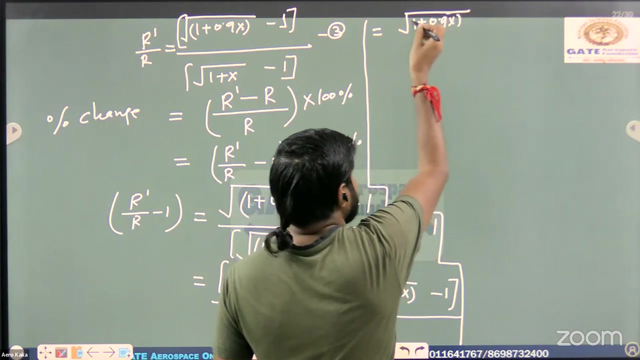 so if you simplify it further, what we can write- those now we can write this value- is equal to look. if you take, if you open this bracket, what happens? this minus becomes plus only, minus one becomes plus one only. so this one and this one is get cancelled. so ultimately, how much we'll get root of one plus 0.9 x? right, check, hello, are you getting? 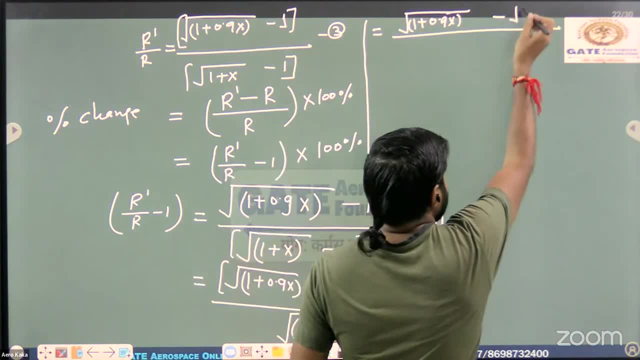 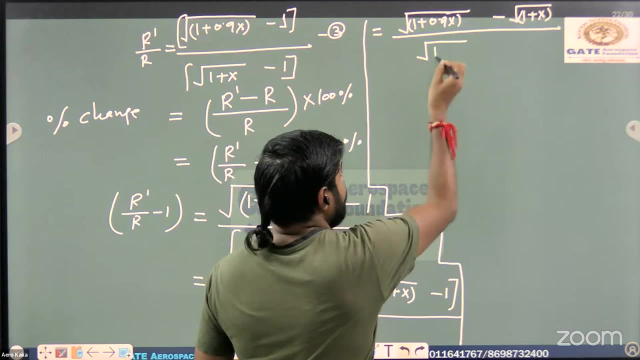 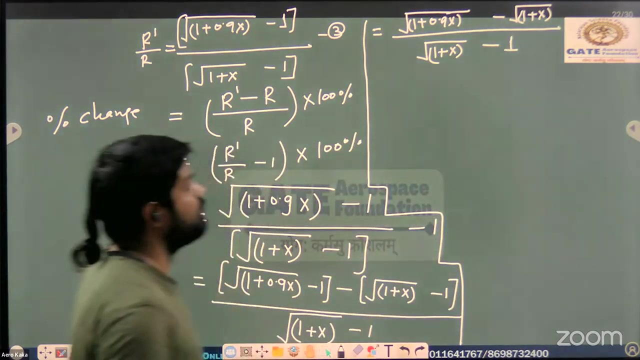 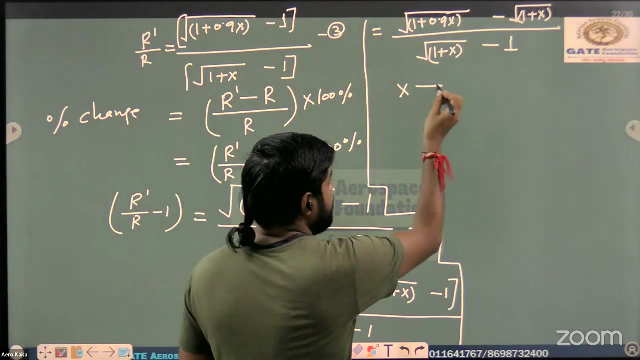 this minus how much minus root of one plus x. agree, divided by how much root of one plus x minus how much minus one, that's it. that's our final value of r prime upon r minus one. now here, what is the range of this x we can? 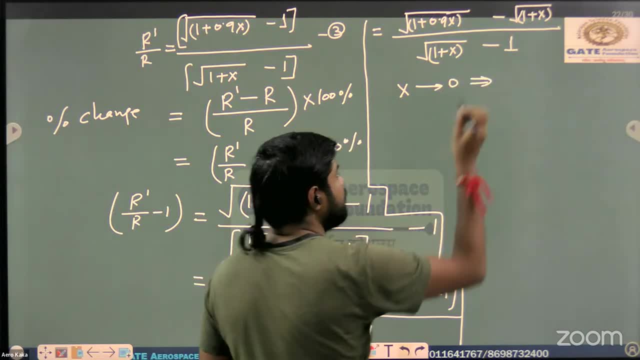 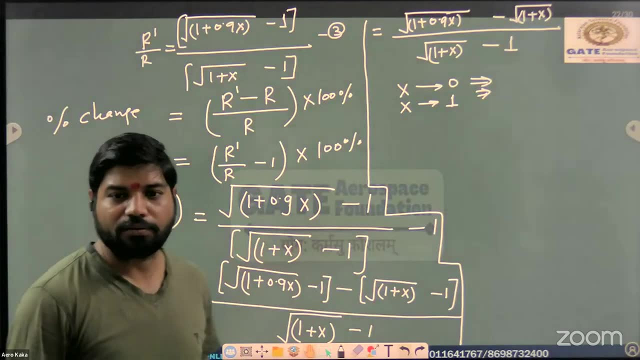 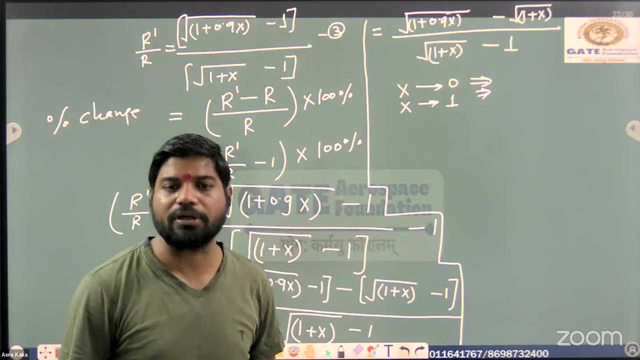 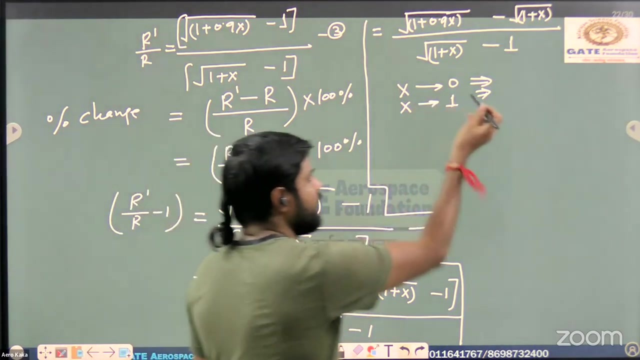 take this: x tends to zero, one of the. you can see the extreme conditions. mathematics: x tends to one. this is another. you can see the extreme conditions. this maximum minima, hello yes, mathematics. if you are weak in mathematics, it's very difficult to survive in means in engineering. okay, now take, if you are saying it's x tends to zero, it is not. 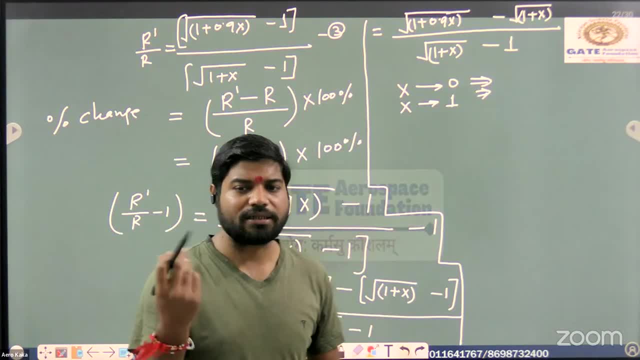 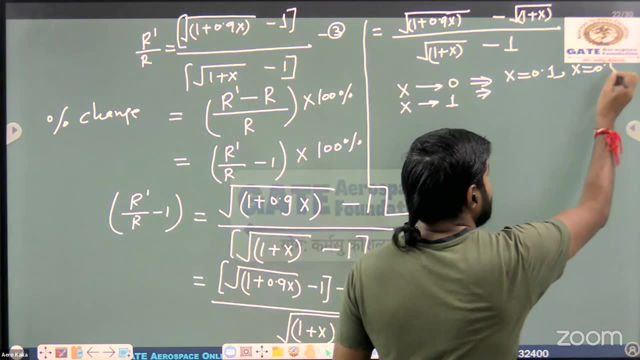 exactly equal to zero. you can say it's a nearby zero only, right. so let's consider one value: is x is equal to? let's say 0.1, then you may consider: x is equal to 0.5 and in extreme means, near to one. 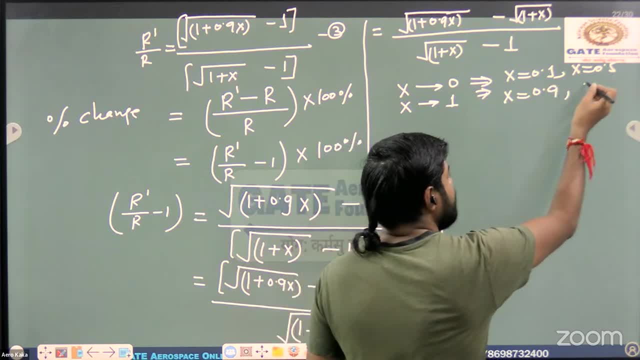 you can take x is equal to 0.5 and in extreme means near to one- you can take x is equal to 0.5. consider, let's say it's a x is equal to 0.9. even if you put x is equal to 1. let's see how much you. 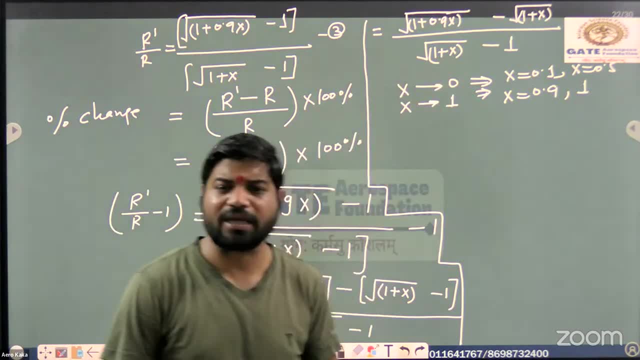 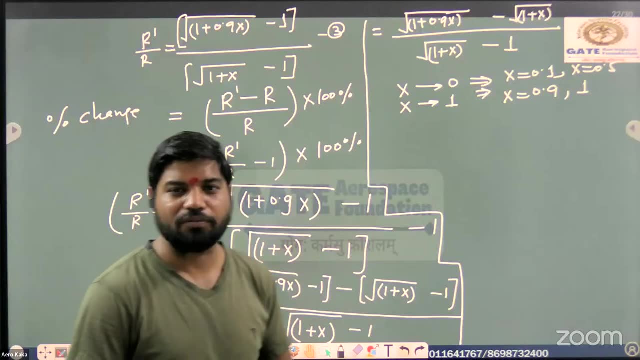 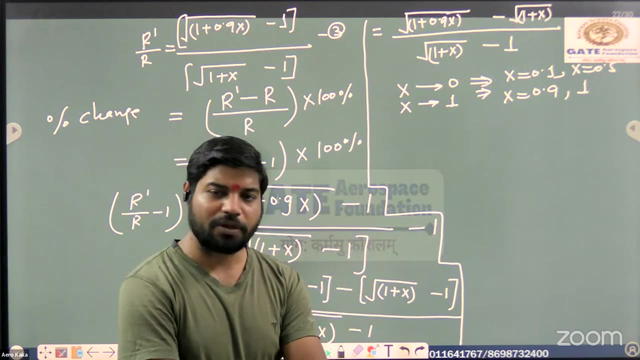 will get, but it fails exactly at: if you are putting x is equal to 0, will you get anything. you will get. it's a 0 by 0, right? which form is this? 0 by 0, what we call mathematics. what is this? 0 by 0, what we call. which form is this? 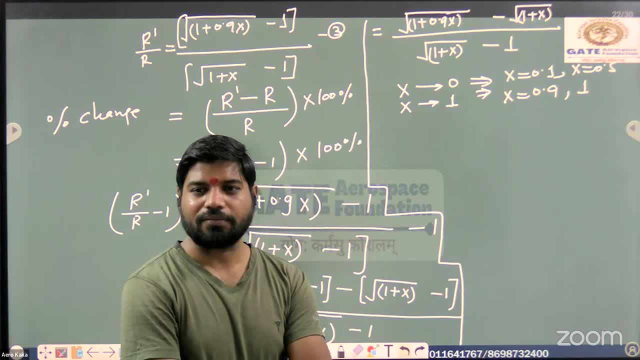 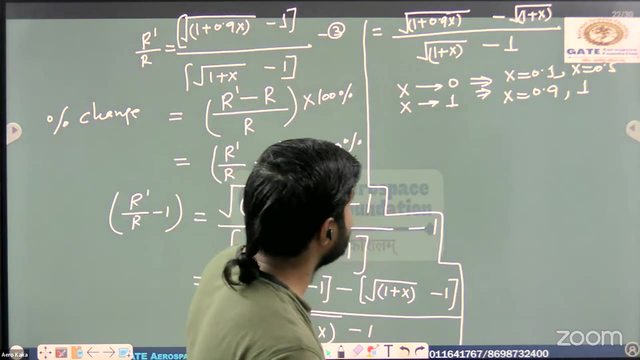 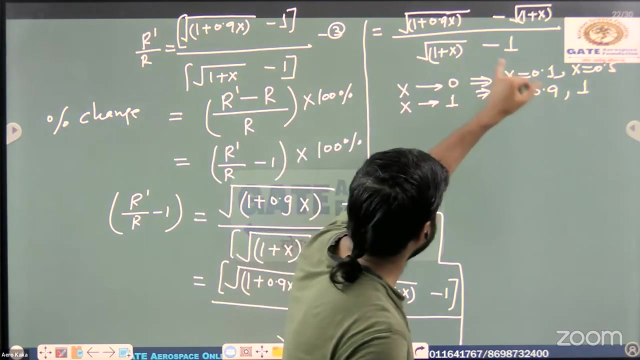 l hospital rules are used in determinate form, but it is called: yeah, very good, that's a 0 by 0 form, right? so if you are putting exactly, x is equal to 0 here. how much we'll get root of 1? here? also, it's a root of 1, so 1 minus 1 becomes 0 here. 1 plus x, right? so how much we'll get? 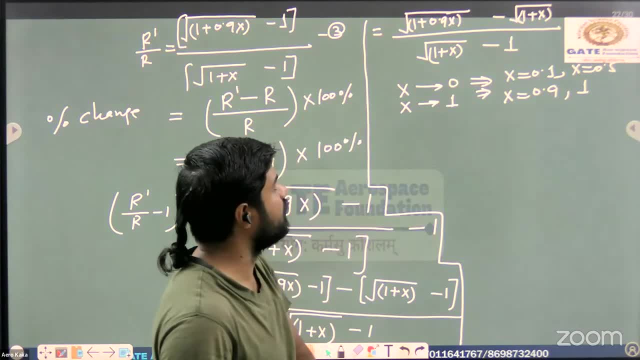 no, you will get 0, right, you are not getting here. no, no, you will get 0, only right 0 by 0. so if you are putting x is equal to 0, you are not getting here. no, no, you will get 0, only right 0 by 0. so if you are 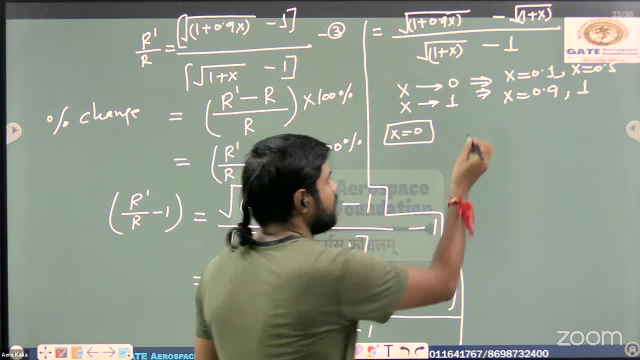 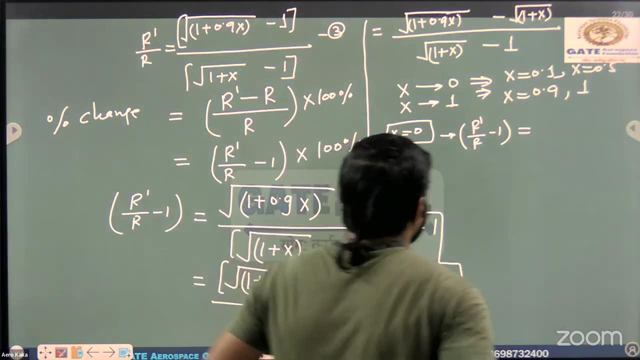 putting x is equal to 0 here what you can write this r prime upon r minus 1, u is equal to how much we are getting. tell me, 0 by 0, what you mean by x. are you going to do? what's the meaning of? 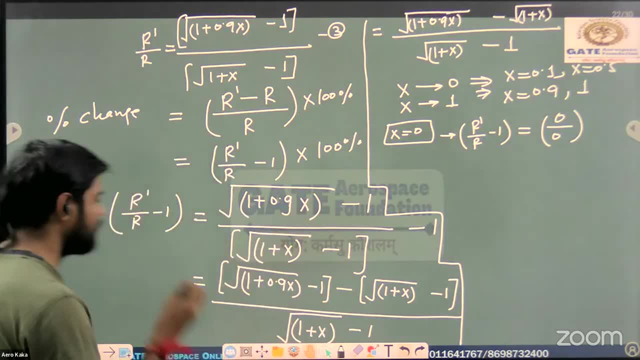 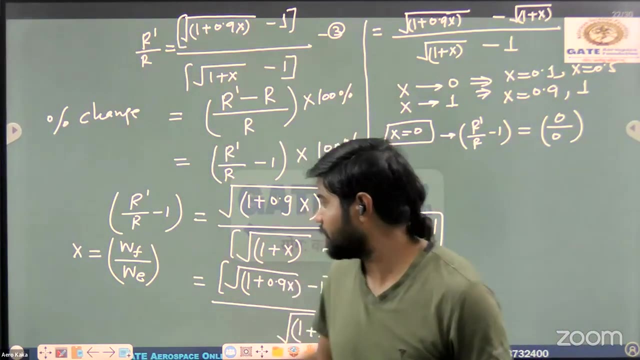 0 here. look what is x here you are taking this. x is nothing, but you can see weight of weight of fuel divided by how much w e. hello, just try to relate it. error in error not. or aerospace engineer right. so if suppose this is the you can see this x can be zero. if suppose 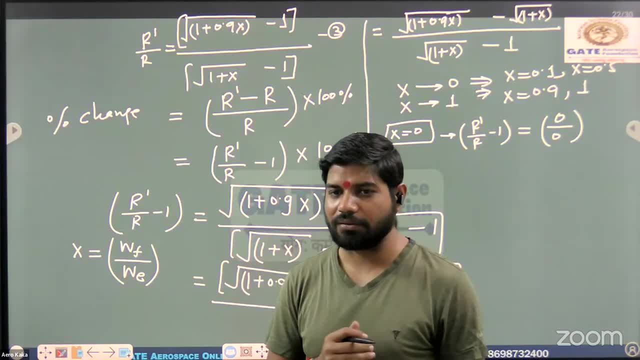 the weight of the fuel carried by this aircraft is zero, right? or if suppose the value of we is how much infinity? am i at all audible or not? so these are the hypothetical situations. is that clear? can you fly aircraft if suppose it is not carrying the the fuel? don't say that it's. 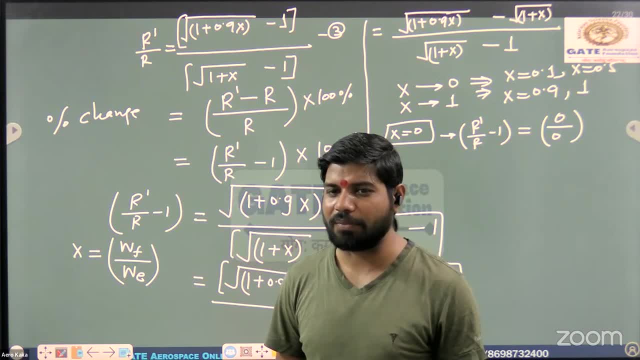 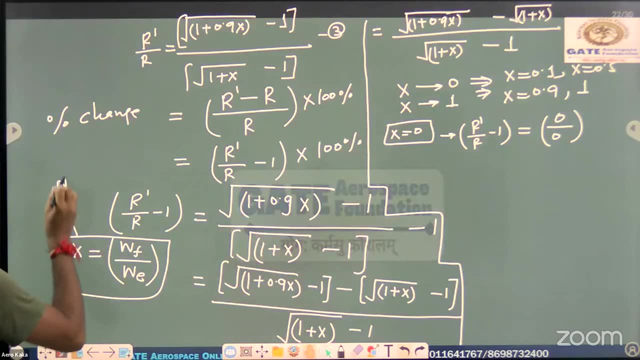 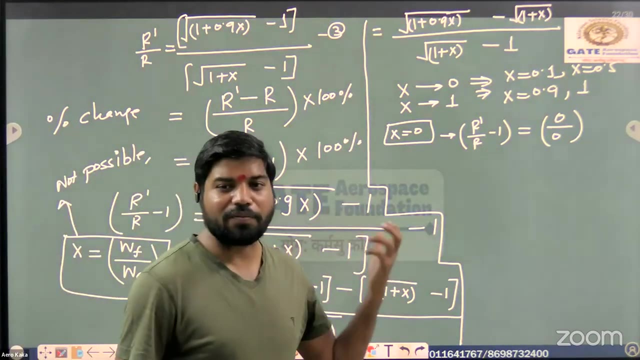 electric, or you can say solar kind of it, okay, or rc plane. am i audible or not? so this situation is not possible. this is not possible. but let's say: can we have some value? if you are putting near to this zero, let's say 0.1, okay, consider t is 1. 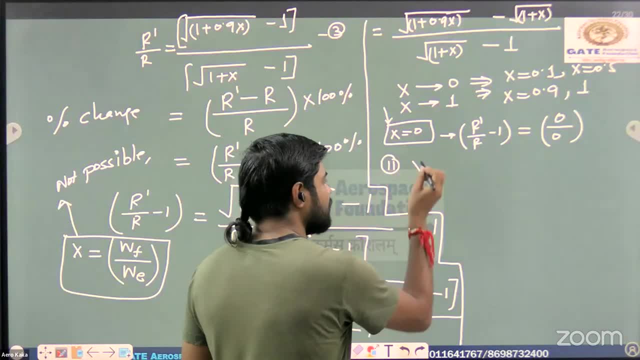 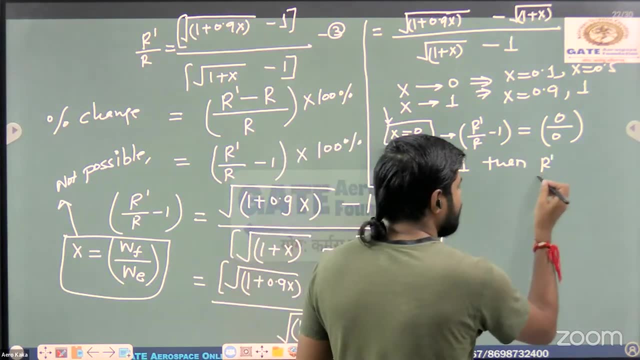 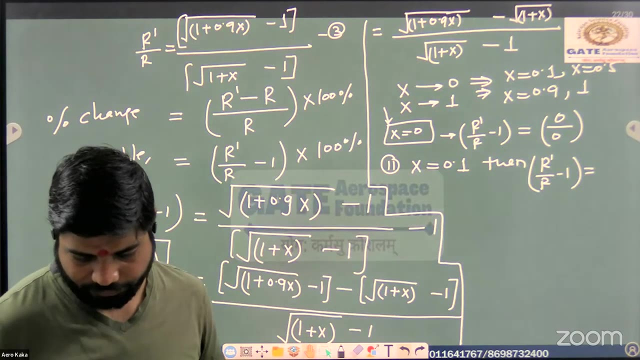 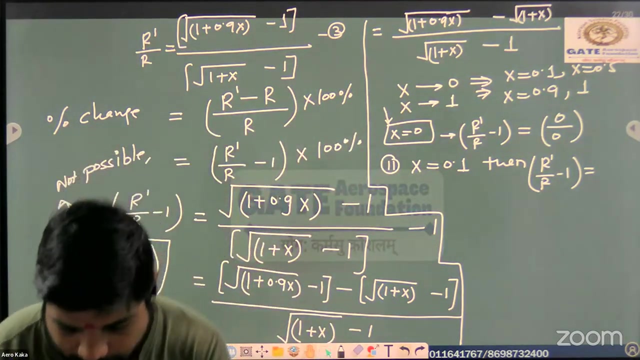 okay, so you can see. this is the hypothetical case case to here. if suppose this x is equal to 0.1, then can you tell me what's the value of this r prime upon r minus 1, how much you are getting? yes, anyone put here: x is equal to 0.1, so it is how much root of 1.09? that means, let me check. 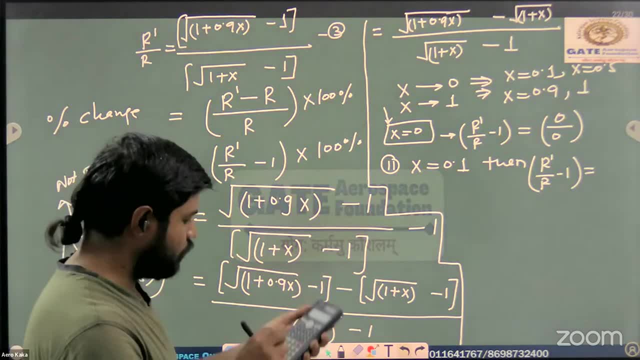 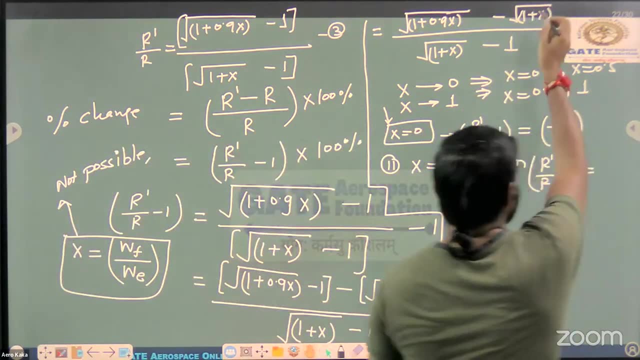 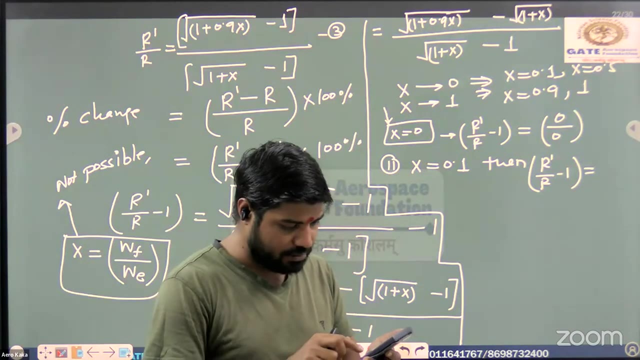 here is the calculator, so you will get root of 1.09, right minus. if you are putting x is equal to 0.1. so what you will get, root of 1.1, 1 plus 0.1, is how much 1.1, only so minus root of 1.1 divided by root of 1 plus x. what is the root of 1 plus x here? 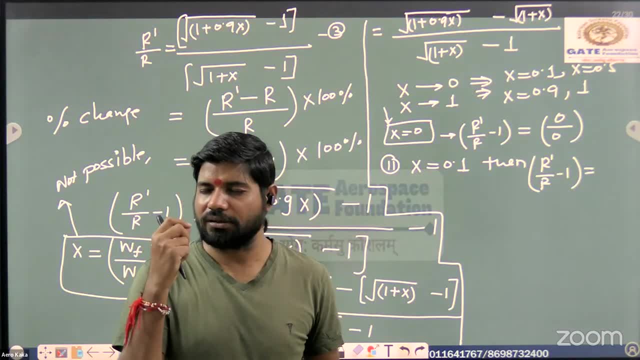 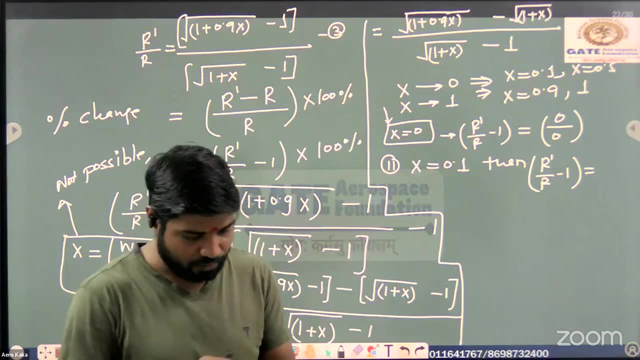 x. you are considering it's the 0.1. sorry, it's a, it's a, yeah, 0.1. so how much we'll get root of 1.1 and then minus 1 here. so, root of 1.1 minus 1, how much we are getting? 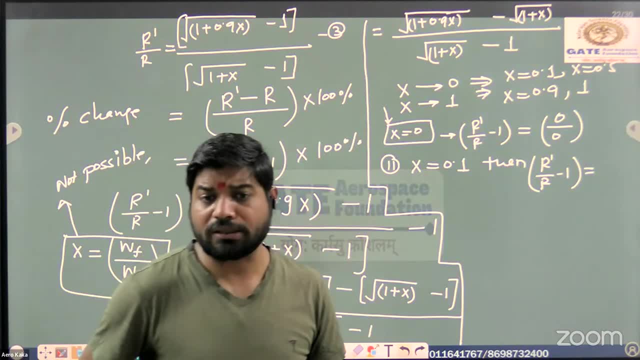 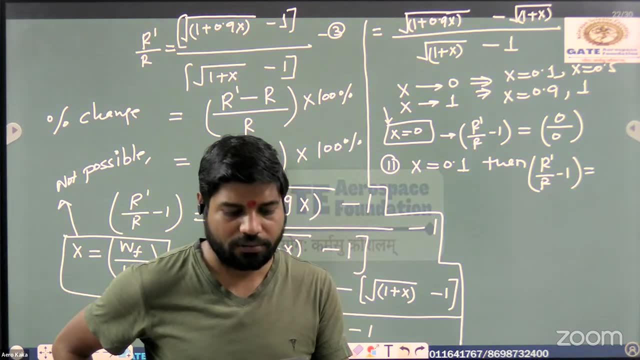 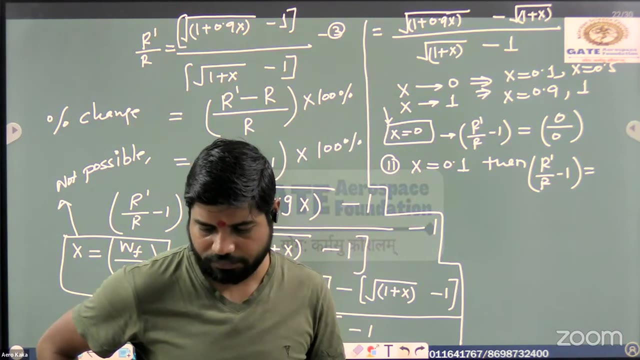 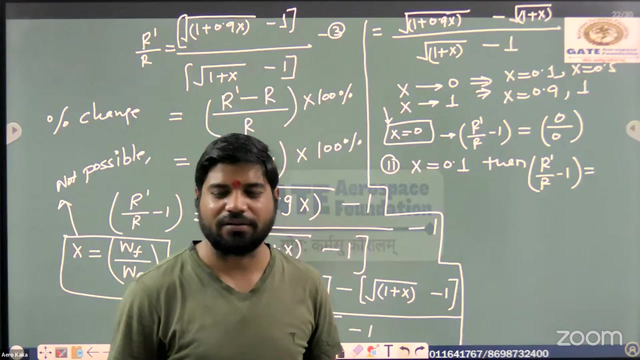 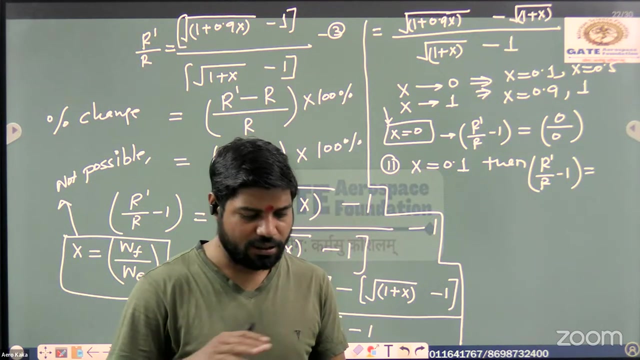 are you getting around? minus 0.0978 something? please verify. so minus 0.0987, i'm getting 0.0978 something, or please verify? okay, take your time. minus 0.0833, so it is coming. minus 0.097896, come again 0.097896. i'm getting very near value which you are saying. 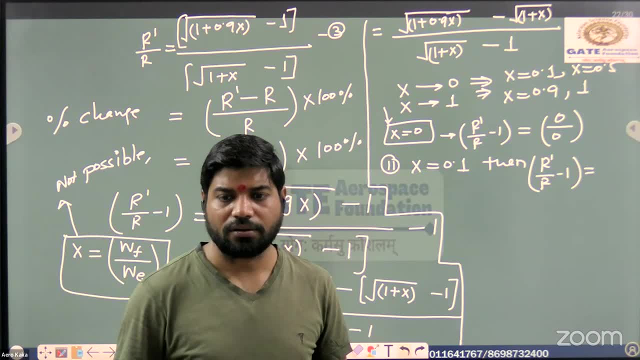 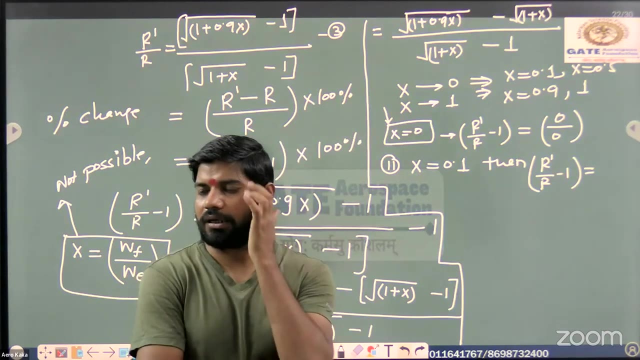 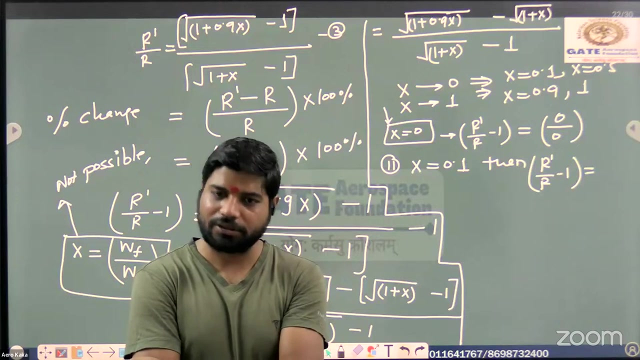 yes, any other student tell me up to the four decimal places, at least up to four decimal places. error 眼? oh yes, how much you are getting gradient 0.tech confidence. why is it finding me now and not having to speak somewhere? big irgendTurke. 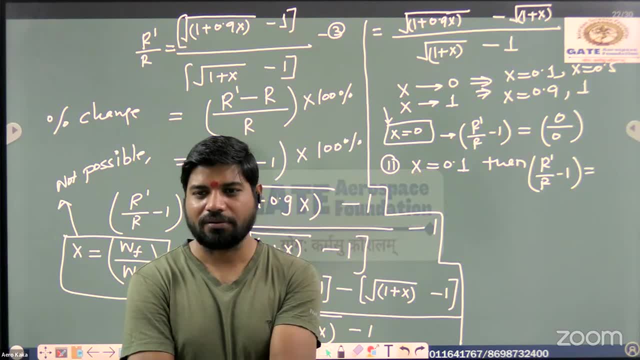 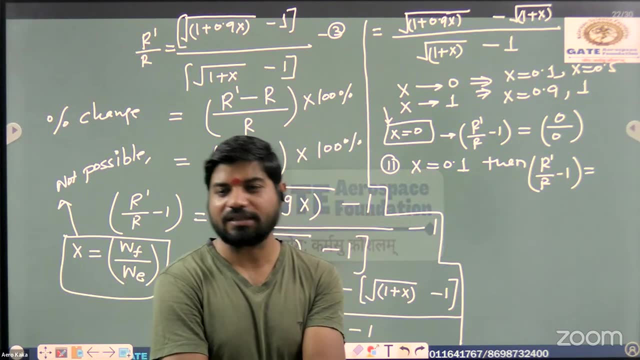 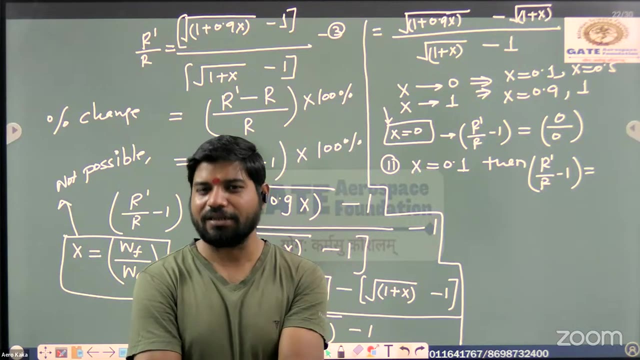 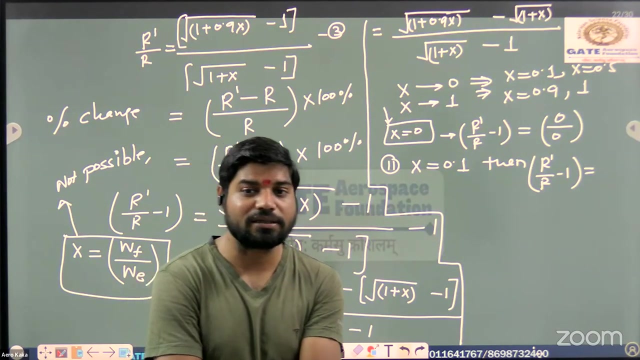 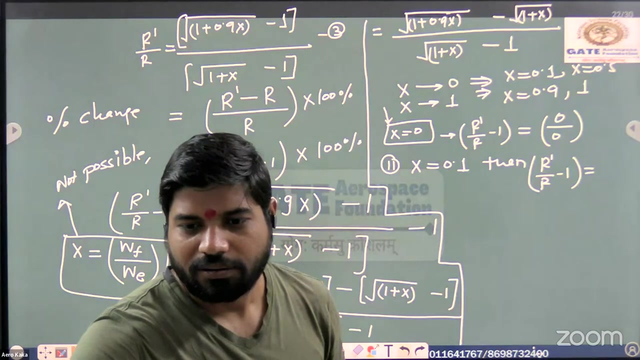 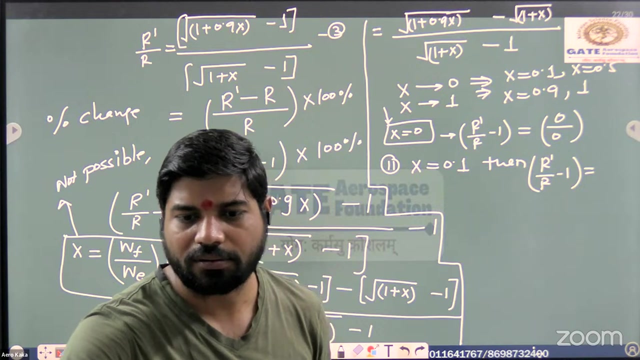 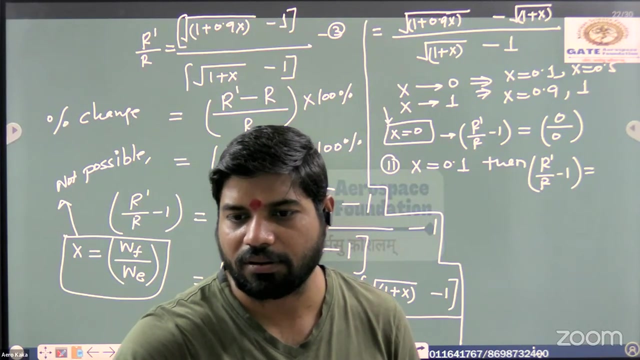 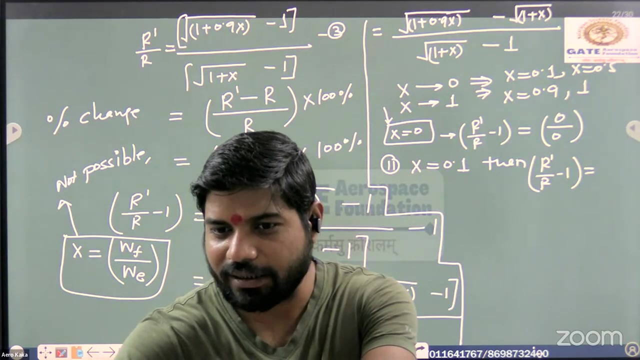 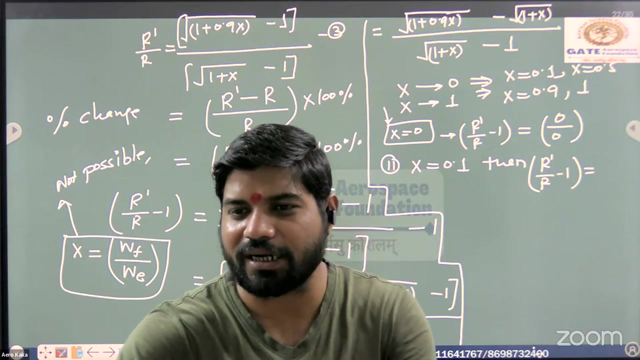 Is it making sense now, friend? yes, how much you're getting? oh my god, yes, yes, hello, how much you are getting? hello, am i audible? who's there? who's that? mansoori, are you there? how much you're getting? ishika shavan, how much you're getting? am i audible to you or not? first, first, let me know. hello, am i audible? 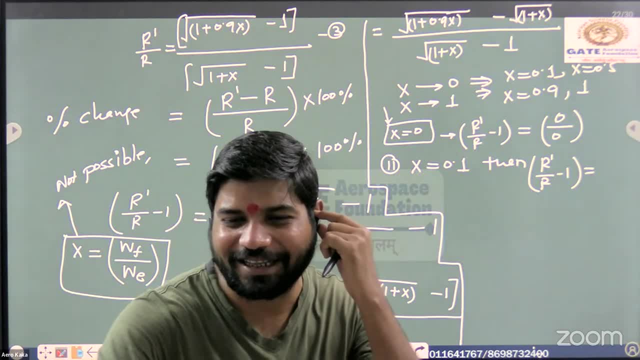 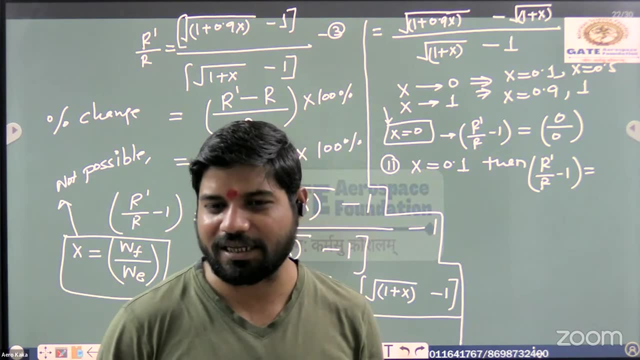 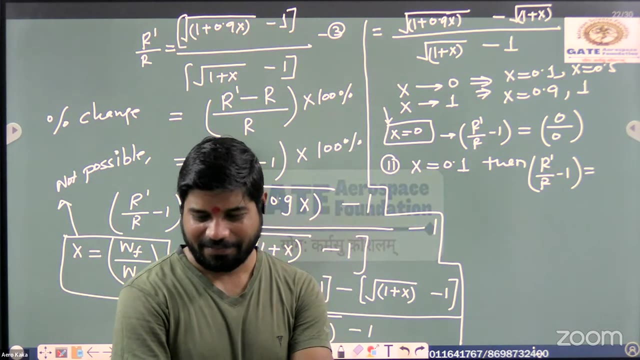 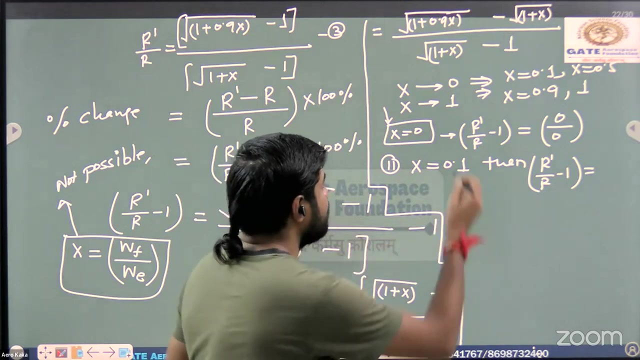 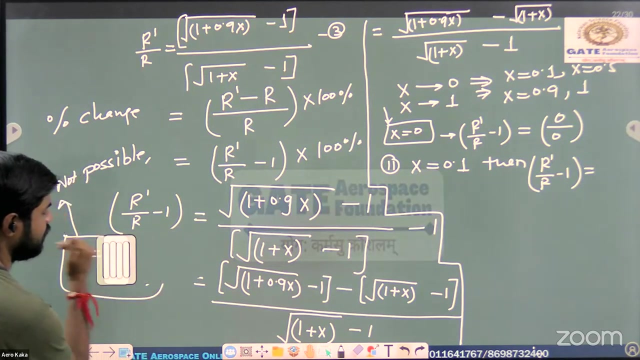 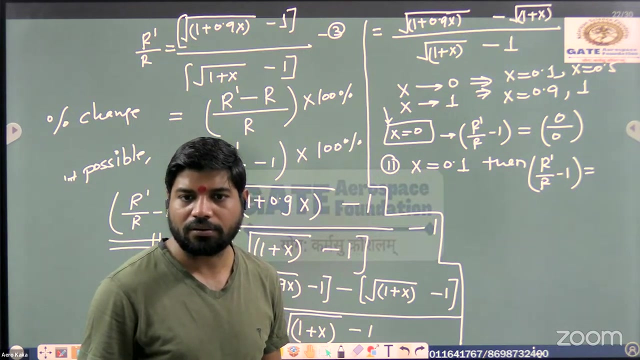 hello, am i audible? yes, sir, sorry, come again. i'm seeing. what is this? tell me, hello. what are you saying? r prime by r minus one or r prime by r only? what is this? hello? so tell me this value only minus 1.0833, really. so by taking x, 0.1, x is equal to 0.1. if you are taking x equal to 0.1, 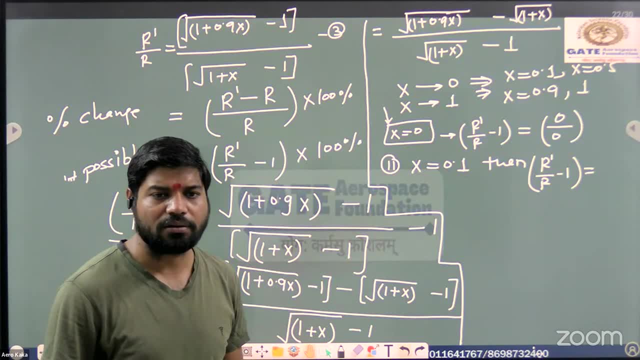 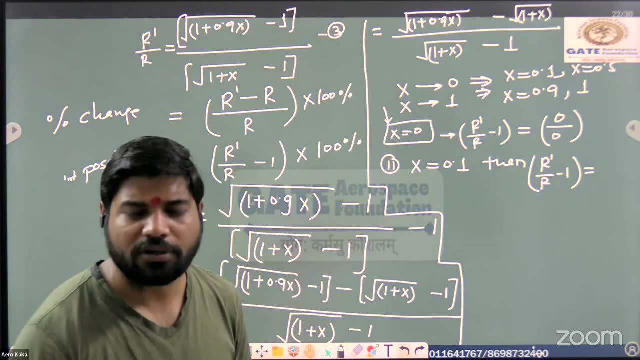 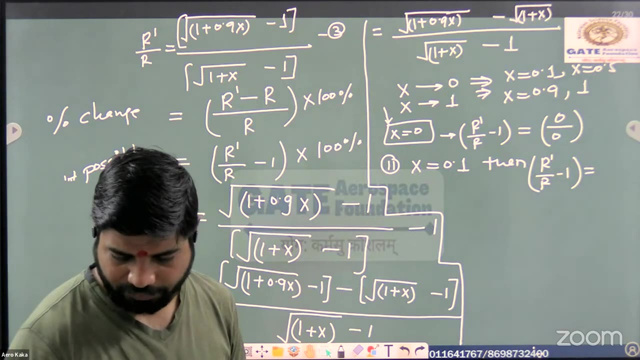 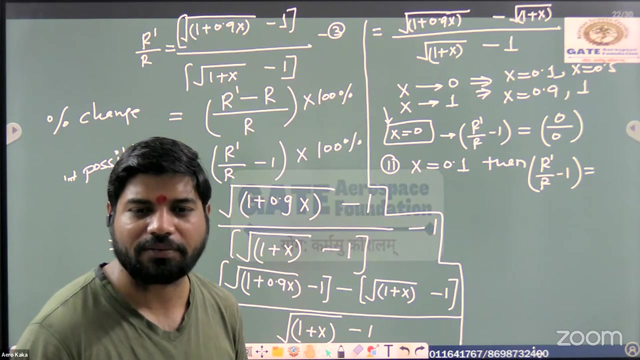 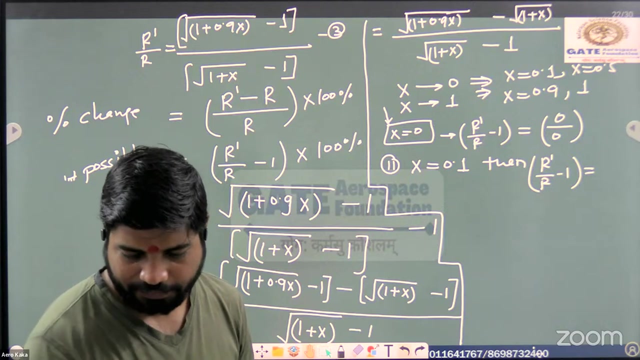 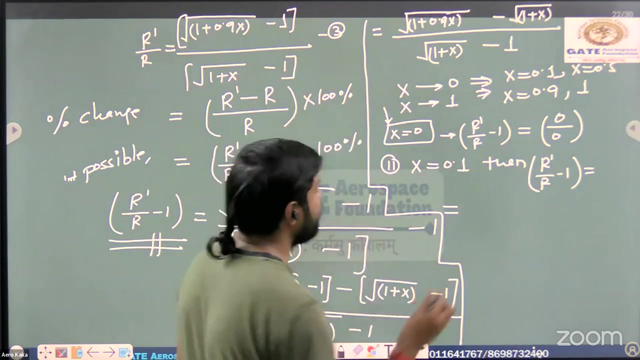 then how much? how much? you are getting minus 1.0833, are you sure? yes, sir, what about other students? so it is coming minus 0.097896. yes, any other student? hello, let me saw. if you're putting x is equal to 0.1. 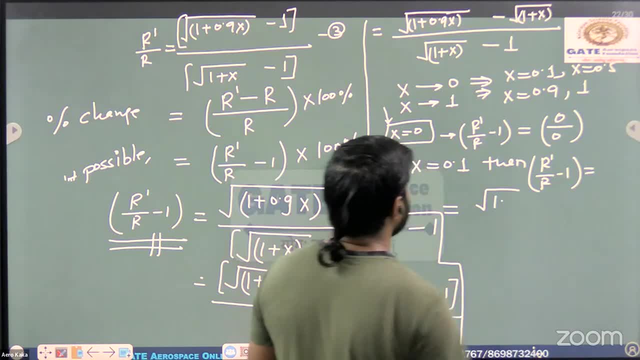 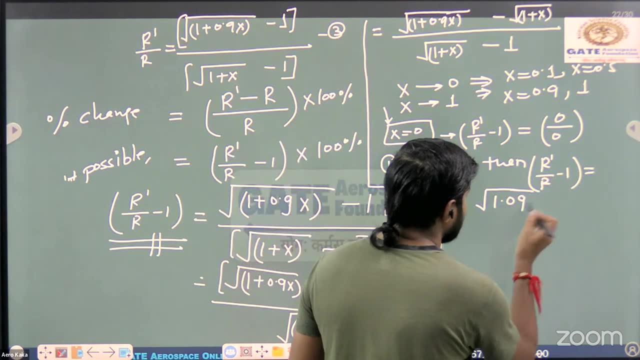 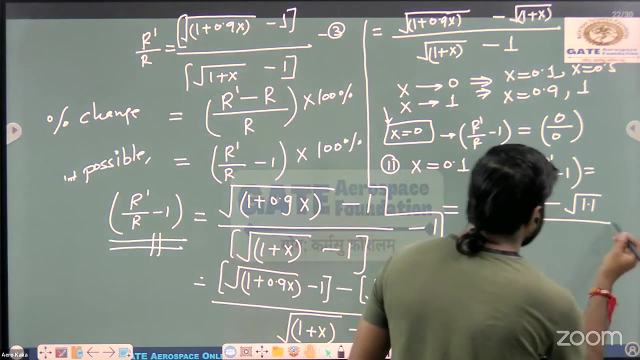 please verify how much we'll get root of one point. how much 0.9 into 0.1. how much you'll get 1.09. check please, hello- minus root of how much: 1.1. please verify. if i'm wrong, please let me know first. 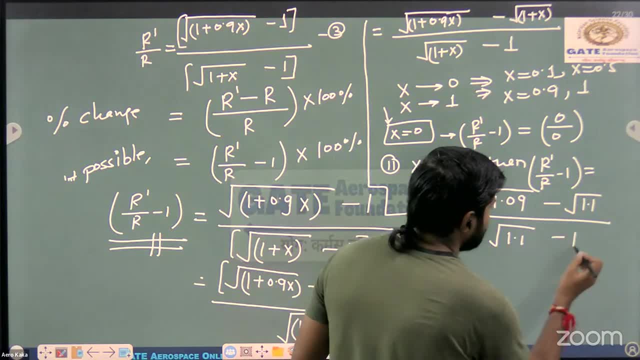 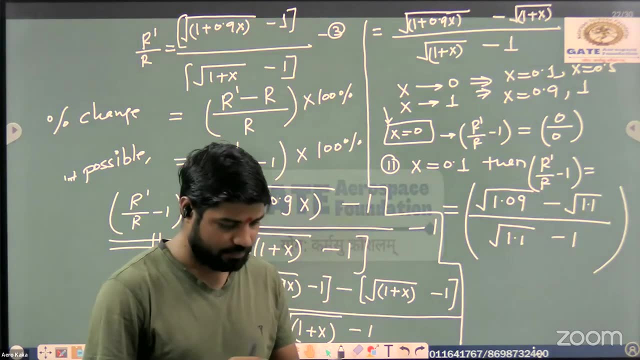 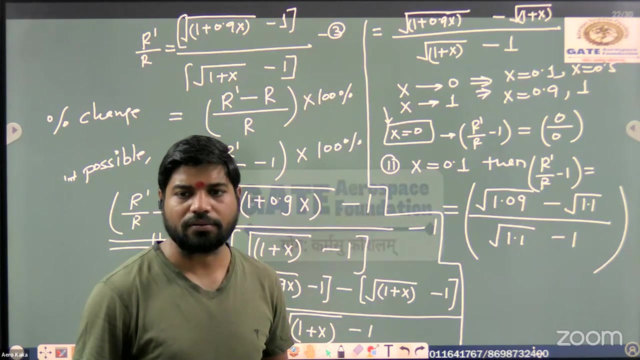 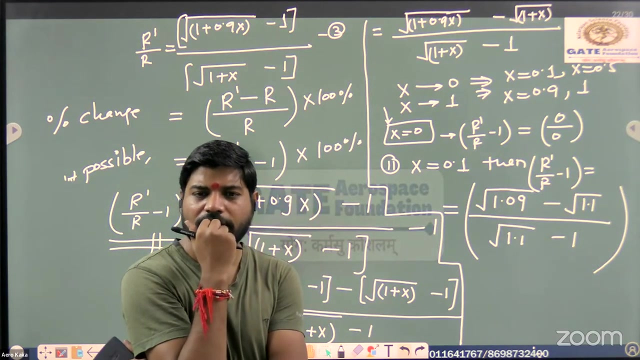 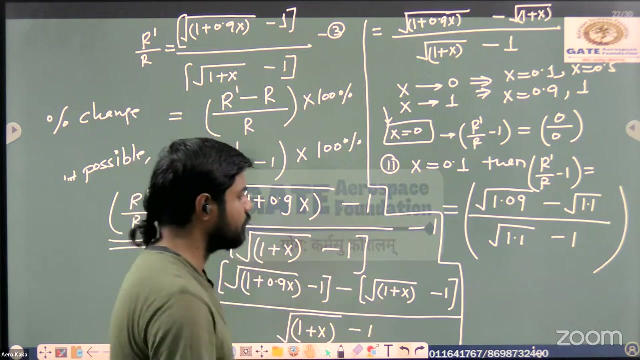 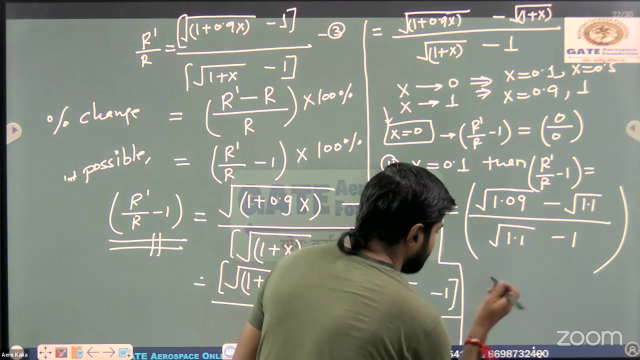 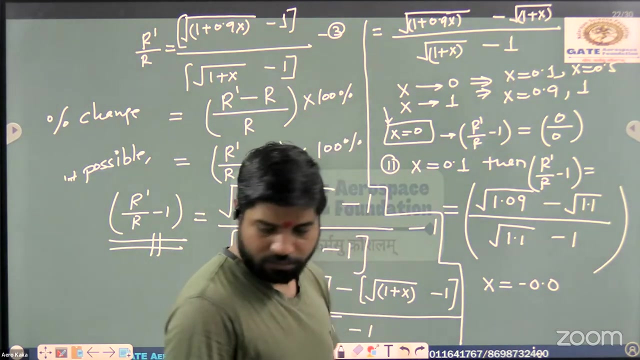 yes, sir, 1.1 minus 1 0.083- please verify, sir- minus 0.09789. yes, sir, yes, sir, minus 0.09789. so you guys missed this calculation. yes, sir, okay, i'm getting this value. x is equal to sorry, x is equal to minus 0.08732. are you getting? 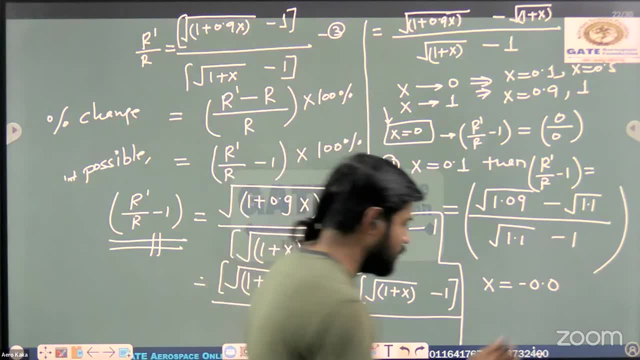 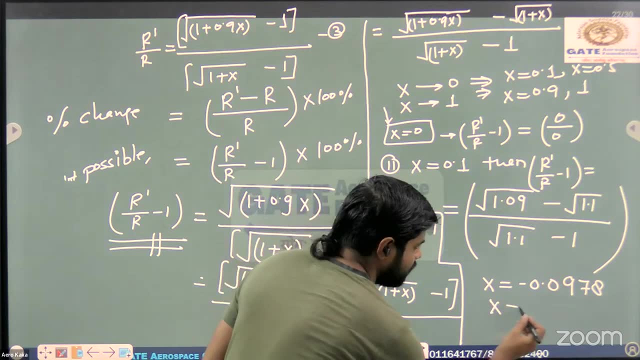 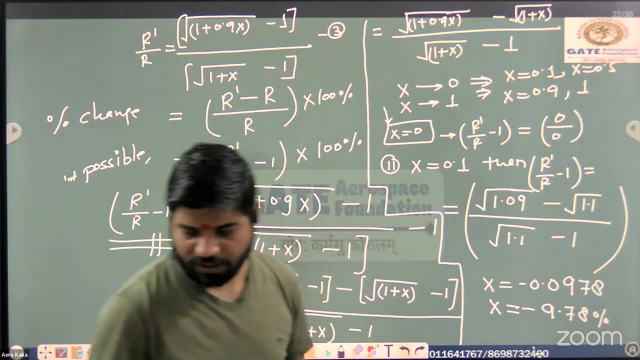 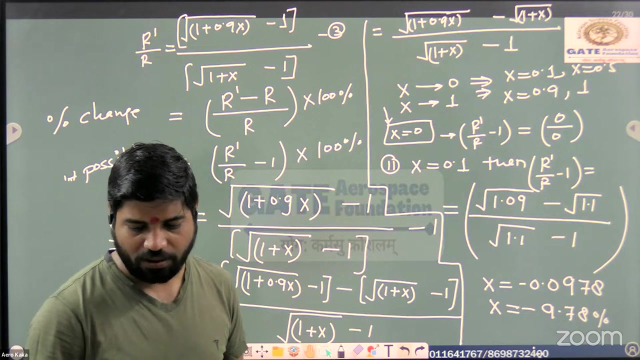 sorry, 0.0978 i'm getting. are you getting this one or not? yes, sir, so if you take this in percentage, then how much you will get minus 9.78 percent? are you getting this value? please verify. we put: x is equal to 0.1 here. are you getting? yes, sir? okay, suppose, take another. 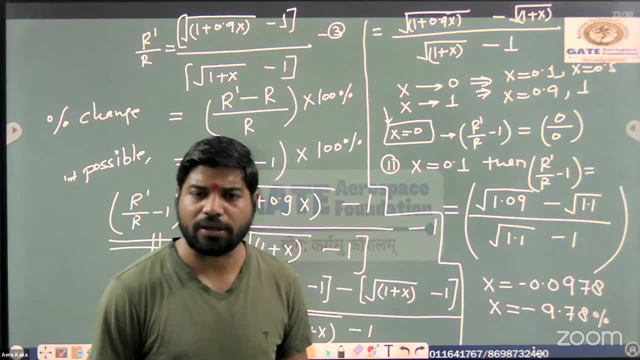 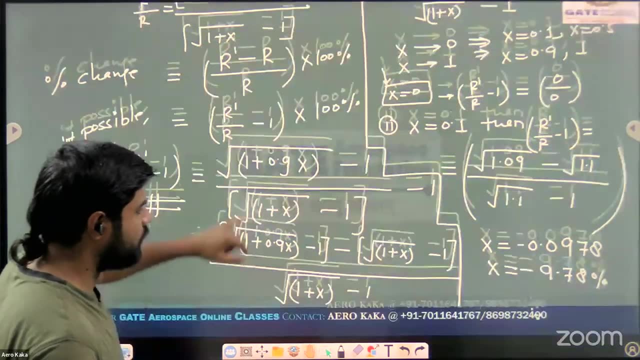 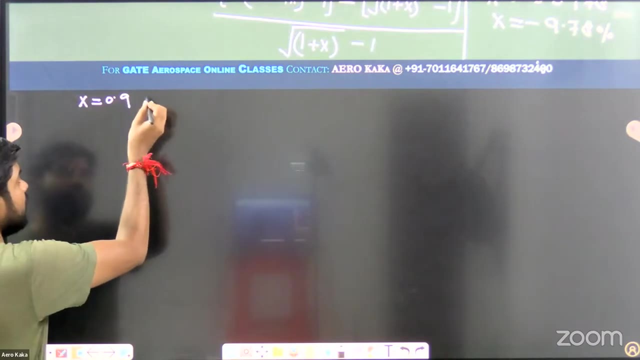 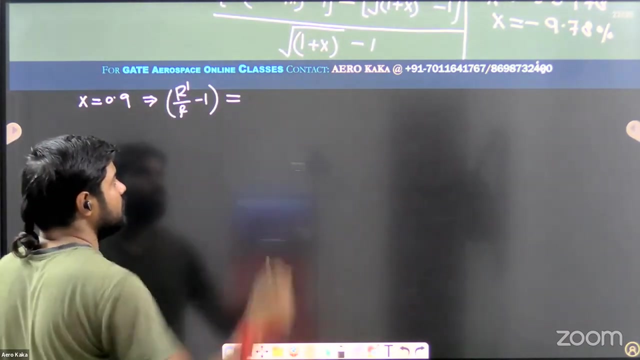 value. let's consider x is equal to 0.9, hypothetically. okay. consider other value: x is equal to 0.9. just wait, okay. you even then consider x is equal to 0.9 here. then what is this r prime upon r-1? how? 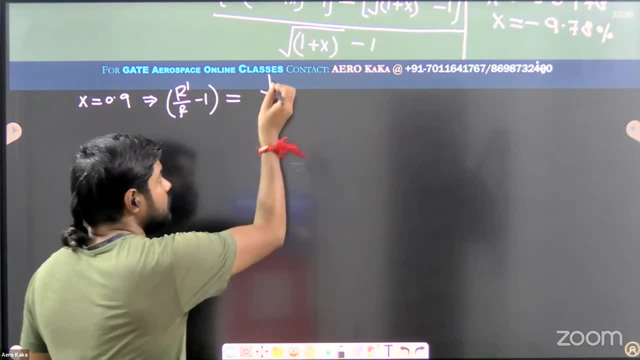 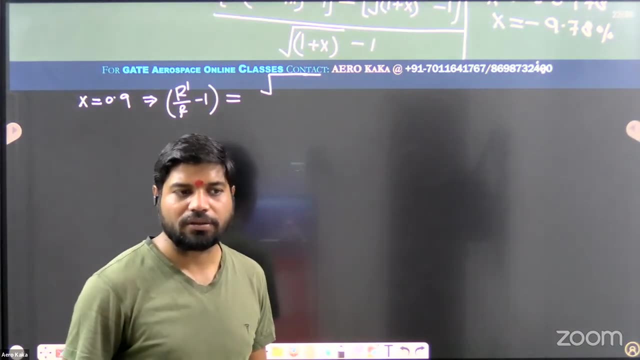 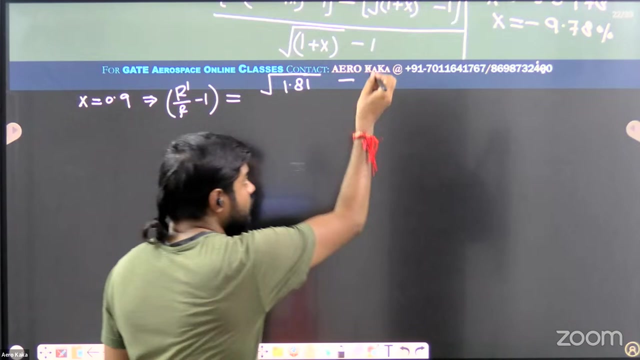 much. we'll get root of 1 plus 0.9 x, right? so how much? we'll get root of 1.81, something nine, nine, is that eighty one? so how much? yes, sir, one point eight, one, minus root of one plus ten, plus three point fast point slash one, so it is less than 1, where is that? 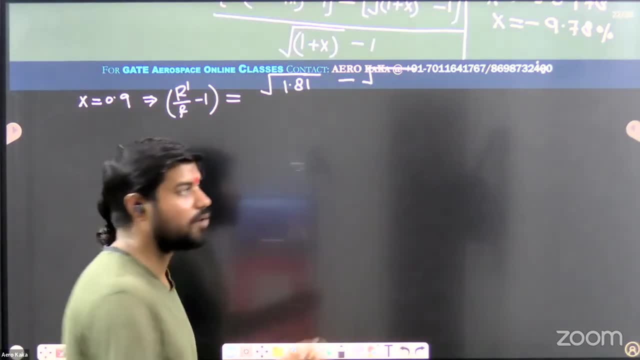 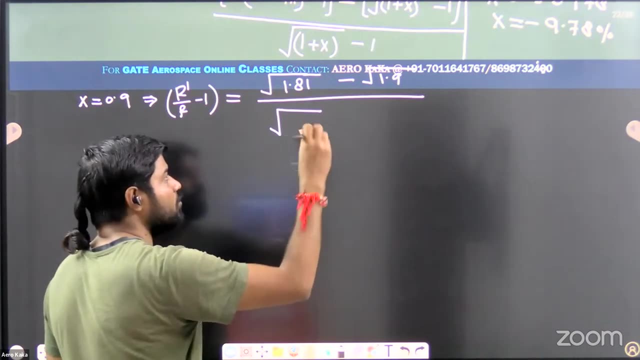 x, right? so what do you mean by x here? x is 0.9, so how much it is 1.9 divided by how much? root of 1 plus x. so x is equal to 0.9, so root of 1.9 minus 1. just simplify it and let me know. 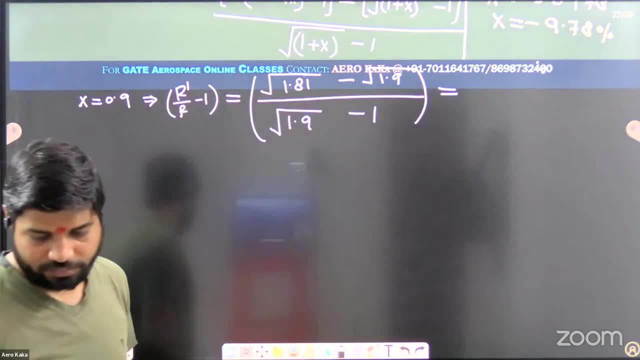 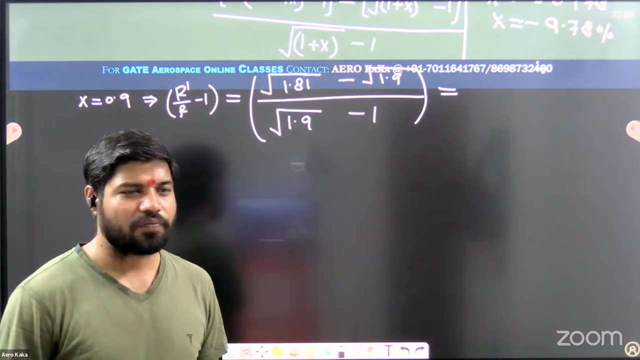 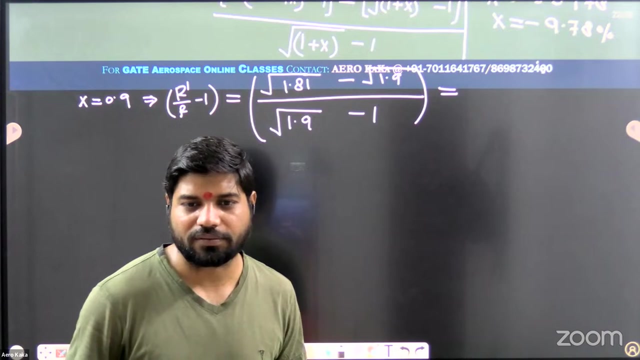 how much you're getting. please take care of your calculations. at least you are going to lose five to ten marks if you will make calculation the way you are doing in this class. so please take care. having the knowledge is not enough practice. how much you're getting? 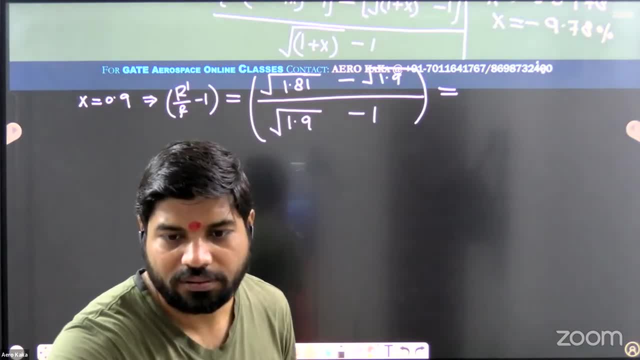 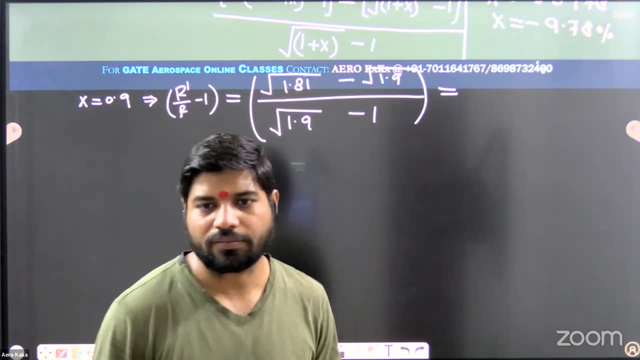 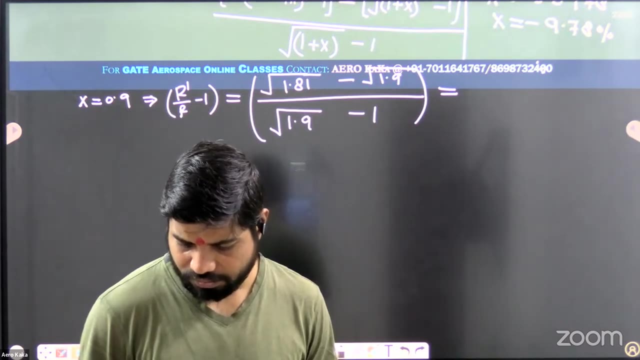 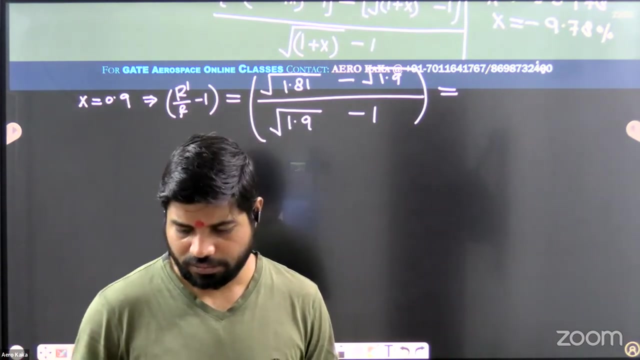 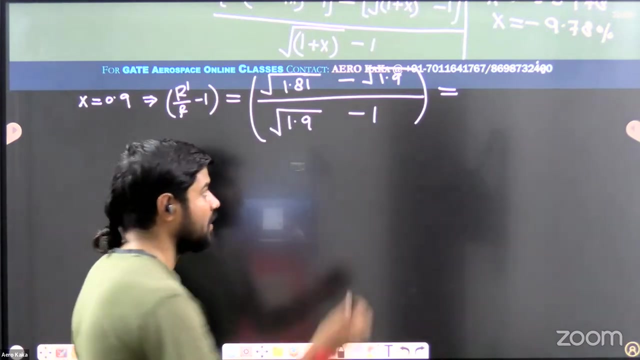 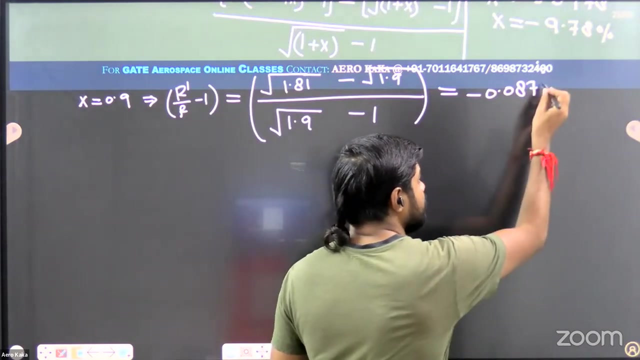 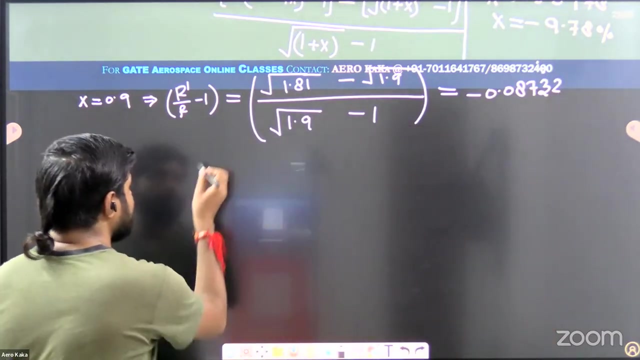 so it is coming minus 0.08732, 041. how you are getting? minus 0.09715, yes. minus 0.087320412, yes. so minus 0.08732, 0404, 0404, 0413, 0413. okay, so if you want to take the percentage, so what you can do it's a r prime upon r minus 1 into 100. 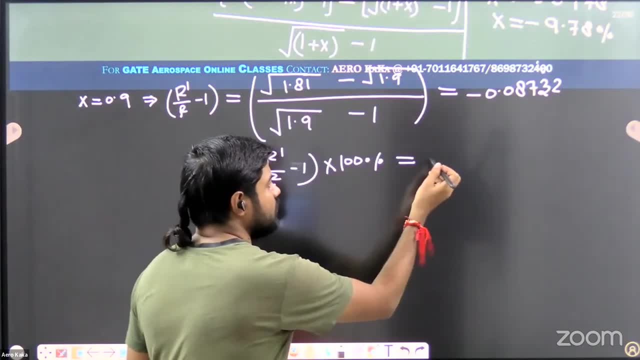 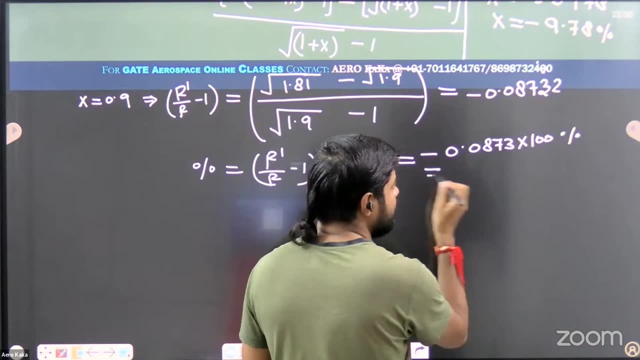 percent, only right check. so it becomes: how much minus 0.08732, right in 200 percent, how much will get up? eight point seven, eight points. negative sign of meaning. but even if you, if you will say, how much will you get? okay, so many percent. 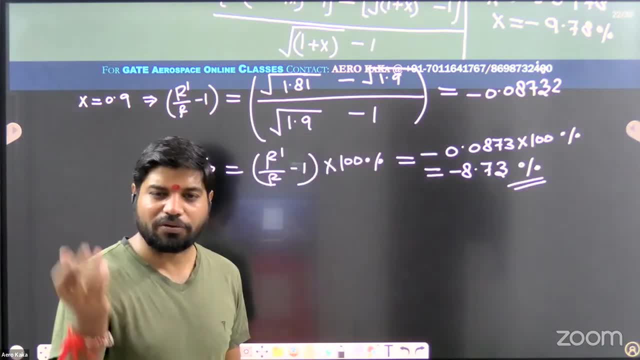 0.08732, 0.08732. right check so it becomes: how much minus 0.08732 right into hundred percent, how much will you get? If you take x is equal to 1, okay, another case, it's a case number 3, right. 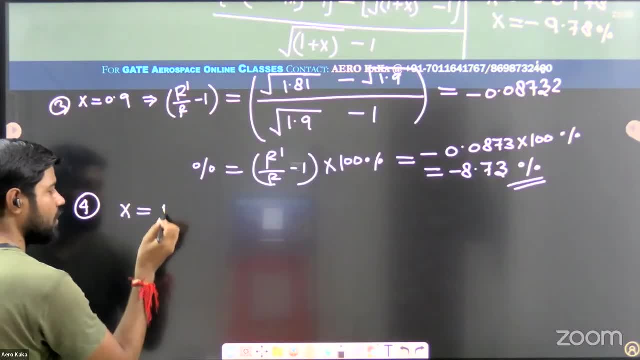 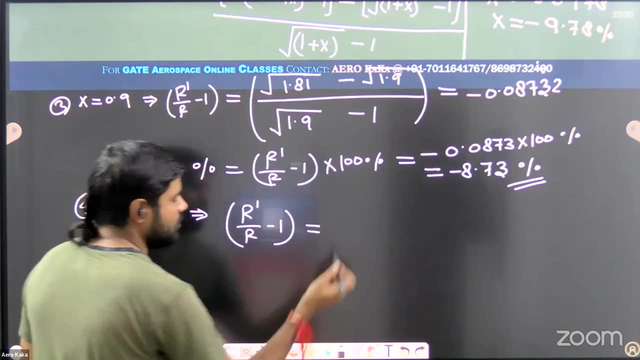 Another case you can consider. let's say x is equal to 1 here, Then how much we will get this value, r prime upon r minus 1? Root of 1 plus 0.9x. so how much we will get. 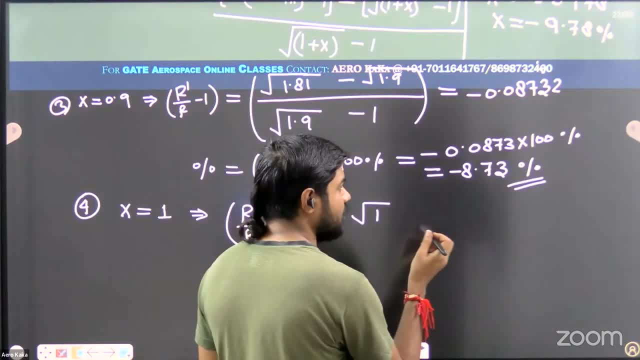 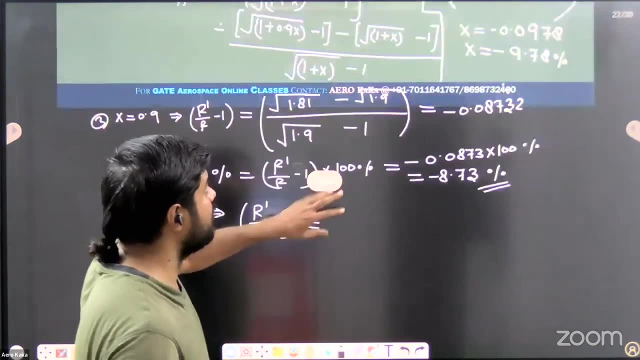 Root of 1,. is that clear? Hello, if I am putting, x is equal to 1, right? So what is the final form of this equation? Let me check: root of 1 plus 0.9x, right? 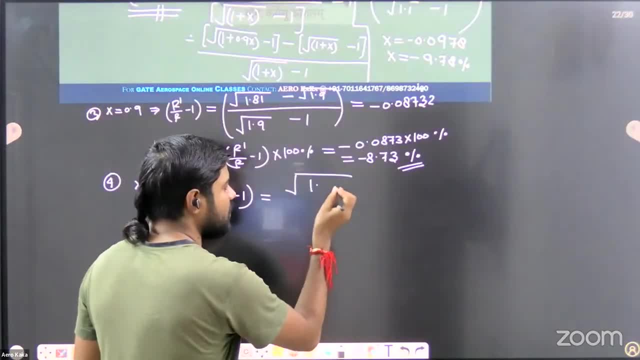 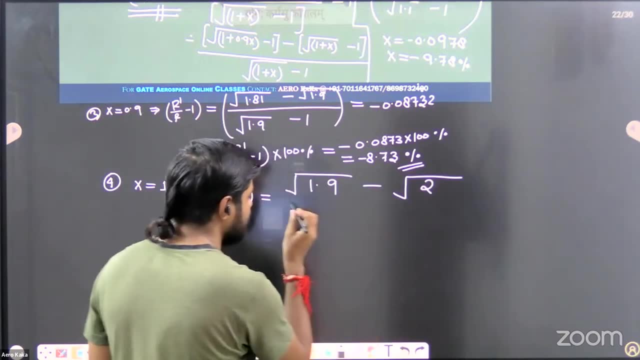 So it becomes root of 1.9,. check please: minus root of how much 1 plus x. so x here is 1, so it becomes root 2, divided by how much Root of yes, please, how much we will get. 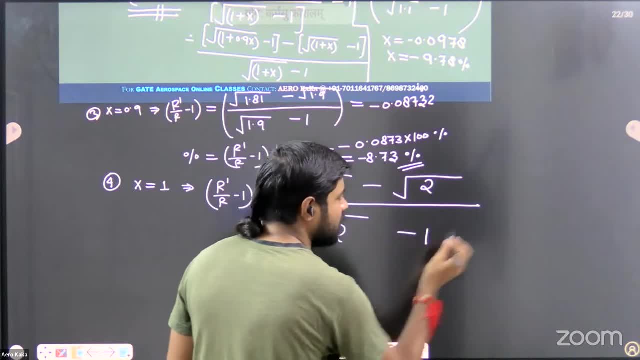 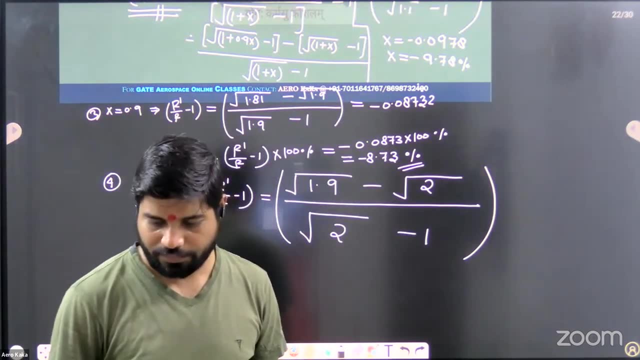 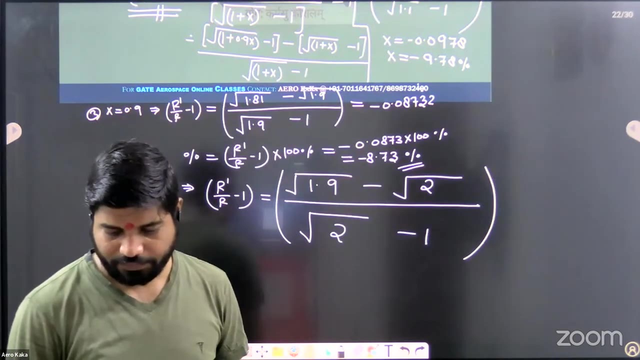 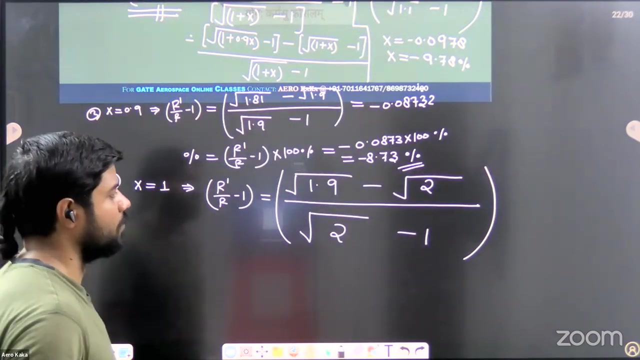 1 plus x. x is 1, root 2 minus 1.. Are you getting any value? Yes, how much we will get? Yes, how much we will get. So minus 0.086494413.. Come again, what is that minus 0.. 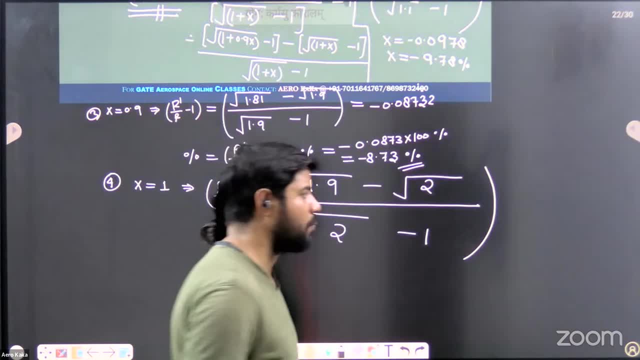 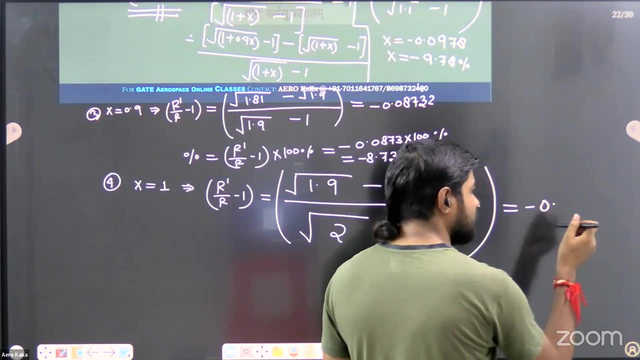 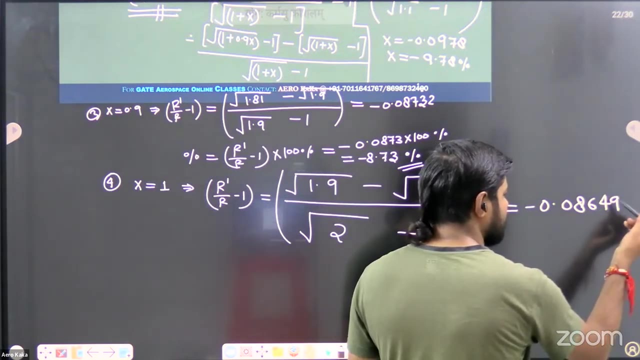 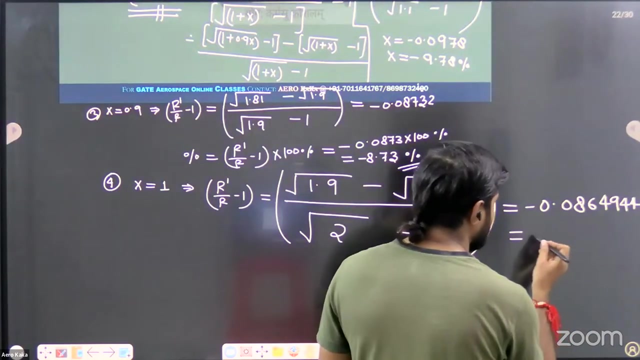 086494413.. Minus 0.. Yes, please. 086.. 086.. 49. 49. 4413.. 4413,. okay, So if you want to write up to, you can see the 4 decimal points so you can write 0.0865. 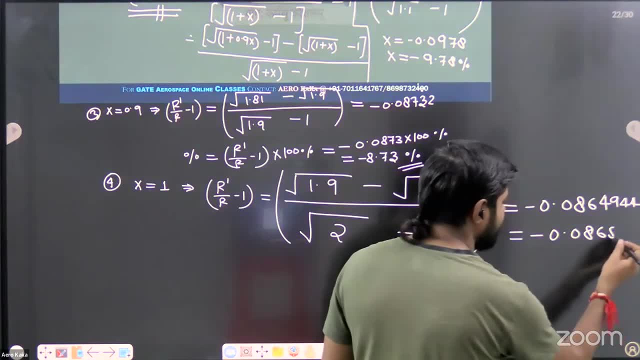 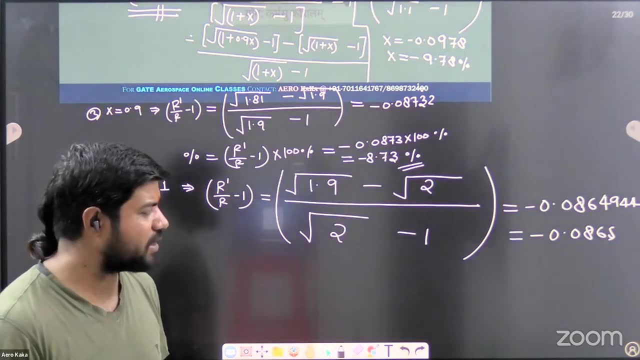 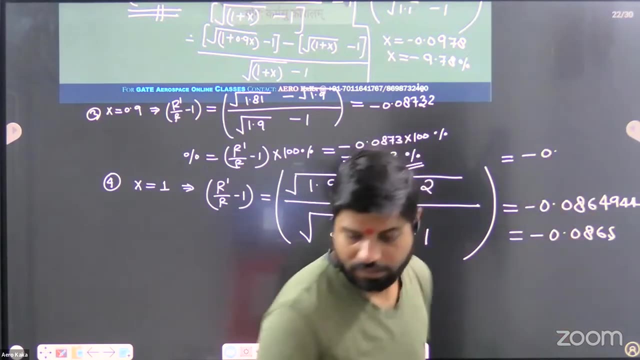 Are you getting this one? Hello, are you getting this one? Please verify this value. Yes, sir, Is it 0.865 or 0.8645?? I am getting this value exactly minus 0 point. how much? I am getting minus 0 point 0.8645.. 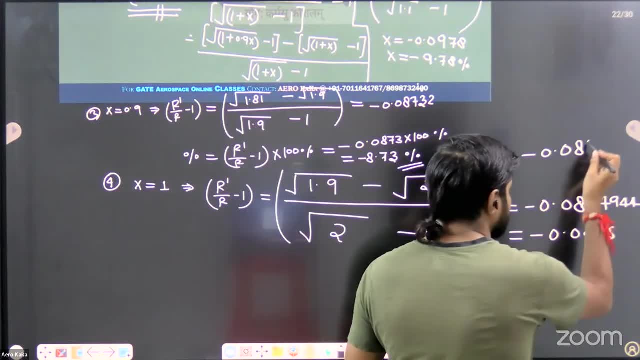 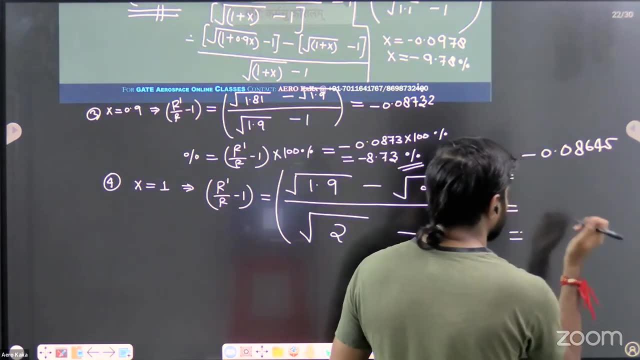 0.8645, right, Yes, sir. Why, Nandini? why are you making so many mistakes, Sir? to round off right, Don't round off this, Okay, sir, Minus 0.08645.. 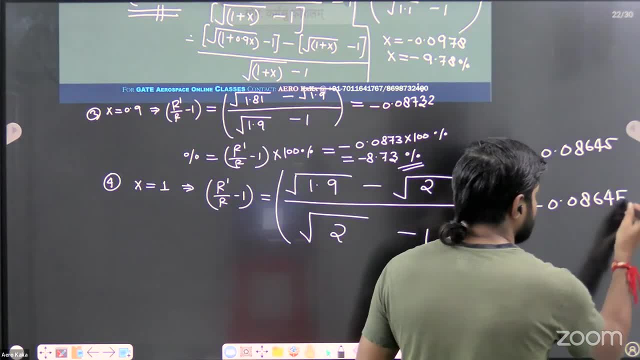 Okay, sir, Are you getting this value exactly? Yes, sir, Yes sir, 0865. 08. 08. 08. 08.. So if you want to write in percentage, then take our prime by our minus 1 into 100%. 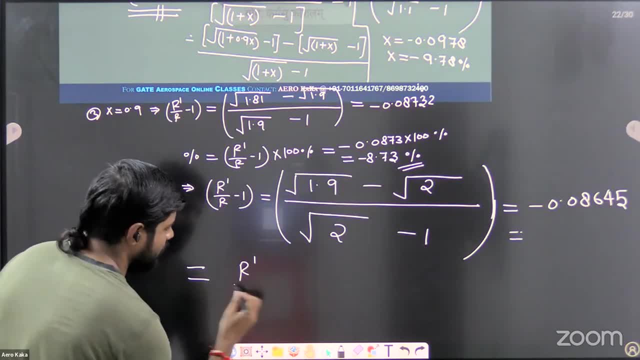 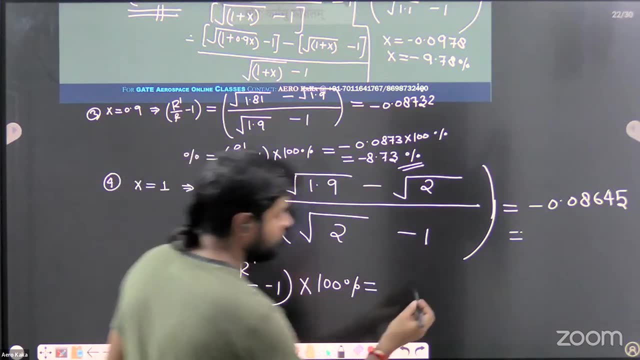 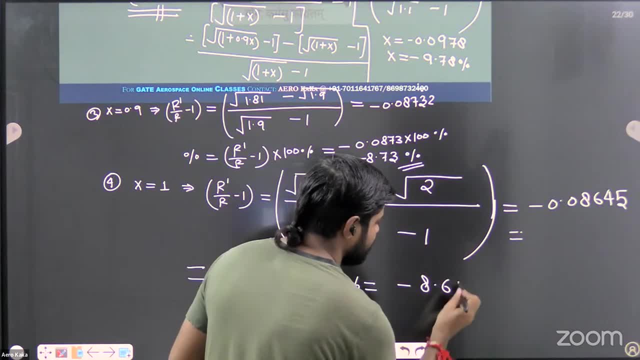 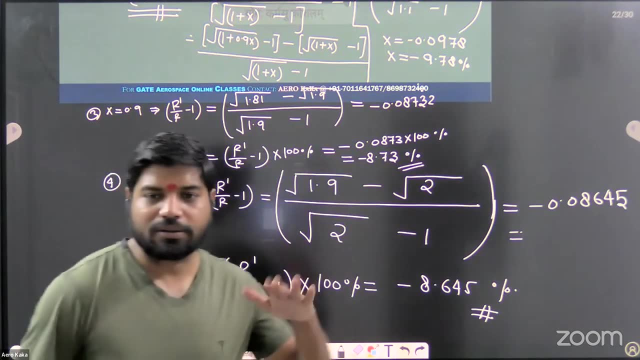 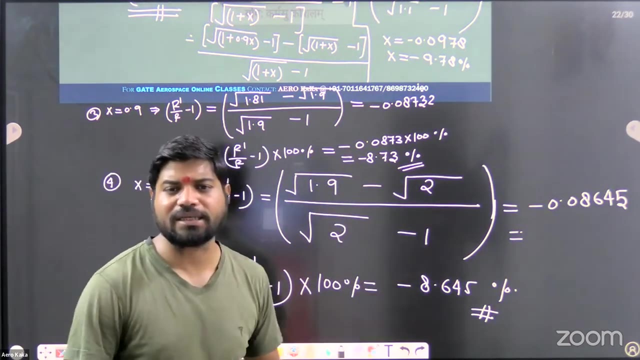 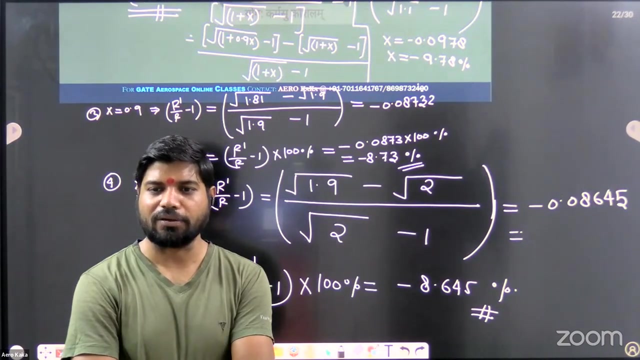 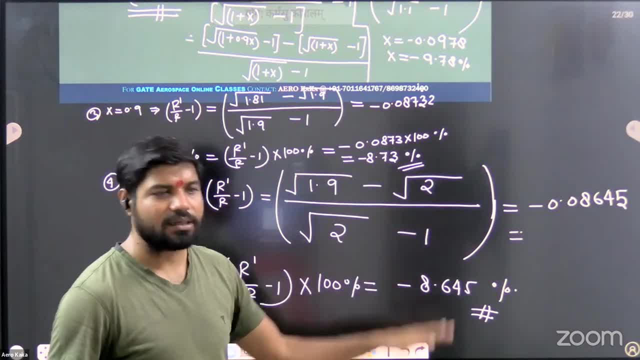 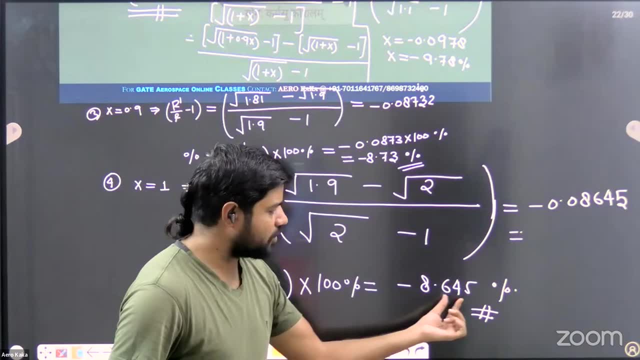 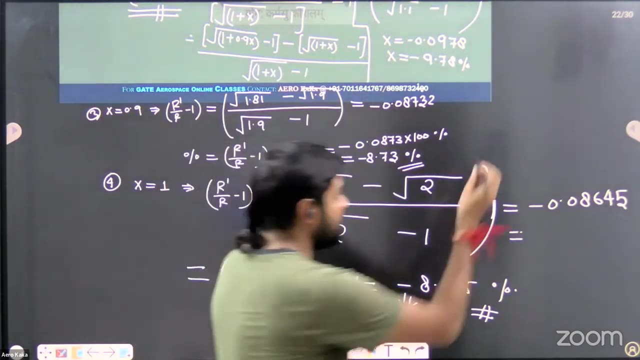 so it says the range is decreasing, or you can say it is lowered by or or reduced by, like that only, or it is to. or you can say minus 8.645, so please write somewhere. minus means lost here. or you can say reduction, so from x is equal to 0.1 to 1 if you are taking. 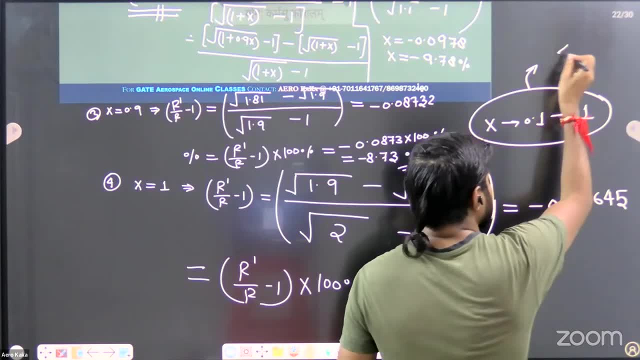 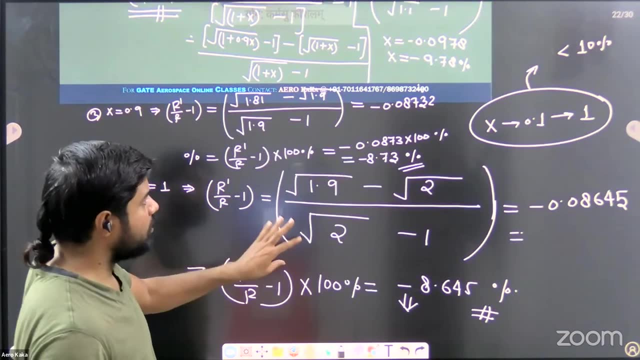 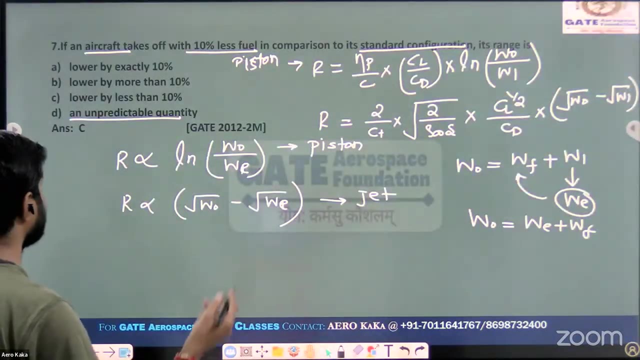 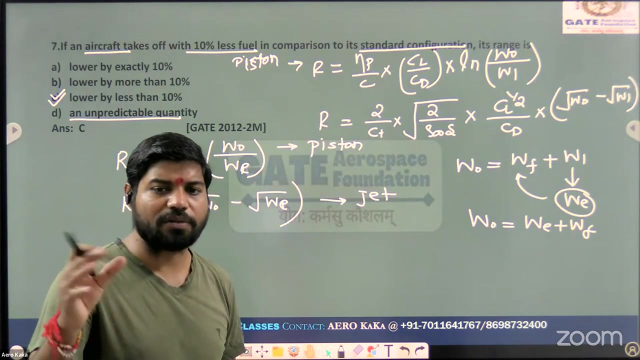 this value? we are getting all the values below 10 percent right. check. it means that what? even if we talk about this jet engine aircraft, which aircraft, which aircraft, which aircraft, jet engine aircraft, then you can say: option c is correct. which option is correct here? option c, let's see what happens. if suppose, if you are considering the aircraft means: 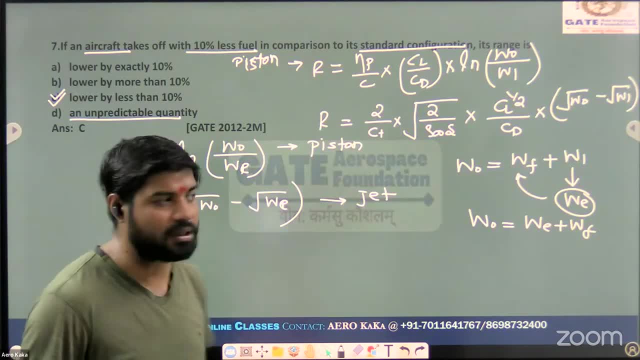 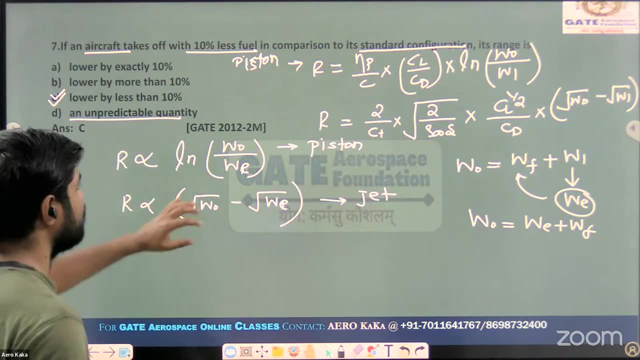 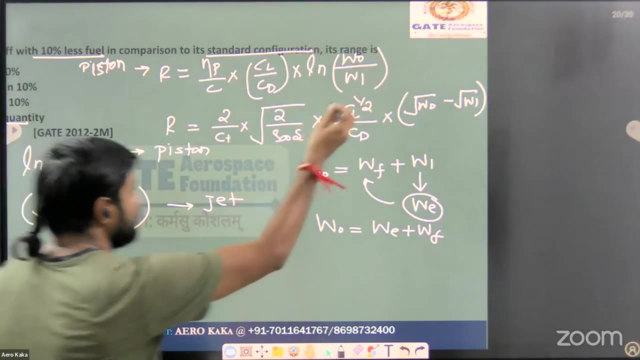 second case is what second case? you can consider the piston engine aircraft. okay, so in case of this piston engine aircraft, what you can write, just write down the formula here: that's a piston engine, this one right hello above that's, that's for this turn engine. so again, from this formula what you 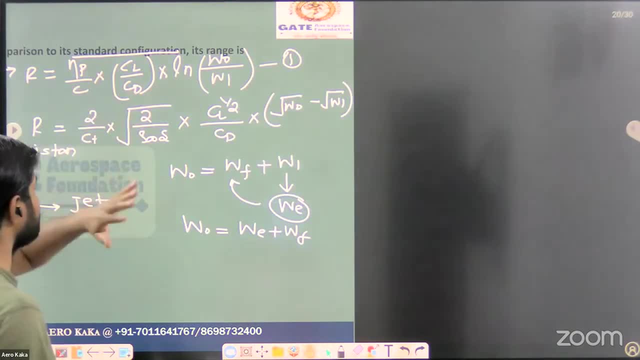 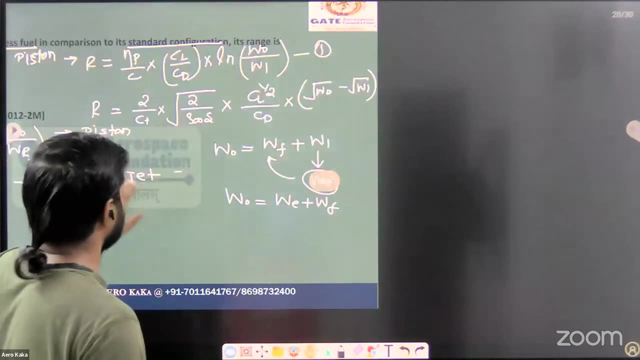 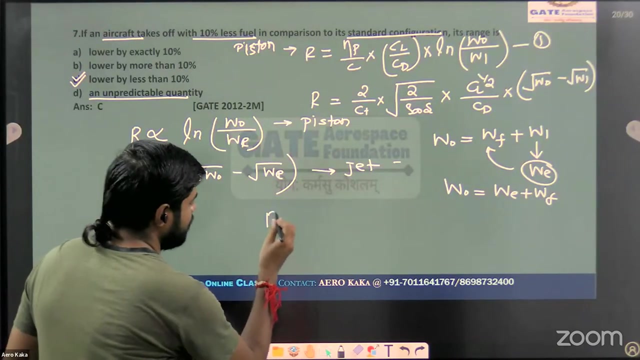 can write, since all the parameters are constant: c, l upon c, d, eta, p upon c, all the parameters. if you are keeping constant, okay, just wait, just wait, wait, wait, wait, something happened. if you are keeping all the parameters same, then we can write: r is proportional to how much. 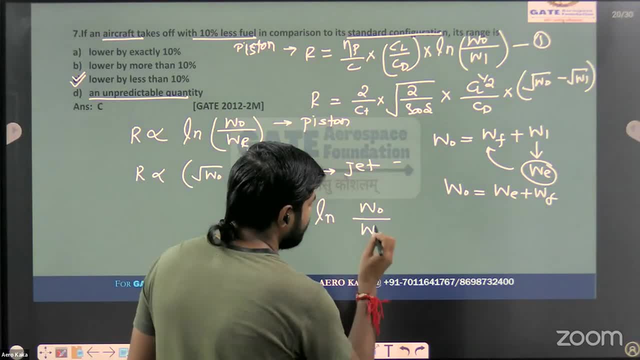 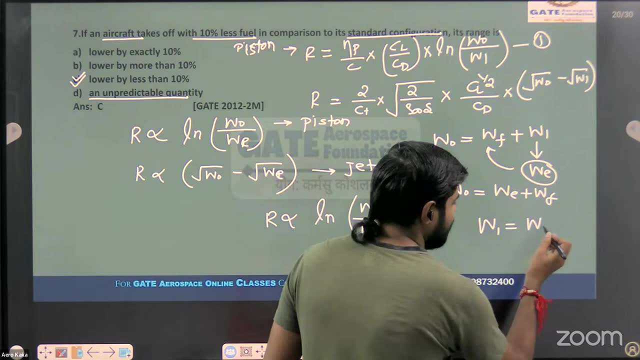 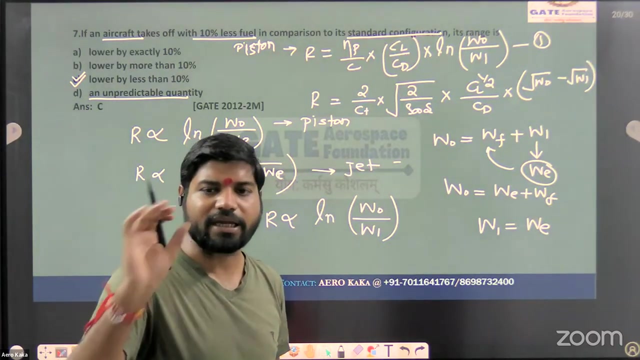 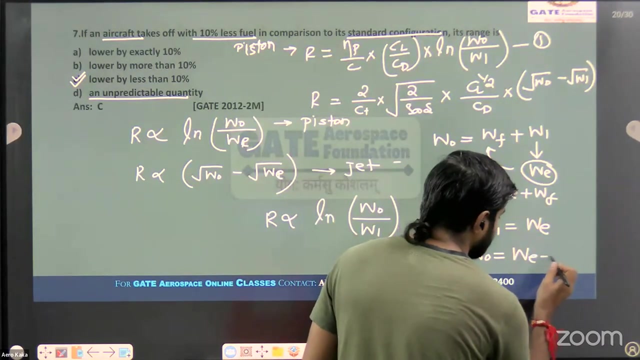 ln of w naught upon w1. say yes or no. yes, you may consider your w1 is nothing, but you can say all the weight, or you can say summation of all the weight of the aircraft excluding the fuel weight. okay, so here you can write: w naught is equal to how much w e plus w f. please take care of this. 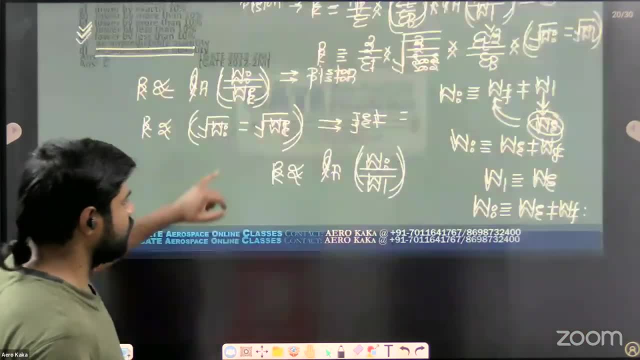 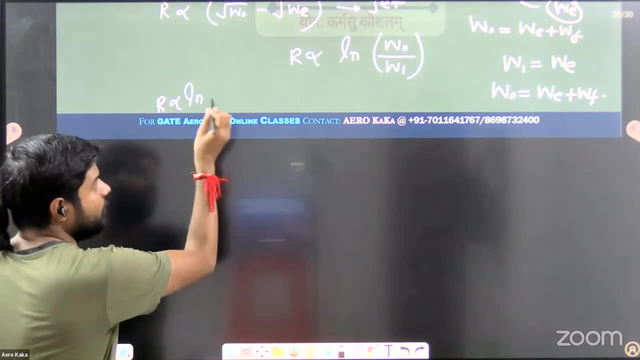 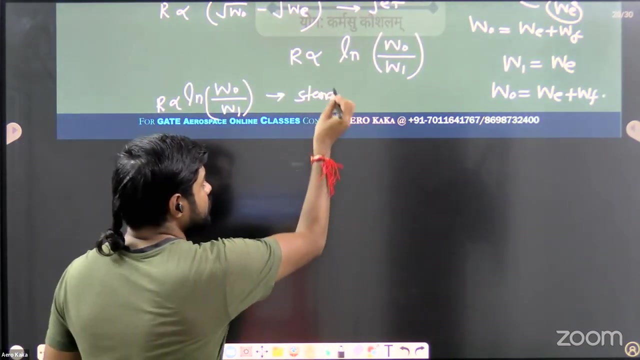 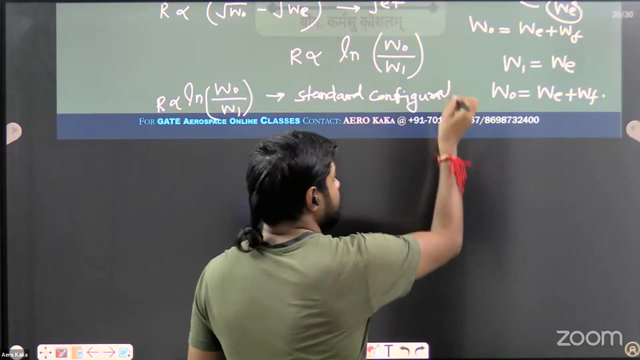 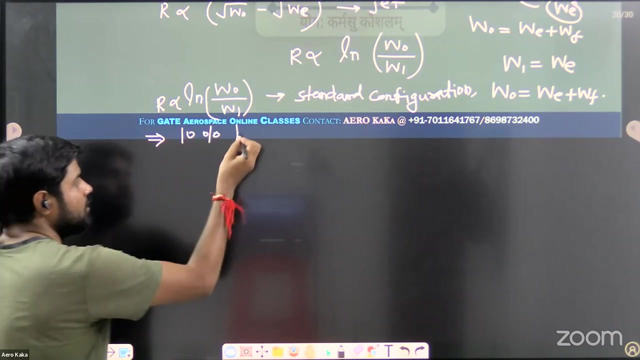 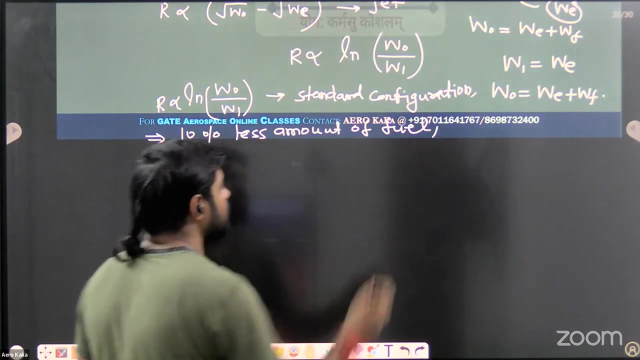 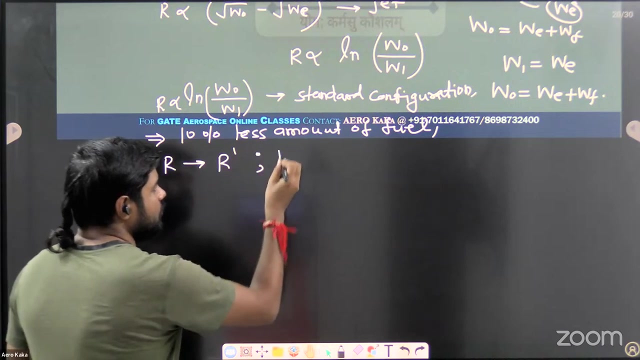 okay, let's solve this question. so what you can write again: same thing: r is proportional to ln of w naught upon w1. that's your standard configuration. now for let's say, suppose it carries 10 percent less amount of fuel. same procedure. let's say then, this range of this aircraft, let's say it's r prime. 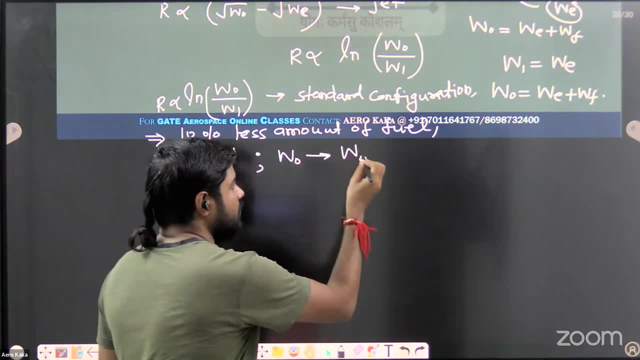 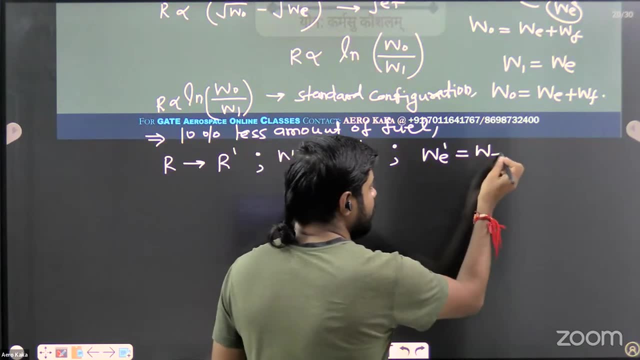 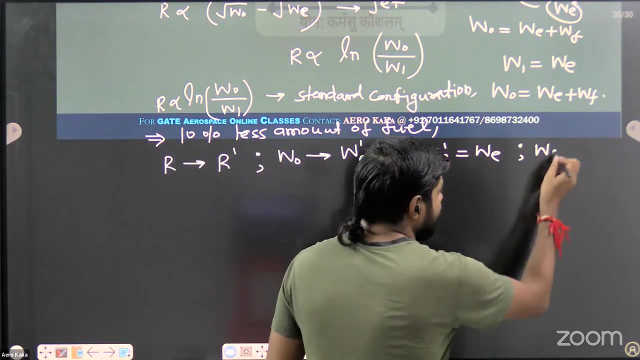 overall weight of this airplane. let's say it's a w? naught time. obviously in this case this w? e prime is nothing. but you can say we only, it is not going to change. say yes or no first hello. and what about the weight of the fuel? obviously the weight of the 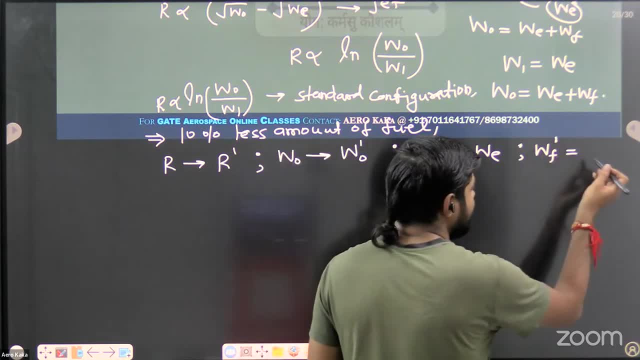 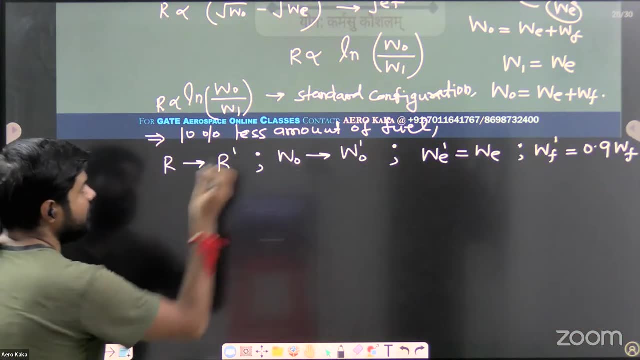 fuel is 10 percent, how much of which is the fuel? 1000, it is there from apuche. whatever the weight is. are 10 percent? less amount of the fuel means what wf prime is nothing, but you can see 0.9 times of wf. only that's it. just apply this condition. you can write: let's say this is nothing but equation. 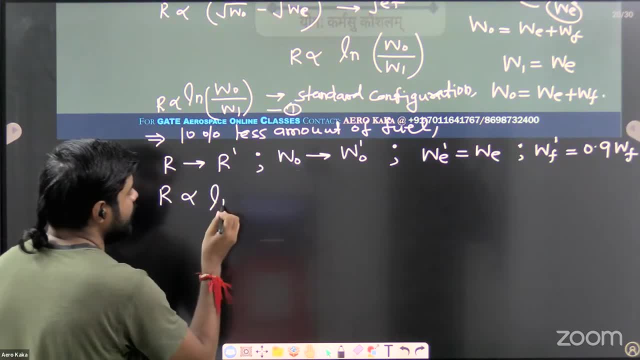 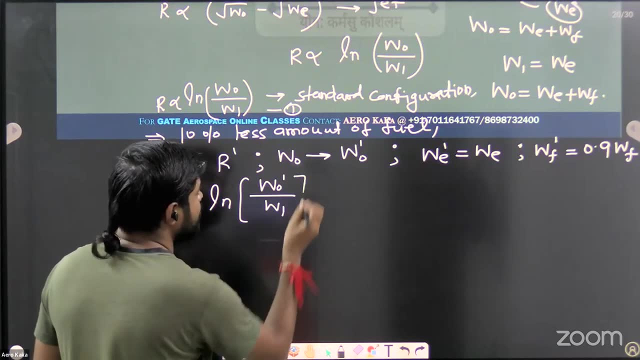 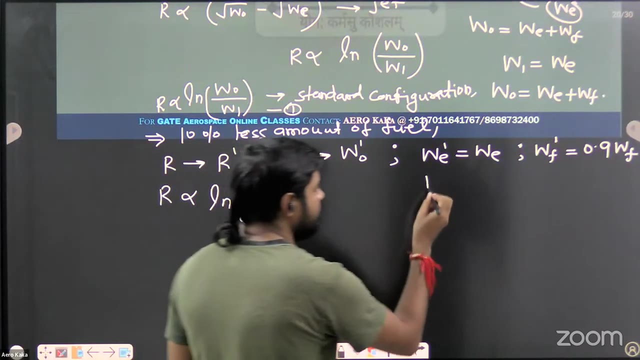 number one. again, you can write equation number two. r is proportional to ln of how much w naught prime check divided by w1. say yes or no, hello, yes, if you want to write in ratio form, you can, no issue at all. so what is the value? w naught upon w1, if you want to write, or you can. 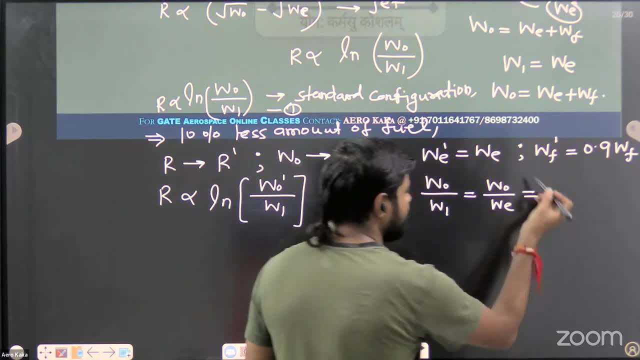 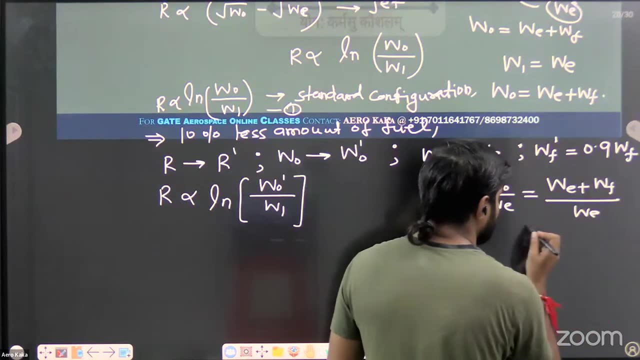 take this w naught upon w e right here. what is the w naught? it's nothing. but you can say w e plus divided by w e. let me simplify it: how much we'll get 1 plus w f upon w e. let's consider this wf. 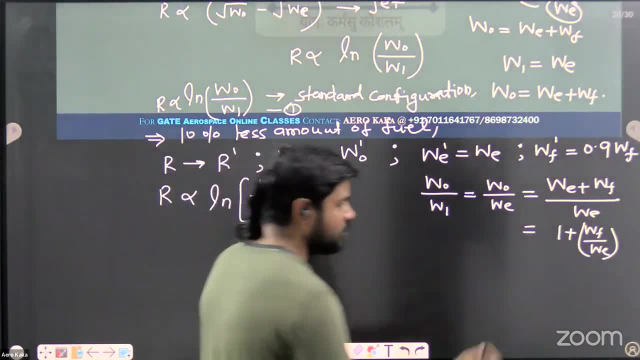 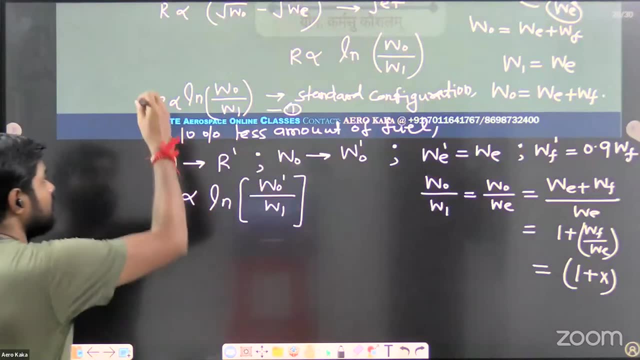 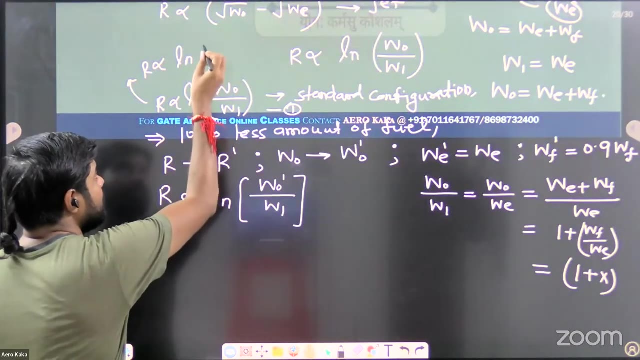 upon w is nothing, but you can say capital x here. okay. so simply what you can write here, let's say it's a one plus x, but please remember what is this capital x here? okay, so your equation number one, finally, you can write: r is proportional to how much ln of. tell me how much will you get ln of how much one plus x. 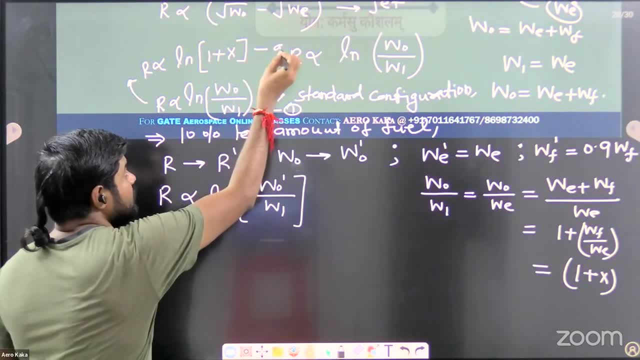 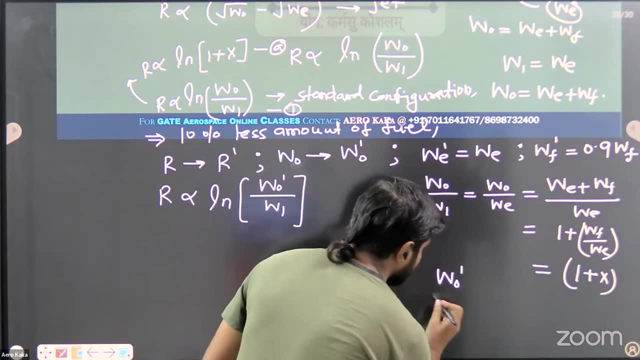 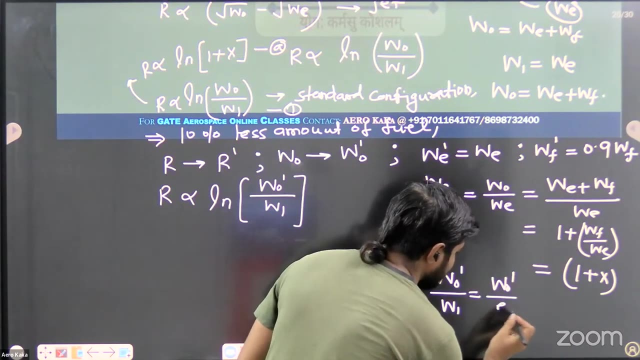 only check one plus x. let's say this is equation number k. similarly, if you simplify it further, then what you can write here, this w naught prime upon how much w1 is nothing. but you can see it's a w naught prime upon w e. 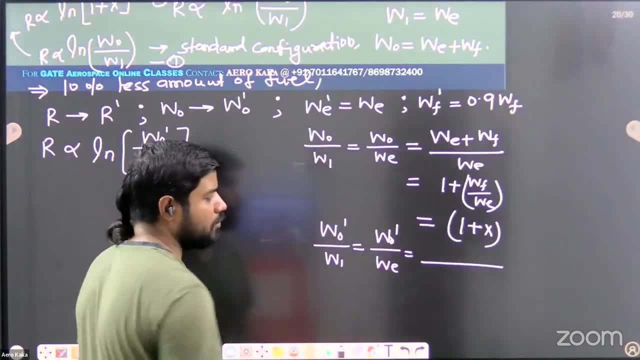 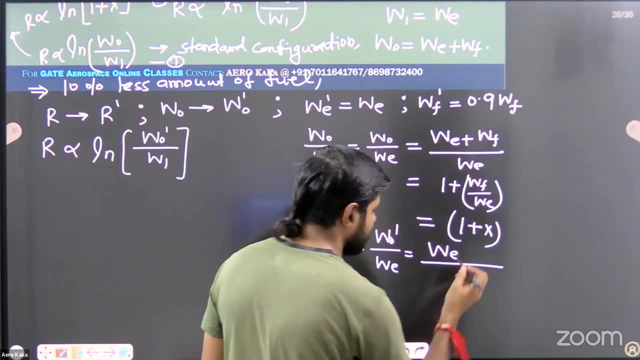 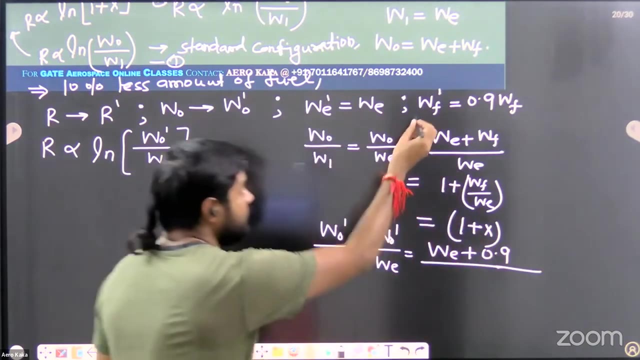 so what is this value? prabhuji, hello, what is this? w not prime. see this w not prime is nothing, but you can see your empty weight is not going to change. so w e plus how much, how much? this value, obviously, in this case this w e prime- sorry, w f prime- is nothing, but how much. 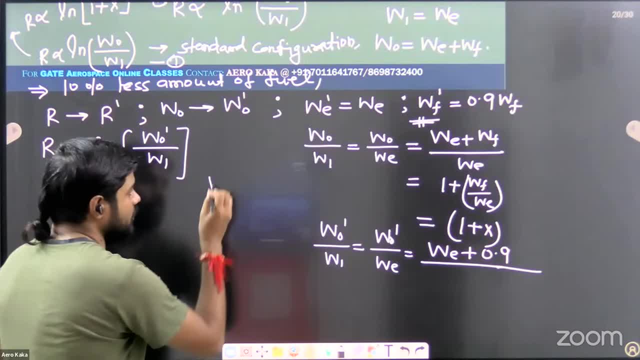 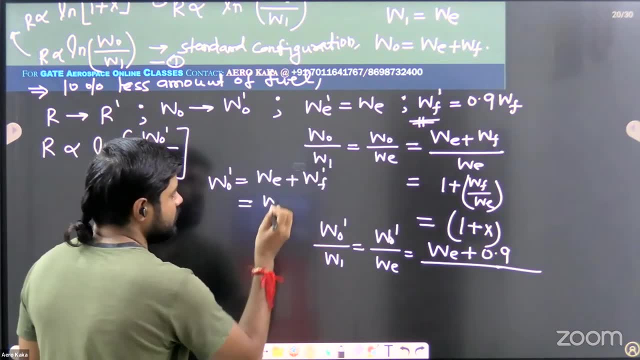 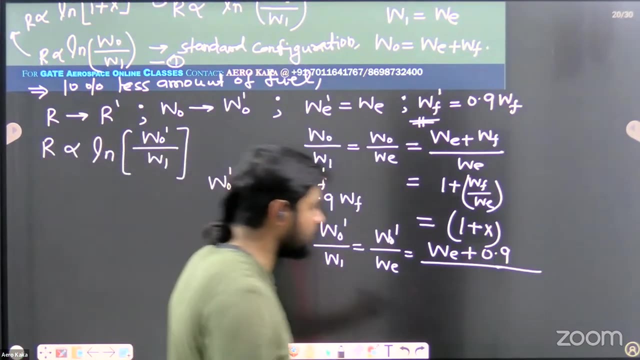 0.9 wf only. so please remember: your w naught prime is nothing, but you can say w e plus w f prime only. so this is nothing, but you can say w e plus 0.9 times of w f, clear, hello. any doubt, please let. 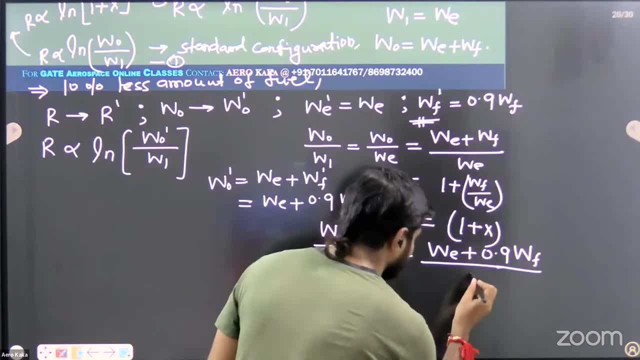 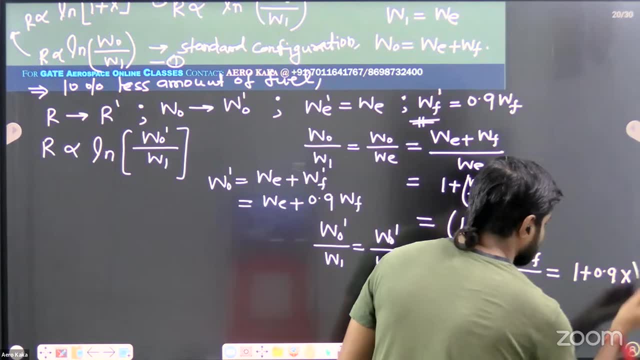 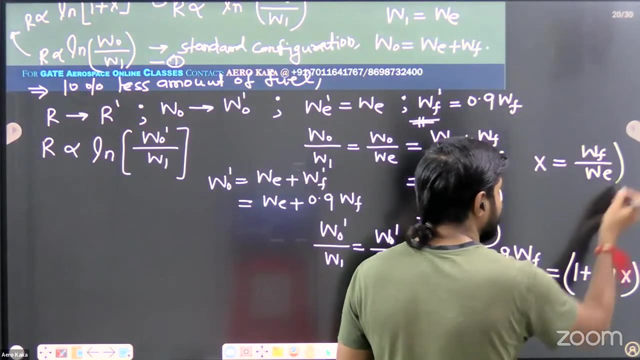 me know, agree or not? yes, sir, if you simplify it further, what you can write it's a 1 plus 0.9 x. what is x here? x is nothing, but you can see w f upon how much w? e. right, check those, prabhuji. 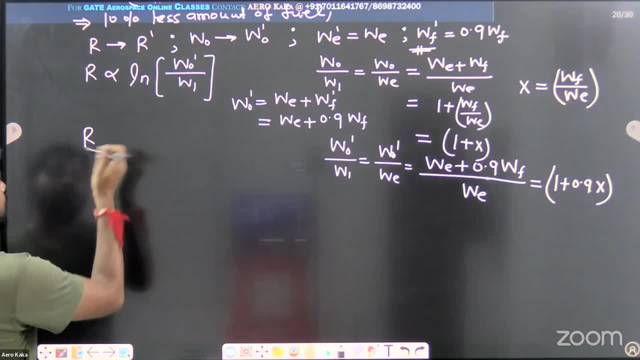 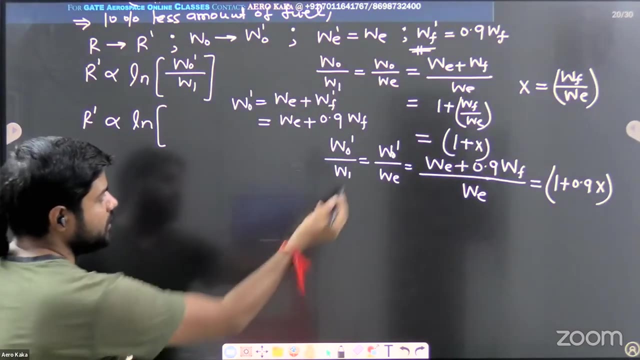 so what you can write r is: yes, sir, take the ratio. okay, let me write here this: r prime right. r prime is proportional to ln of w naught upon w naught prime upon the w. 1 is nothing, but you can say w naught prime upon w e. and what is this value? 1 plus 0.9. 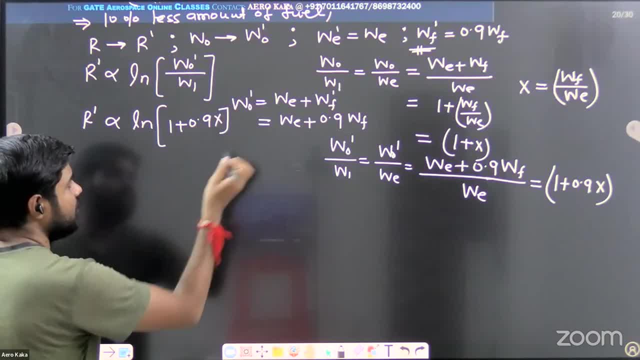 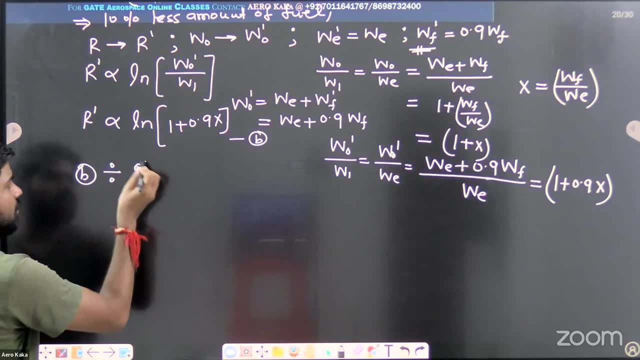 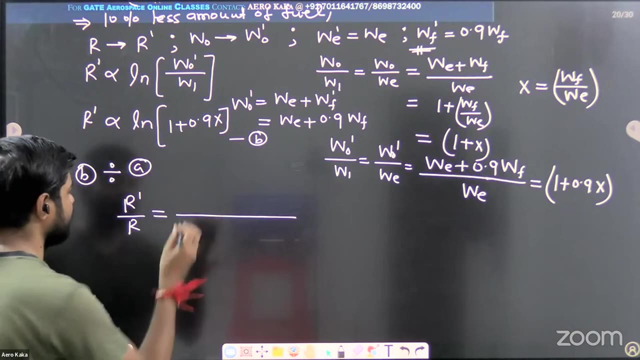 1 plus 0.9 x. right, let's say this is nothing but equation number p. now take the ratio, equation b by equation a, and what you can write: r, prime upon r, which equal to how much prabhuji hello, how much ln of 1 plus 0.9 x, right, check. 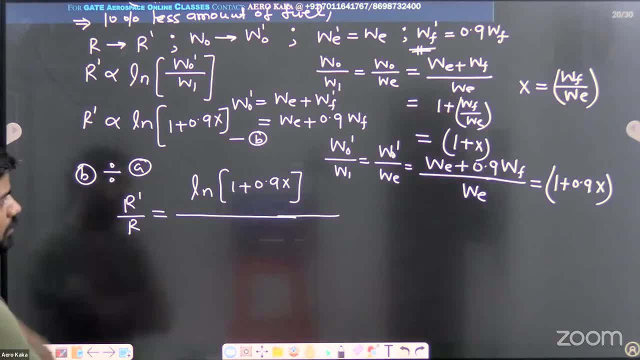 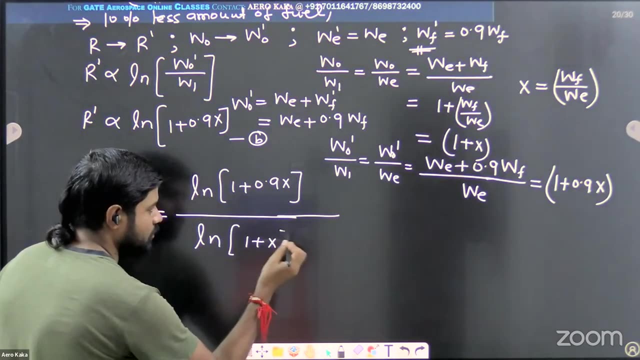 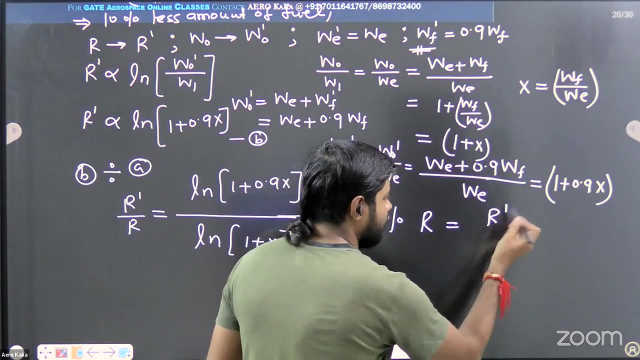 is it correct? yes, sir, are you sure? please let me know if i'm making any mistake, please. yes, sir, are you sure? yes, sir, okay, let's say, if suppose, if you want to check, like, what is the percentage change in r, there's nothing what you can say. final final range minus initial. 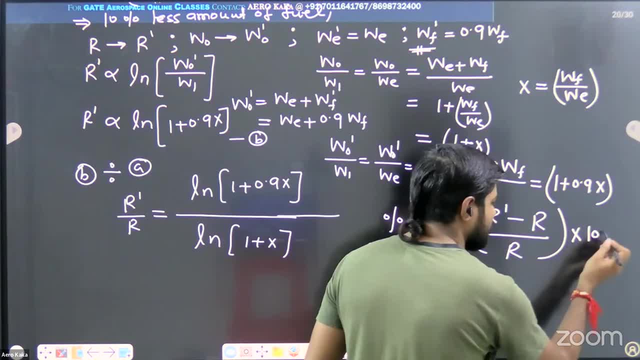 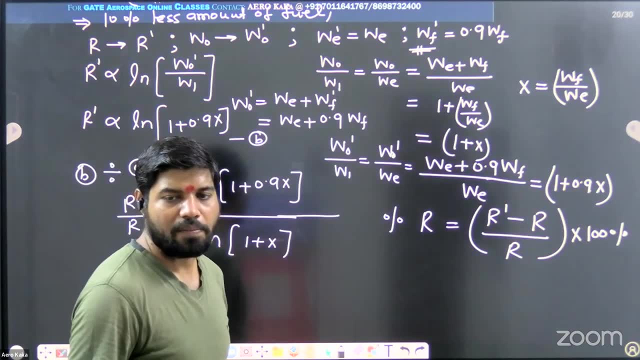 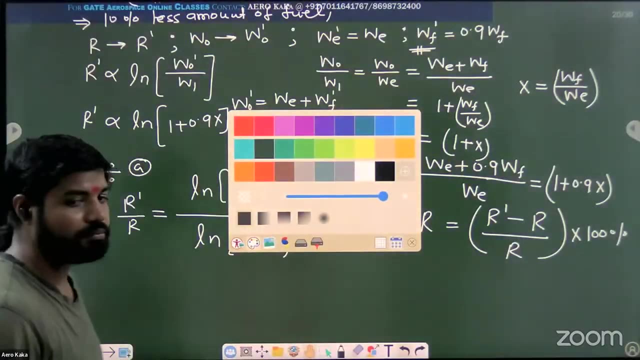 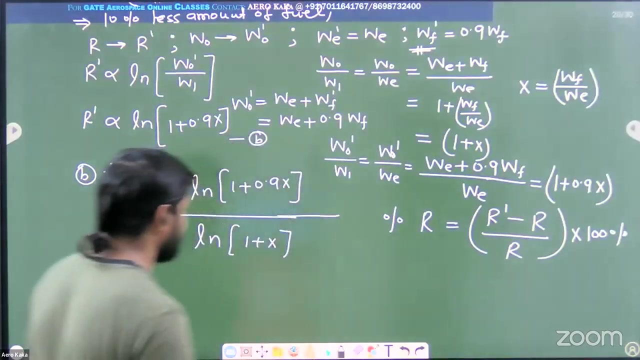 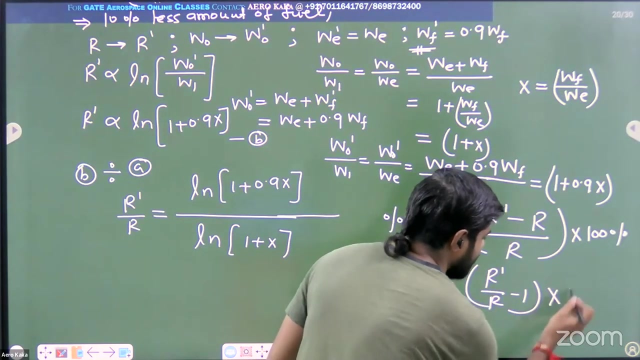 divided by initial into 100 percent. right check, please agree, prabhuji. are you agree or not? yes, sir, are you agree or not? please let me know first. okay, so again what you can write r prime upon r minus 1 into 100 percent. clear, just calculate what is the value of this. 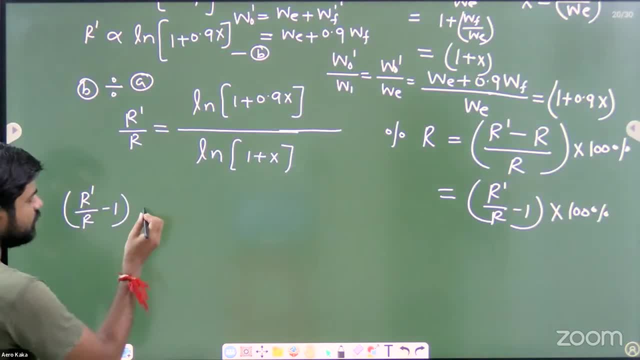 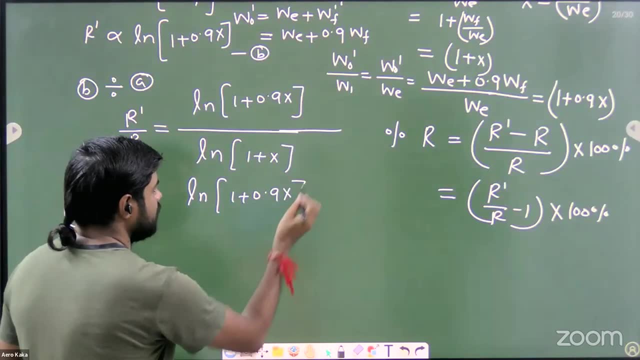 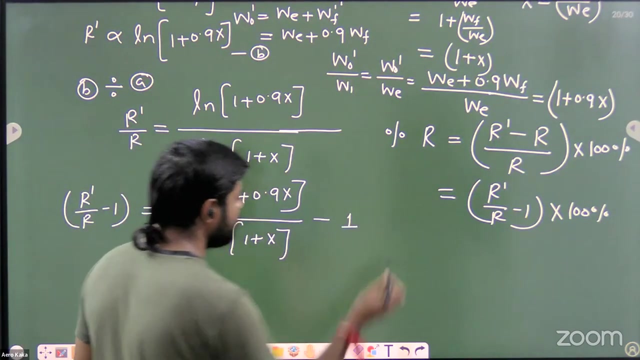 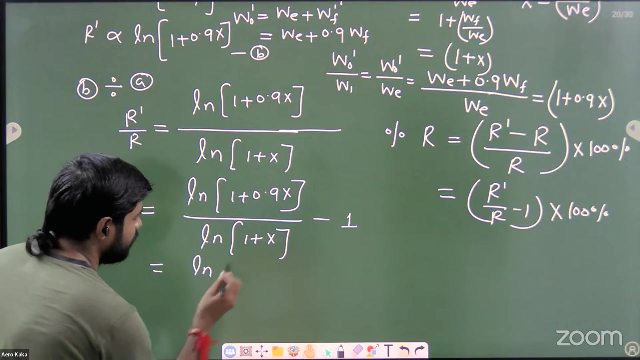 r prime upon r minus 1, how much we'll get? you're getting this is nothing: ln of 1 plus 0.9 x divided by ln of 1 plus x minus. how much minus 1? hello, are you agree? yes, sir, simplified for the how much you will get: ln of 1 plus 0.9 x minus ln of 1 plus x. 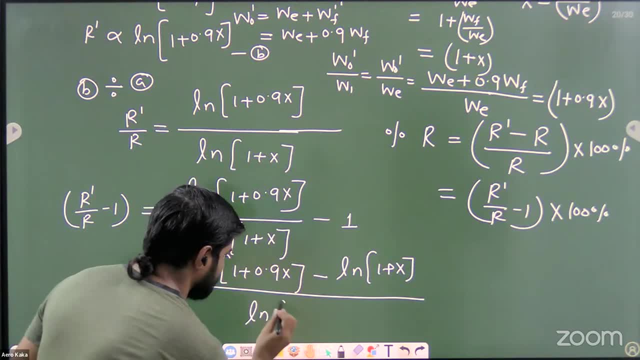 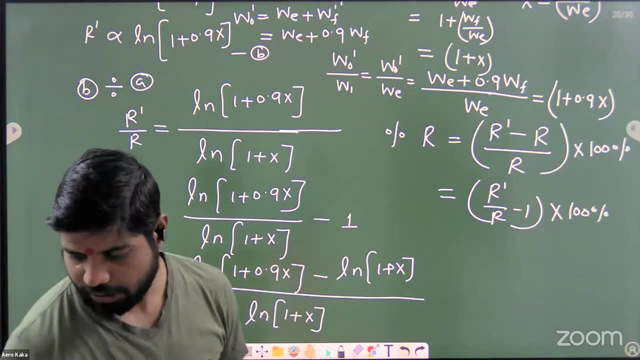 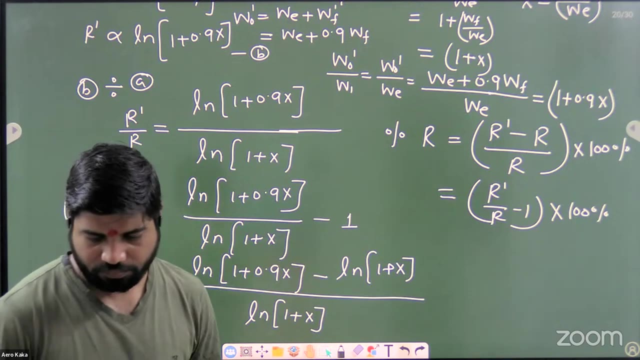 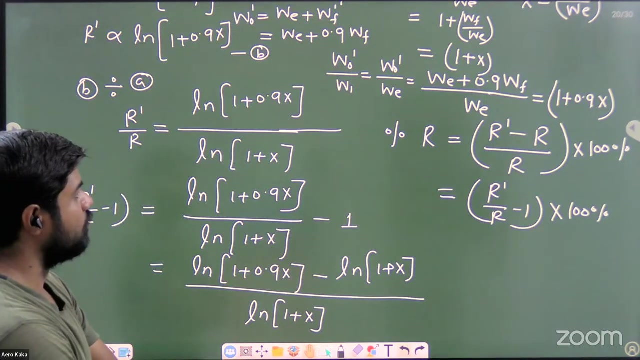 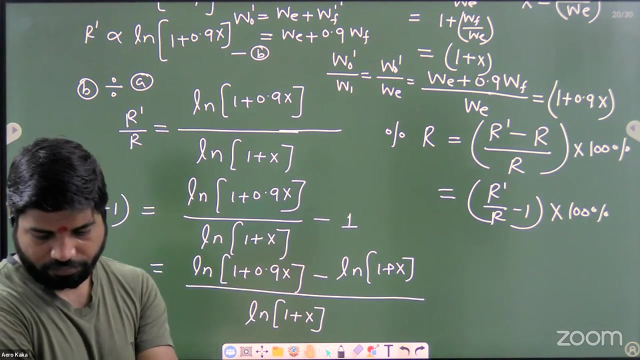 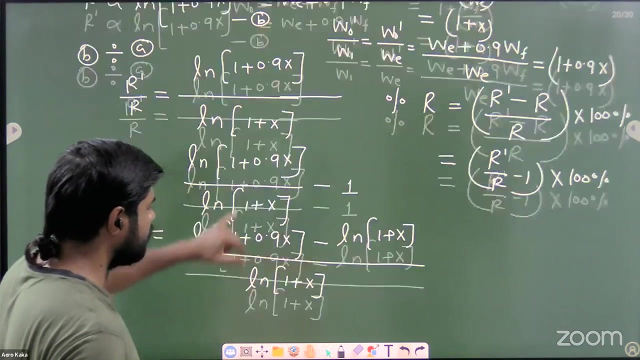 divided by ln of 1 plus x. agree, check please, hello. are you getting this value or not? yes, sir, getting. yes sir, getting. yes, sir, getting latj r prime. ok r prime weak? all right, all right, calculate so that's your final value. now take x, h, equal to again. we are having two extreme conditions. 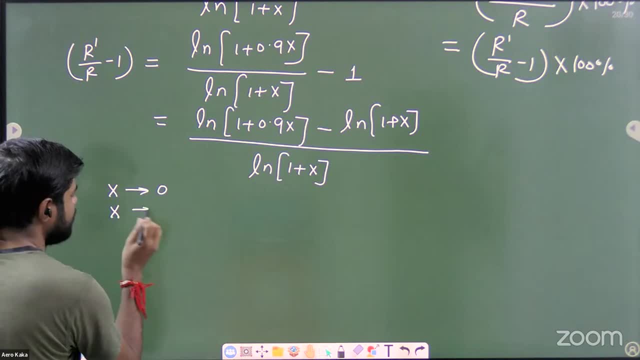 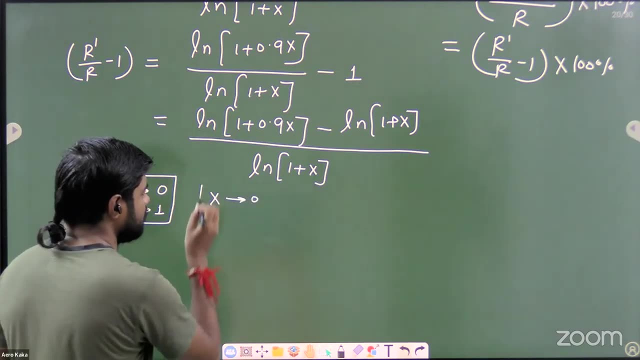 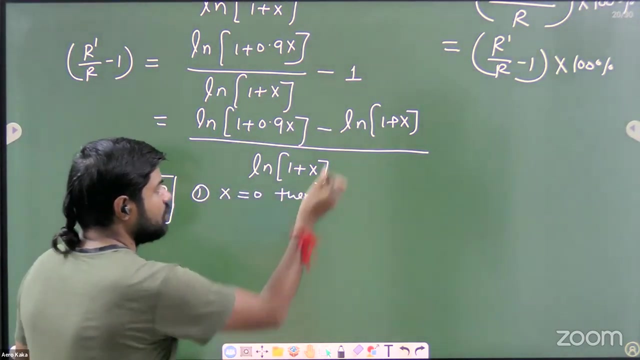 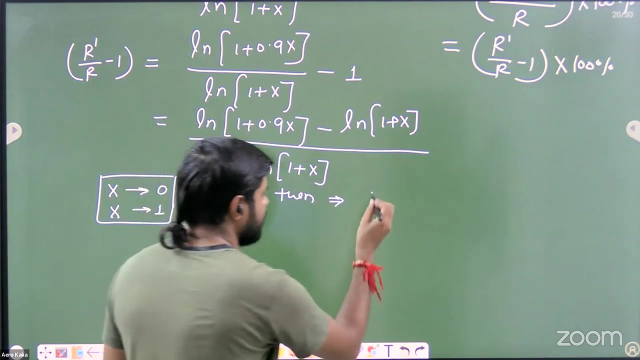 but x stands to 0 and x stands to 1. right check, am i audible? let's consider, if suppose this x stands to 0, or consider this one. let's say x is equal to 0, then what? please check whether this one is correct or not. then what you can write. then you can write this: 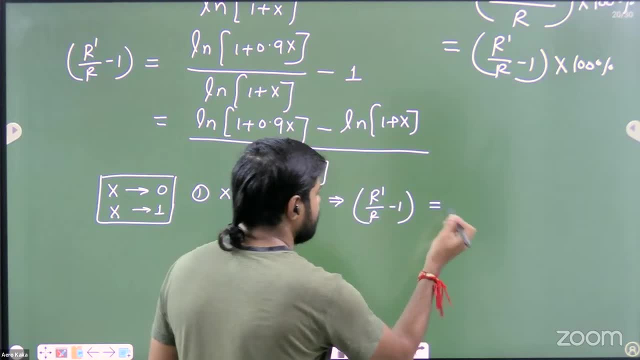 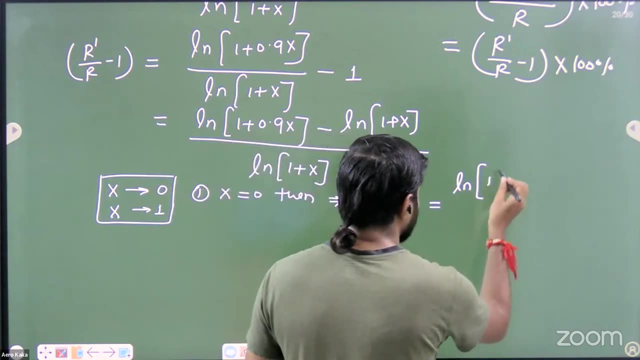 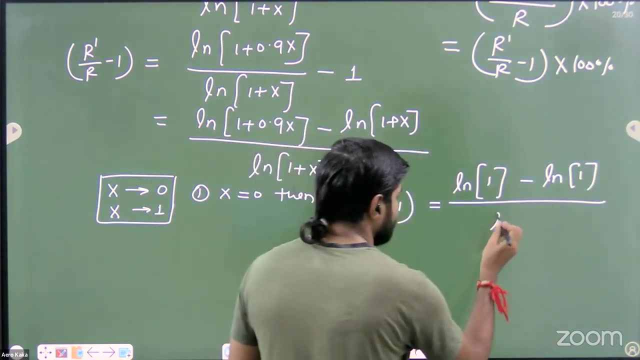 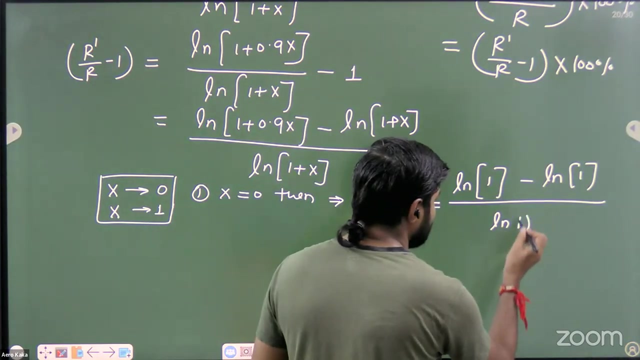 r prime by r minus 1, which is equal to how much ln of how much you are getting? x is equal to 0, right? so ln of 1 minus ln of 1, check, divided by how much? ln of 2? no, ln of 1, only right. so what is the value of ln of 1? anyone? 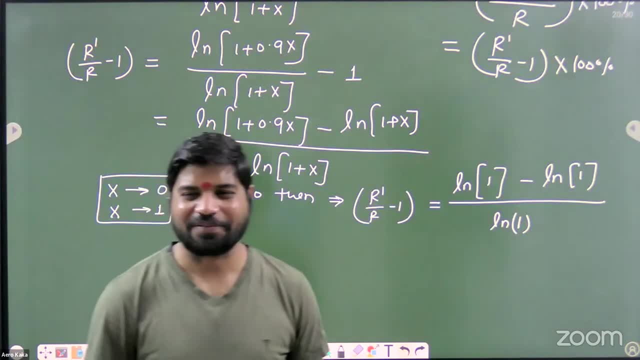 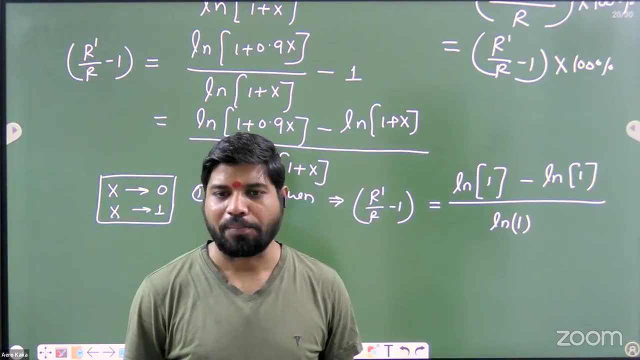 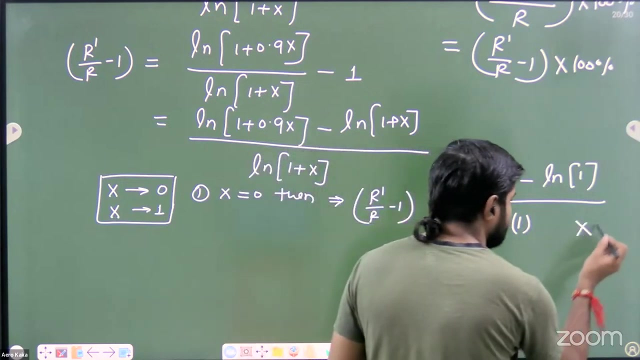 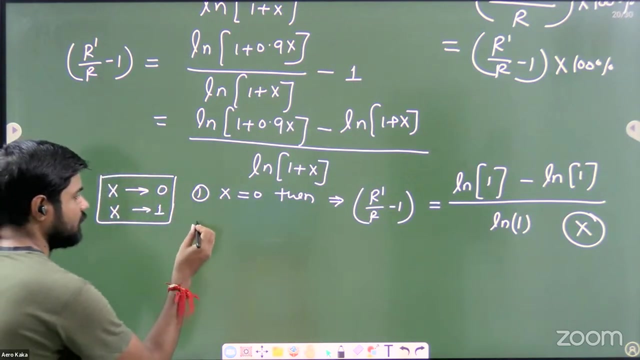 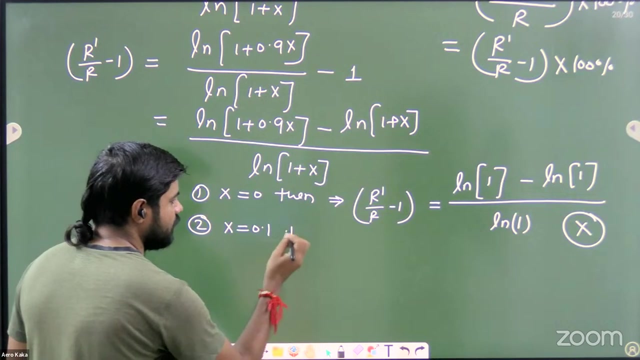 yes, 0, 100, 200. how much? 0 yes, sir. so again, which condition is this? you can say: this is not possible, cannot fly without the fuel right now. consider: is to, x tends to. or you can say: x is equal to 0.1, then 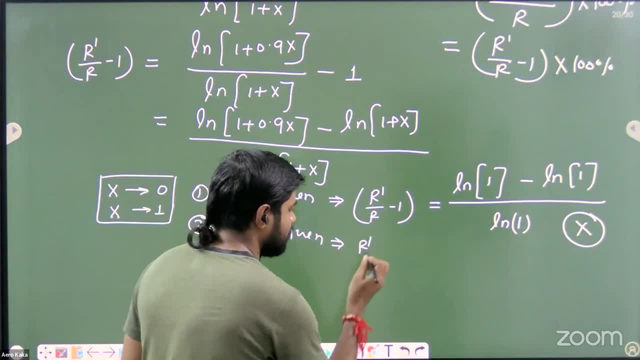 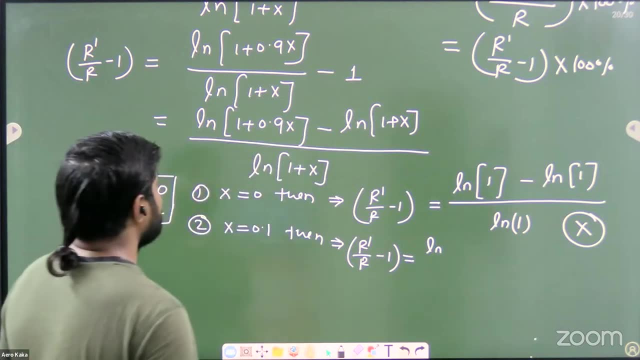 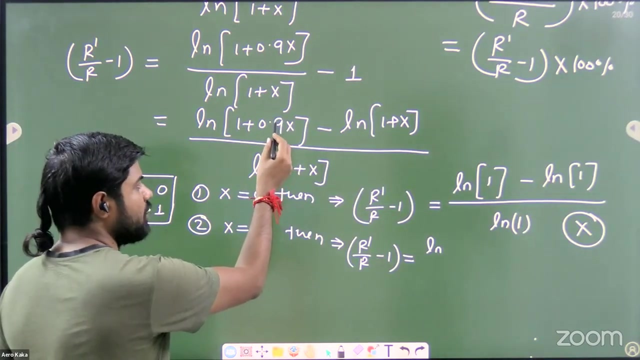 x is equal to 0.1, 0.1, 0.1. You can write r prime upon r minus 1, which is equal to how much? ln of x is equal to 0.1.. So 0.1 into 0.9 is how much 0.09.. Check please, Agree. 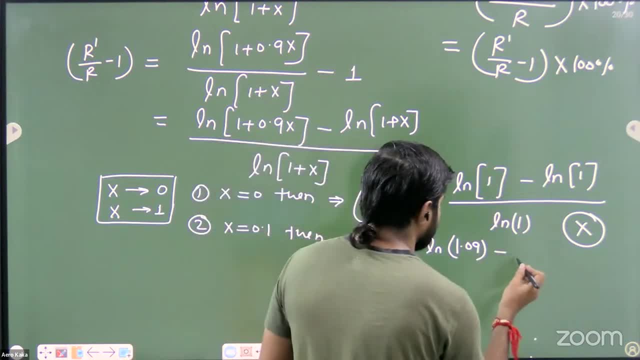 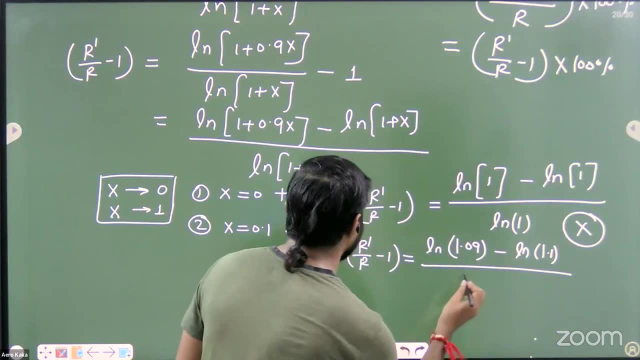 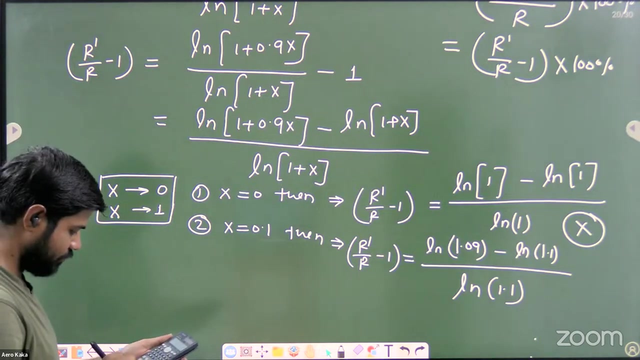 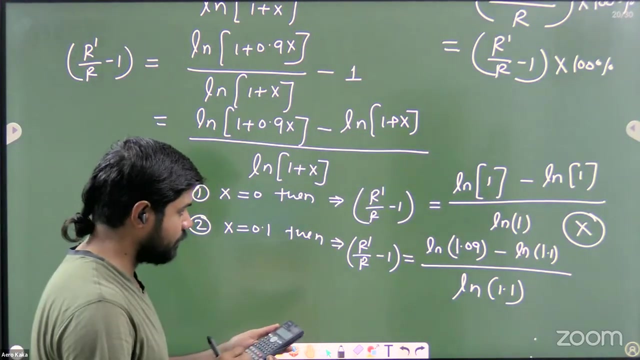 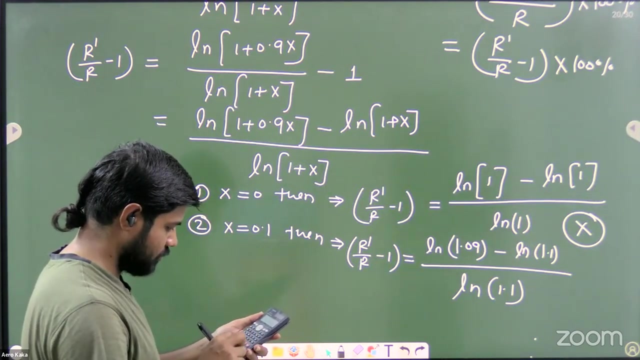 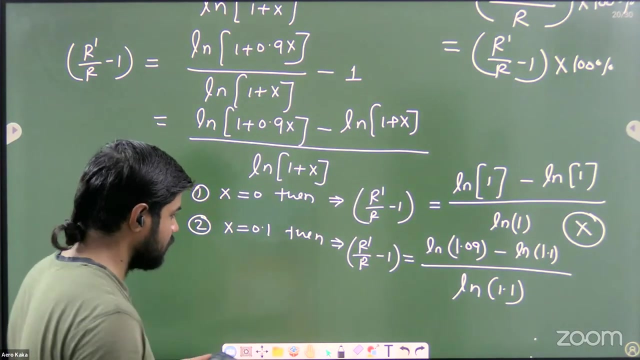 Agree, Minus ln of 1.1.. Agree. Hello, Divided by ln of 1.1.. Please check this is correct or not? Minus 0.0958.. Minus 0.095818.. Yes, how much you are getting, Minus 0.0958.. 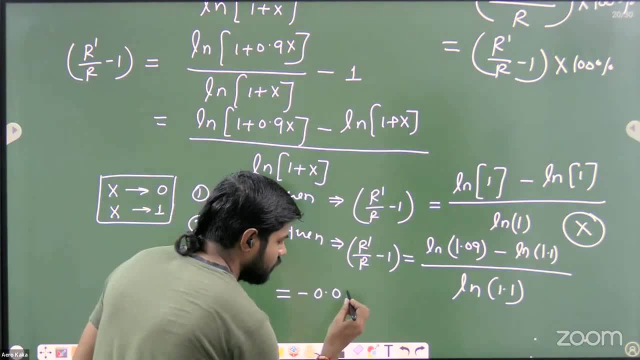 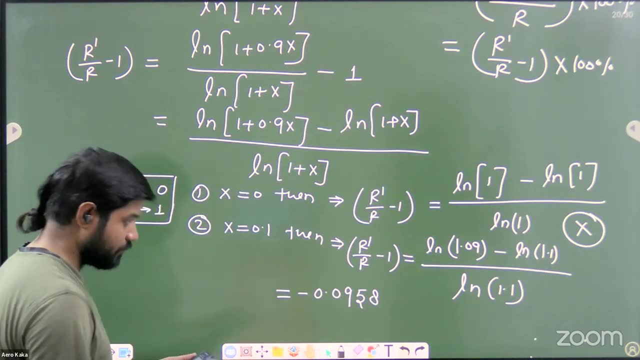 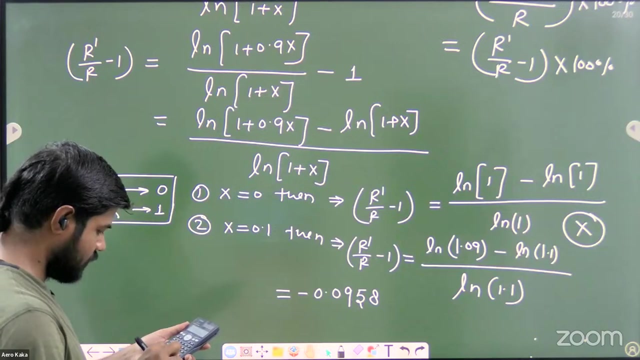 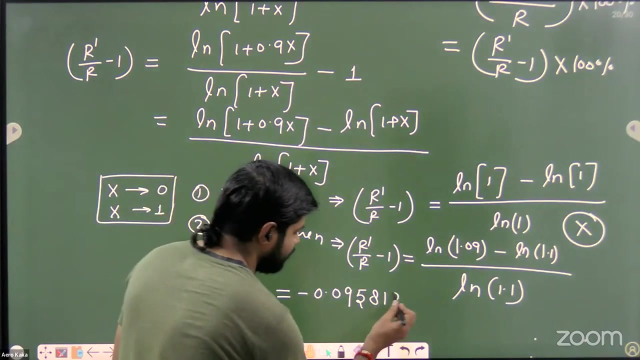 Minus 0.0958.. Yes, sir, Okay, that means, Can you verify? Please verify this value Minus 0.09581855, something like that. right, Yes, That's what you are getting. Yes, sir. 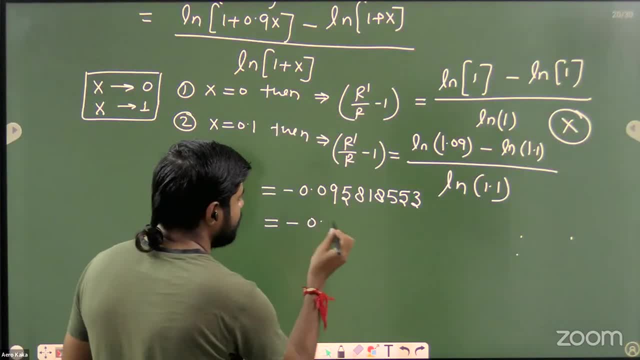 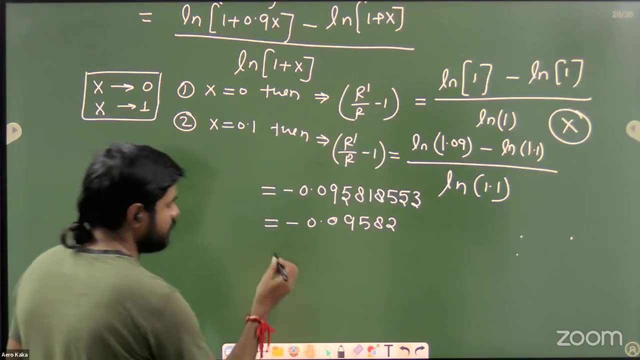 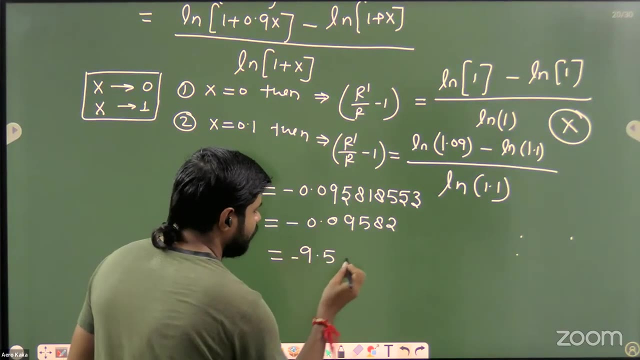 So this value is nothing but minus 0.09582.. Okay, So suppose if you want to write in percentage, then just multiply by 100. So you will get how much Minus 0.0958.. Minus 0.09582%. 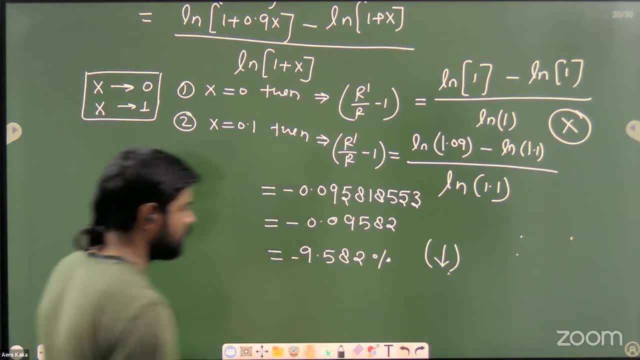 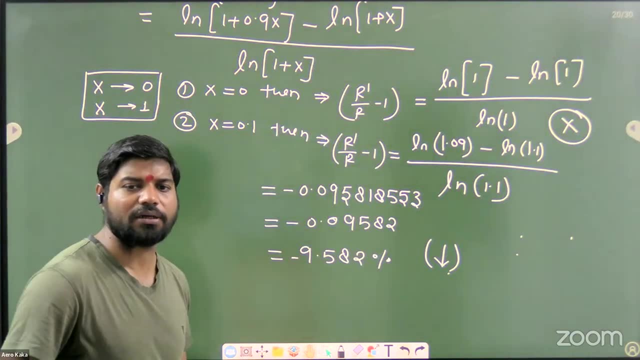 So means what Your range is taken right By what Minus 0.09582%? Let's consider another means, hypothetical, Which is hypothetical: X tends to 1.. So even if you consider X is equal to 0.9, 0.95, you will get some finite value. 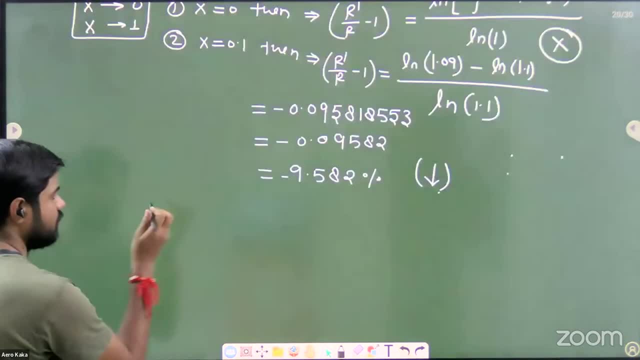 Please check, verify. So let's consider: Let's say X is equal to 0.9.. Then what do you get? Minus 0.09582%. No need to verify these all things. okay, It is just only for the clarity. 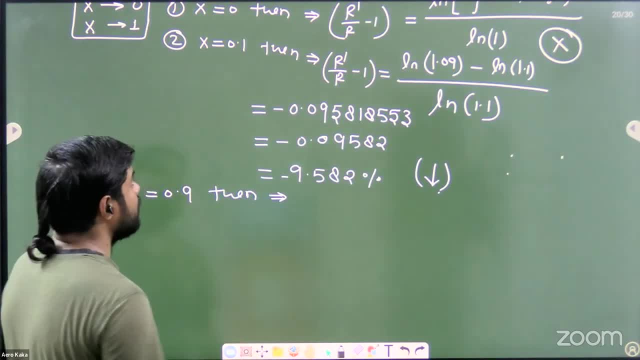 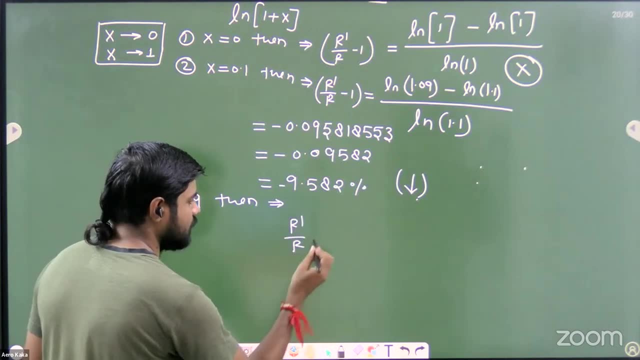 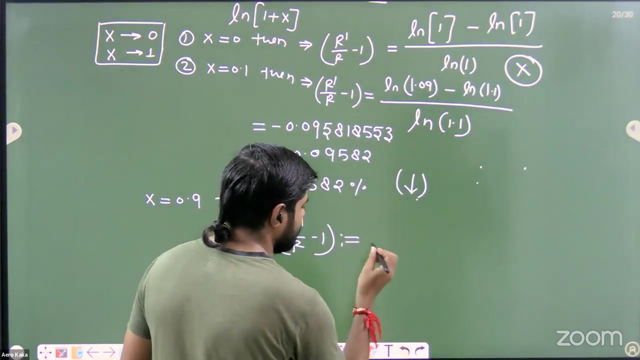 Is that clear or not? X is equal to 0.9.. So if you are putting this value here, then what you can write R times upon R minus 1 into 100%. Sorry, which is equal to how much? 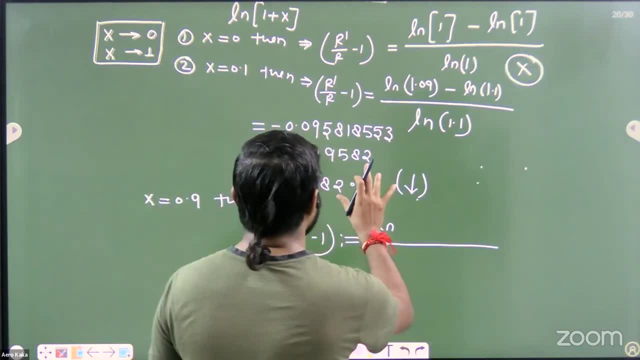 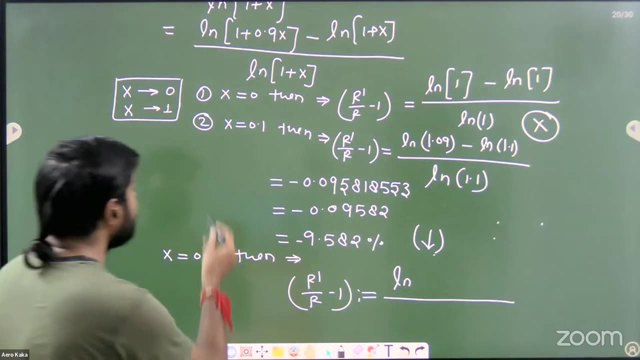 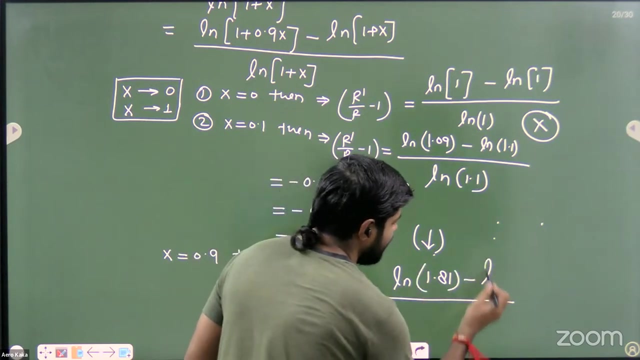 ln of. look, if you are putting X is equal to 0.9 in this equation, then definitely how much you will get 0.9 into 9.. How much ln of 1.81.. Please verify Minus ln of. 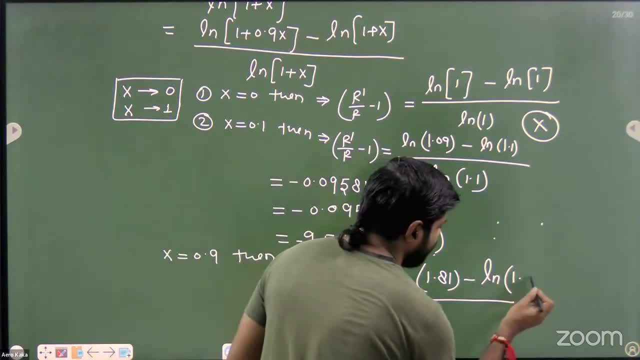 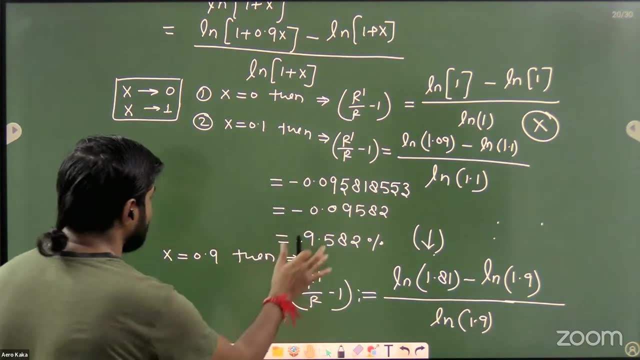 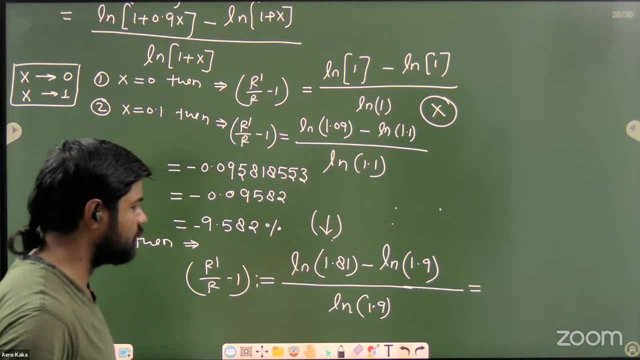 How much 0.9.. So it becomes ln of minus 1.9.. Check Divided by ln of 1.9.. Please let me know how much you are getting, Yes, How much is it Minus 0.075604.. 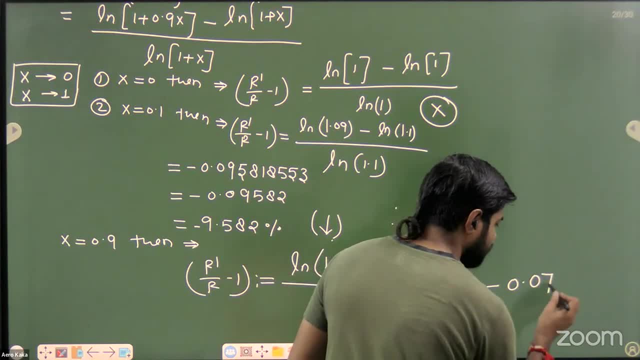 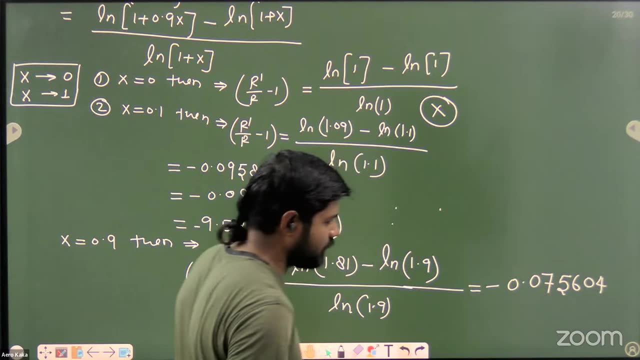 Minus 0.0?. 7, 5, 6, 0, 4, 0, 4.. Yes, sir, Okay, Leave it. Leave it, So please verify this value first. Hello, Please verify whether you are getting this one or not. 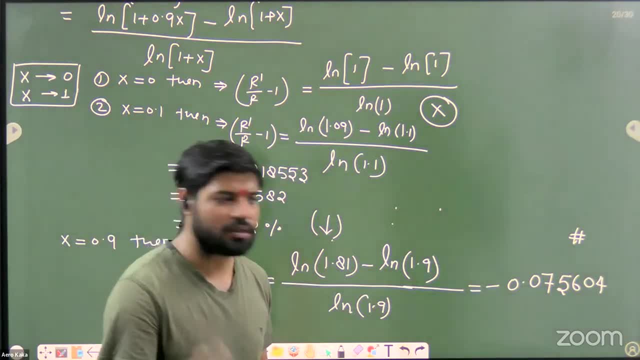 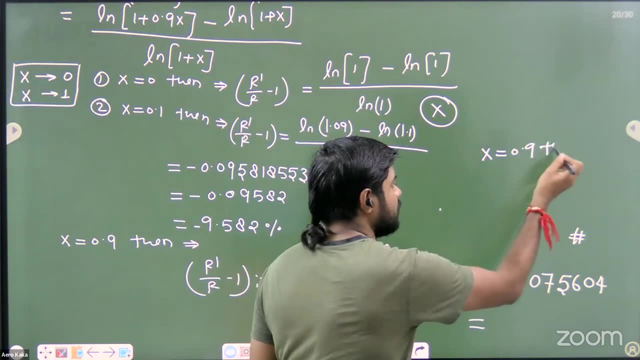 Yes, sir. Okay, So just multiply your 100.. So that's the percentage. So you can write here: This is nothing, but you can see, when this X is equal to 0.9, then your percentage chance is how much. 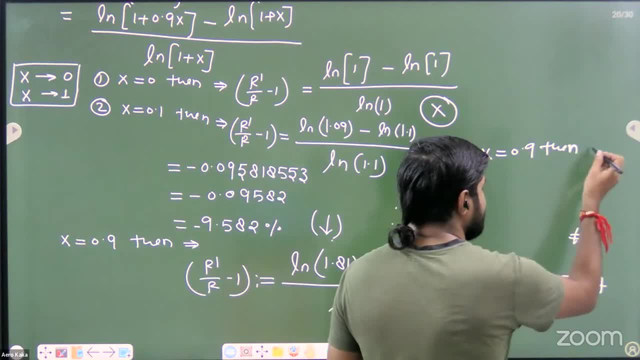 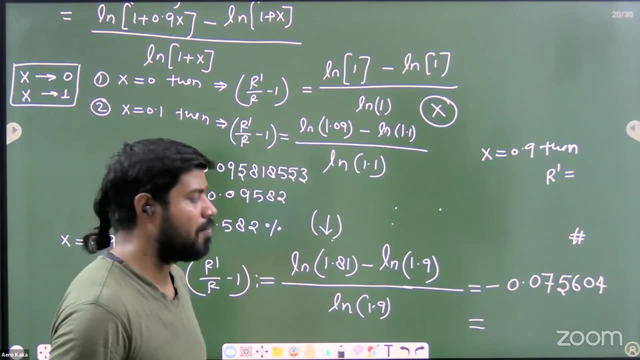 Minus 7.56.. Minus 7.56.. You are getting this. So this value R, prime each value, how much, How much we will get? Yes, please, You are getting this ratio. This is how much. 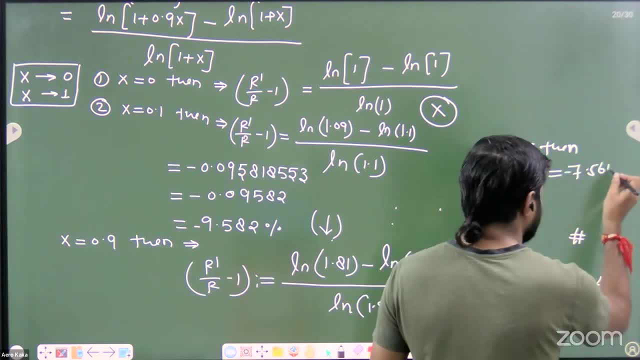 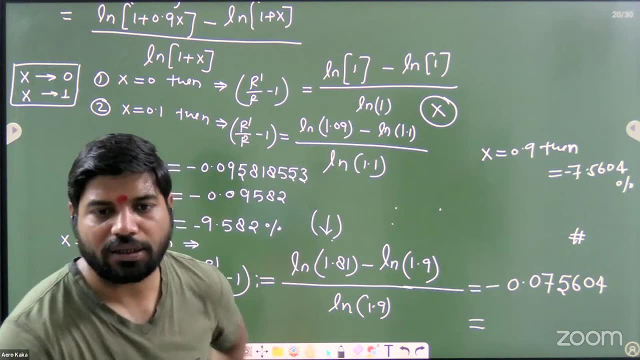 7.5604, right, Yes, So again, this is what You can say: lower than 10%. So, whether it's a jet engine aircraft, or you can say piston-based, or you can say whether it's a propeller-based aircraft, okay. 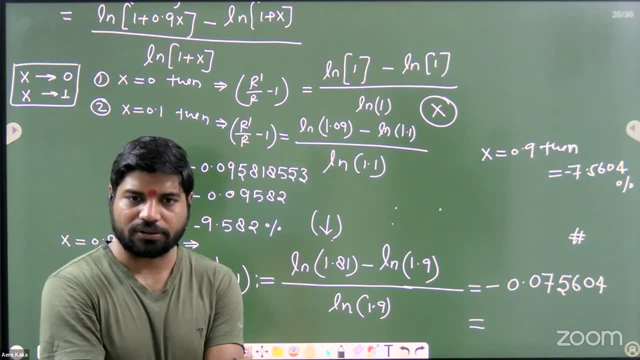 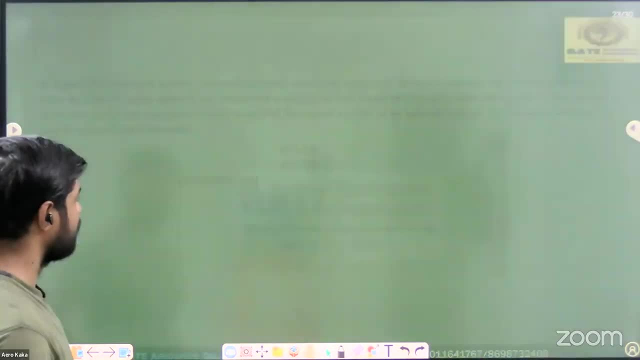 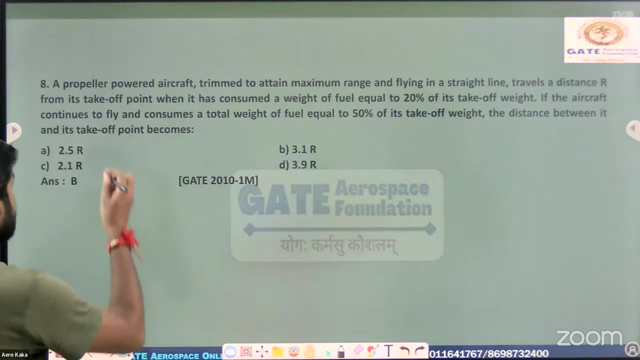 Okay, We are getting this value. These are lower than 10%. Okay, Khushi, are you getting this one? Yes, sir. Now another question, Question number eight. Now they are saying a propeller-powered aircraft claim to attain maximum range. 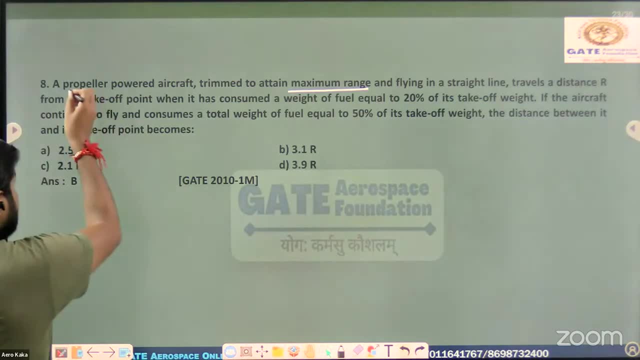 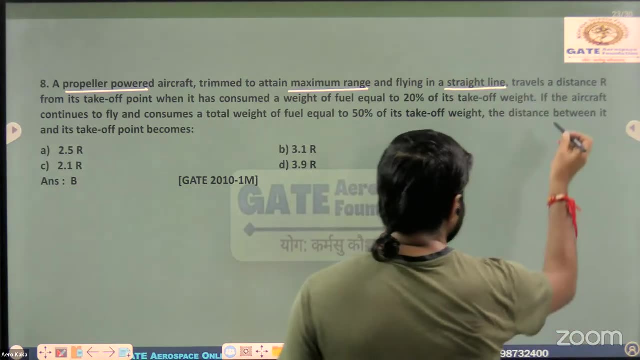 What they are saying. Maximum range: Which aircraft is this? Propeller-powered aircraft Okay. Flying in a straight line means in a steady-skating level. flight travels at this speed. So the distance capital R okay from its take-off point. 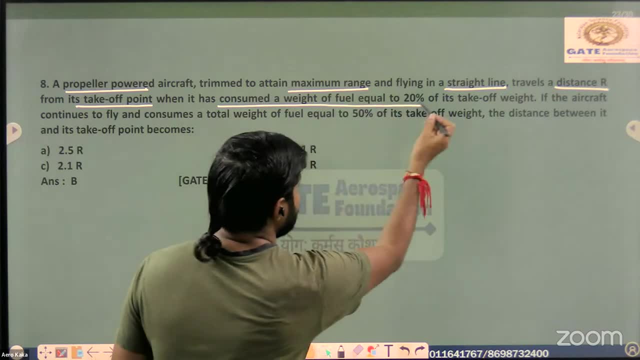 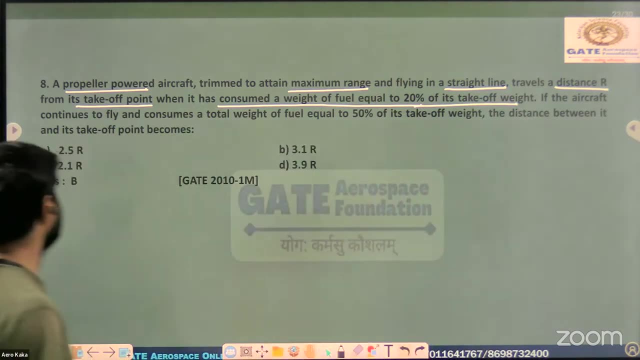 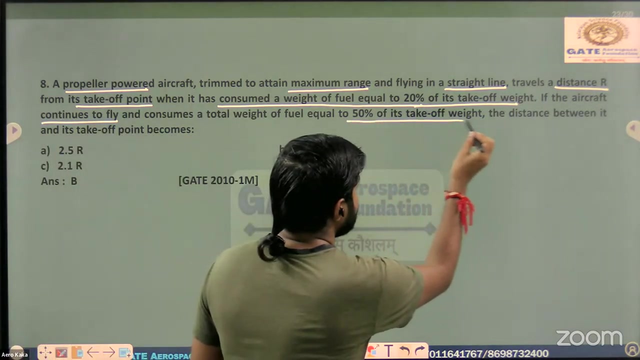 when it has consumed weight of the fuel equal to 20% of its take-off weight. Please read this question carefully. If the aircraft continues to fly and consumes a total weight of fuel equal to 50% of its take-off weight, the distance between okay? 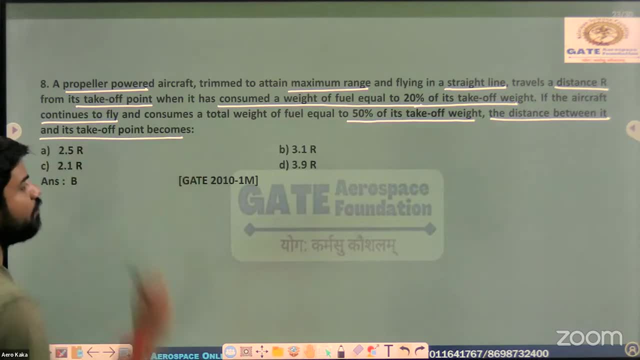 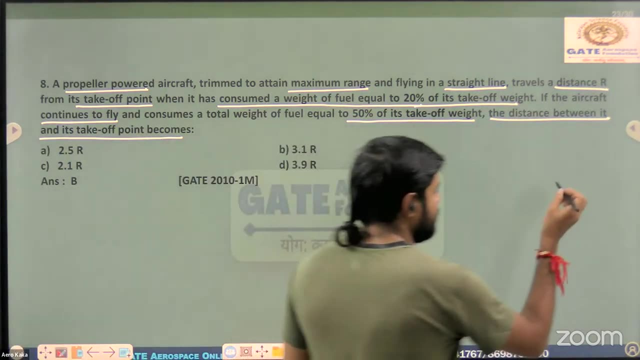 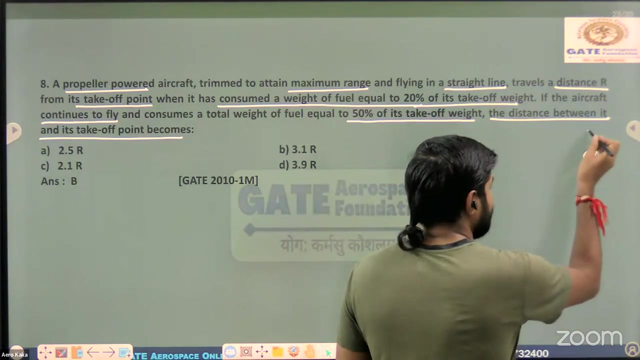 distance between it and its take-off point becomes. Try to understand this question, So better you can draw the diagram. Okay, Let's consider This is nothing, but you can say take-off point What it is. Let's consider That's your take-off point. 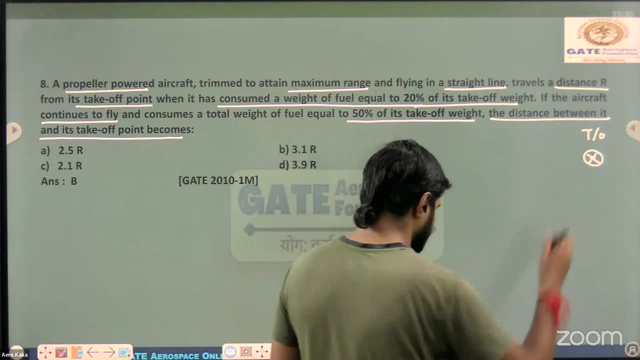 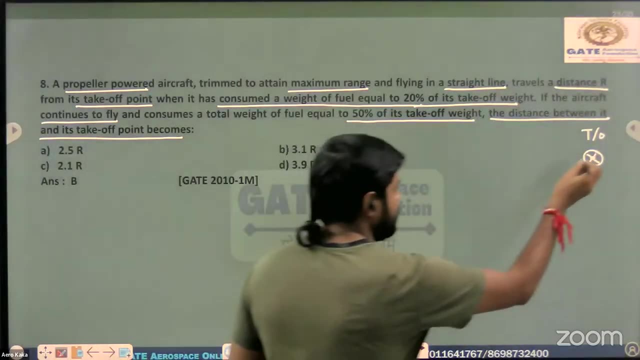 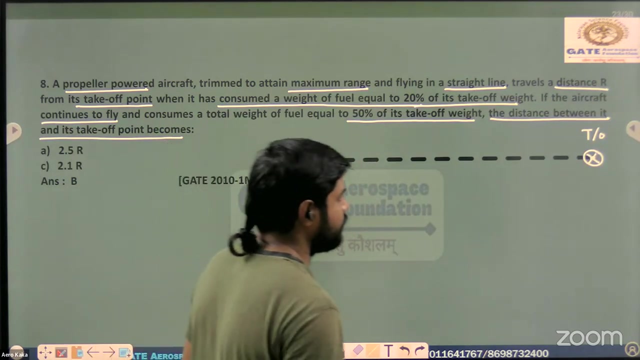 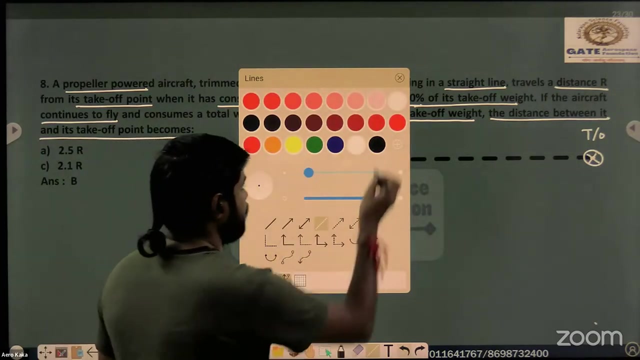 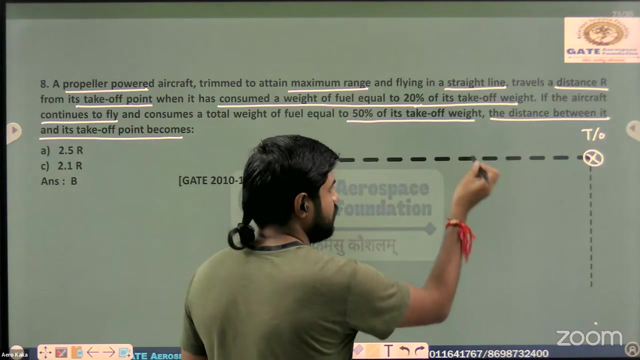 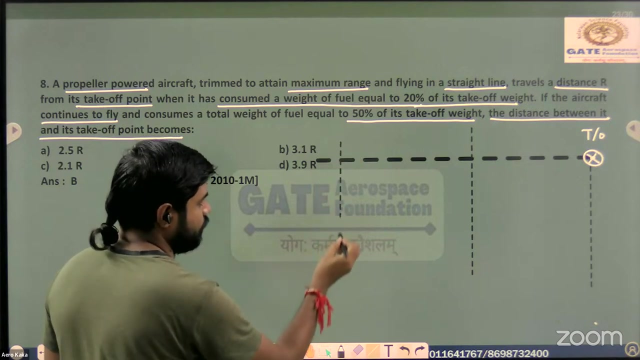 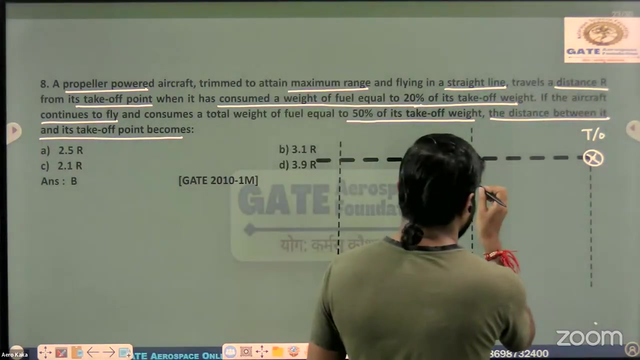 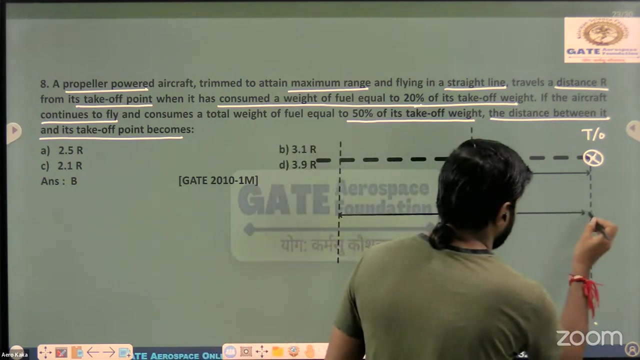 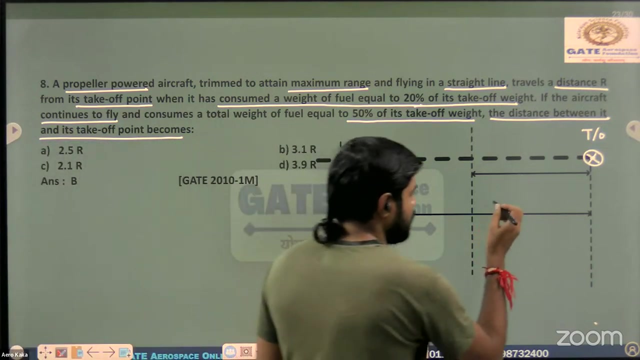 Okay, Now, let's see. This aircraft is flying in a straight line, something like this: Okay, Now, Now try to understand this question: guessing when this is capital R, when the weight of 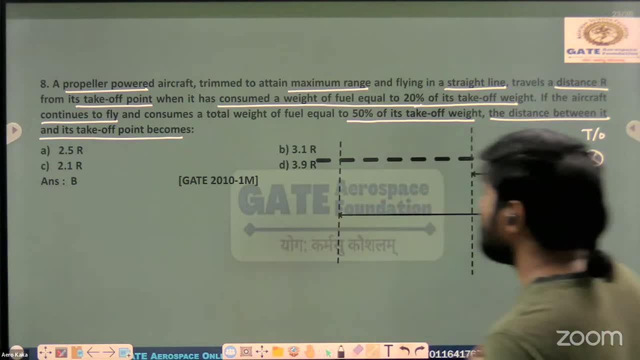 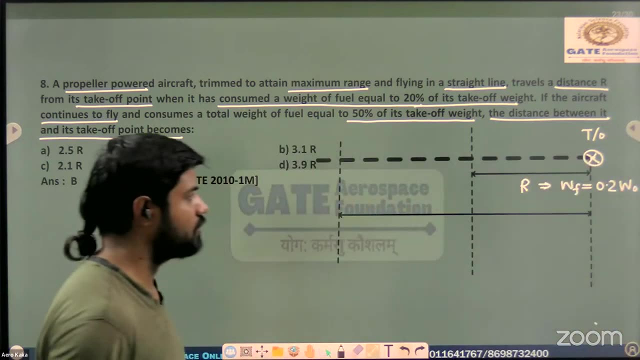 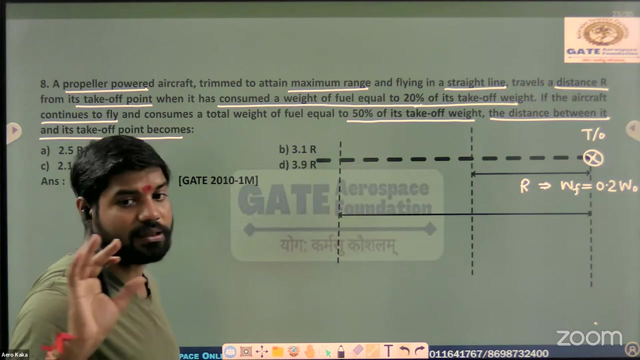 fuel consumed is how much? 20% of its takeoff weight, So 0.2 times of its W naught. Is that clear Check, please? Now they are saying: if suppose the weight of the fuel, when the fuel consumed by this aircraft is 50% of its takeoff weight, or it is initially, let's say at this point, 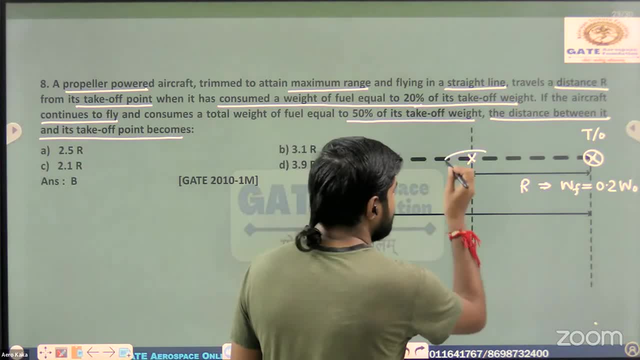 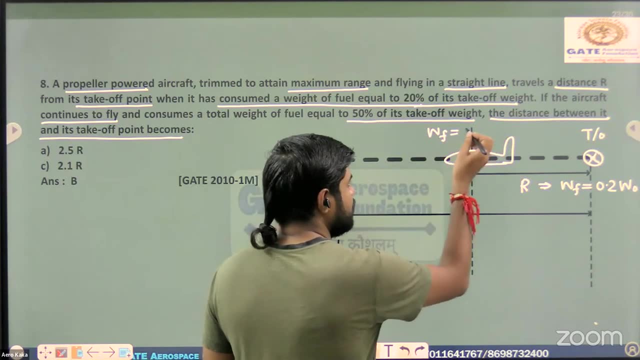 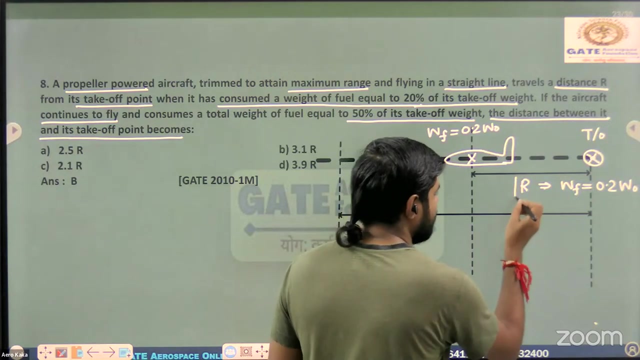 so you may consider. this is the point. okay, let's say: this is our aircraft, it is flying. so they are saying, at this point, when this weight of the fuel consumed is 0.2 times of W naught, then the distance covered by or range covered by this aircraft is capital R. Now let's say this: 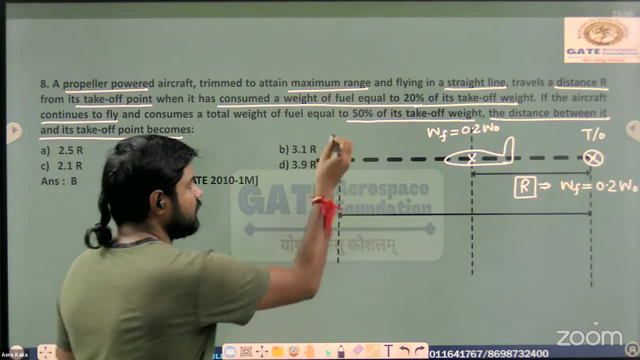 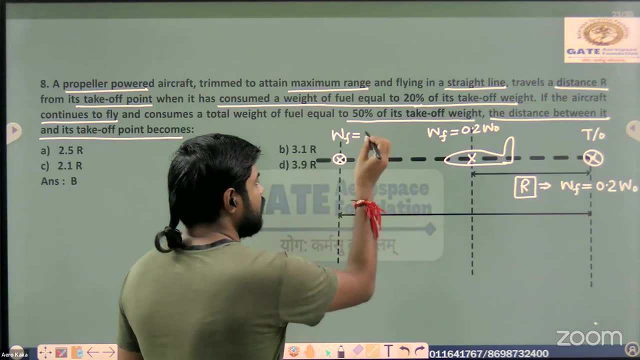 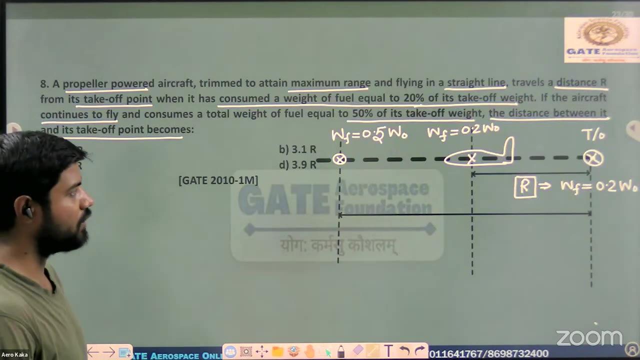 is another point. in a steady level flight, Let's say when the weight of the fuel is 50% of its takeoff. So you can write when the fuel consumed by the aircraft, aircraft is 50 percent of its initial weight of takeoff weight. then you are seeing what. 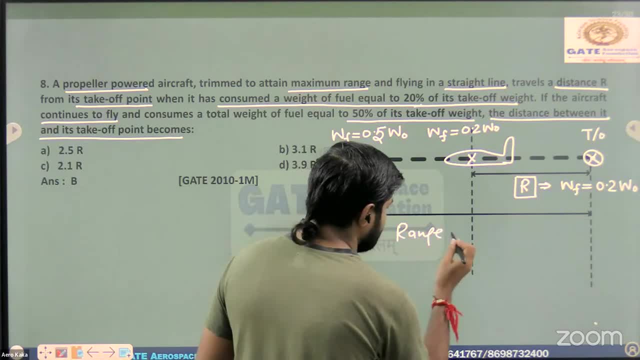 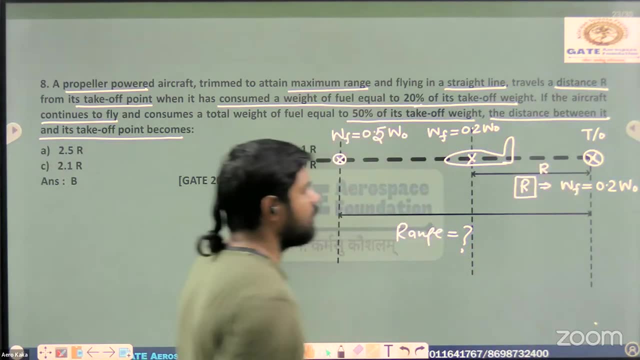 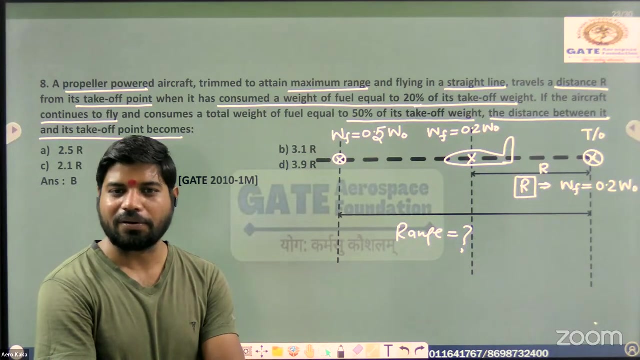 is this range here? that's what they are asking. are you getting this one? hello, Prabhuji. so what is given here? you are saying this range is capital R. so what you can do here, anyone? it's very straightforward question, right, hello? am I audible or not? yes, sir. so what is the 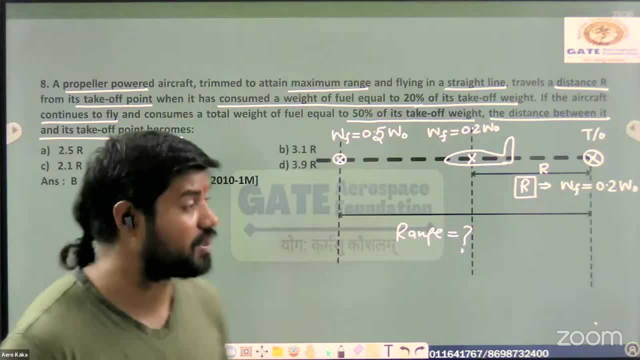 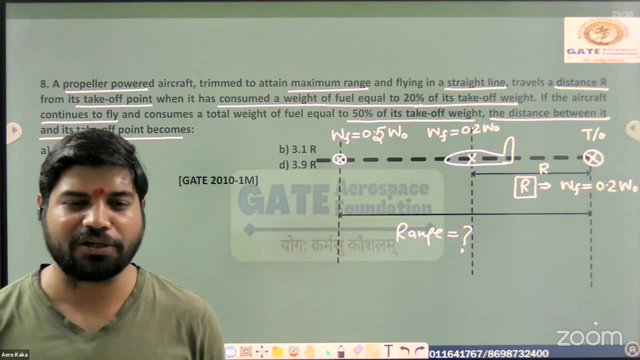 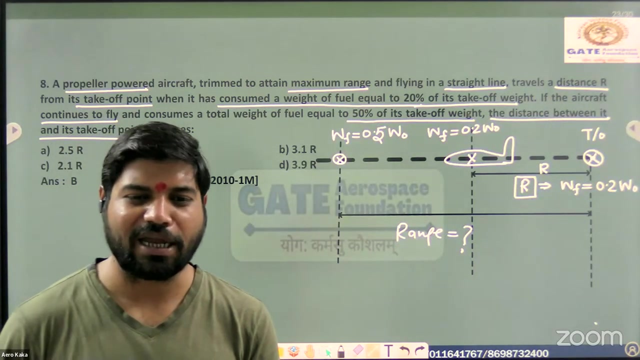 range formula for your jet engine aircraft. with which aircraft is this? it's a propeller powered aircraft. so what is the range formula? again, capital R is equal to eta p upon c. into how much, yes, c, l, y, c, d, l, n, of how much w 1 upon w? naught, please take care in your exam. 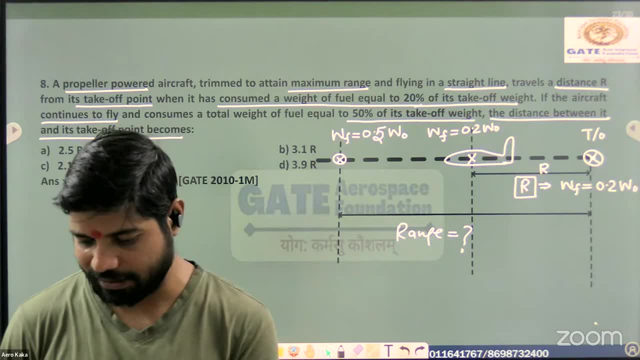 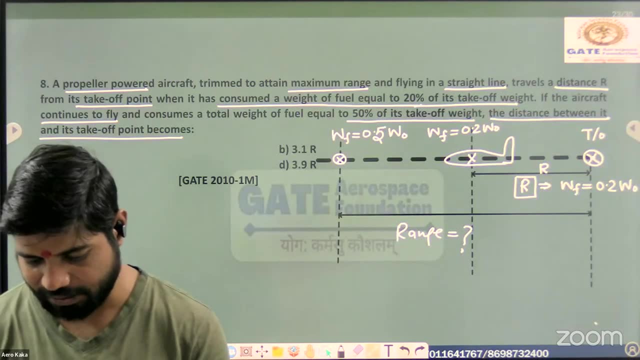 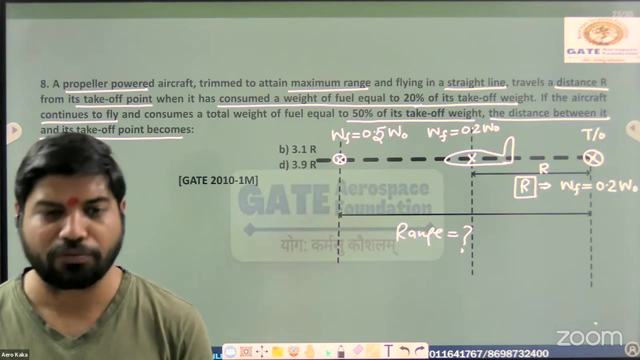 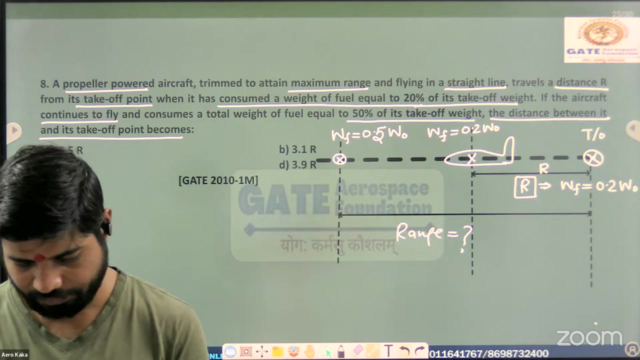 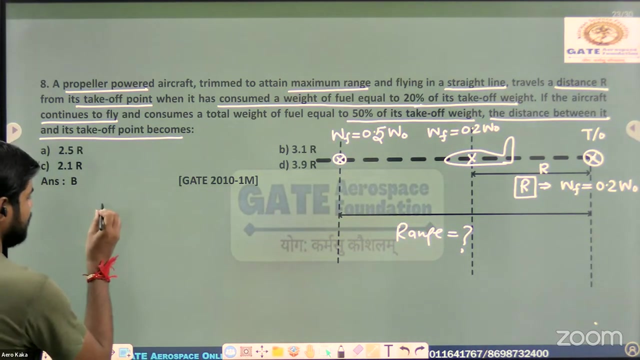 okay, exams. is that clear or not? just write down and simplify and tell me how much you are getting. which option is correct here. I think one more question is there then can we will stop. okay, it's the second last question. you, it's very easy. look: R is equal to how much propeller efficiency divided by c into l, y. 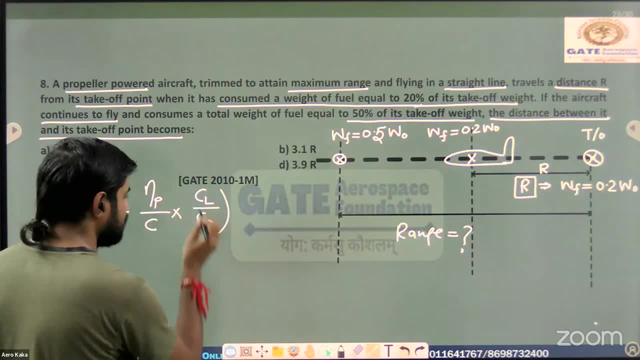 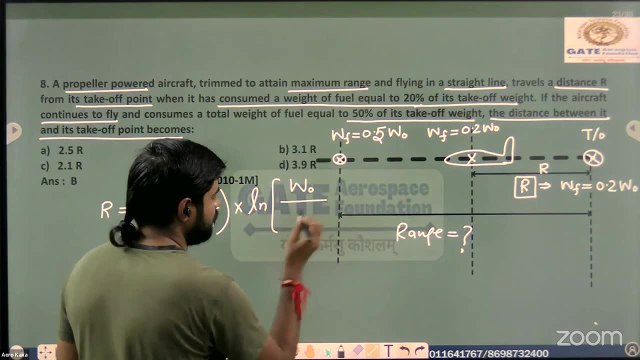 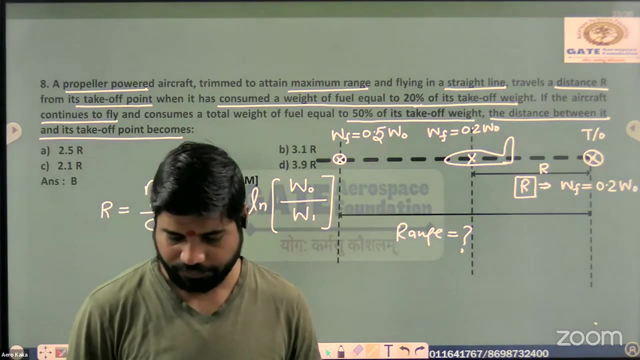 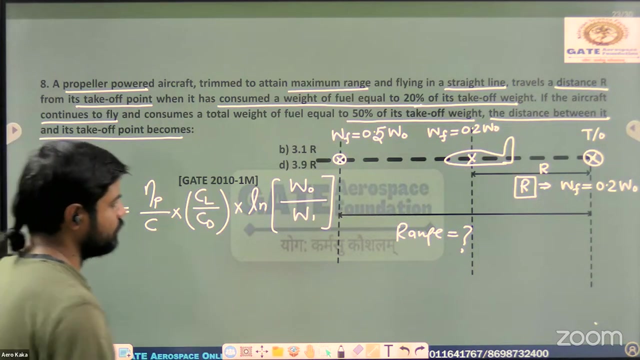 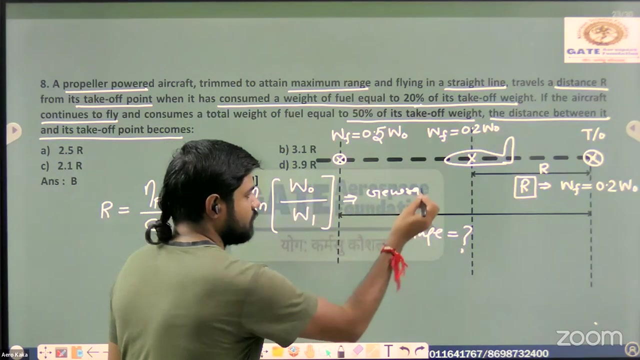 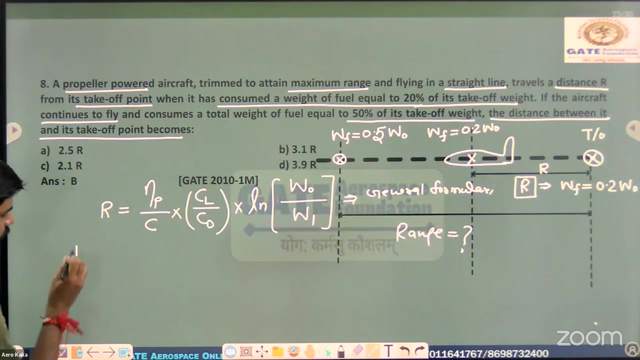 d ratio or c? l by c d ratio into how much l n of how much w naught upon w1 right check clear. So this is a general formula. okay, let's say this is our standard problem. okay, pattern case 1: what is given? let's say: 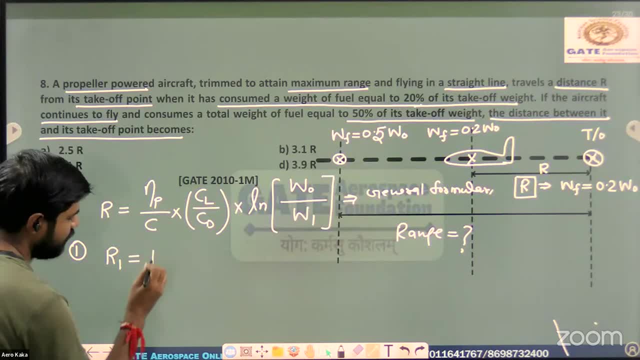 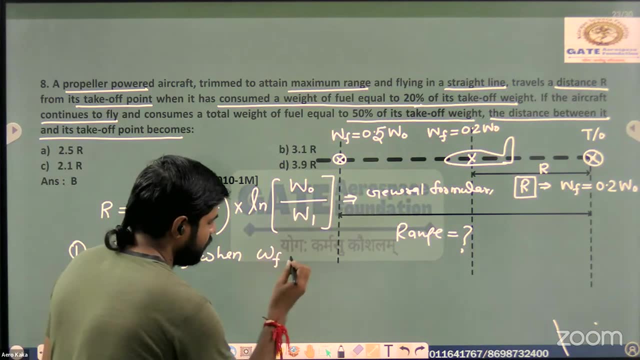 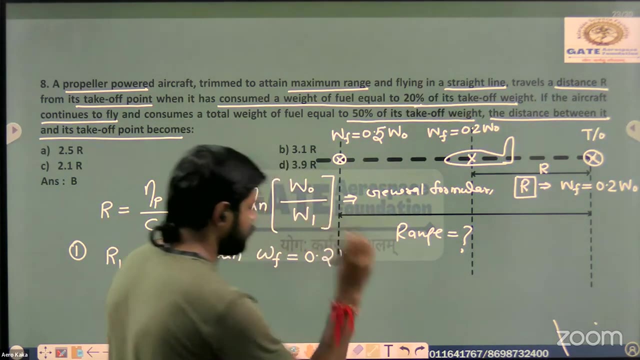 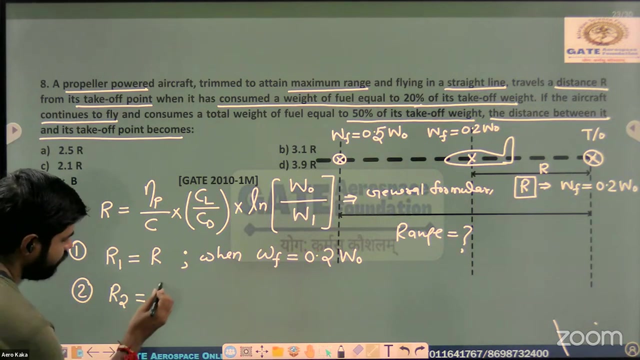 first case i am considering. let's say r1 is equal to r, when this weight of fuel is nothing but how much 0.20 percent of its initial load. right, let's consider case 2. let's say r2 is equal to. we don't know what is this when? 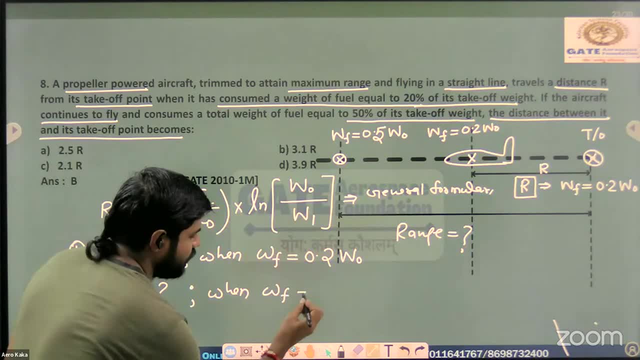 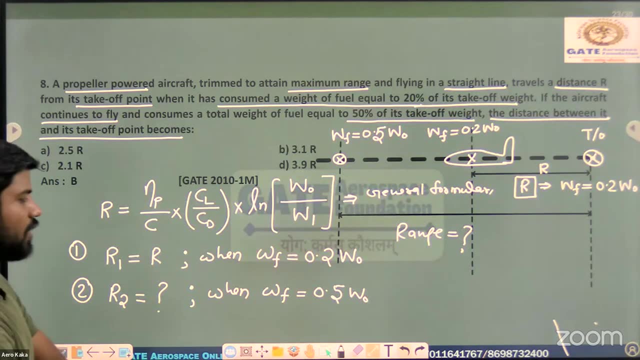 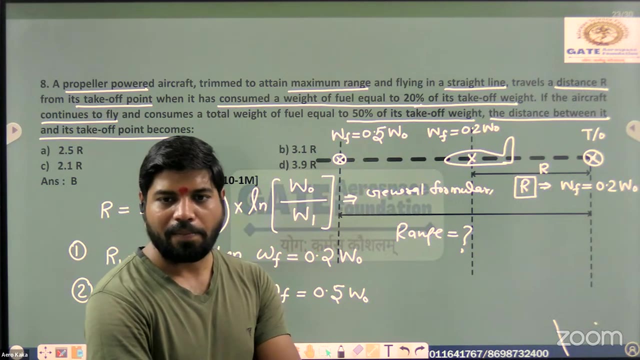 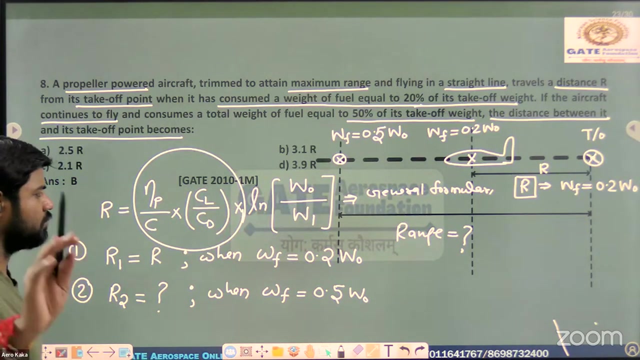 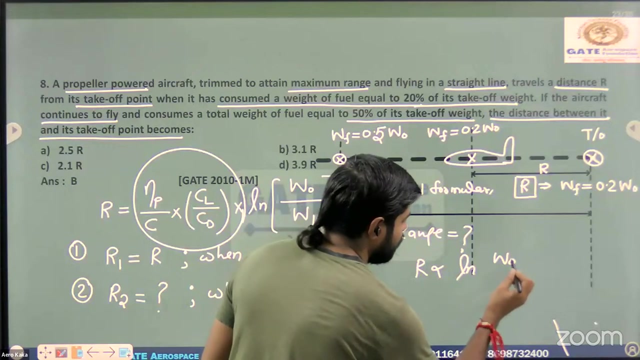 wf is how much 0.5 times out w bar what we can do. yes, anyone, am i audible or not? so from here again, you may consider c. this is a constant value. okay, so you can consider. let's say r is proportional to how much ln of w naught. 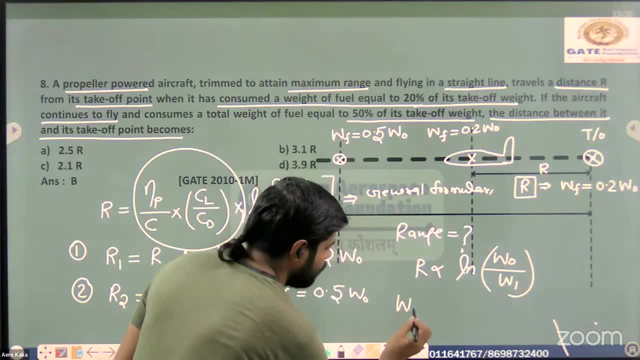 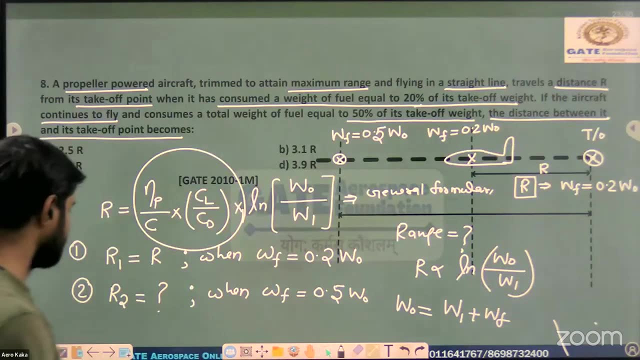 upon w1. you know very well what is this w naught. this w naught is nothing, but you can see what is this w naught? this w naught is nothing, but you can see. let's say it's a w1 plus wm. right, that's it, simplify. 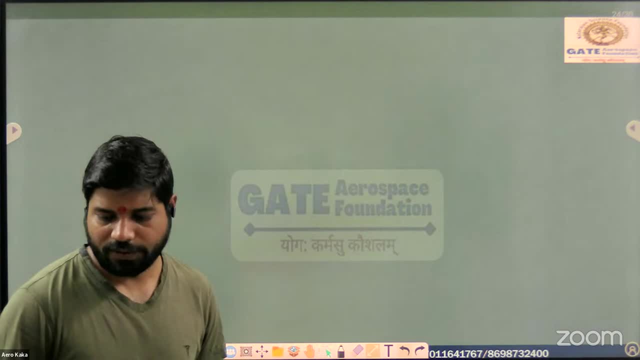 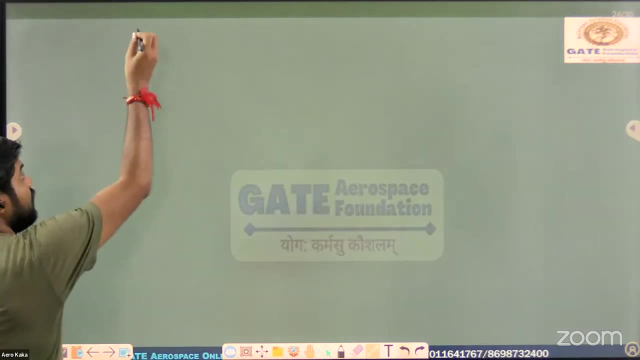 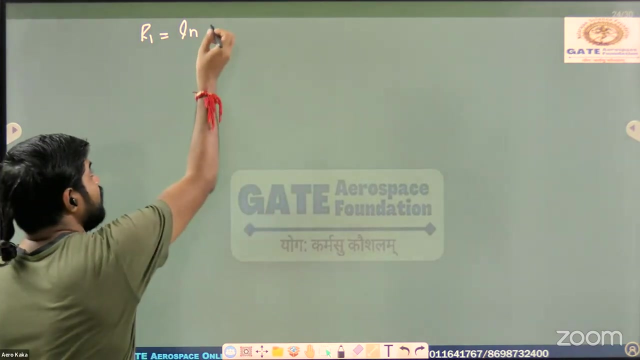 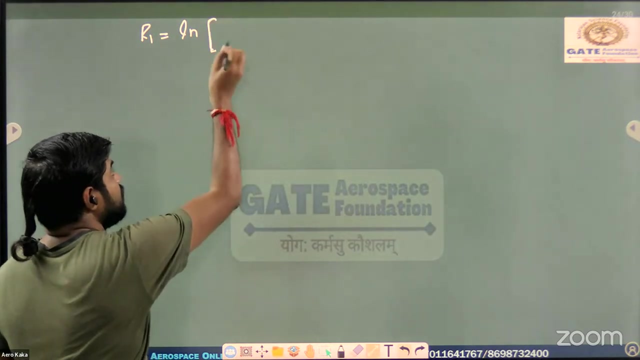 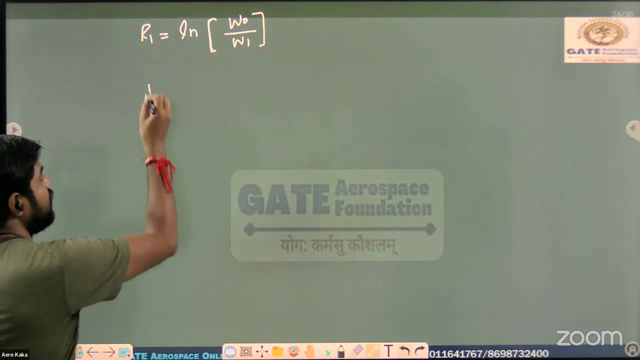 calculate. so you can write here: let's say: r1 is equal to ln of how much prabhuji, yes, please. ln of you can write it's a w01. sorry, now r2 is equal to field 2. okay, now r2 is equal to, let's say it's tutorial. 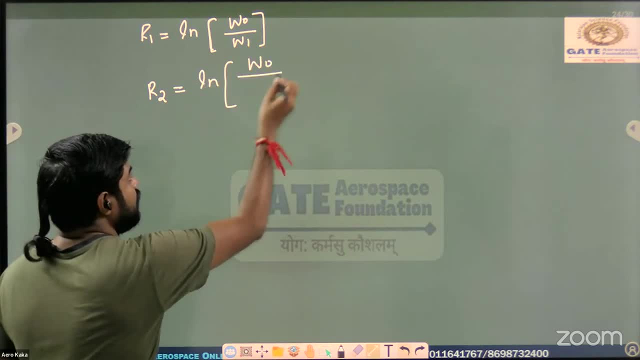 now r2 is equal to. let's say it's nothing but ln r w naught upon w 1, okay, or if you want to write this, is we no issue at all? okay, so here what you can write: this cleaning window. okay, if you are writing fx no little, where x plot kaff in terms of n, we will write this. 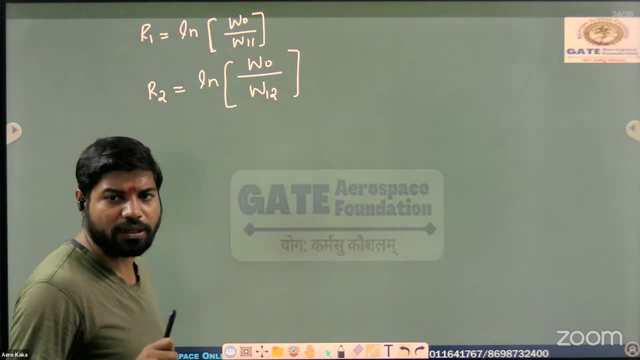 is w.12, okay. or if you want to write this, is we no issue at all, okay. so here what you can write: this is w11. or let me write here: виде be six bobby sample. and then for this, whether or not the so see that p dotness will in, it is equal to one whole point that you kство. even so, at current 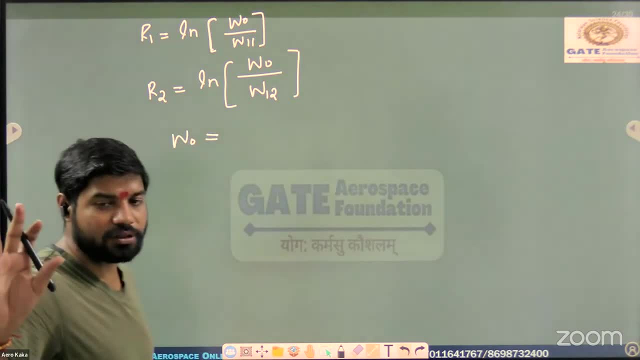 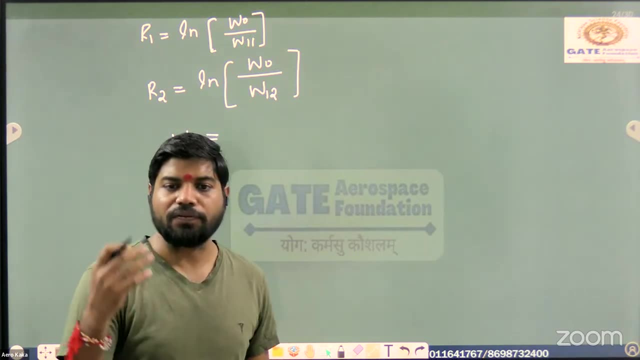 Dosson's value is the kernel value of this. two are precise, yes, but it also provides This W naught. See, the total weight is not going to change in this case. Okay, In previous case, what happens? The overall weight was changing because the fuel carried by the aircraft were 10% lower than its standard configuration. Right Here the overall weight is same. Am I audible or not? But during the flight time- obviously it's a final weight or you can say its instance weight- is keep on changing. Like how, If suppose, if you want to calculate, like, what is the weight of fuel required? 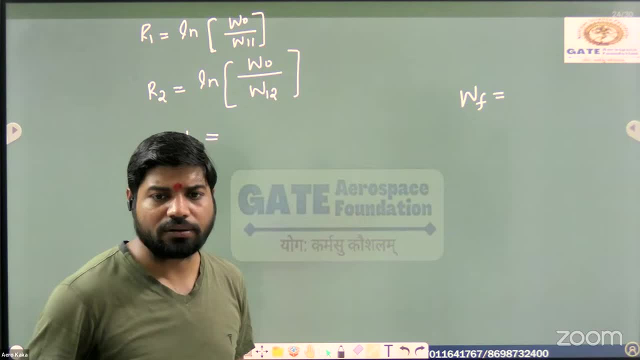 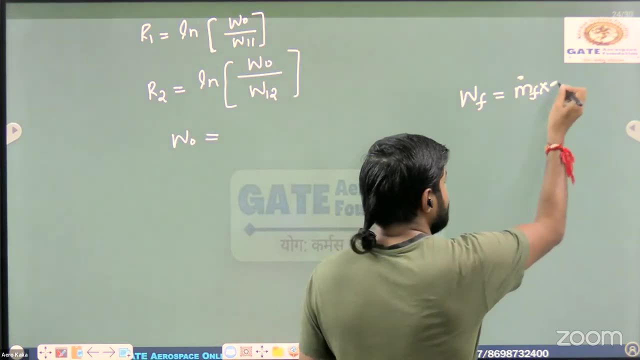 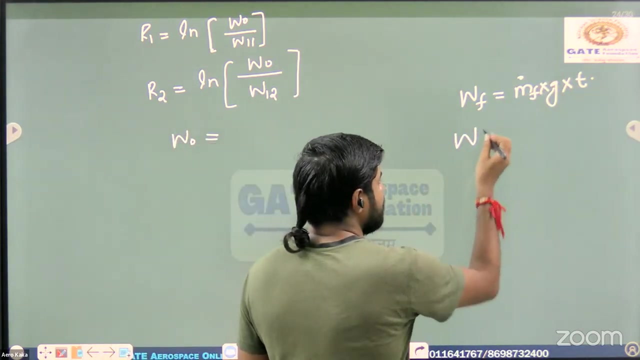 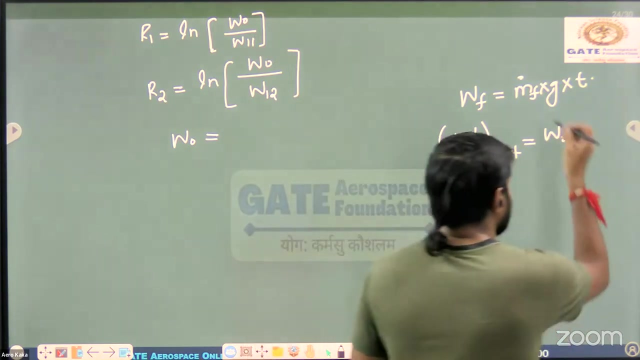 Let's say for 2 hours of flight- Okay, For flying hours. Then if you know like what is the mass flow rate of the fuel, then you can write the mass flow rate of the fuel into G, Into what? Into the time. So that's how you can calculate. Or instantaneous weight you can calculate like W. instantaneous Can you calculate anyone Is how much Initial weight minus, how much Minus this one only. Mass flow rate of the fuel Right Into G, into T. 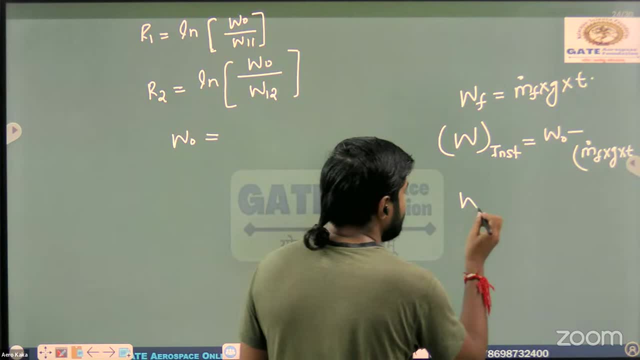 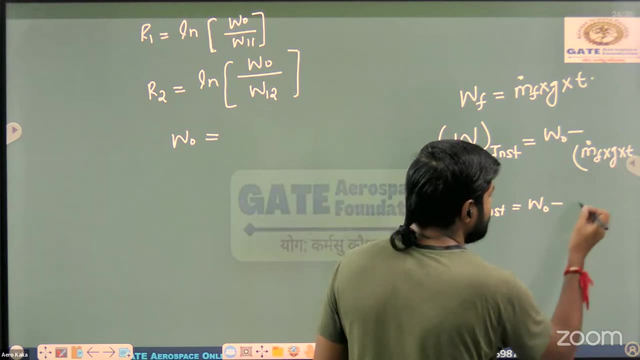 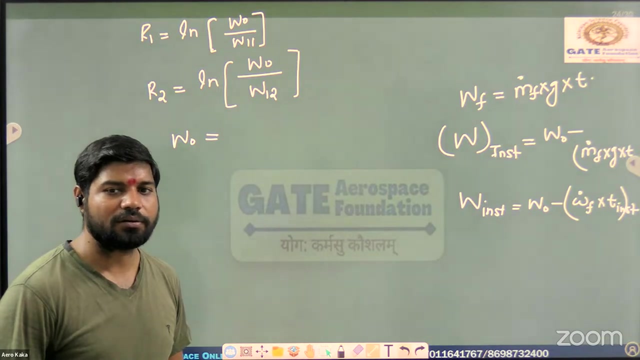 So that's how you can calculate the instantaneous weight of your aircraft: W instantaneous, which is equal to- let me write once again, W naught minus. So m dot f into G. Let me write here: It's the weight flow rate of the fuel into. you can say time, Instantaneous time. Are you getting this one? So that's how you can calculate. Am I audible? So what is the value of W11 in this case? So you can write here: 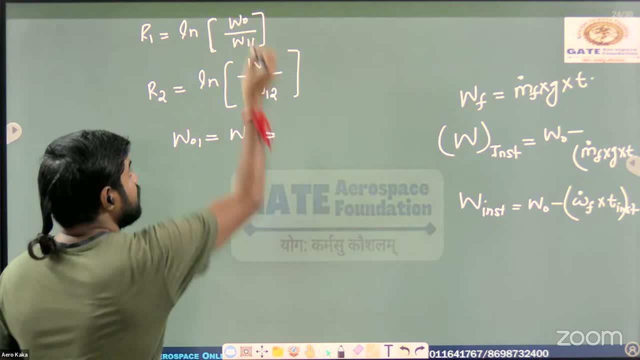 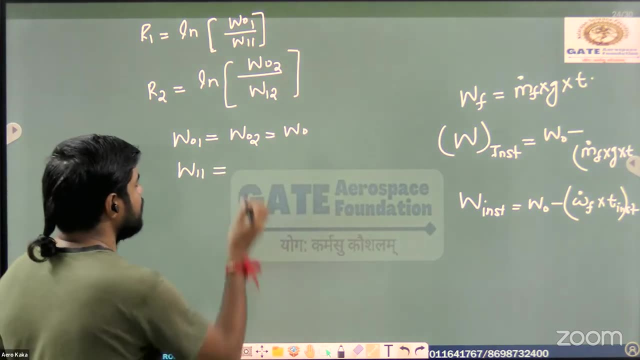 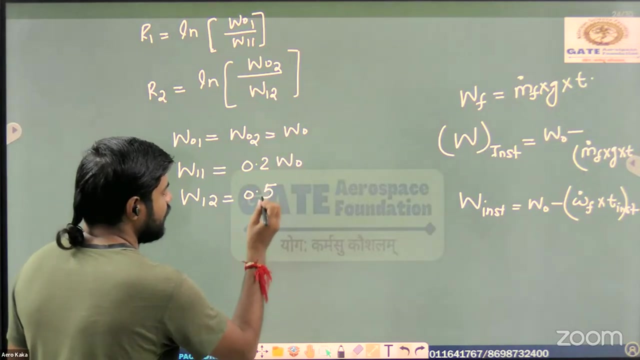 W01, which is equal to W02, which is equal to W naught. What is your W11?? The W11 is given here: 20% of W naught. It's a 0.2 times of W naught. Am I audible to you? Please let me know first. And your W12 is nothing, but you can write it's a 0.5 times of this W naught. Just put these values here. Okay, Let's say this is: 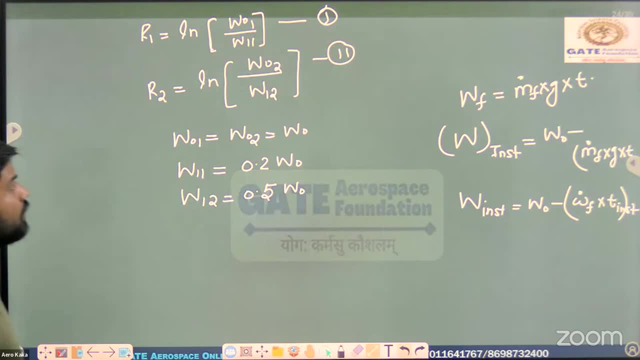 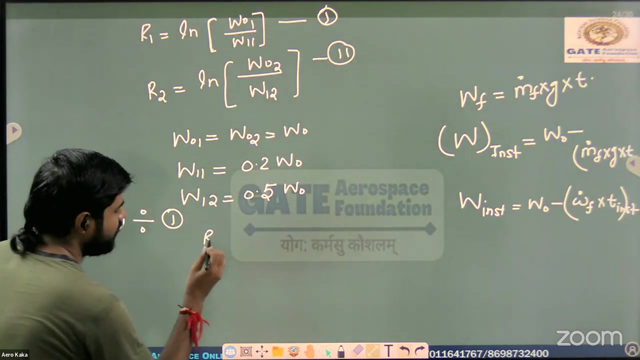 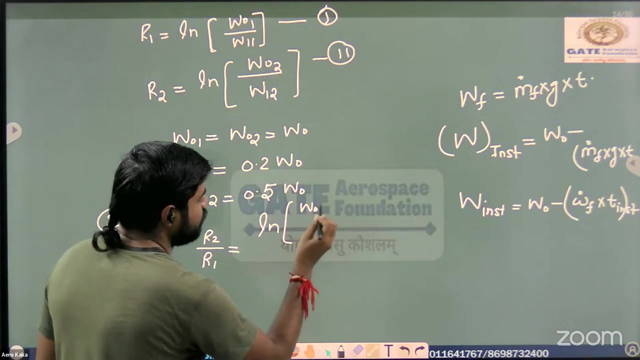 equation number 1, and this is nothing but equation number 2.. Okay, Check. So take the ratio, Let's say equation 2 divided by equation number 1.. Let me call it. How much is it? So what you can write? R2 by R1 is equal to how much ln of W02 by W12. 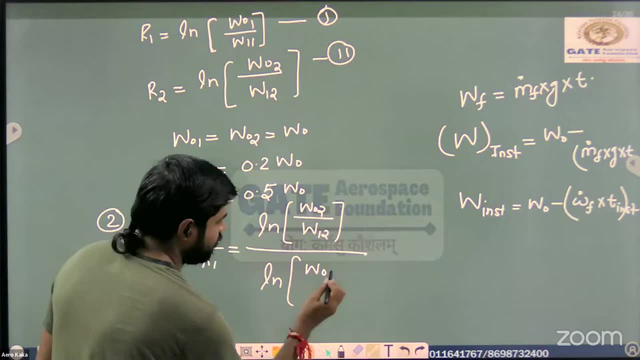 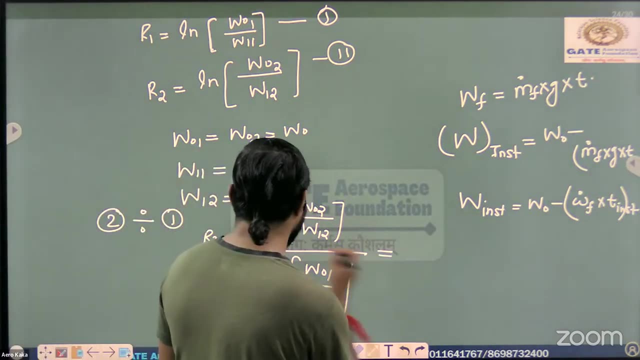 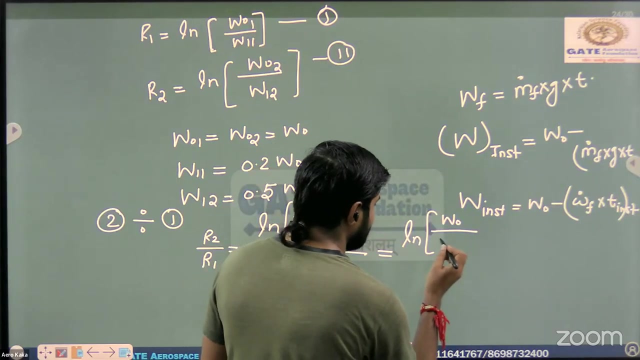 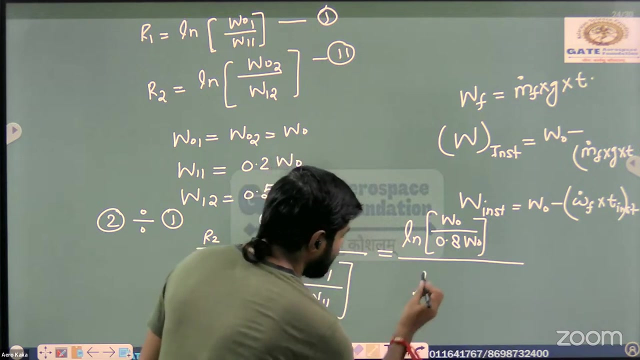 ln of W01 divided by W11.. Check please. So what is the value of W02? That's nothing, but you can say initial weight, It's not going to change. And what is W12? It's nothing, but you can say 0.8 times. Please check, Prabhuji Devi. are you there? ln of 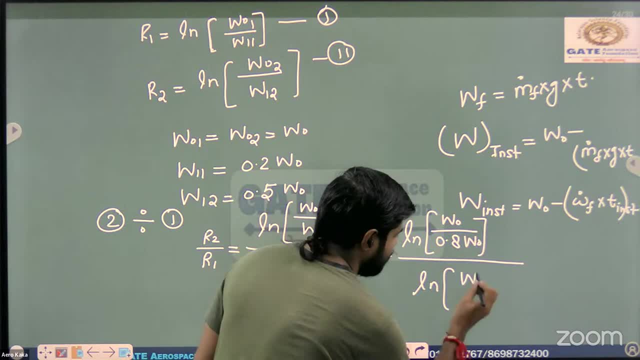 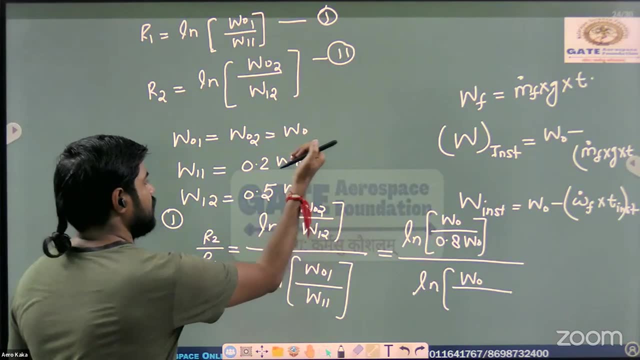 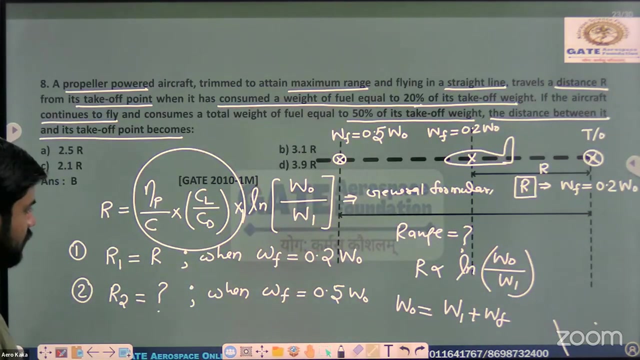 Yes, sir, Sir, what is 0.8?? What is 0.8? Where It's W11.. Just, just, just just a minute. What is given here, Wf is 0.2 times of W. naught Yeah. 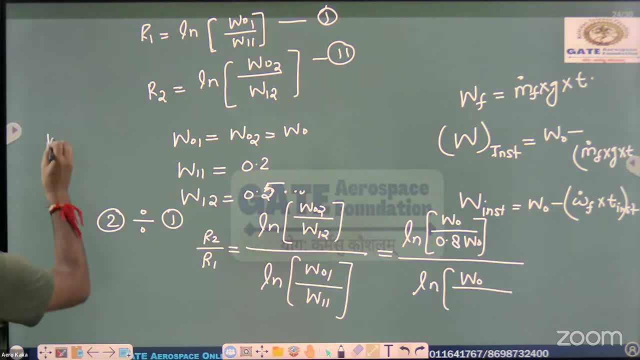 you are right. So okay, Let me write here: W11 is how much You can say: 0.8. W11 minus how much Minus how much? 0.8. 0.8. 0.8.. 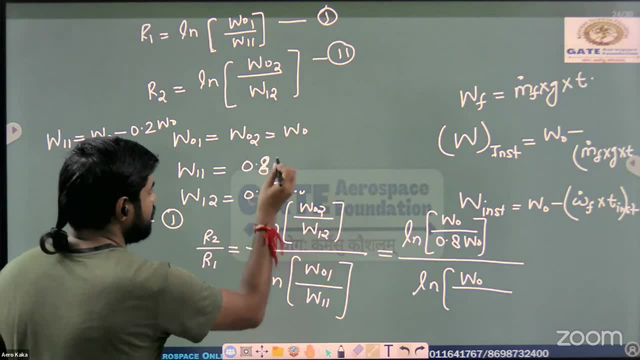 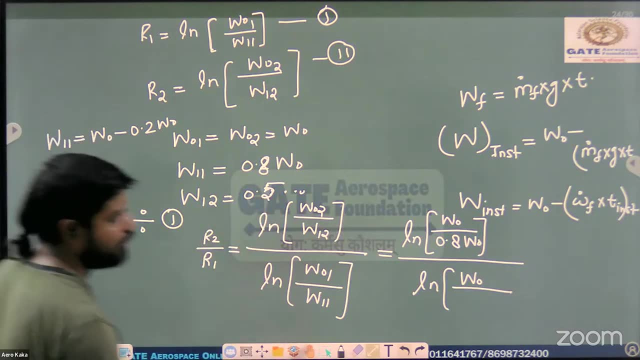 0.8.. Okay, W12,, 0.8. W0.. So it should be 0.8, right, 0.8 W0.. Okay, Then W12,. we are getting, say, 5 year. How? 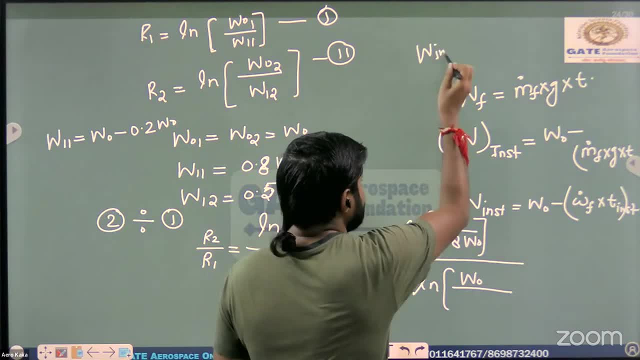 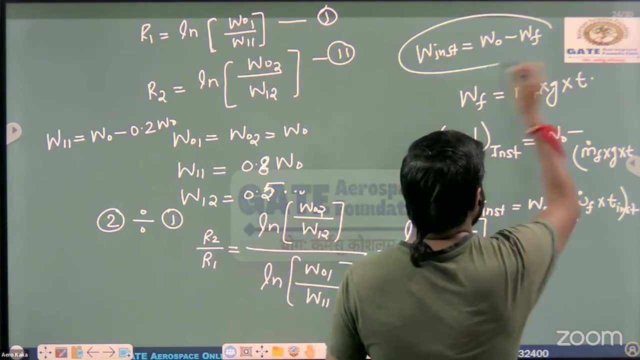 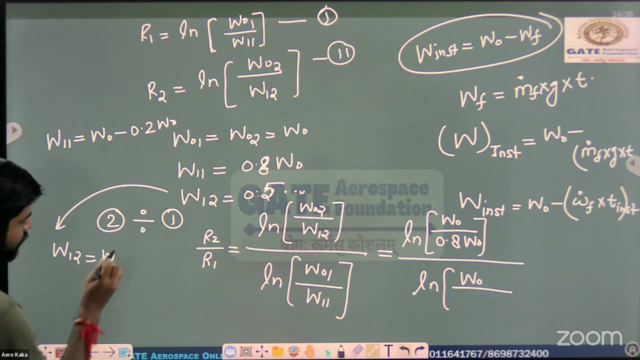 we are getting With the help of this formula, only The instantaneous weight is how much Initial weight minus weight of year? Right, That's what we are using here. So again, this W12, we are getting. W12 is equal to W naught minus how much 0.8.. 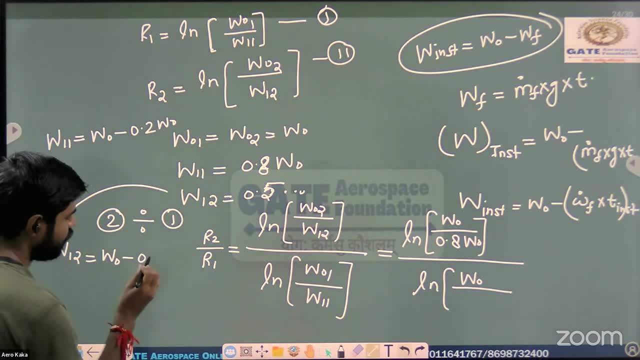 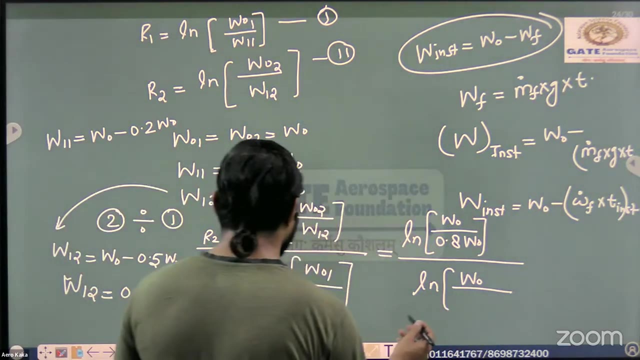 minus how much? uh, 50 percent, so 0.5 times of w naught. so we can write: w 1, 2 is nothing but how much w 0.5 times of w naught. only check w naught divided by w 1, 1 is how much 0. 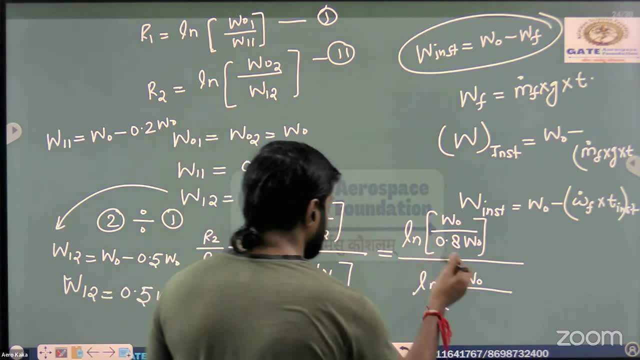 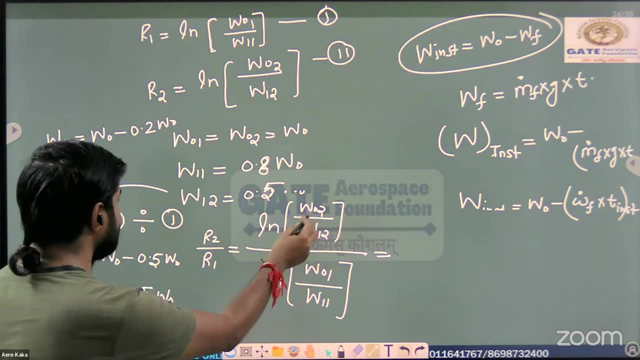 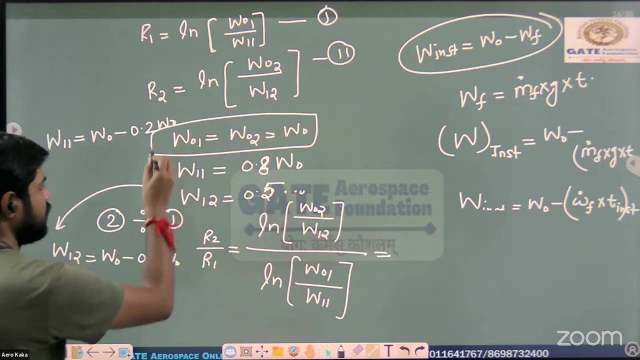 something is wrong. it should be 0.5. now look it's a r2, right. so what is the w 0, 2? w 0, 1, which equal to w 0, 2. okay. w naught w 1, 1. okay, 0.8 times of w naught w 1, 2: 0.5, okay. 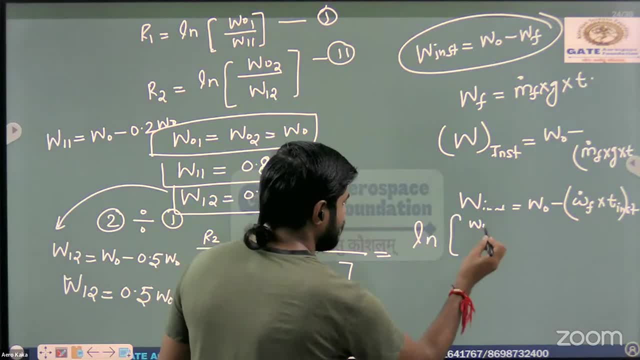 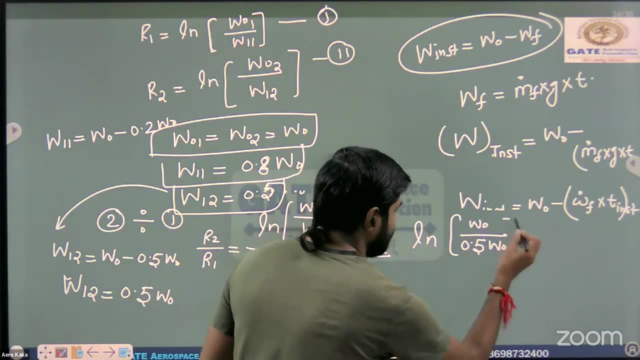 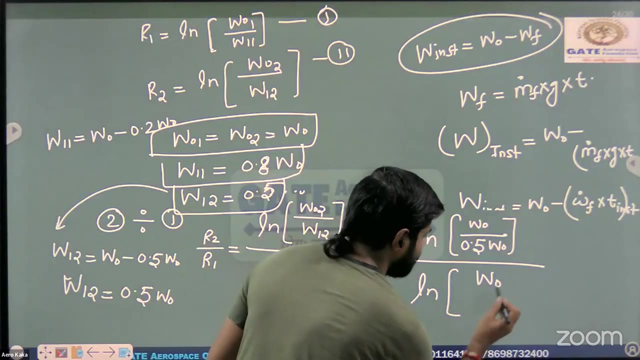 let me write ln of w naught. okay, what is w 1, 2, 0.5, right check, yes, sir. okay, divided by ln of w 0, 1 is how much w naught. only divided by what is the w 1: 1? w 1: 1 is given 0.8. 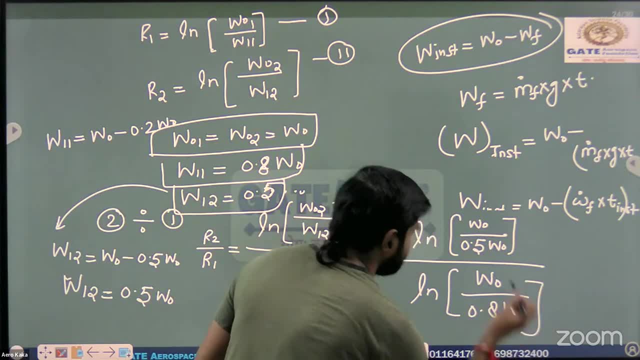 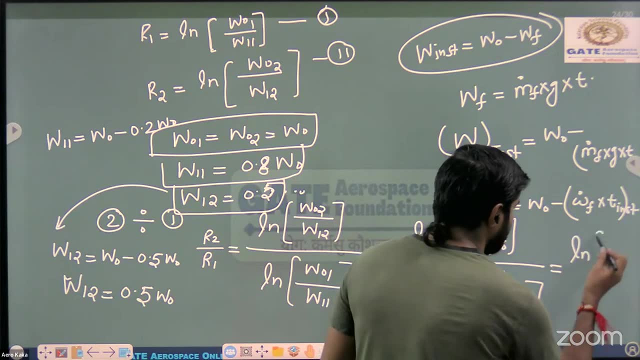 right, 0.8 times of w naught. so you have this. w naught w naught get cancelled here. also, just simplify how much we'll get here. you are getting ln of how much 1 upon 0.5, so are you getting ln? 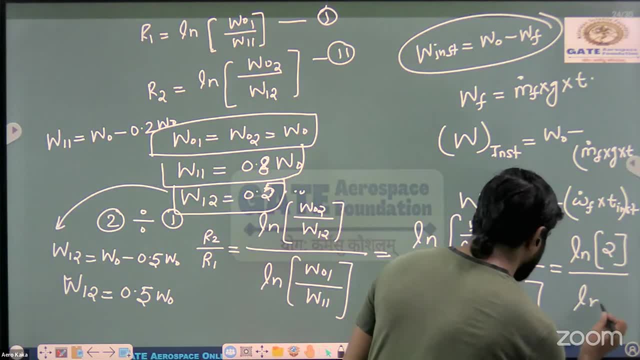 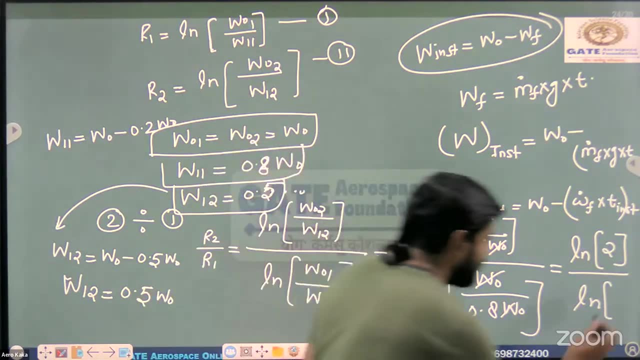 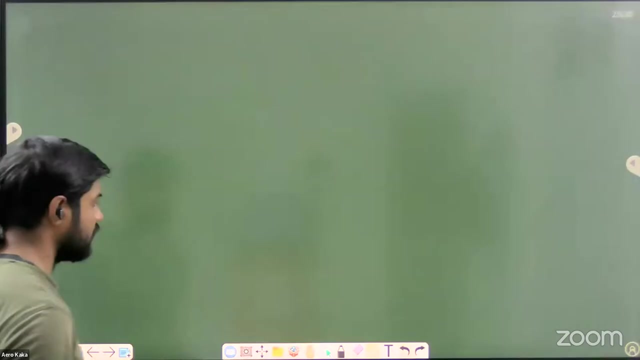 of 2, yes, please. divided by ln 1 upon 0.8, so 10 by 8, are you getting 1.25, something? yes, sir, yeah, ln of 1.25, ln of 1.25. please calculate and let me know how much you're getting. 3.106, 3.10628. 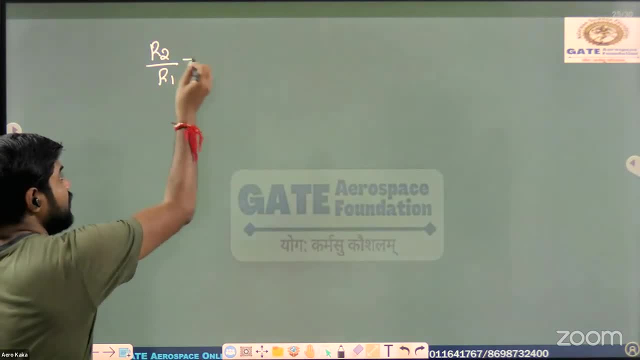 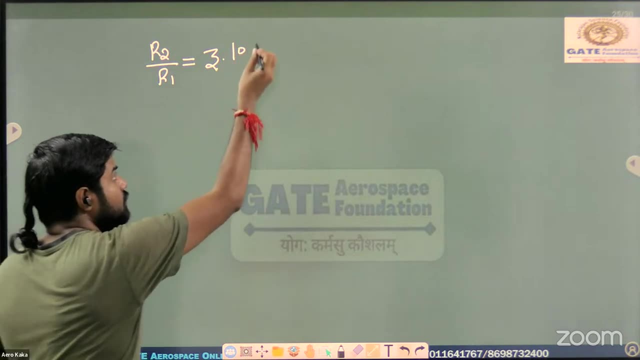 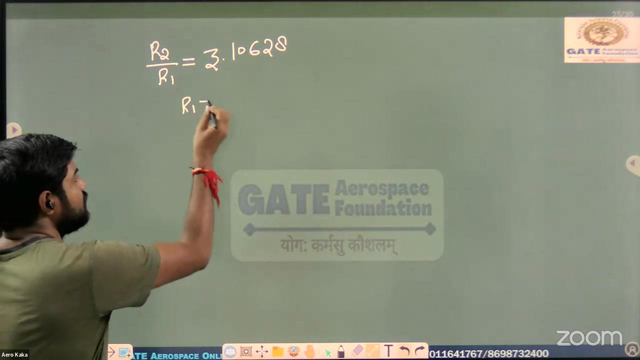 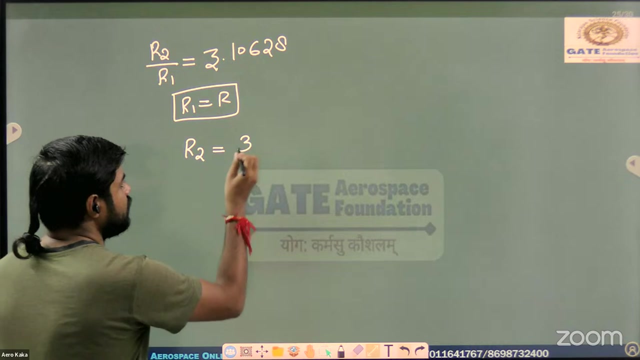 just a minute. r2 by r1, how much? you're getting 3.10628. so what? we're considering what is given here, r1. they are constantly- it's a capital r right and they are asking: what is the value of r2? so put here how much you're getting r2- ylKuH. 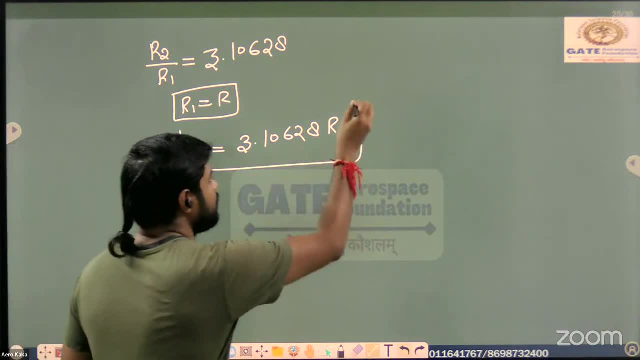 3.10628 times of w chocolate r1. what is r1? yes, sir, yes or no? check please. so what is the? u value? you're getting? r2 equal to 3.10628 times of w r1. say yes or no, check please�. So what is your value? you're getting once to r1, u t1. So how much is that? so you'll? what is your value? a, v1, so if you've got a, you call back r2 equal to what is the value of 0s and c is equal to what f and q? what is your value? aqq, yq, 30, yq, a? really learning to Number Ten for the. 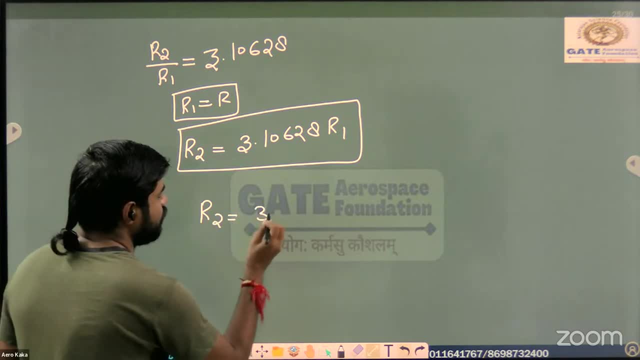 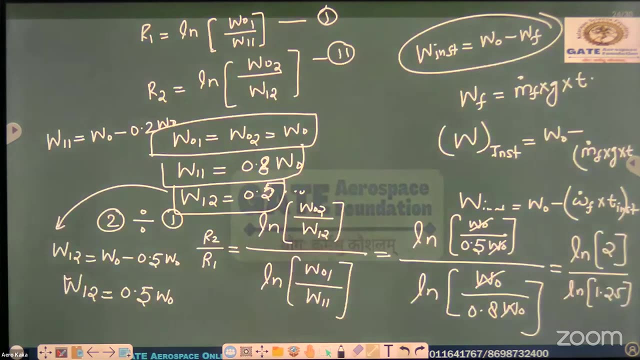 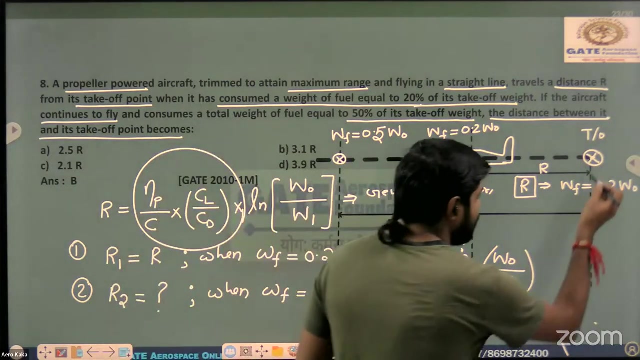 is R1. here You can write: R2 is equal to 3.10628 tons of capital. R. Please take care. You know what is the common mistake generally, student do They do not read the question properly. That is very disappointing. So they are asking: what is the distance from the initial point? 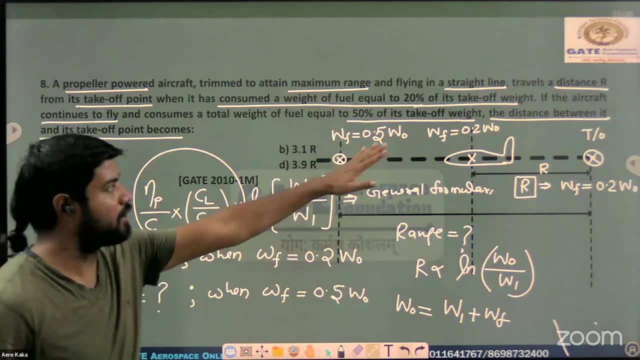 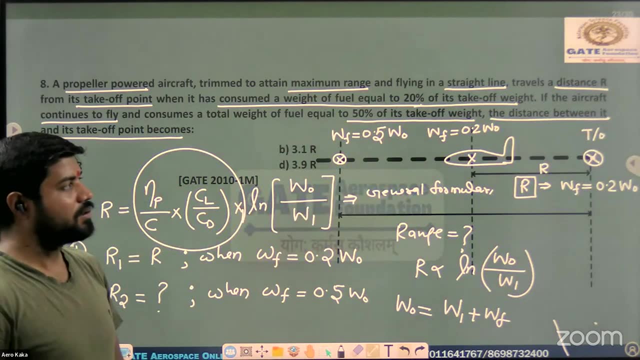 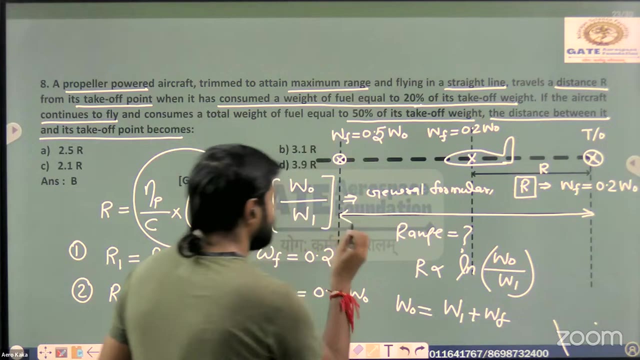 to the point where the weight of fuel is consumed, like when the fuel, when the total weight of fuel equals to 50% of its takeoff weight, or you can say overall weight of the aircraft. So they are asking this distance and you know this option is also given in this question. 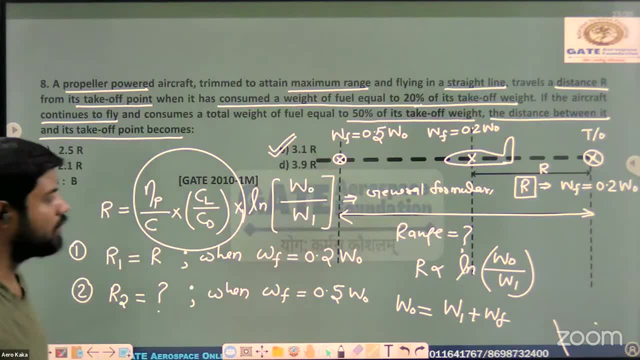 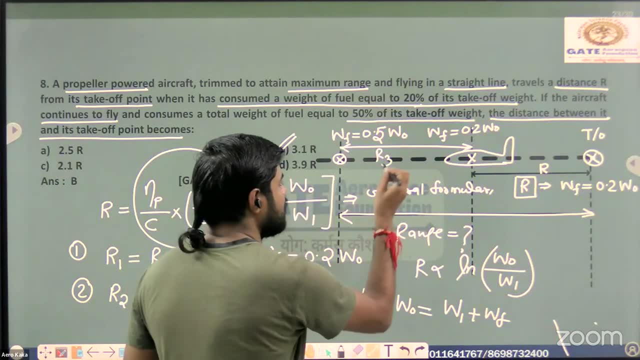 So which one is correct? T.1R. But you know, sometimes students get confused and generally they consider this distance also. So what is this? Let us say it is a R3.. So what is the R3?? You can say this is the range, or you can say distance covered by the aircraft when. 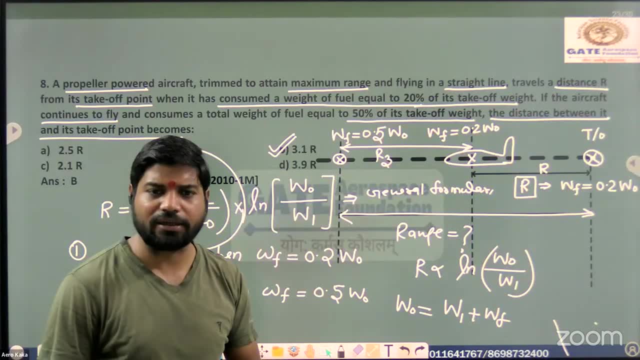 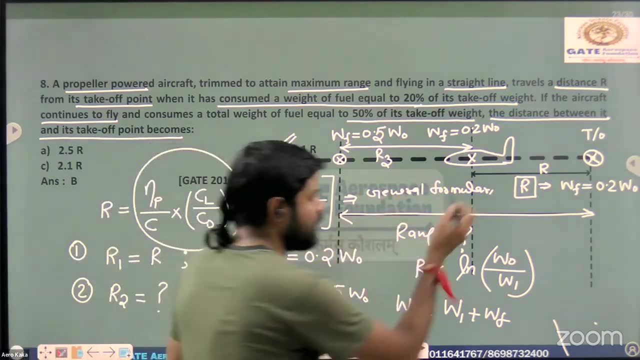 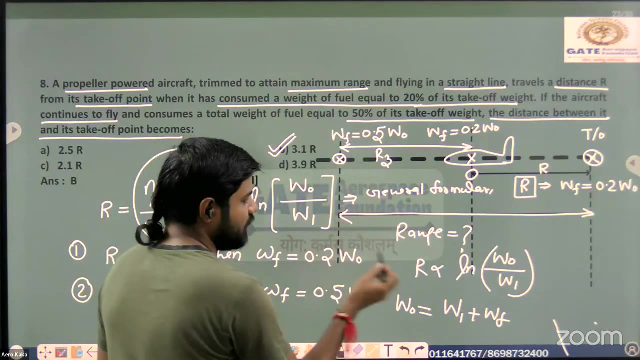 the first reading, First taken by the pilot. Is that clear? And this is the second reading. Am I audible or not? So at first reading the distance covered by the aircraft was how much Capital R. At second reading, when you are considering it is a 50% weight, then you are getting it. 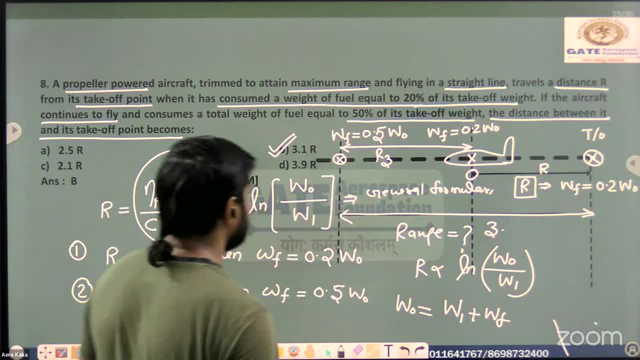 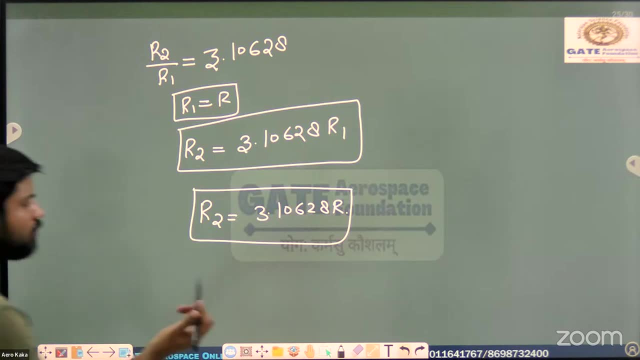 is a three point. You can write here: It is a three point. Are we getting correct value or not? How much are you getting? 3.10628.. So if you want to write up to one decimal point, let us say if you want to write. 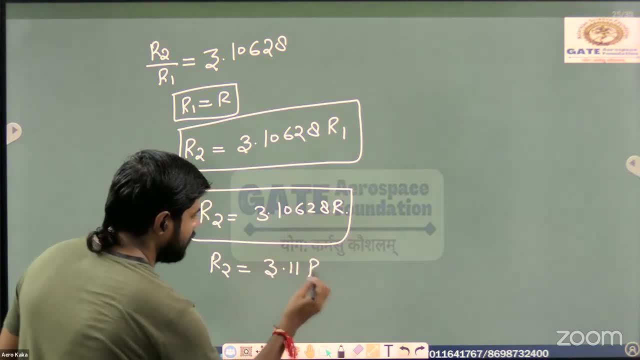 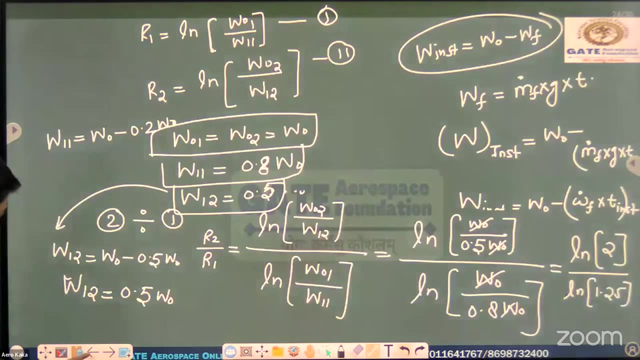 Up to two decimal point and you can write it is a 3.11R. Up to one decimal point, R2 is equal to 3.1 capital R. So let me show you in this diagram. So this R2 you are getting 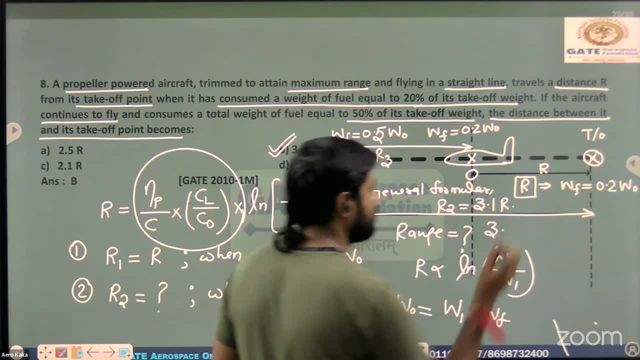 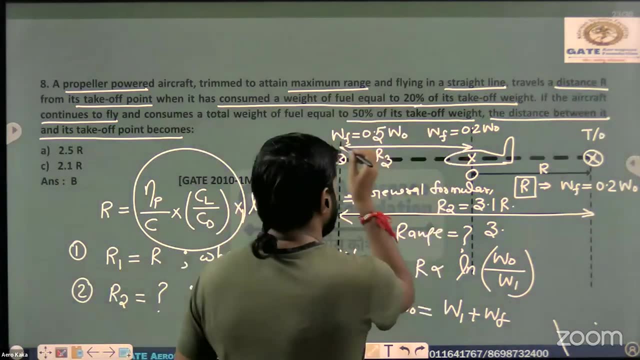 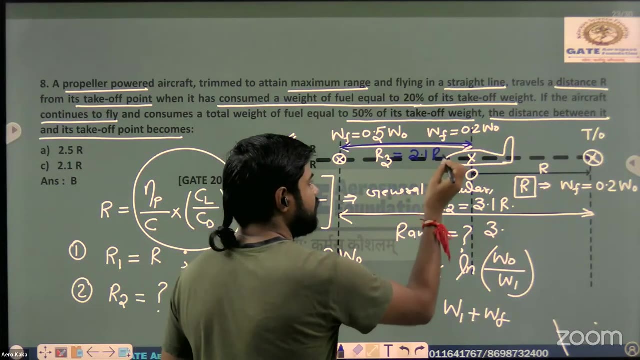 how much, 3.1 times of this capital R, Right. So what is this distance? 2.1R. So this option is also given in this Right. R3 is how much It is a 2.1 capital R. Take care of this one, Okay, So the correct option. 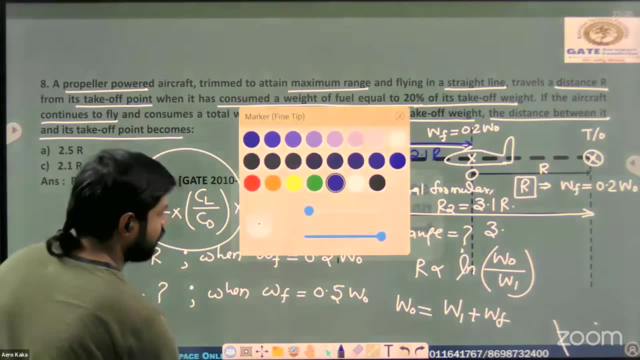 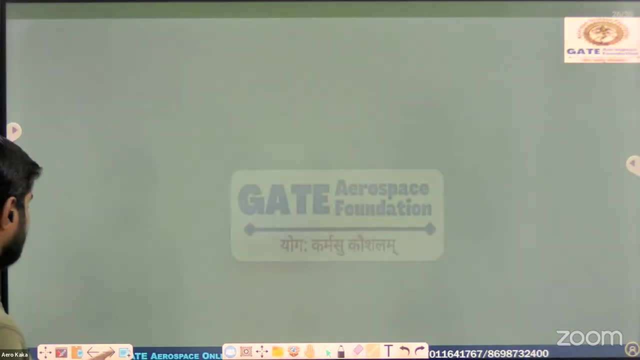 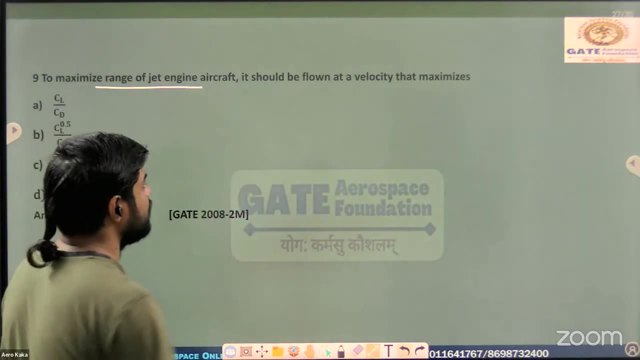 here is option B 3.1R only. That is the last question. To maximize range of jet engine aircraft, it should be flown at a velocity that maximizes the jet engine aircraft. first, C-L by C-D ratio. Second, C-L raise power 0.5 upon C-D meaning. 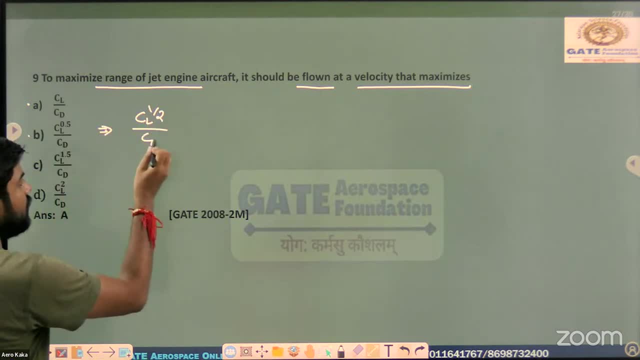 what? It is nothing, but it is. C-L raise power 1 by 2 upon C-D, only Okay. Then C-L raise power 1.5 upon C-D and C-L raise power C-L square upon C-D. Which option is correct here? 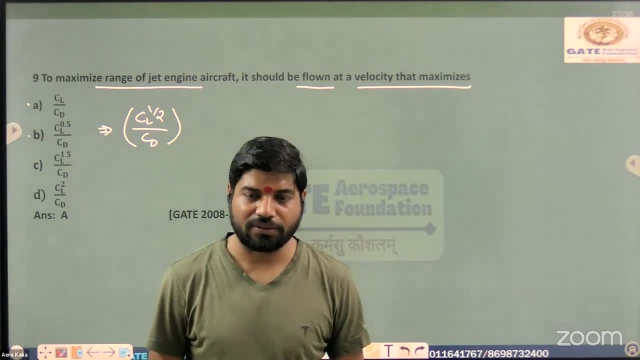 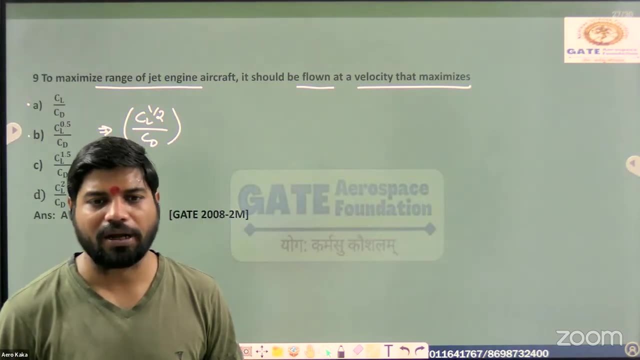 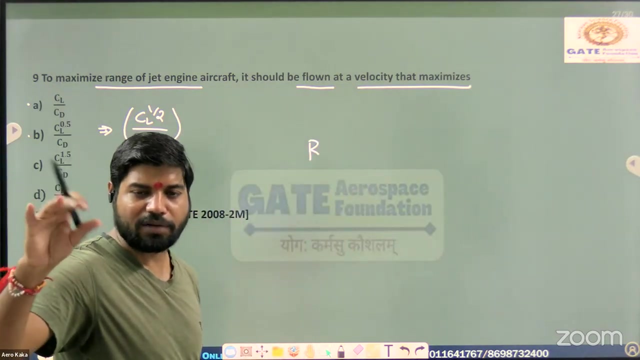 Which option is correct? B- Which aircraft is this? It is a jet engine aircraft, Right, Hello. So what is the range formula for this jet engine aircraft R 1.5.. What is the range? no, no, tell me in terms of cl upon cd terms. what's the length for?